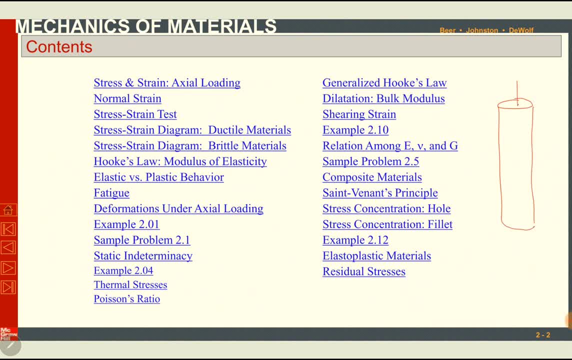 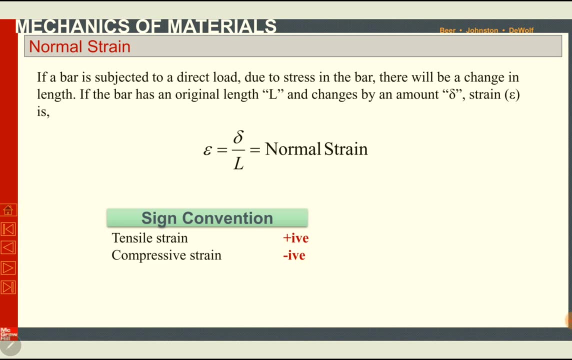 the centric axis. it is called axial load. this load passes through the centroid of the member. the member can be round or cylindrical, or it can be square. it can be any other shape. okay, before that in the first basic topic is normal strain. in the first chapter we have already discussed about stresses. now we will. 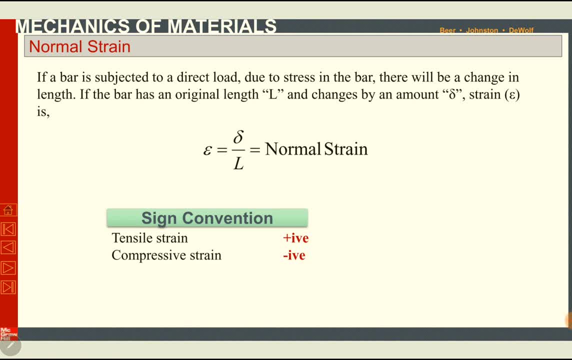 discuss about strains and deformations as well. normal strain is caused due to normal load. if a bar is subjected to a direct load due to stress in the bar, there will be a change in the length. if the bar has an original length of L and it changes by an amount Delta, the strain will be Delta or L for. 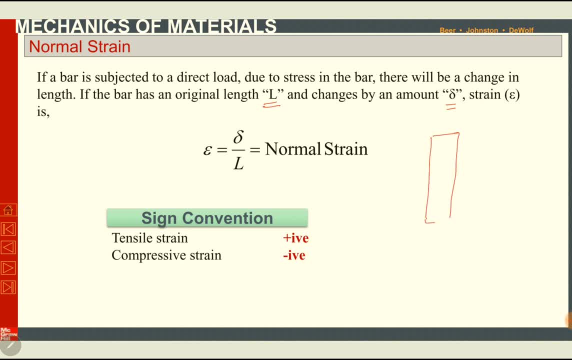 example, if I have a bar and it is fixed from an end, for example, there is a load P- if the initial length of the bar is delta L and after the load it is extended by an amount of delta, this is a positive change. this is an increase in length. it can be a decrease in the length as well. so this: 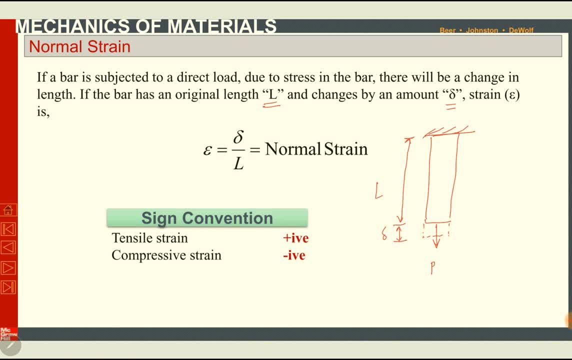 change in length. delta divided by original length, it is normal strain. delta is deformation, remember it. it is change in length and strain is ratio of change in length divided by the initial length. so strain has no unit, while deformation will be will have a unit of length. it can be meter inch, millimeter, foot or whatever. so if this load p is compressive instead of 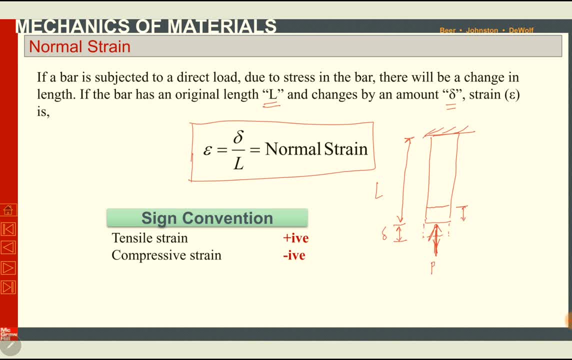 tensile. so there can be a negative delta and the strain will be negative. so if the strain is tensile, it will be positive. it is compressive. it will be negative due to tensile strain. we have a increase in length and you have to compressive strength. we usually get decrease in length, okay. 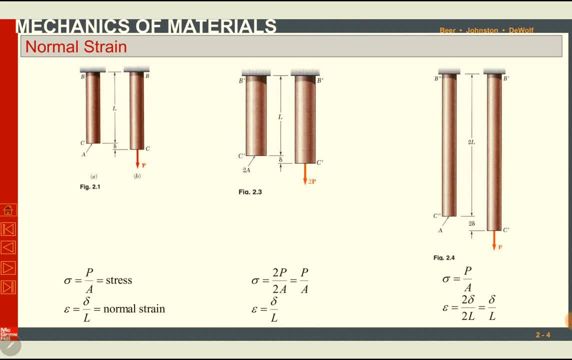 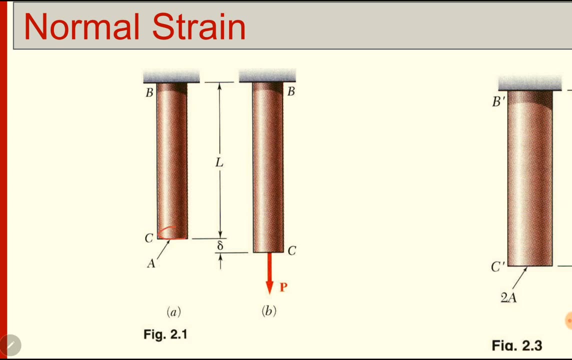 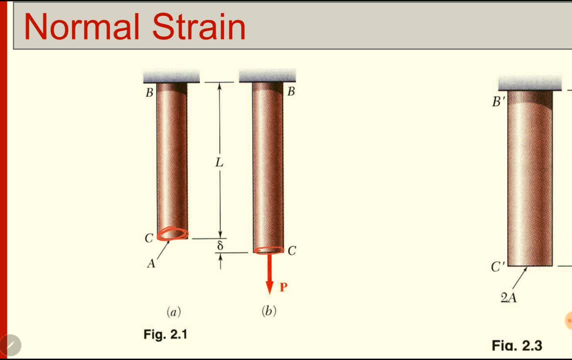 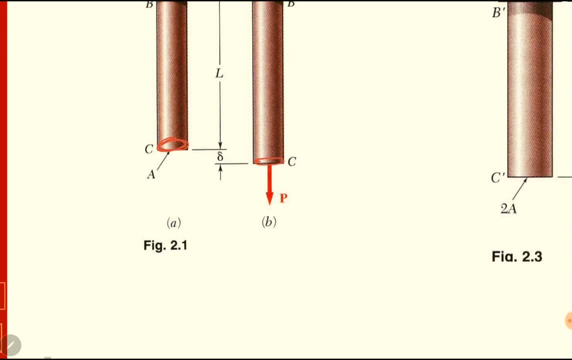 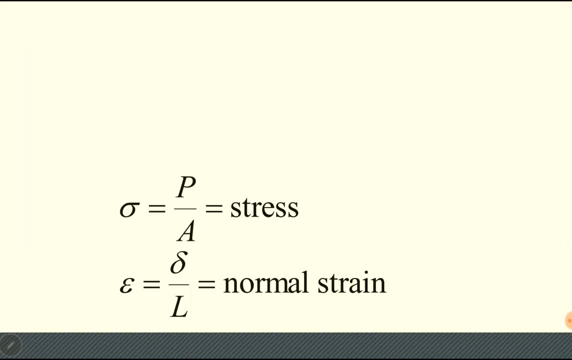 area. if you see it in the third dimension, the bottom view of this bar, this is perpendicular to the load. that is why it is called normal. so the load is normal to the area. so in such case strain is equal to Delta or length, and stress is equal to force divided by area P or a. now what happens? 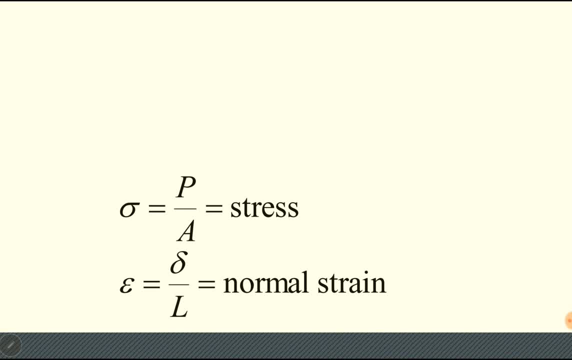 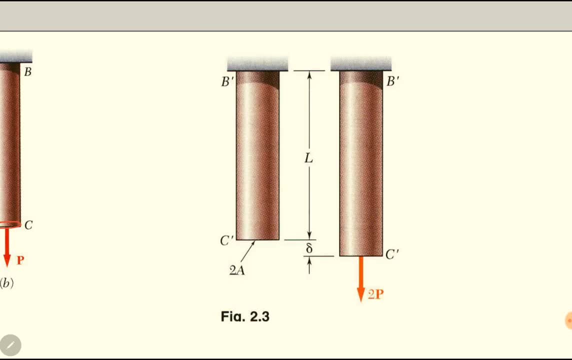 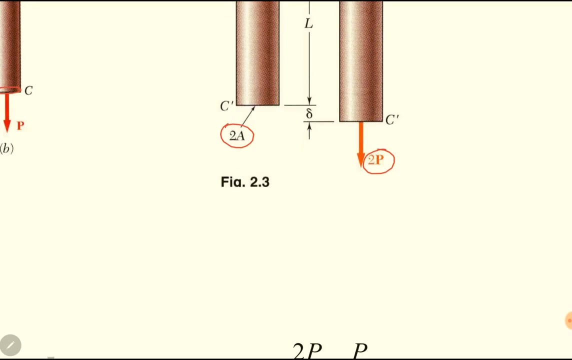 if we double the load or if we double the area or if we double the length. so if we double the area and also double the load, so stress will be 2 P over 2 a. double load divided by double area, so 2 p or a. so it again, it is again P or a. now we have doubled the load. 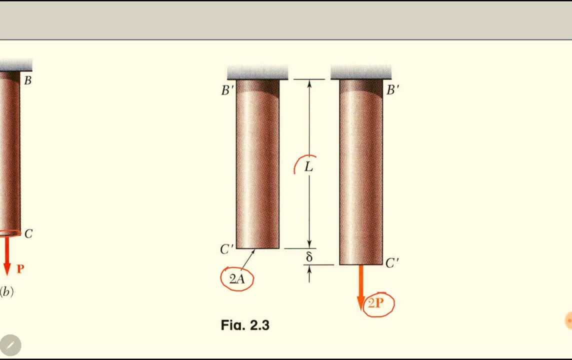 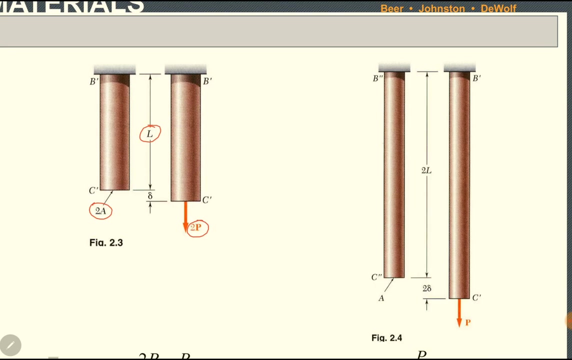 but the length is same. if the length is same, so the deformation will be same. it will not be doubled. the deformation does not depend upon the load, it is a, it depends upon the material. actually, if the length is l, deformation is delta. if we increase length to 2l and stress is again the same in all the three cases, stress is p over a. 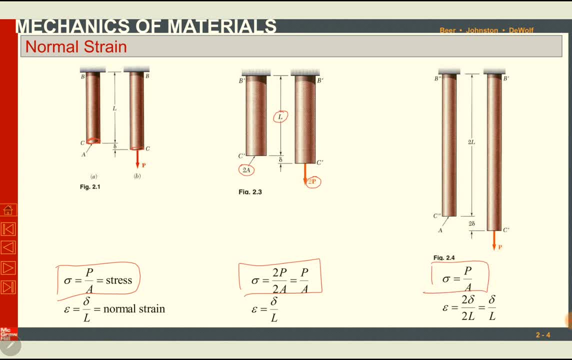 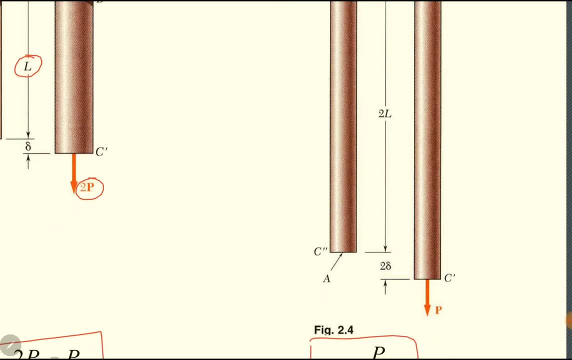 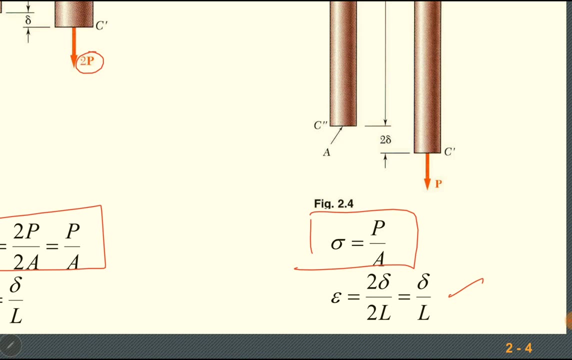 if the stress is same, so the strain will be same. we have doubled the length, in this case 2l, so deformation will be doubled automatically. again, the ratio 2 del divided by 2l will be del over l, so strain will be same. so if the stress is same, strain will be same. it does not depend. 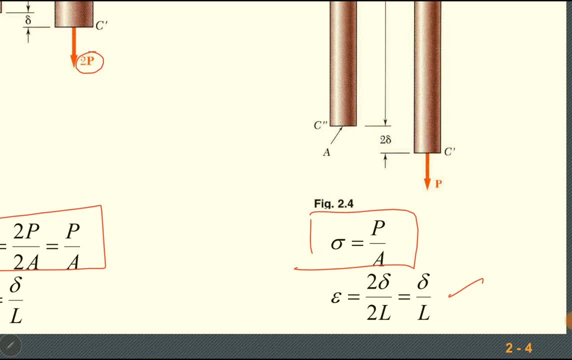 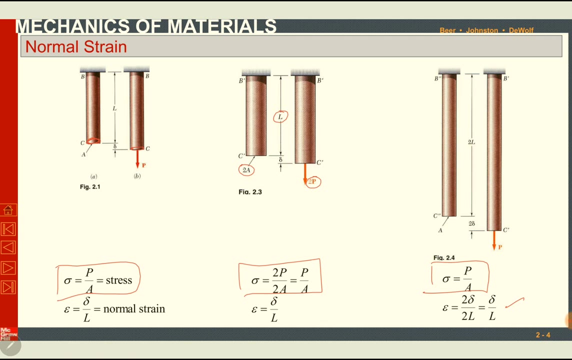 the strain does not depend upon load, it depends upon stress. actually, the stress depends upon strength. so the strain is same, stress is same. okay, so it means if we are doubling the length, if the material is same and the applied stress is same, so the strain will be same if we are doubling the length. 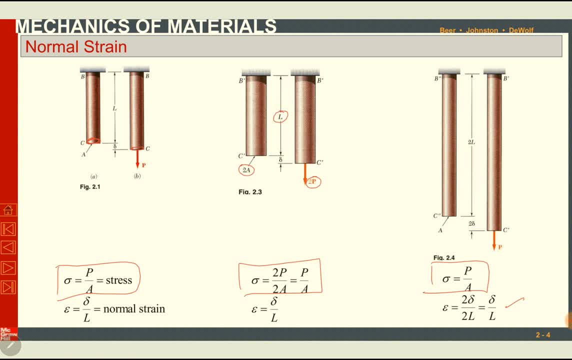 so the deformation will be doubled by itself. so it means strain is actually a material property. if the material is same, strain will be same and we will discuss it. how the strain is a material property and how does it depend upon the material, we will discuss it in hooks law later on. 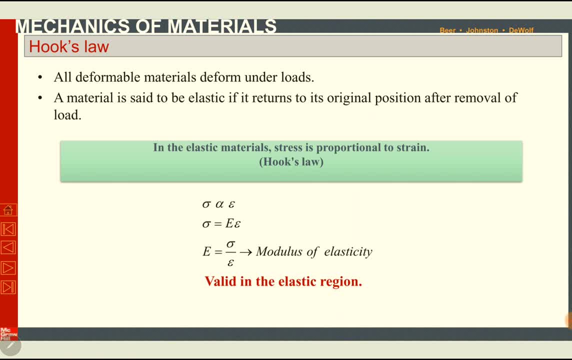 here it is. what is the hooks law? it was introduced by hooks and law is all deformable materials deform under loads. definitely before this, in engineering statics, we have discussed about non-deformable materials, rigid materials and rigid materials are rigid bodies, are those bodies which cannot be deformed under. 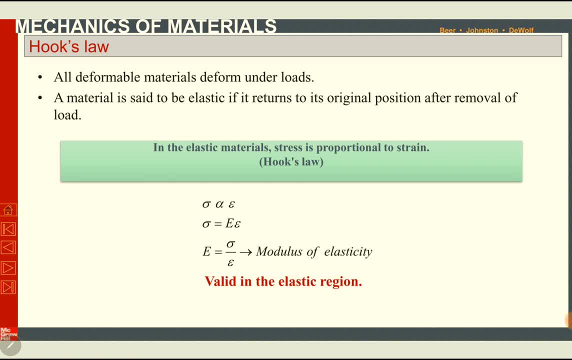 load. but in this subject we are discussing about deformable material. so we will discuss about deformation now. so deformable materials can be deformed under loads. in the absence of load, there will be no deformation. so under load, there will be deformation. a material is said to be elastic if it returns to its original position. 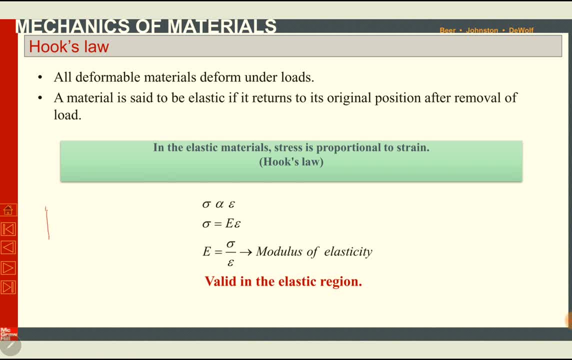 after the removal of the load. if there's a material and we are applying a load p on it and it extends by some amount delta, if i remove the load, it will return to its original position. this delta will be where this delta will disappear. this is this, this property of the 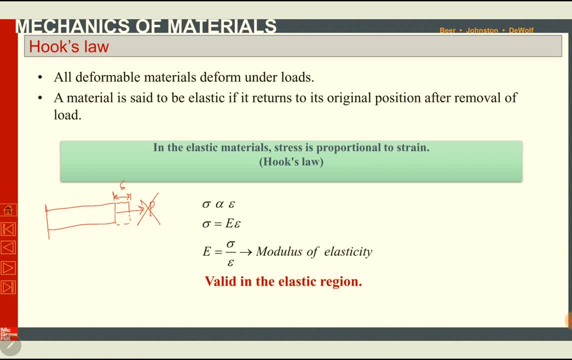 material is called elasticity and the material is called to be an elastic limit or elastic region. so if we remove the load and the material returns to its original position, this is called elasticity and in this elastic region or in this elastic material, stress is proportional to strength. this is hook's. 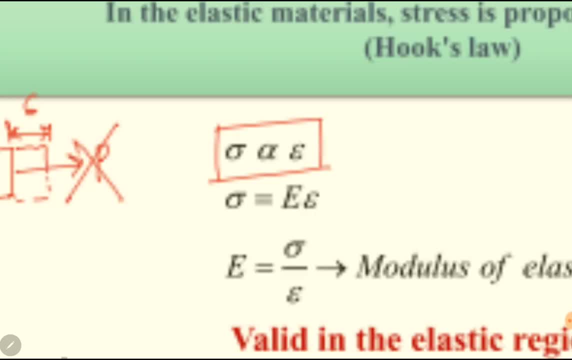 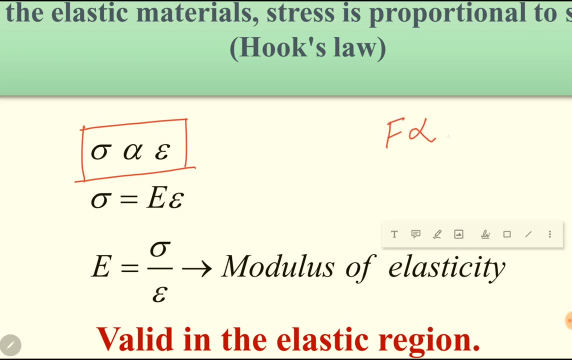 law stress is proportional to strength. previously we have studied in engineering physics a force or load is proportional to deformation. our load is equal to k delta. now we are saying stress is proportional to strength and stress is equal to e, epsilon. e is modulus of elasticity and it is the proportionality constant here. e is a material property. 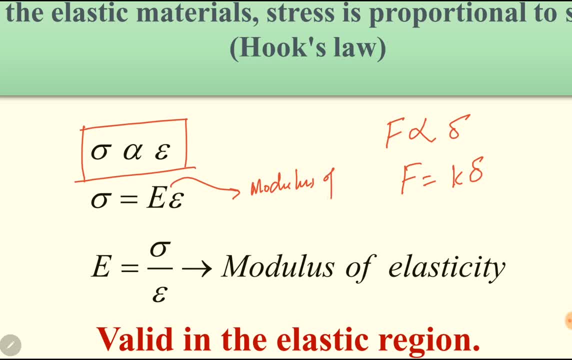 modulus of elasticity. okay, it is here. this is a material property. different materials have different moduli of elasticities and the strain depends upon this. e- okay, so e is a ratio of stress and strain. if the material is changed, the value of e will be changed. this expression of hook's law is the power of electricield voltage, which is represented in the symbol e. this is the tension of the hoyer. well, it is the potential for回來 strain and it is the marked value of voltage. so i am creating undefined. you can just see that only some explaining later. i have burned the voltage you can identify. 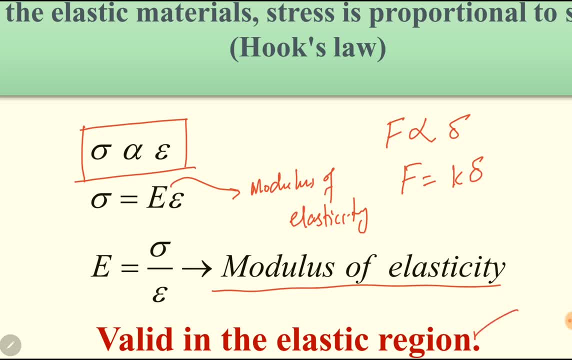 is only applicable within the elastic region. what is elastic region? we will discuss it in the next slide in the topic of stress-strength curve. some materials are totally elastic. there is no permanent deformation in those materials. the materials are called elastic materials. some materials undergo elastic and plastic deformations in under different loads, under some. 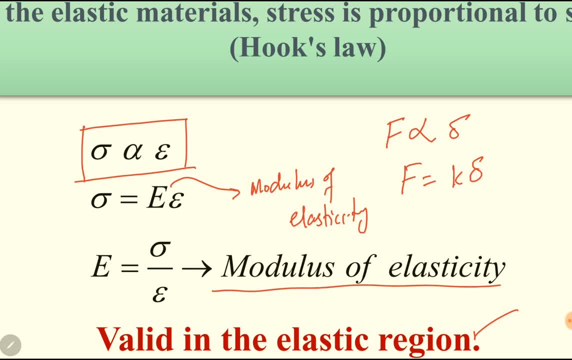 loads, under lower loads, under the loads of low magnitude, the materials do not deform permanently. they remain in the elastic region. whenever we remove the load, the material will return to its original position, so that region is called elastic region. and after some certain amount of load the material will 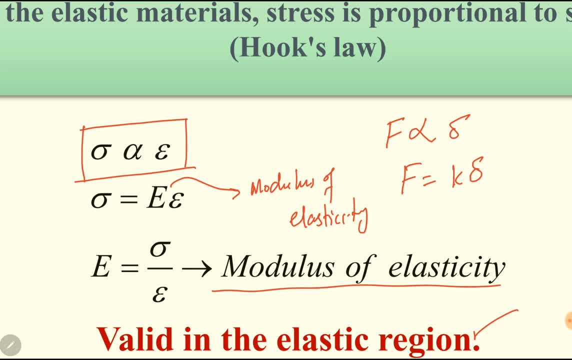 be permanently deformed and that is the elastic limit. beyond that limit material will be permanently deformed. so below that load the material is said to be in elastic region. some materials are totally elastic. some have elastic and plastic regions separately. okay, now we will discuss the elastic and plastic regions separately. 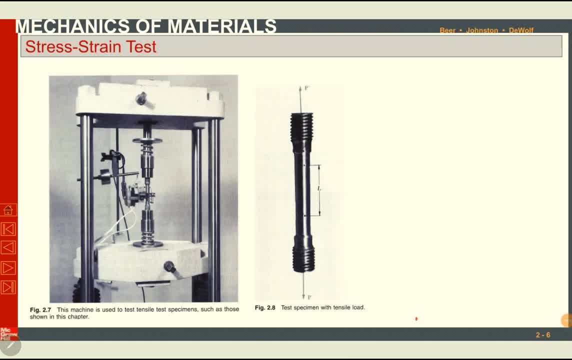 okay, so our next topic is stress-strength test. this is a very important test, a very basic test for in the for the subject of mechanics of materials. by this test we can evaluate aneau test, we can draw a diagram between salt 발ants of a certain 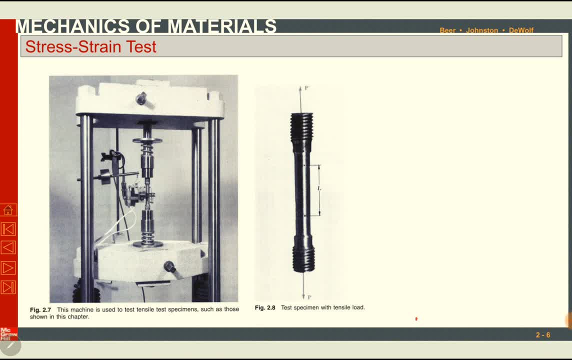 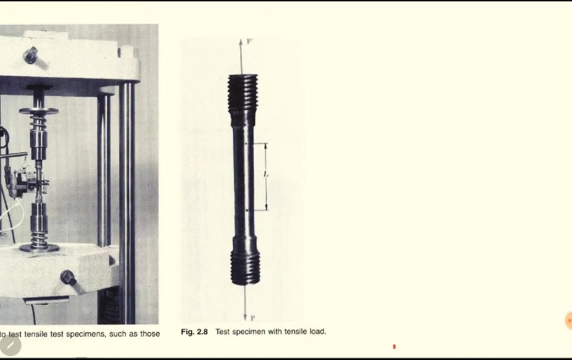 stray hall of glass of a certain style of material. we call itcektron hierarchies of a material or compressive properties of material. as the result of stress run test, we draw a diagram between stress and strain. in this test we usually cut a specific specimen- testing specimen- from a material. the test is 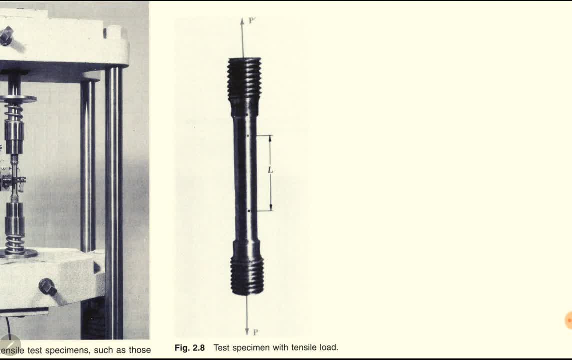 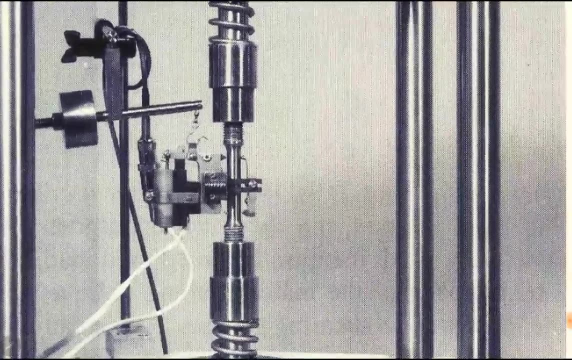 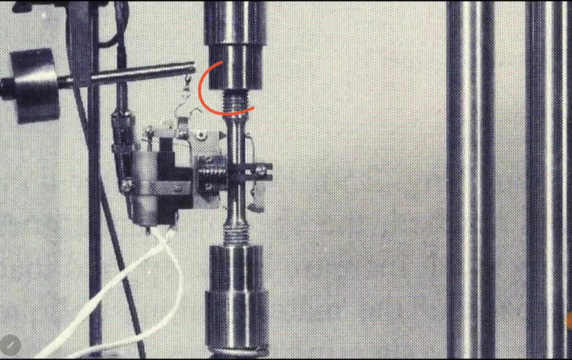 performed under some standards, against some standards, usually Americans. or about testing materials: ASTM standards are some other society standards, established society standards. okay, we just hold this specimen in a universal testing machine. here is the specimen. it is held by the machine jaws from the two ends and tensile force is applied on it. our compressive forces apply either the 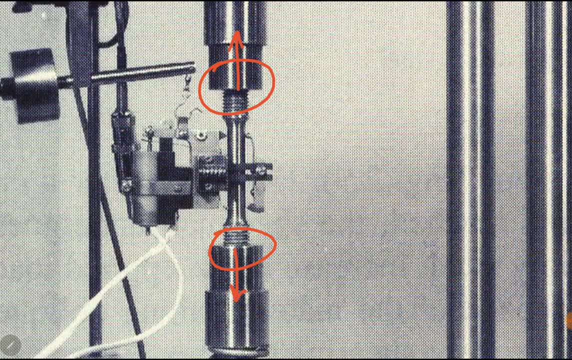 jaws move away from each other or they may move towards each other. in case of moving towards each other, the same- the sample or the specimen- remains under compression. if the jaws are moving away from each other, the specimen or the material will be under tension. okay, so this material is under. if this, 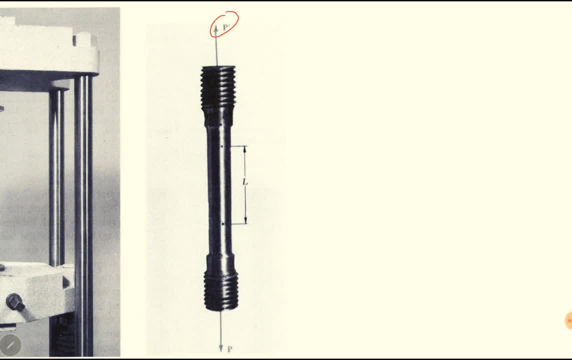 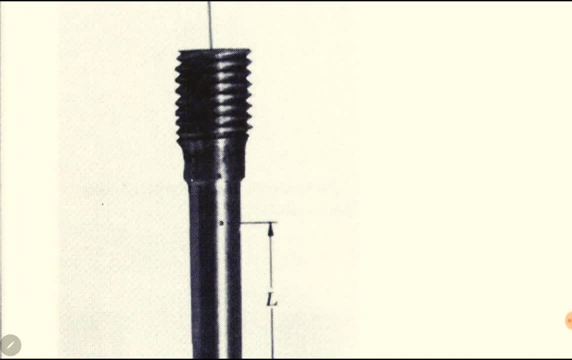 material is under tension, there will be tensile loads. thanks this threaded, shaped for this materialis, an essential component in the tension work in end, is held in the machine. the threads are to produce friction between the machine jaw and this specimen to held. to held it tightly so that there is no slippage. we usually specify two points. 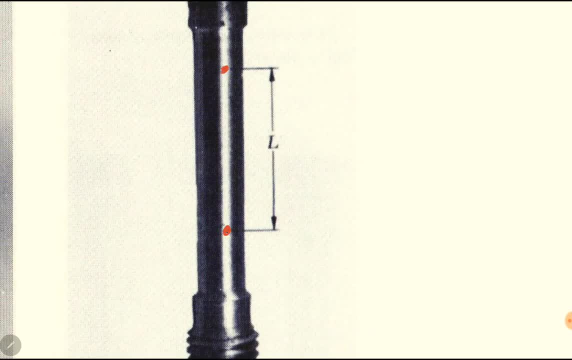 on the specimen. between the two points we have length, initial length l, and after applying force on it, these two points will move away from each other and this length will increase. there will be a change in length that will be called Delta and we can find this the the strain from Delta. 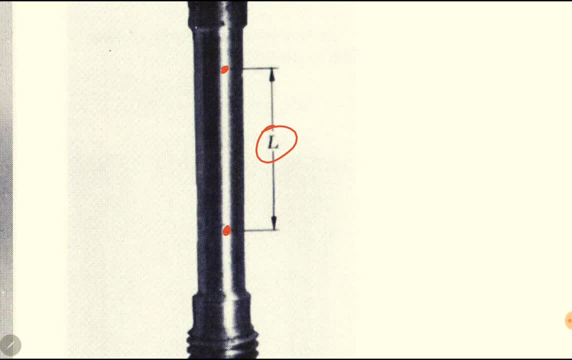 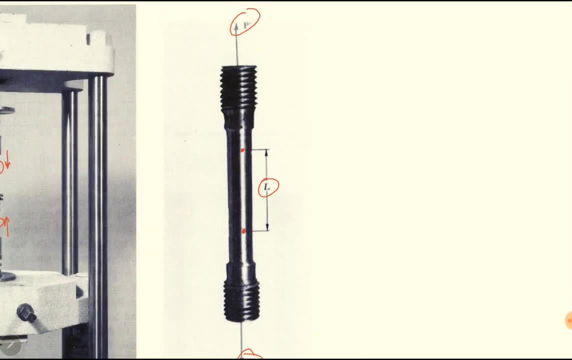 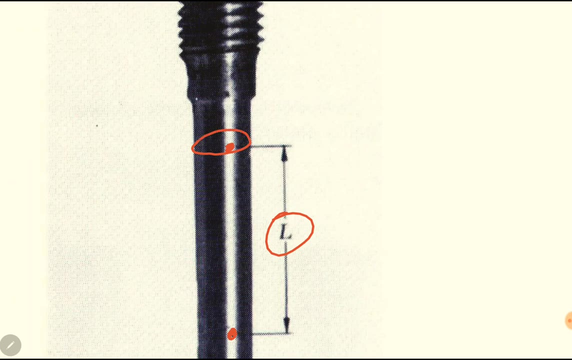 divided by L. this, the value of Delta, is given to us by the machine and the applied load is also given to us by the machine. from the applied load we can find stress. how we can find stress? simply, the cross-sectional area of this portion where we are considering the length. so the area will 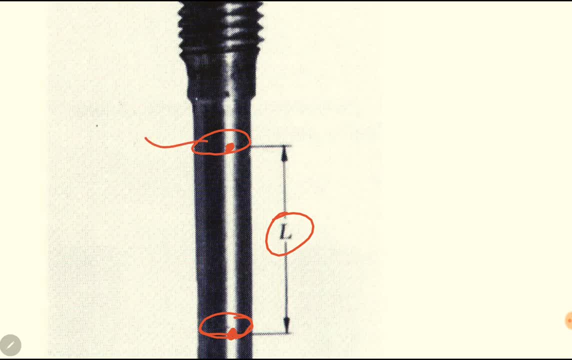 be constant between these two points. this is cross-sectional area and third dimension. so we can simply divide load, applied load divided by area, to find stress, and change in length divided by original length to find strain. as soon as we increase the load, the stress will increase and similarly. 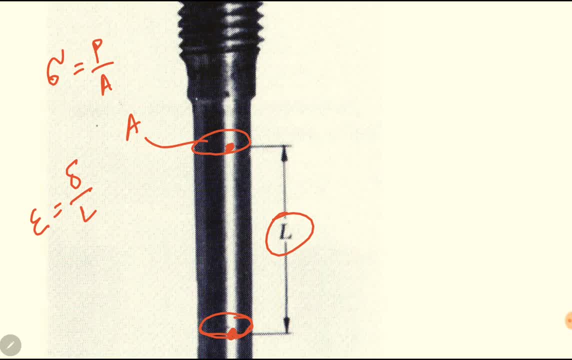 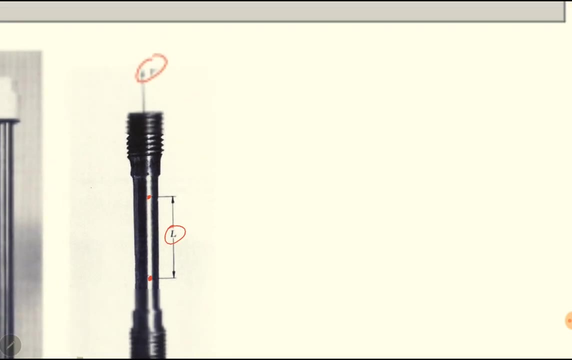 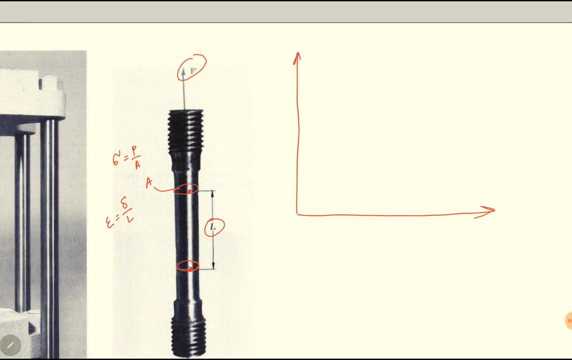 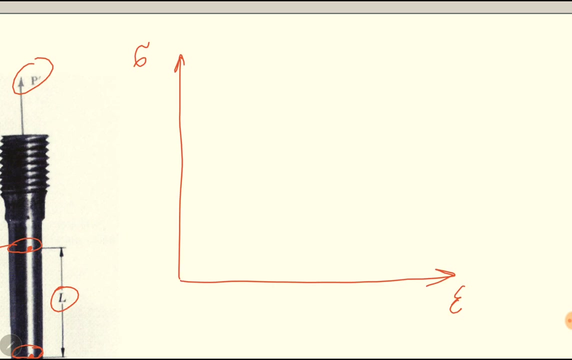 Delta will increase, so strain will increase. so we record different values of load and deformation and similarly we can calculate different values of stresses and strains from the loads and deformations. then we draw them against each other. here I will draw a diagram between stress and strain. on the horizontal axis we have strength and on 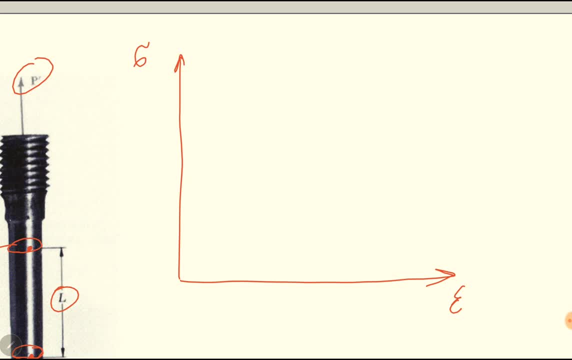 the vertical axis we have stress. okay, initially, when there is no load, there is no deformation. or if there is no deformation there is no, it means there is no reaction force in the material. but what the stress is calculated from it is load divided by area. but that load is actually the reaction force. P is 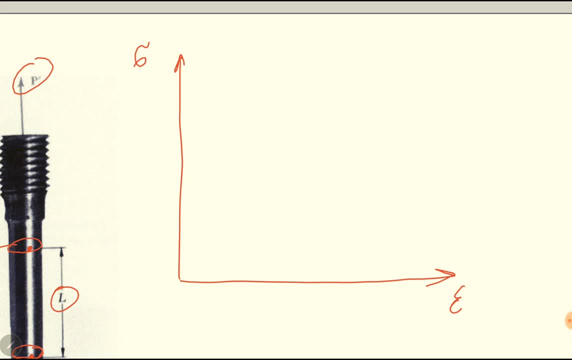 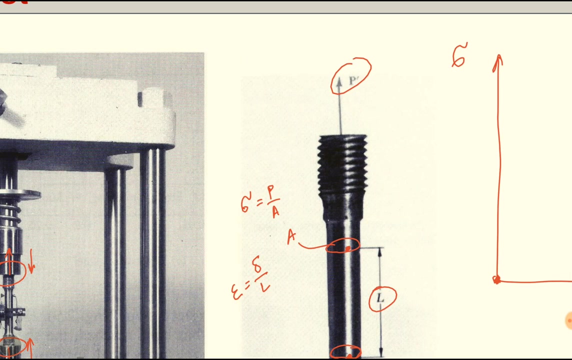 actually the reaction force against the external load. okay, so at zero load there is zero deformation. as soon as we increase the load, or if the machine applies load, so the material will deform due to the deformation. strain will increase, using this expression, due to the deformation, if deformation is. 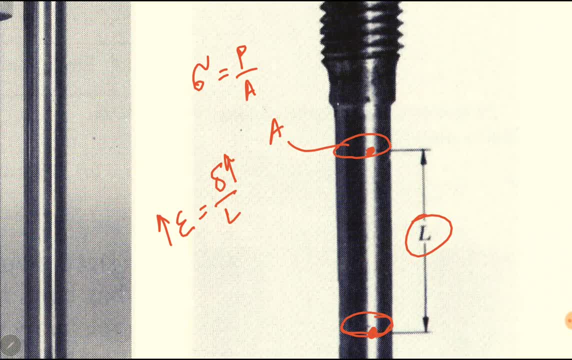 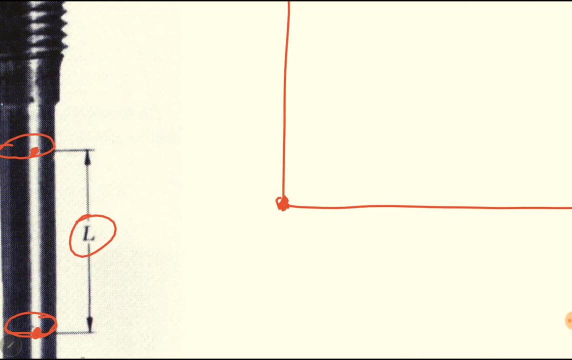 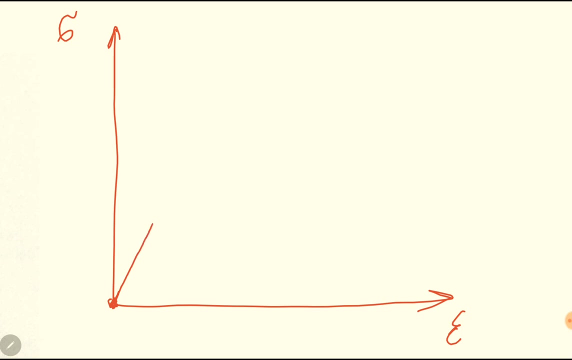 increasing, strain will increase. okay, with the strain increasing we will have stress increasing. internal reaction force is P divided by a. the internal reaction forces will increase. so stress will increase. so as the strain increases, stress will increase. internal resistance of the material will increase. initially it will be linear relationship up to certain point. this is called proportional limit. 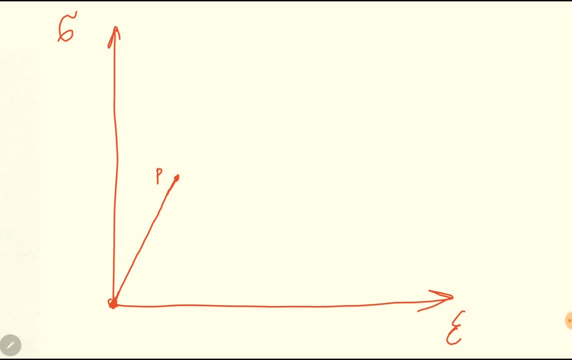 until proportional limit, P point, the stress will be linearly proportional to strain. okay, after this point, shortly after this point, very near to it, there will be elastic limit E. after point P, after proportional limit, if we keep on increasing the deformation, keep on applying the load, so again, more. 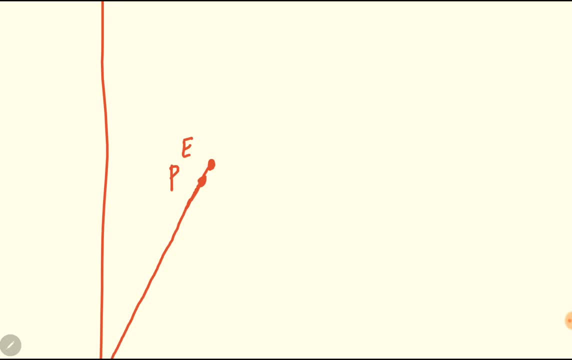 deformation will be produced, there will be more stress. so there comes point E. until E, the material is elastic. if we remove the load, this material will return to its original point, its point O, initial point, origin. so the difference between P and E, proportional limit and elastic limit. 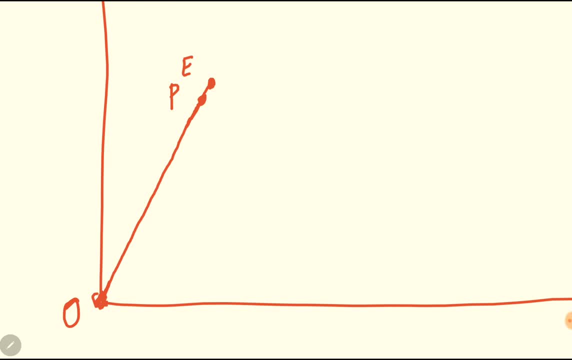 is after proportional limit, stress is linearly proportional to strain. after point P, between P and E, the stress is not linearly proportional to strain. but again, the material is still elastic. it will return to its original position. okay, but these two points are very near to each other and they are considered to be. 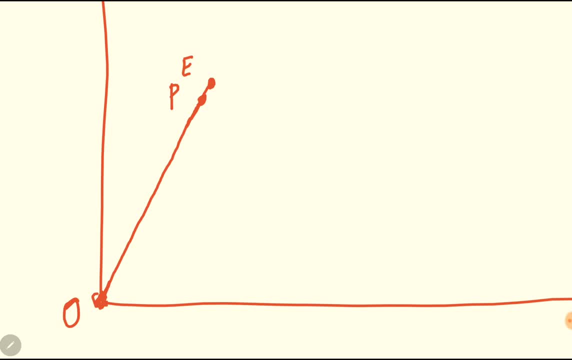 same. generally we cannot differentiate between P and E. for all the for, for, generally for all materials. it is very rare that we the difference can be recognized between P and E. generally for all materials P and E is almost the same. they are considered same, okay, suddenly, after E there is yield point. yield point is the point from where permanent. 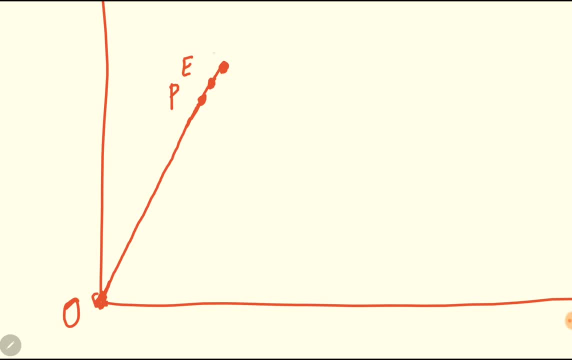 deformation in the material starts before yield. there will be elastic deformation only, non-permanent deformation only. but as soon as we reach the yield point, permanent deformation will start in the material. okay, now there are two types of yield points. one is upper yield and the other one is lower yield. okay, what is upper yield and what is lower yield when? 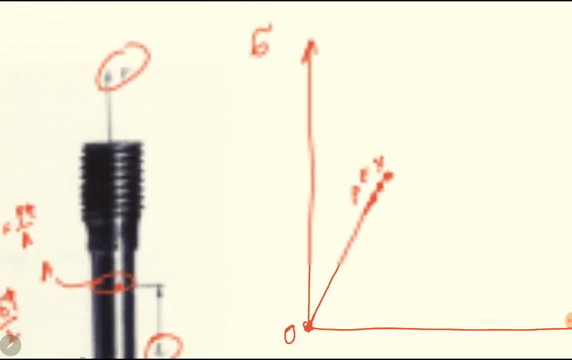 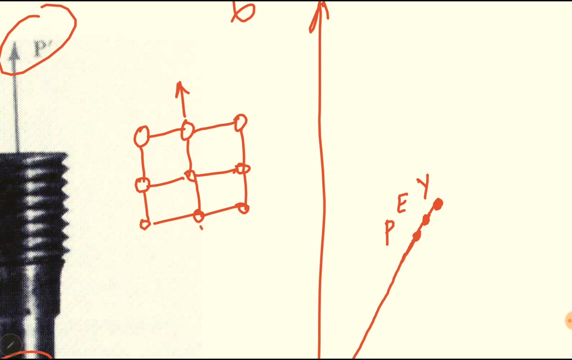 we apply force on materials at on the atomic level there is an atomic structure. the atoms are connected to each other through some bonds, and when we apply forces, external forces- these bonds are under external loads, so they will either stretch or they will be compressed. the bond length will tend to 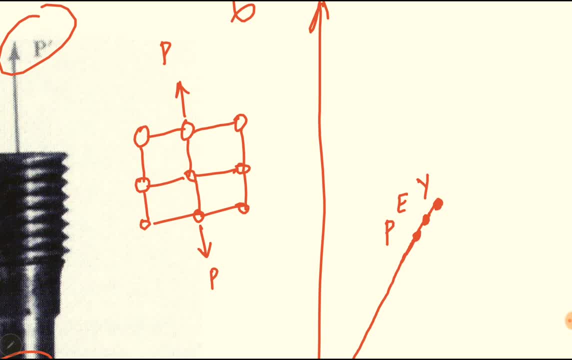 increase or decrease. so definitely, naturally, a material resistant material to it, so the it will resist against the change in length of the bond. if, in this case, in this figure, we are applying a tensile force, the, so we are trying to elongate the bonds, the bonds will resist if we remove the external load. these 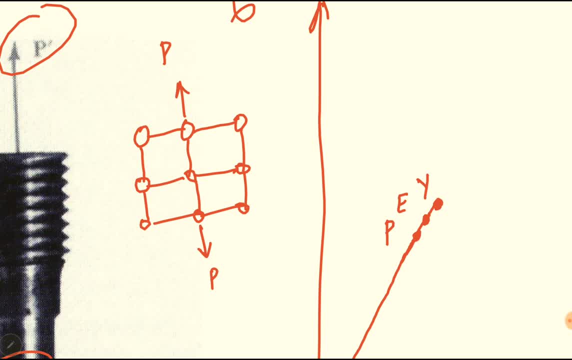 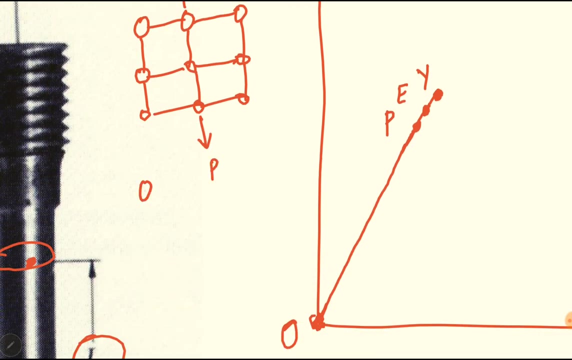 bond lengths will be restored to their original position- original lengths. okay, this is internal resistance of the material at atomic level. okay, if we keep on increasing the force, there will be a point when this bond cannot resist permanently and it will be deformed permanently. this is initial. 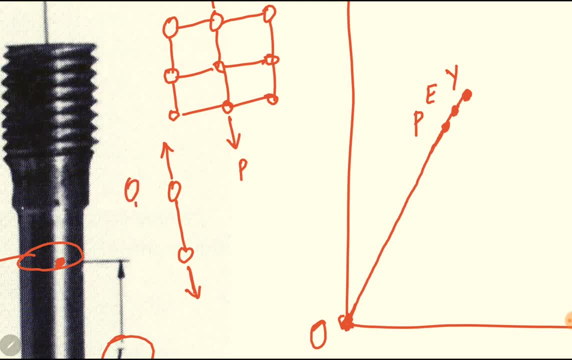 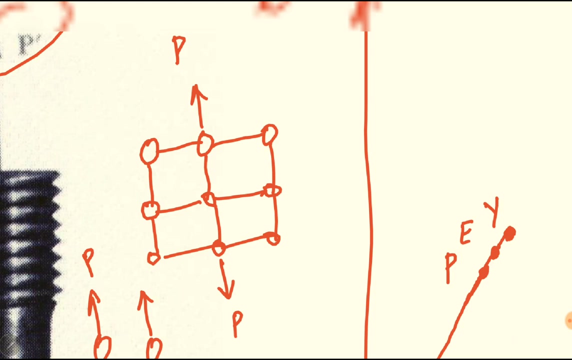 length. so after yielding point it will be permanently deformed. it will not return to its original position after the removal of the load. so there is a permanent deformed point. okay, before the yield point. if we remove the load, it will return to its original position. okay, now there is an equilibrium arrangement of atomic 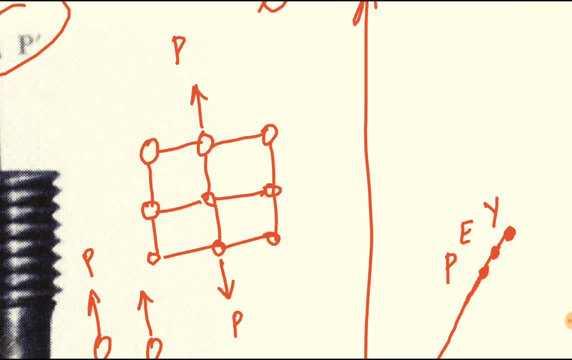 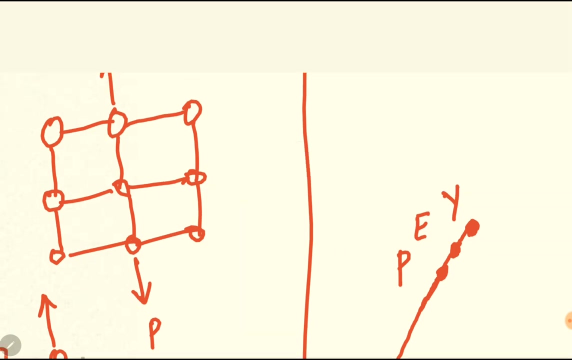 structure. when we apply force, we are trying to disturb that equilibrium within the elastic region are below the yielding point. there is a one kind of equilibrium arrangement. if we just keep on going forward this carefully, once the material reaches yield point, where I have written y, that is the actual top point- then, as I will mention, 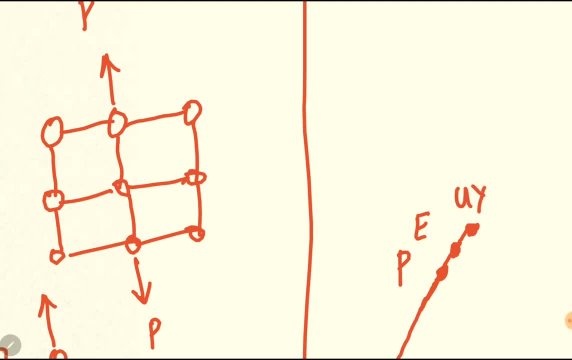 here. that is the top point of the elastic environment. these different criteria, okay. and once the material reaches upper point, ok. so actually, cis boxer will slip round in between the曲 Mega movies, as swollen. so once the material reaches point, why slip upon each other? and it at, it shifts itself from one equilibrium state to another equilibrium. 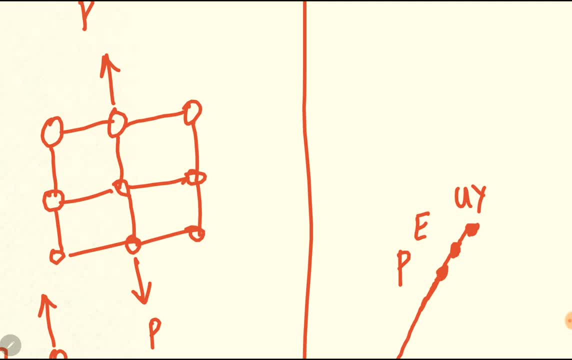 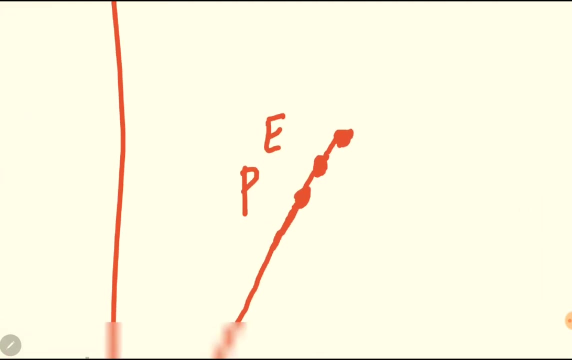 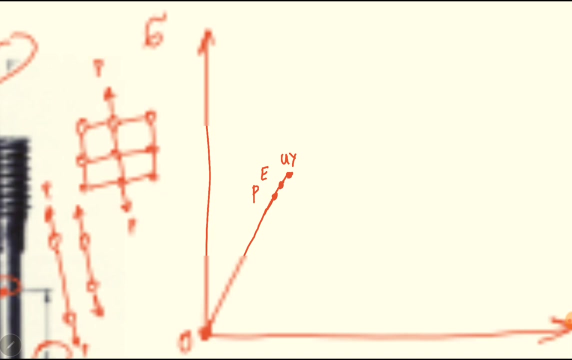 state. there is a new equilibrium state of at the atomic level in this uh, this transition state. when the material achieves uh, or when the material shifts from one equilibrium state to another equilibrium state, so its resistance falls, it cannot resist as much as it could do earlier. so if the resistance falls, stress will decrease again. vertical axis is stress axis, so 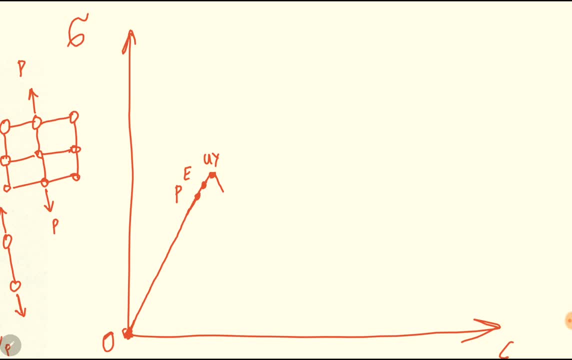 stress will decrease again. the resistance will decrease. so definitely, stress is has decreased, although the strain has increased. but stress is decreased once the material reaches a new equilibrium position. so it will again starts resisting to it, will again start resisting to the external loads or resistance to the deformations, and again, with increase, 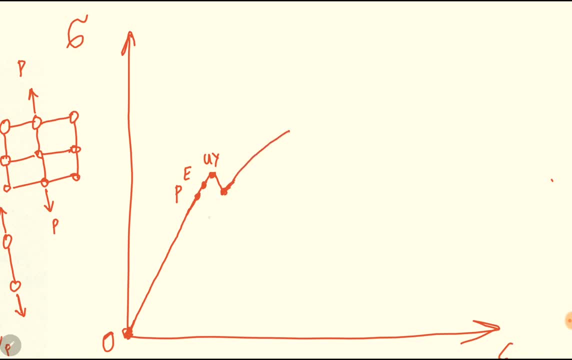 in deformation, stress will increase. so this point is lower yield, point between upper yield and lower yield. stress is decreasing although stand is increasing. but stress is decreasing although we are applying external force. with the force, the generally the stress should increase because we say that stress is equal to force divided by area. 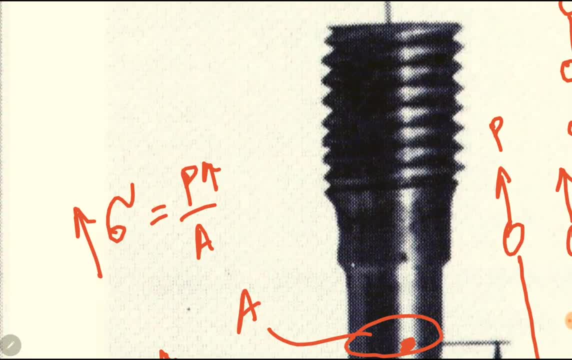 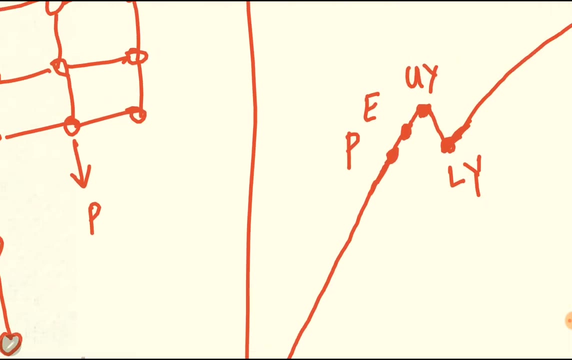 if the external force has been increased, there should be an internal resistance, equal internal resistance and the force by the resistance. force divided by area should be stress. but the internal resistance is weaker because of the change in the equilibrium state at the atomic level. so the stress decreases for some time and after lower unit point is achieved it means the 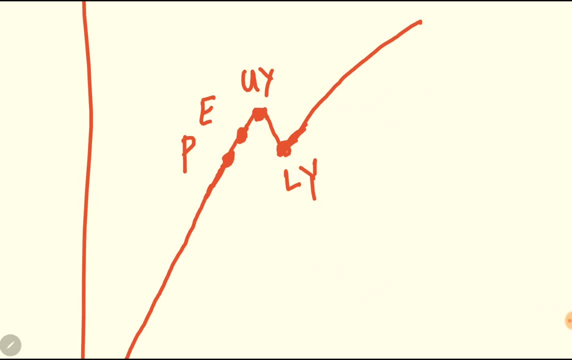 the at the atomic level, the material has achieved a new equilibrium state and then again it starts resisting and with the deformation, stress will increase again until some point, which is called ultimate stress. this is the maximum limit we can achieve, or the maximum capacity of our material, which can it can resist against the external loads and the deformations. 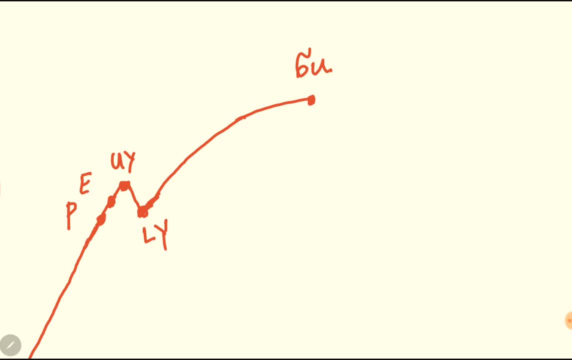 after this, material cannot resist, even though the strain is increasing or the deformation is increasing. stress will decrease. ultimate strength or ultimate limit is the maximum limit or the maximum resistance of the material that can offer. so after this, even though the stress is in, the strain is increasing, external loads have been increased, but the stress will not increase stress. 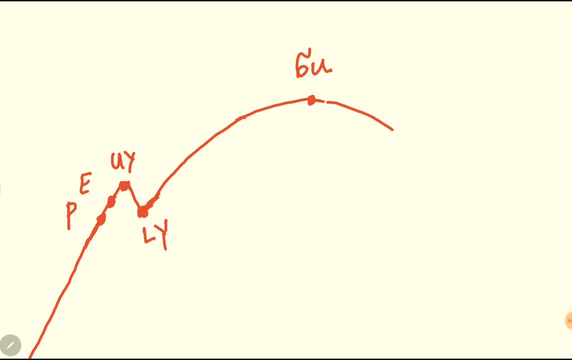 will fall down. so it means the stress is materialized in this case. okay, now what happens here? the stress is decreasing, although there is a strain in the material. until some limit, or after some deformation, the material will rupture. it will be broken down into two pieces. we are talking about tensile loads, so it will be broken. 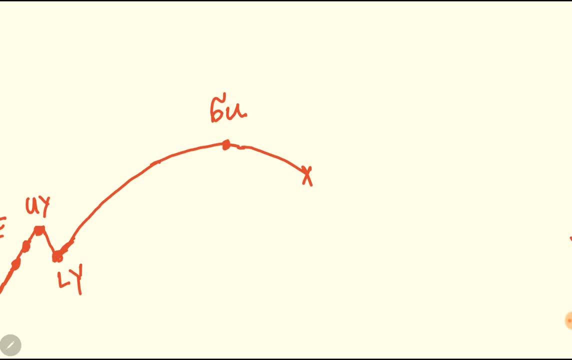 into two pieces. fracture occurs under tensile load. this is called rupture point or sigma r, rupture after sigma u, after ultimate limit. actually it should go like this by definition. by mathematics stress is equal to p over a. so once we are increasing load, the external loads are being 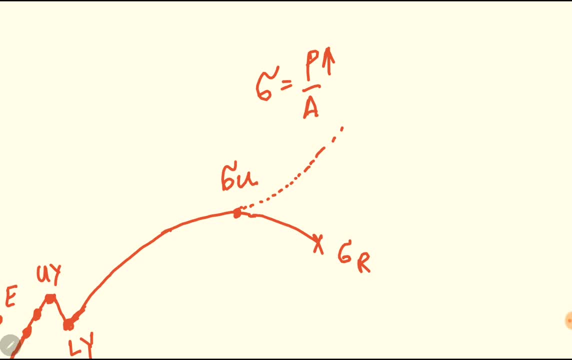 applied by the machine and the universal testing machine. so once we get And after increasing load, so stress should actually increase. so by this formula of stress, stress should increase. so I have shown it with the dotted line. this is called true stress strain curve, but actually it is decreasing. 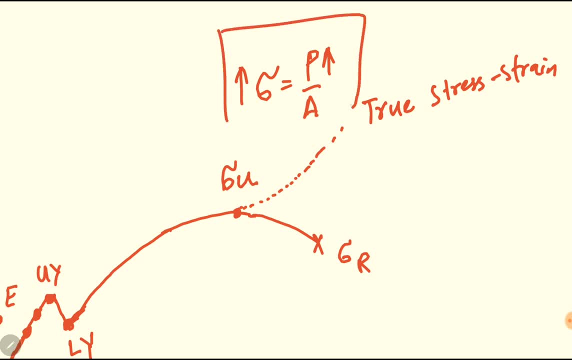 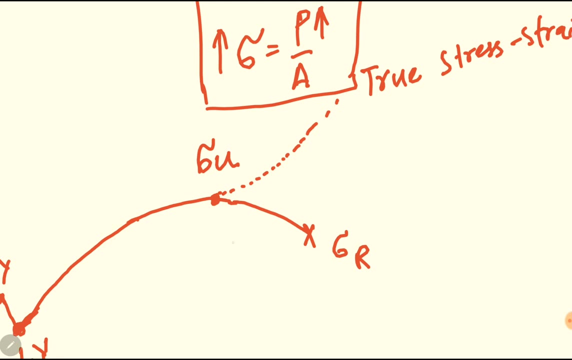 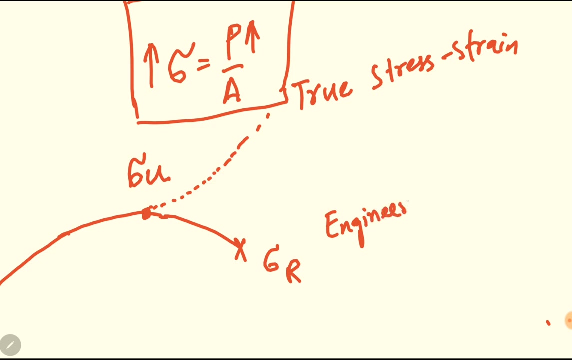 in this region. it is not following. the formula of stress is equal to P over A. it is actually decreasing at the material level. so why is it decreasing? because the material cannot resist, so the stress will fall down. this curve is called engineering, stress strain curve engineering, which is the real one. 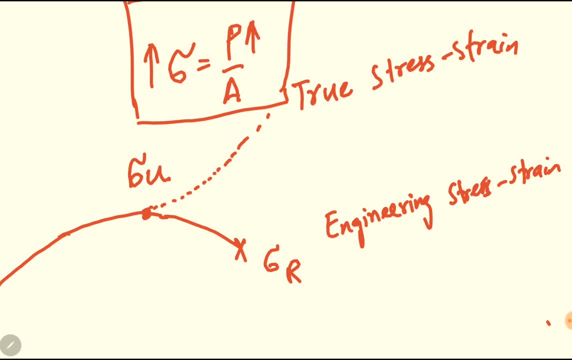 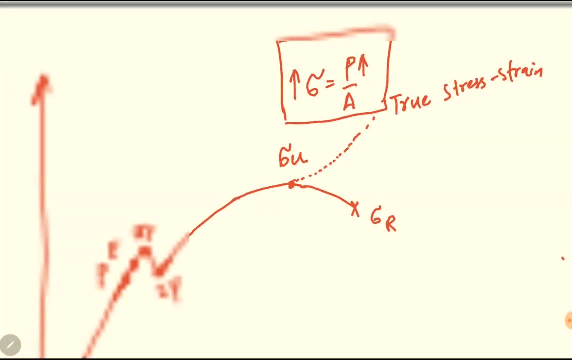 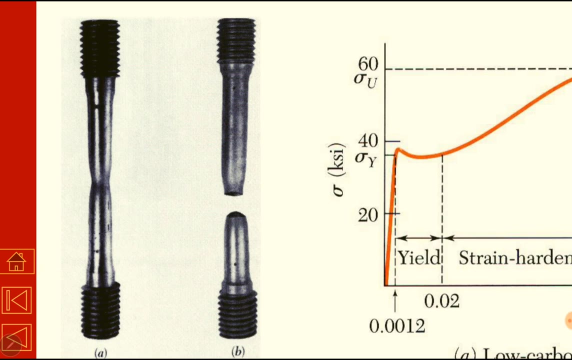 this happens actually. now why it fractures? why it ruptures actually when we apply force on a material, on a ductile material. specifically, what is a ductile material? ductile material is a material which can be permanently deformed into a new shape or into a new length under load. 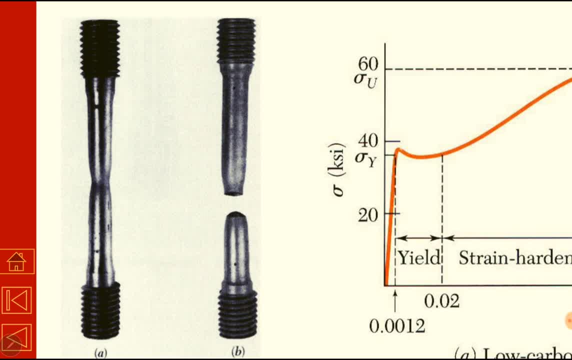 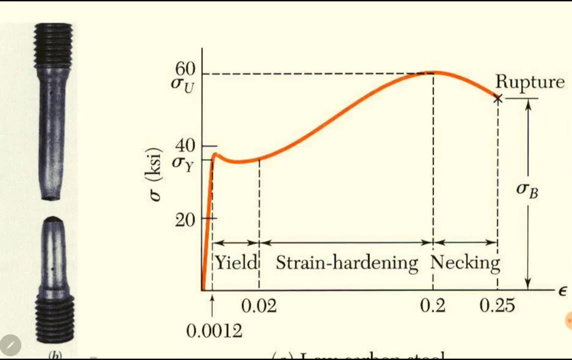 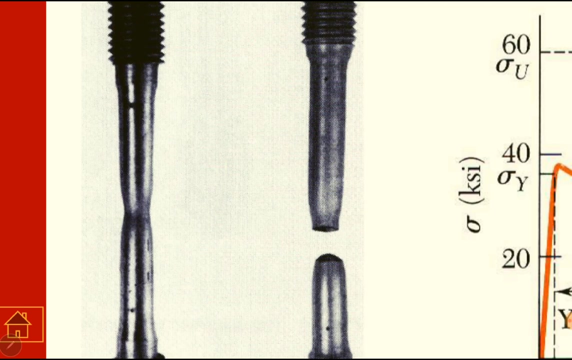 brittle materials cannot be deformed permanently, so we will discuss about brittle and ductile materials later on. ok, now, currently we are talking about ductile only. once we are applying external forces and we reach the ultimate limit, this limit, what happens? the area at some point starts decreasing. 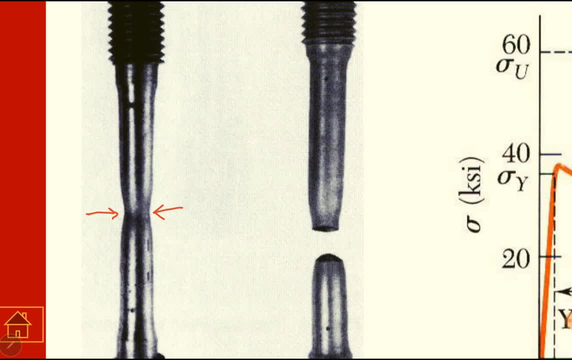 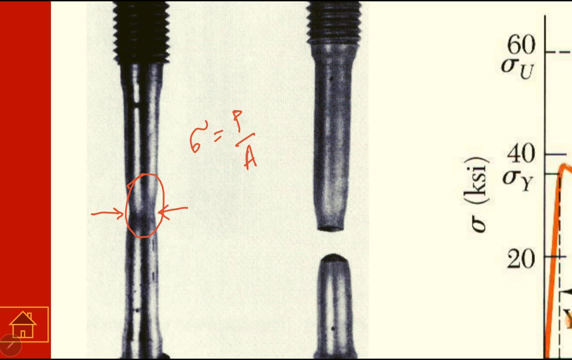 the cross sectional area. this is called necking. you can see a neck here. area has started to decrease. if the area is decreasing and external load is increasing, stress should increase. actually, because stress is proportional to load. load is increasing, stress should increase. stress is inversely proportional to area. 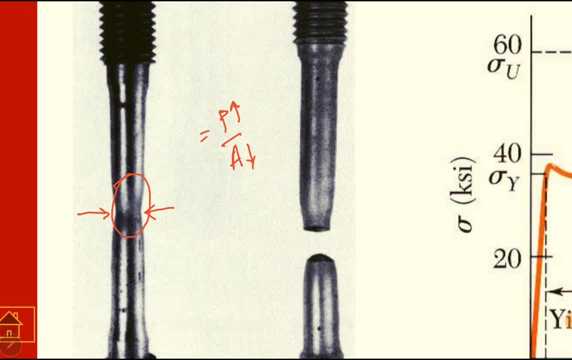 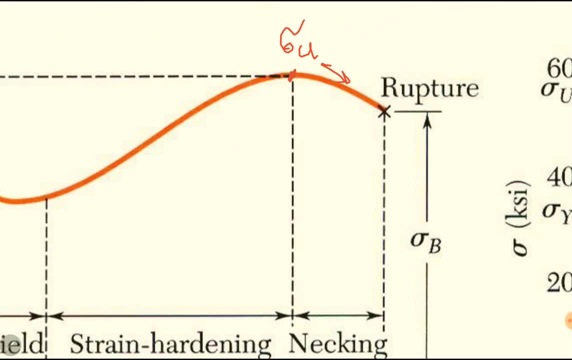 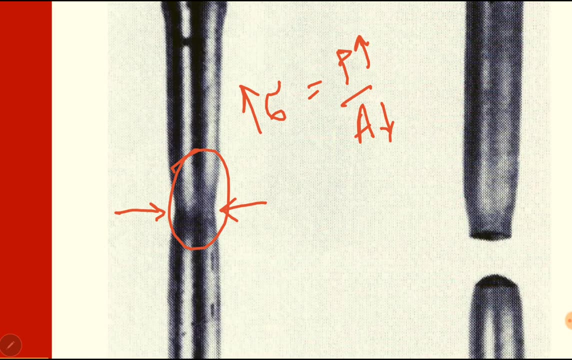 area is decreasing, stress should increase, but actually it is not increasing. you can see here it is not increasing, it is decreasing here. so what is going to happen? because the material cannot resist. that is why stress is decreasing. there is no internal resistance. area is decreasing. there will be some point that the area will reach to a minimum value, almost. 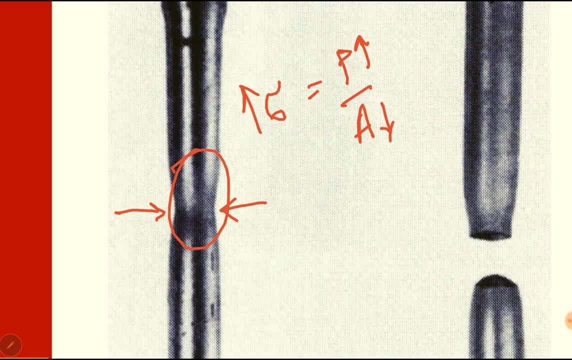 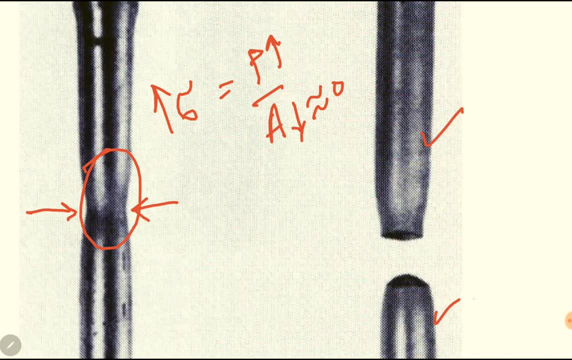 equal to zero if area is decreasing at some instance. if area is almost equal to zero, it means there is just a point contact between the upper part and the lower part. stress will be almost infinite, theoretically. should it should be infinite? okay, if it should be infinite, the material cannot bear it and 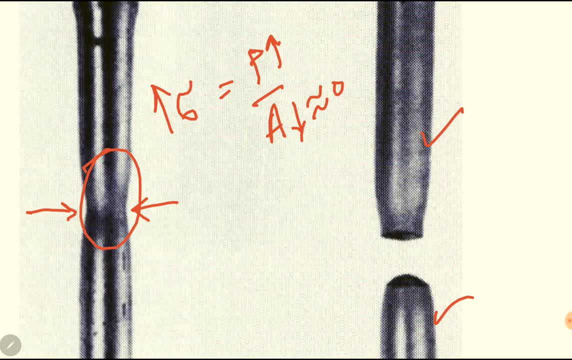 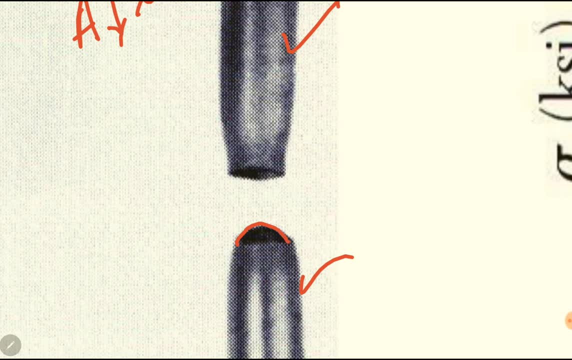 it will be. it will fracture into two parts. after fracture we can see that there are two parts. one is cone, the other is one is cup. so there is a raised part and there is a part. this is a concave part and this is convex part. you can see such kind of 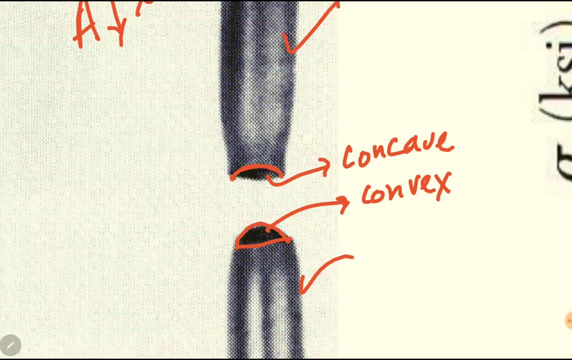 shapes. if you practically deform a ductile material under load, you can personally observe it. or if you do a test in a mechanics of materials laboratory under a UOTM machine, so you can see like this: most of the metals are ductile and the metallic specimen are. the polymer specimens can be deformed in such a way. 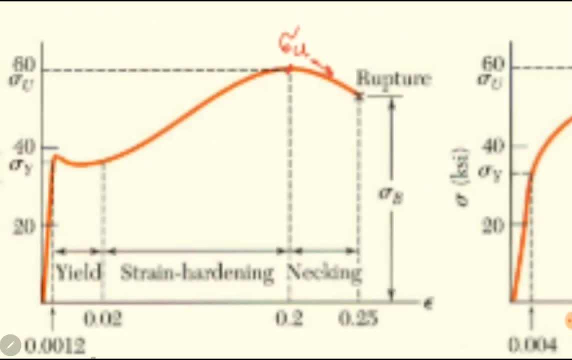 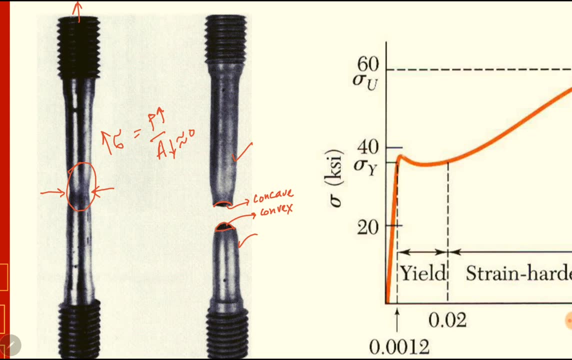 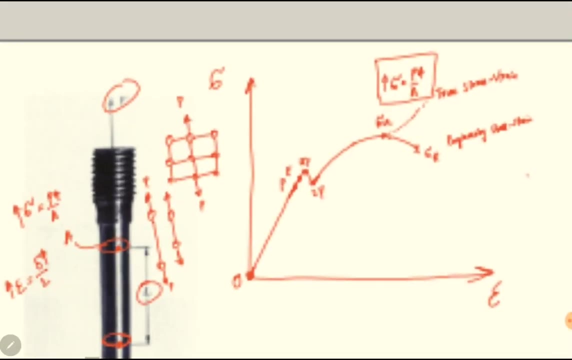 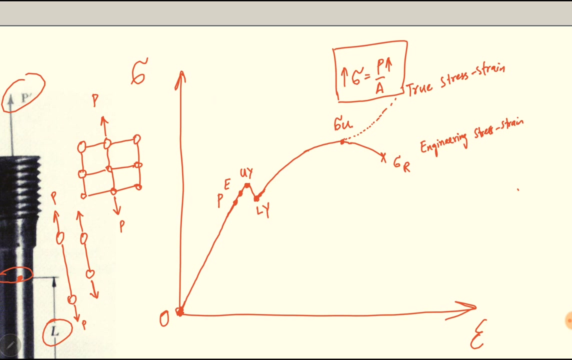 so this test of this shape of a stress turn diagram is that of ductile material- ok, and the cup and cone structure happens in ductile material, okay. so previously I have shown here a detailed stress turn diagram where I have shown proportional limit, elastic limit, yield point or yield limit. 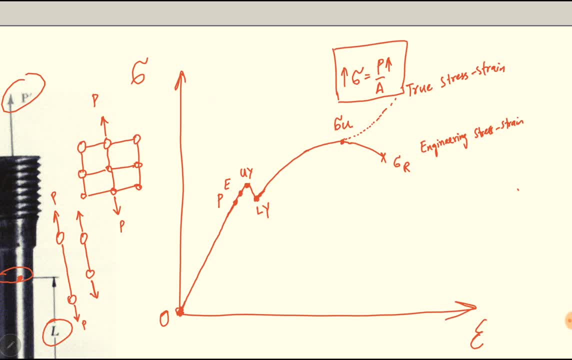 The elastic proportional and yield points are so near to each other that they are generally considered single point and they are simply labeled as yield point or yield strength, or sometimes in some books they are called. this point is called actually elastic limit or elastic strength, So generally it is yield strength or elastic strength, yield limit or elastic limit. 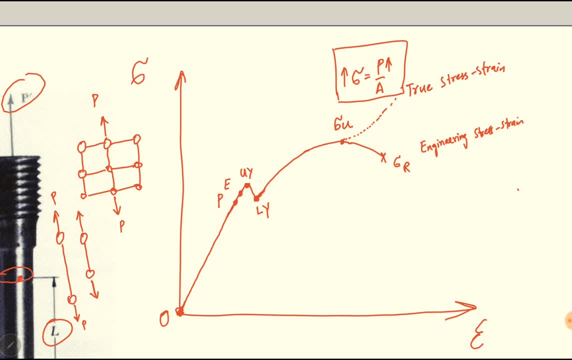 Beyond this limit- sorry, below this limit- the material behaves elastically. it will return to its original position after removal of the load. Beyond this point, the material behaves plastically. it will be permanently deformed if the load is above the yield strength. So from now on we will: 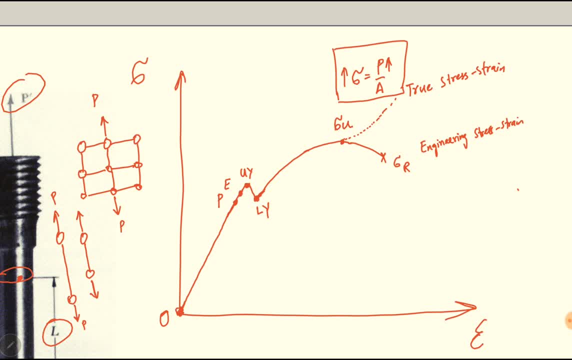 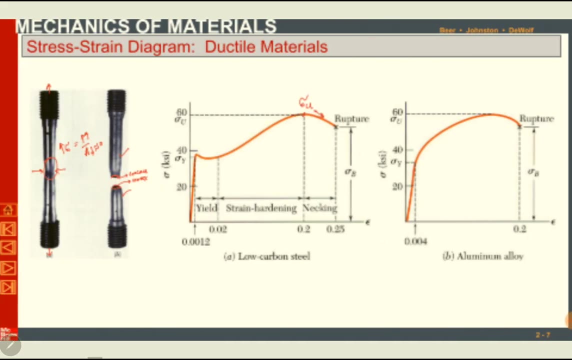 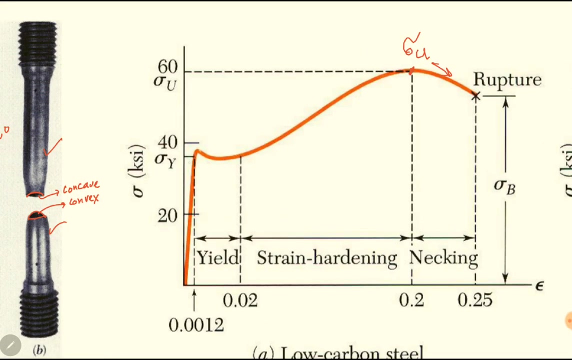 simply talk about yield strength only. we will simply mention yield strength. we will not discuss about elastic limit plus proportional limit and yield limit separately. So all these points will be called yield strength or yield point. Okay, so here in this diagram- this is a diagram for low carbon steel- we can see here is a yield limit. 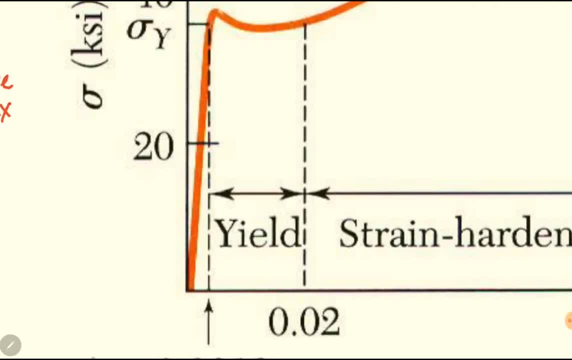 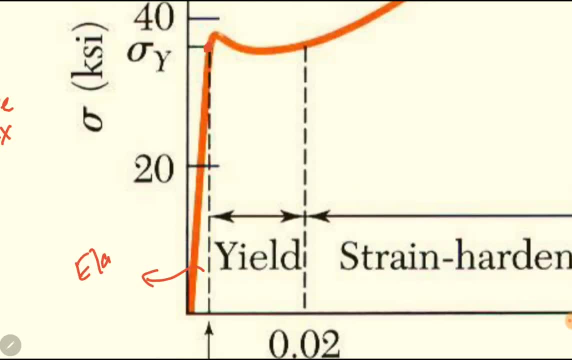 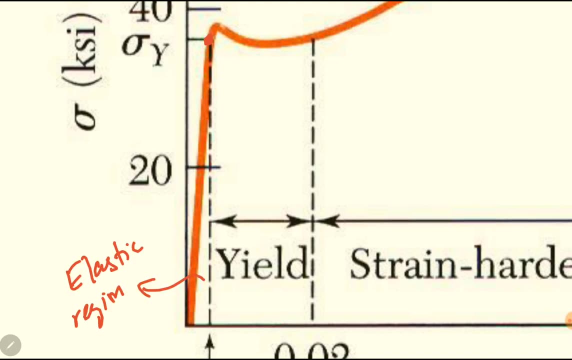 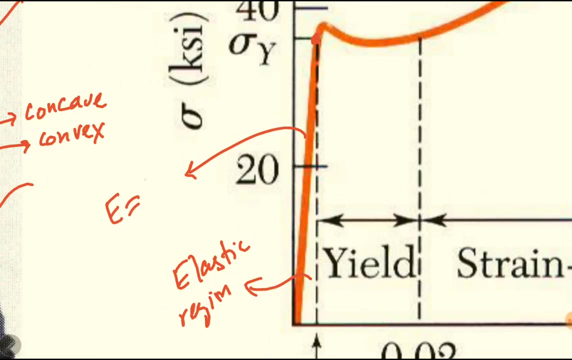 sigma y: Okay, below the before the yield limit. this is elastic region. In the elastic region, the stress turn curve is a straight line. it is a linear relationship. So Hooke's law can be applied as follows: E is slope of this line, which is modulus of elasticity, which will be equal to stress divided by strength. 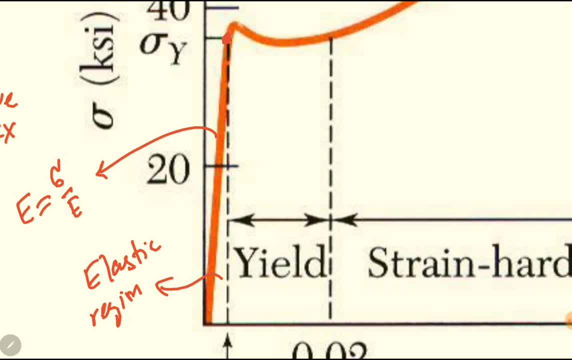 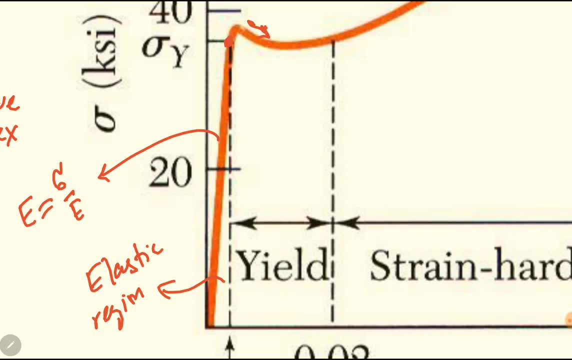 Okay. between upper yield and lower yield, as I have discussed earlier, there is a fall of stress. stress is decreasing because of the rearrangement of atoms in the material. at atomic level There is a. the atomic structure shifts from one equilibrium point to another equilibrium point. 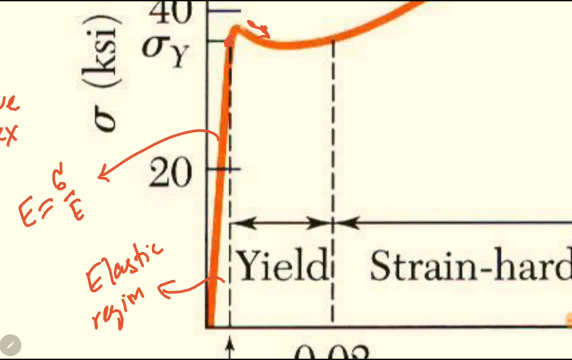 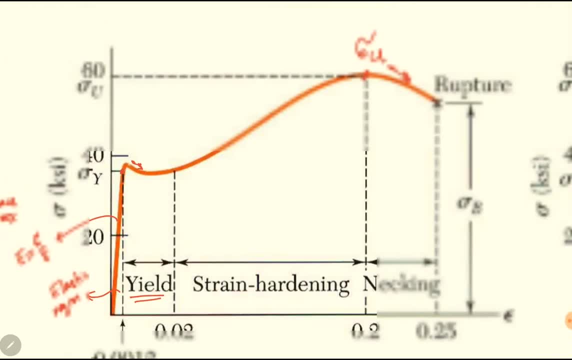 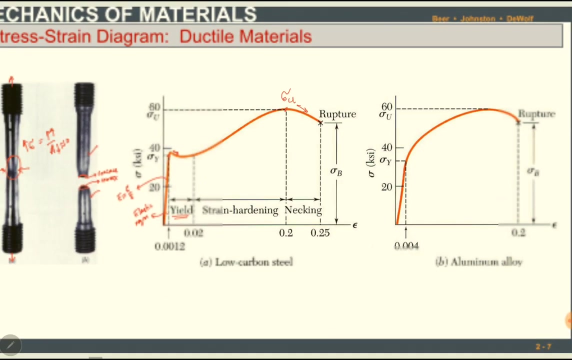 one equilibrium state to another equilibrium state. So this region is called yielding region After lower yield point. in some materials we cannot even observe this yielding region. There is no separate upper yield and lower yield point. So in some of the materials we can observe it. in some of them we cannot. 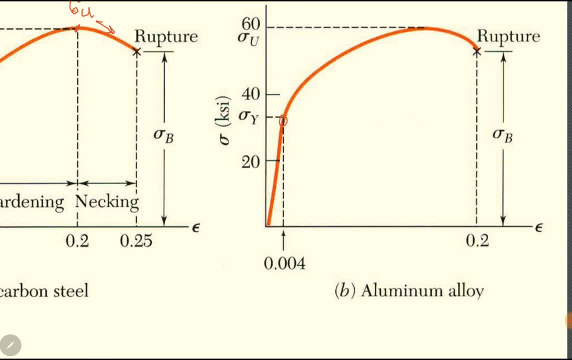 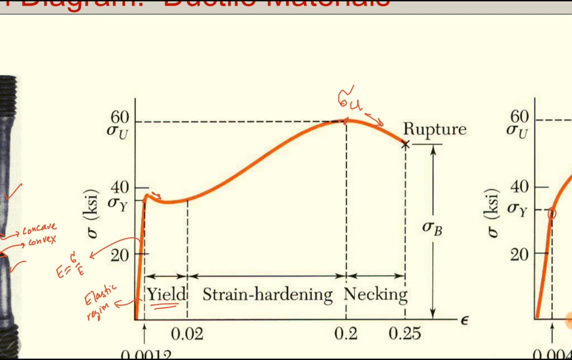 Like in the aluminum alloy. here we can see, After yielding point the stress will keep on increasing, So we cannot observe the yielding region at the macro scale. Then, after yielding, there is strain hardening. Strain hardening is a phenomena Which is actually the permanent deformation of a material without applying load. 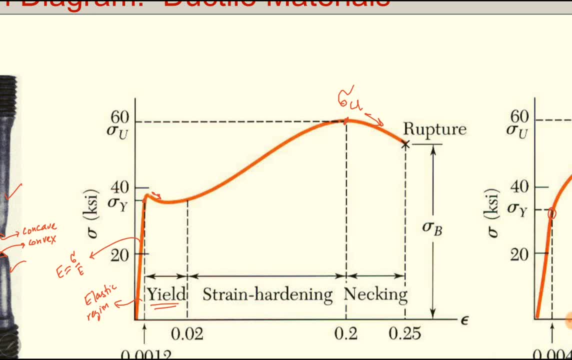 It is just like hot working. we have discussed in material sciences subject That if a material is deformed permanently by applying heat to it, By softening it through heating And then permanently changing its shape, it is called hot working. But if we change the shape of a material without applying heat, 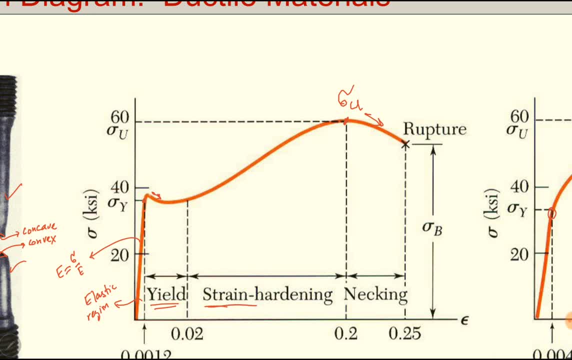 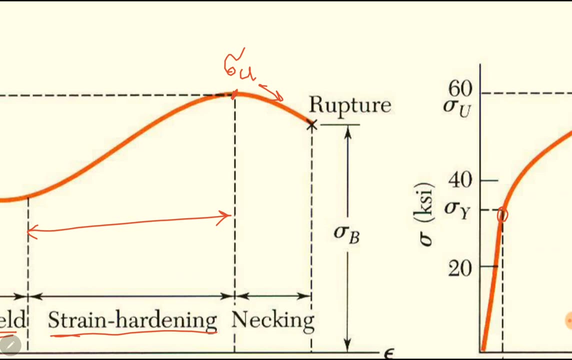 It is called cold working or strain hardening. So this region is actually a permanent deformation region without applying heat. So that is why this is called strain hardening region. And after ultimate limit, until fracture, as I have discussed earlier, That cross sectional area starts decreasing. 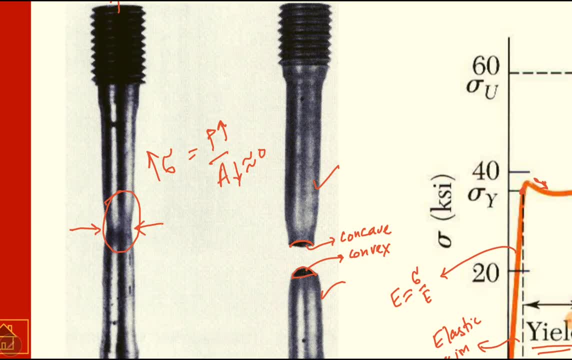 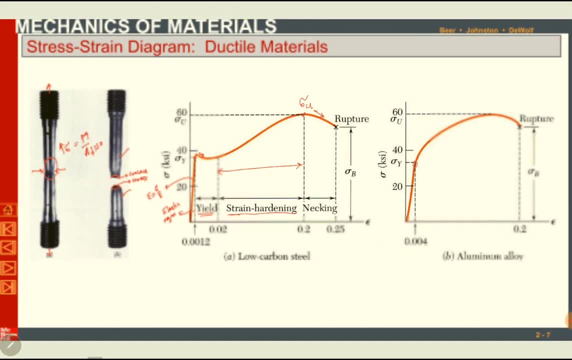 Just like this one. This is called necking region, This is necking phenomena And after necking, the material ruptures or fractures. These detailed points, the proportional limit, the elastic limit, the upper yield and lower yield, The yielding region, The necking, They are not all visible for all materials. 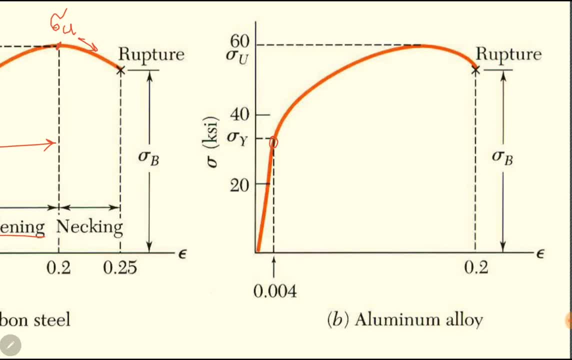 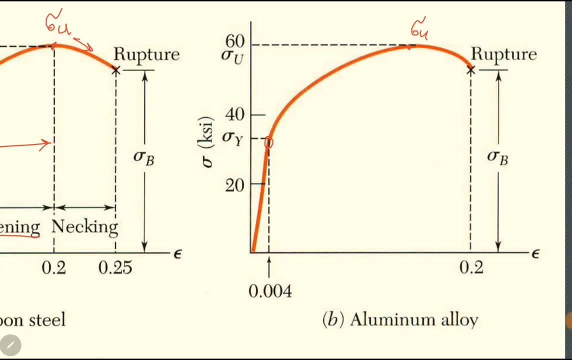 For some of the material we cannot even see the upper and lower yield points And there will be single yield strength point And then there will be ultimate And then rupture. For us usually the elastic region is important. This is elastic region And from the slope of the first linear relationship between stress and strain. 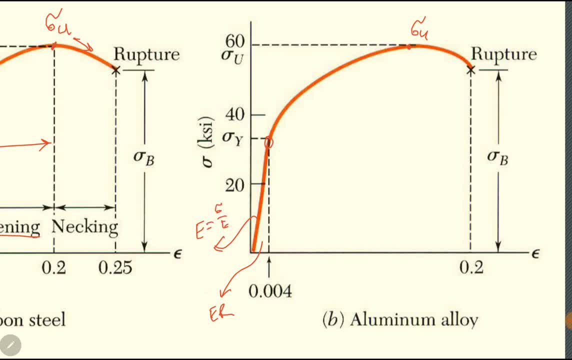 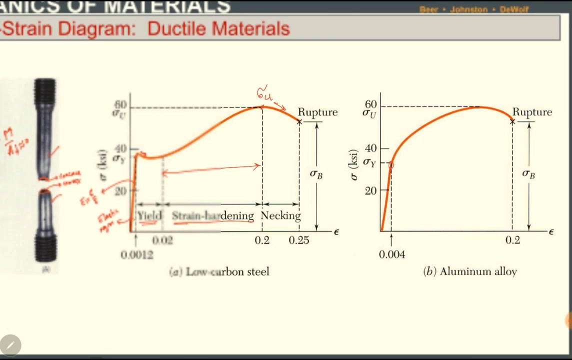 We can find E Modules of elasticity And then we have ultimate strength. These are some of the important points in the stress-strain diagram. Yield point is important, Sigma Y, Ultimate strength is important, Sigma U And then Strain at break up. This is also important. Okay, These two diagrams shown on the screen are for ductile materials. 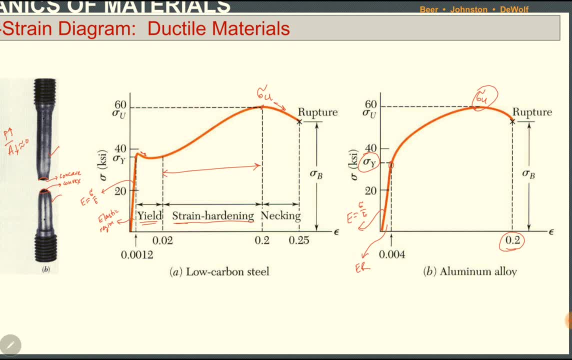 Ductile materials are those materials which can be drawn into wire shape by applying force. Ductile materials are those materials which can be deformed permanently. Usually you can deform most of the metals permanently. You take a metal wire or a metal body of any shape. 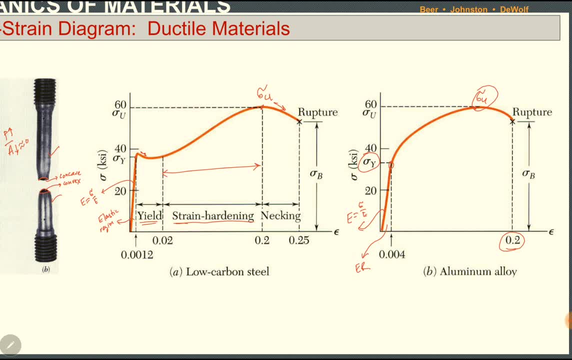 You can deform it permanently by applying force. A very simple example is a bubble gum. You can achieve it and you can deform it by applying force. You can make any shape out of it. Most of the polymers are actually ductile materials. Even rubber is a ductile material. 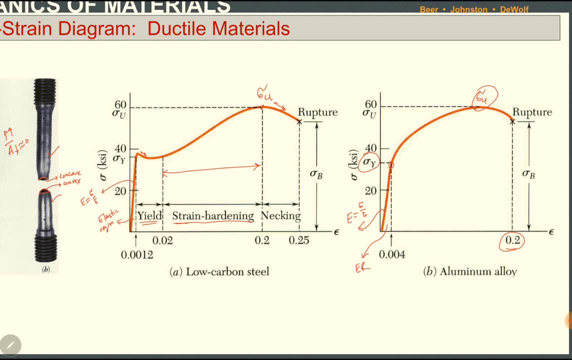 But it is a super elastic material. You can see elasticity. You can observe elasticity at macro scale. Once you apply force on a rubber Or any other polymer, You can see deformation in it And after removing the force, You can see that it will return to its original position. 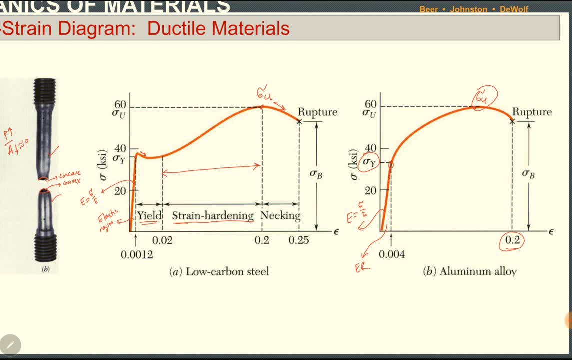 But if you keep on increasing the load, There will be a point that after that The material will not return to its original position And it will keep on deforming permanently. Such kind of materials are called ductile materials. Polymers are an example of ductile materials. 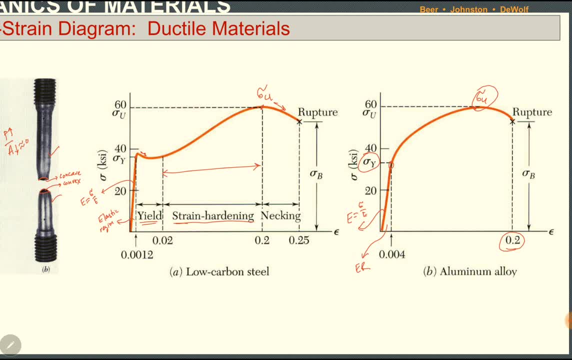 Most of the metals are ductile materials. Low carbon steel is here in front of you. Aluminum alloys are mostly ductile materials. Then there is another type of material Which is called brittle material. Like glass is a material. If we apply force on glass, It will deform If we remove the force. 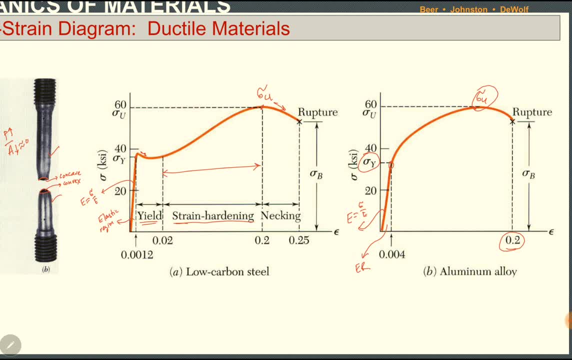 It will return to its original position. Most of the time. we cannot observe it at macro scale, But on micro scale The glass deforms elastically And after removal of the load It will return to its original position. But if we keep on increasing the load It will fracture suddenly. 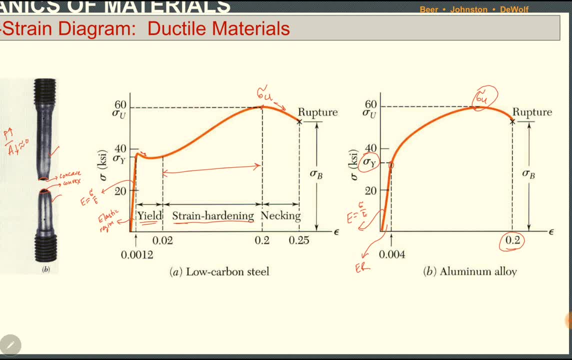 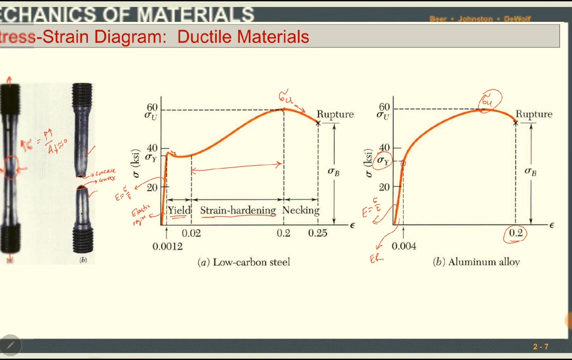 You cannot produce permanent deformation In glass at room temperature. It will fracture suddenly. So the brittle materials cannot be deformed permanently, Just like polymers and metals. You cannot simply deform glass permanently At any force, So it will fracture if you cross its elastic limit. So brittle materials do not have yielding region. 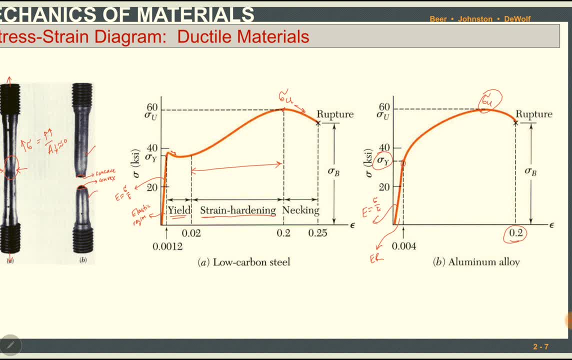 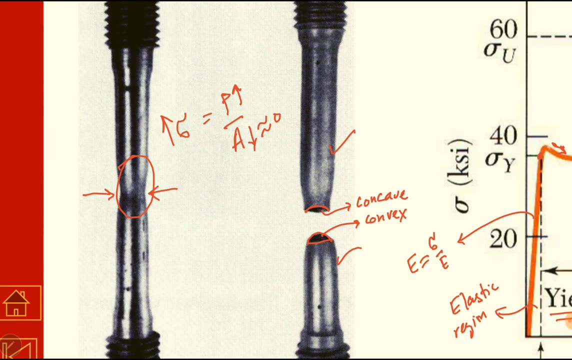 Or yielding strength. They do not undergo through yielding phenomena So they will directly rupture. They directly have ultimate strength. Even there is no necking in the brittle materials. You can see necking is actually permanent deformation. You can observe it If you remove the load. You can see the neck. 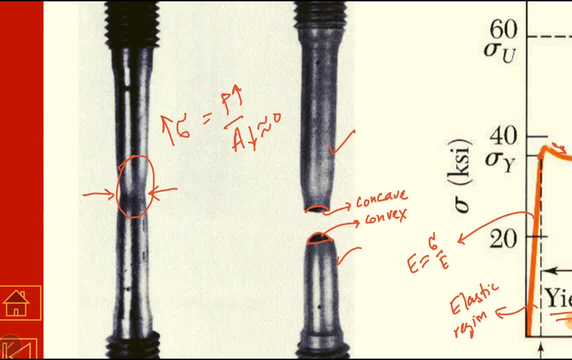 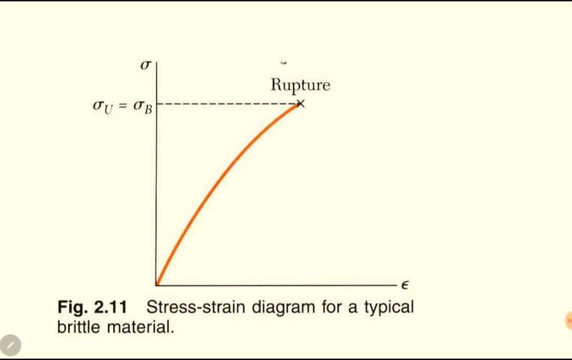 But in glass or in any other brittle material You cannot see a neck Or any kind of permanent deformation. So they will rupture suddenly. There is no permanent deformation. So for brittle materials We have this kind of curve. There is an elastic region And there is only an elastic region. 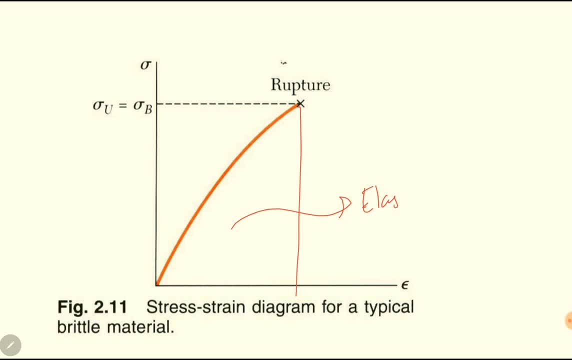 This whole region is elastic region, For brittle materials only. Okay, The slope of this line will be E, It is modulus of elasticity, And then there will be sigma ultimate, Which is also sigma rupture. There is no sigma yielding. There is no sigma y for brittle materials. They do not undergo yielding. 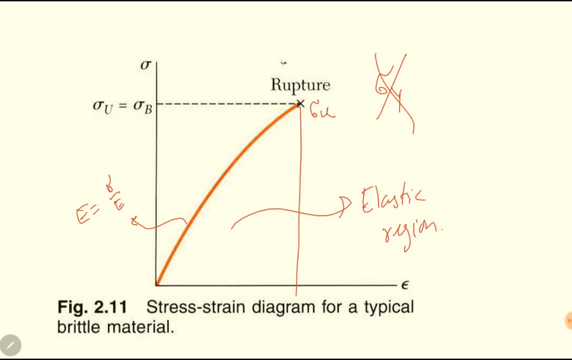 They do not undergo permanent deformation. They do not undergo a change of equilibrium state At atomic level. The change, The only change, will be a fracture. The bond will be broken permanently. It cannot be deformed. The bond will be fractured. actually, It will not be deformed permanently. 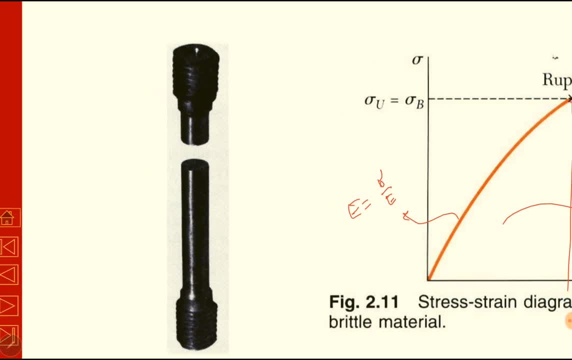 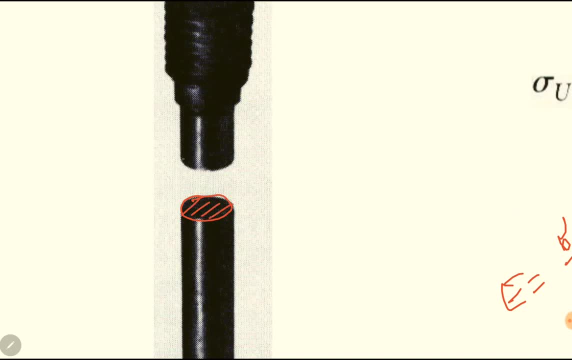 Okay, And there is no cup and cone shape after fracture. There will be planar fracture. You can see This is a plane. Similarly, at this level, there will be a plane. There is no cup and cone raised shape And a cup shape, Concave or convex surfaces. There will be planar surfaces. 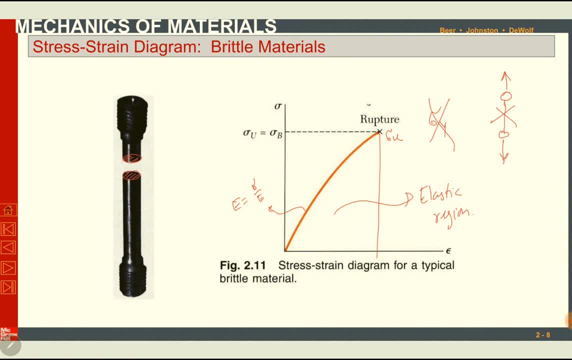 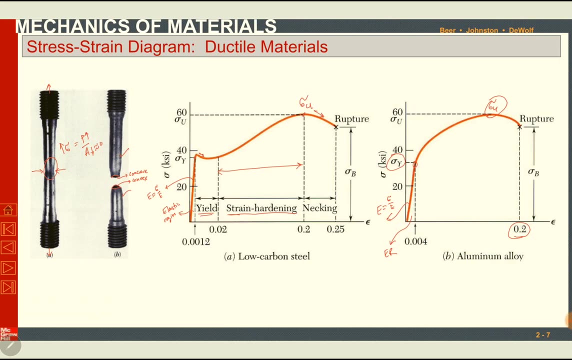 Okay, So brittle materials do not deform permanently. Ductile materials deform permanently And the stress and curves are different Than each other. Brittle materials have only elastic region. Ductile materials have elastic region, Yielding region And then plastic region Or permanent deformation region, Which is also called strain hardening region. 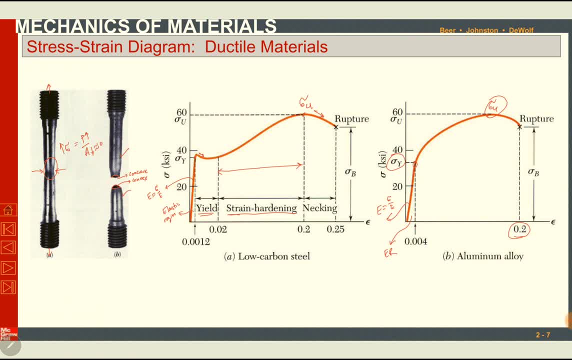 And then there is necking. So the stress-strain curve of ductile materials Is usually a detailed one. If you can understand stress-strain curve of a ductile material, So this subject will be very easy for you. Usually, the study of materials will be very easy for you. 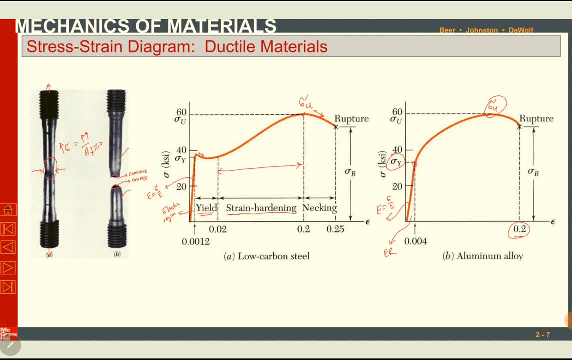 Because Behavior of ductile materials is very detailed one. There are so many minor points, So many details in this diagram, And this is totally a conceptual diagram. By understanding this diagram, You can understand the behavior of a material. What is going on inside a material? under load, A similar kind of behavior can be seen. 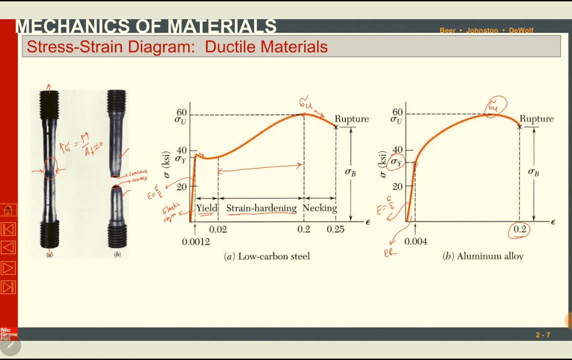 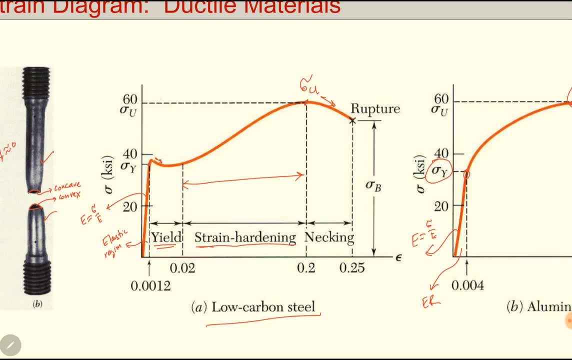 Under compressive load as well, A similar shape of diagram will be made. Numerical values can be different. For example, For a low carbon steel, Ultimate strength is almost 60 KSI Under tensile load. It can be different under compressive load, But shape of diagram will be same. 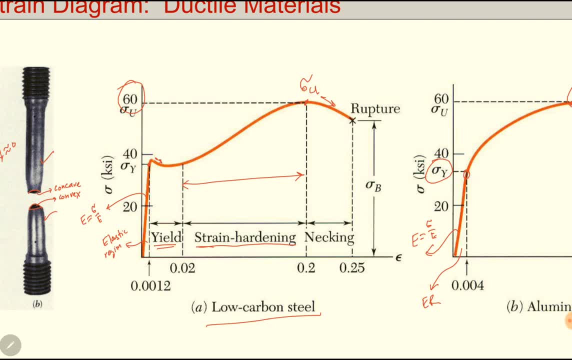 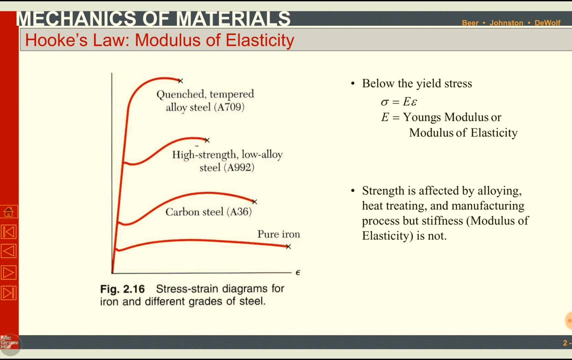 Similarly, there will be ultimate strength under compression, Yielding strength under compression, There will be elastic region, There will be plastic region, There will be strain hardening, But there will be no necking under compression load. Okay, Then We are further studying about models of elasticity Under Hooke's law. 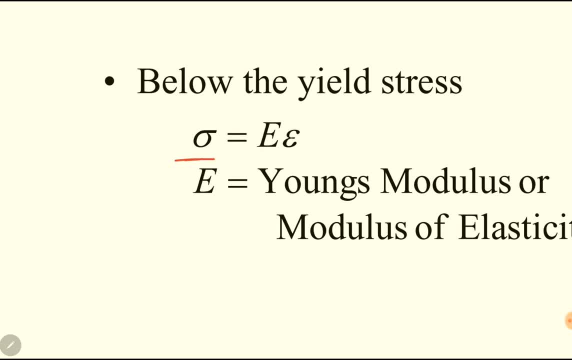 As we have discussed, that Stress is equal to E into strain. This is Hooke's law. This is applicable only to the elastic region. This law cannot be applied beyond yield strength. This is applicable only before the yield limit, Before the yield strength point. Okay, Now, if you see, 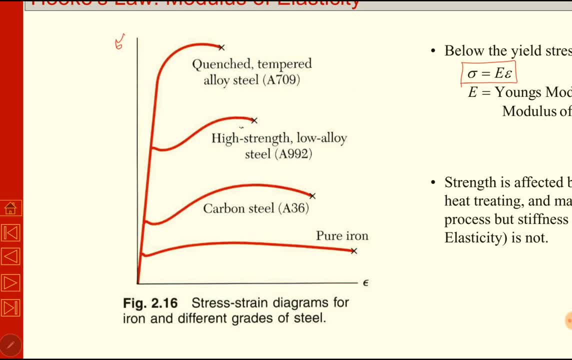 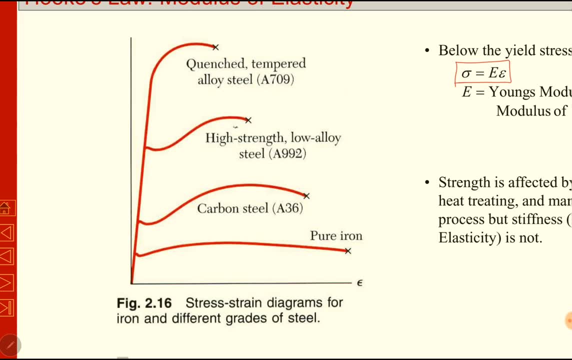 There are stress-strain diagrams For different alloys of steel, Of iron. actually We can see The first one is for pure iron, Then there is for carbon steel- A36- Then there is high strength, low alloy steel- A992. There are different grades of steel. actually, A992 is a grade of steel. 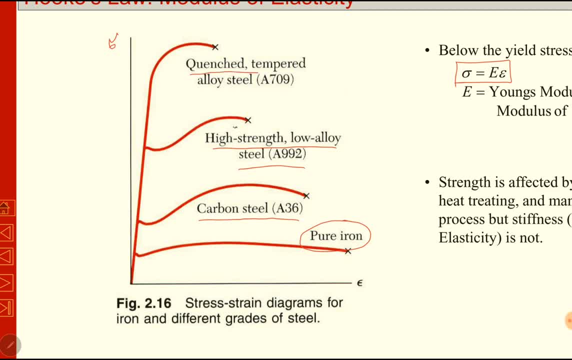 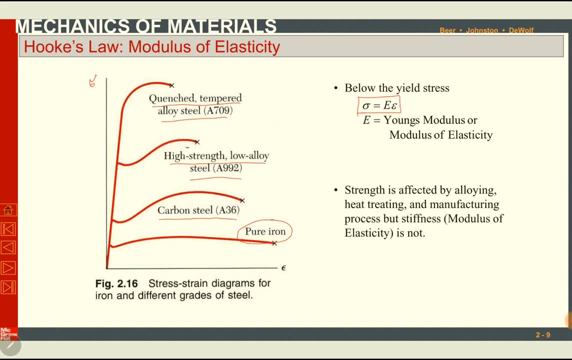 A36 is a grade of steel. Then there is quenched steel, Then there is tempered alloy steel. Now What is the difference between all of them? Pure iron is pure, Okay. Then carbon steel is a different grade of steel. Then high strength, low alloy steel is an alloy of steel. 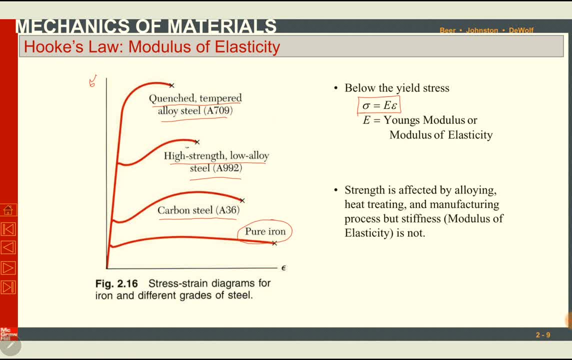 Then quenched. tempered alloy steel is again a heat treated alloy of steel. We have treated it with tempering and then quenching. You know what is tempering and quenching? Just simply heating up a material at certain temperature And then cooling it down. 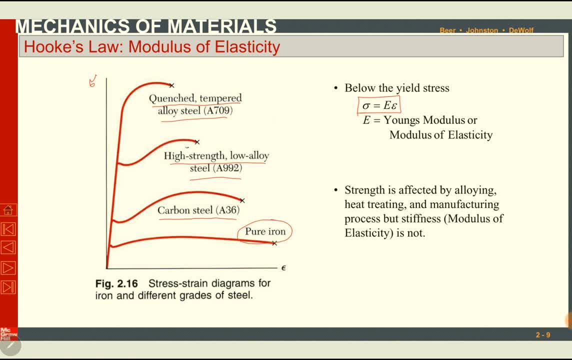 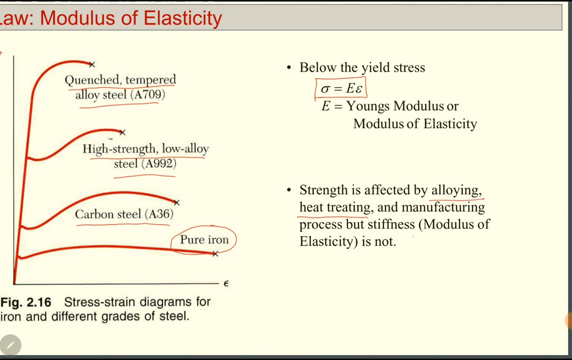 In the quenching. we can simply cool down a material in an oven. So under different heat treatment conditions. You know it from your basic knowledge of engineering, materials, Material science, sorry. So By applying different heat treatment conditions And different heat treatment processes, Or by allowing the material 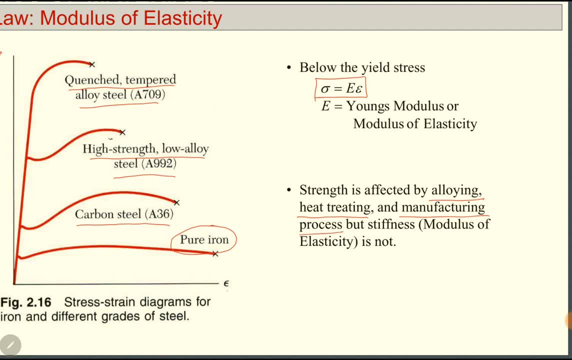 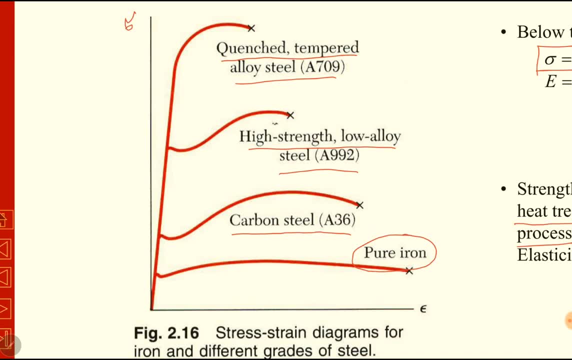 Or by applying different manufacturing processes, What we can do with the material. We can see, for all the grades of steel, This initial line, This line Is same. The slope of the line is same Slope is E, which is sigma over epsilon. So, for all the grades of steel, 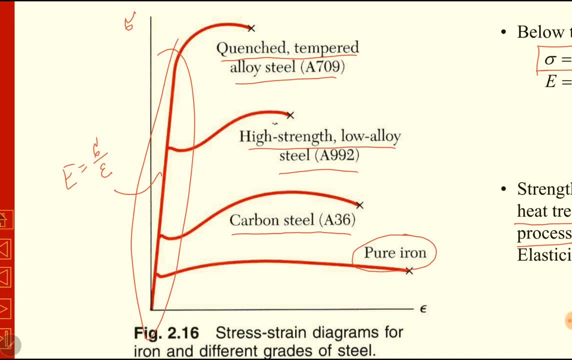 Either manufactured through different manufacturing process, Or different alloys of steel, Or heat treated with different processes, Or untreated alloy of steel. For all of them, E is same. E is slope of this initial line And slope of the line is same for all of them. But we can see. 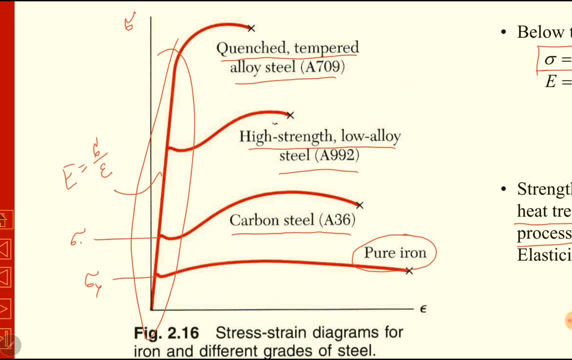 This is sigma yield. This is sigma yield for the different grade. This is sigma yield for high strength low alloy steel. This is sigma yield for quenched tempered low alloy steel. For all of the, For all different grades of steel, Sigma yield is different, So yield strength is different. 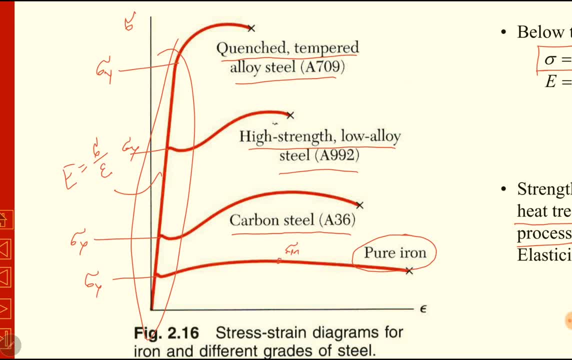 Similarly, sigma ultimate For pure iron, Sigma ultimate for carbon steel, Sigma ultimate for high strength low alloy steel And sigma ultimate for quenched tempered low alloy steel Is different. So yield strength and sigma strength, Ultimate strength, are different. Similarly, rupture Strength is different. Similarly, elongation, Elongation or strength at rupture. 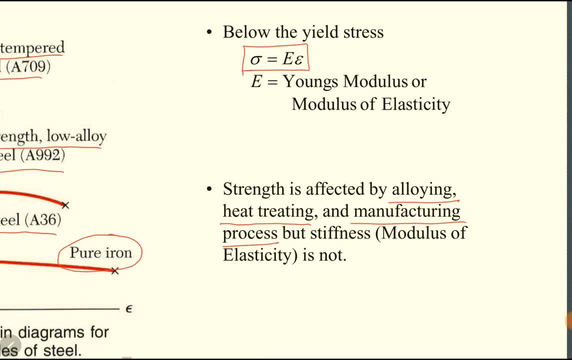 Is different. These values are different. So we can say that Strength, Ultimate strength, or yield strength, Even strength. It can be affected by Alloying, Heat treating And manufacturing processes, But E modulus of elasticity Cannot be changed, Cannot be affected. So modulus of elasticity Are stiffness. Modulus of elasticity of a material is actually calculated. 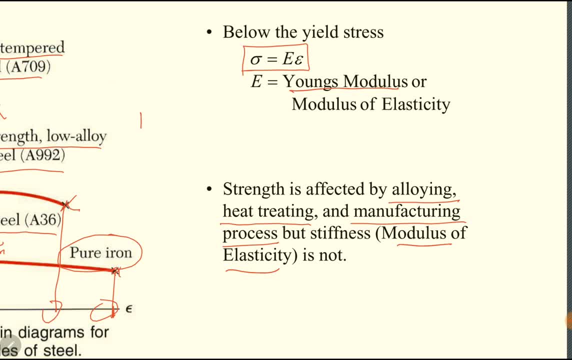 From the stiffness of the material. Stiffness Is force divided by Deformation- This is again by Hooke's law- And modulus of elasticity is stress divided by strain. They both are resistance against deformation. Stiffness is resistance against deformation, E is resistance against strain. So stiffness or modulus of elasticity of a material, 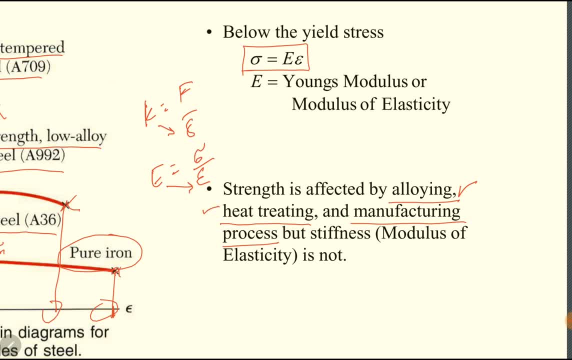 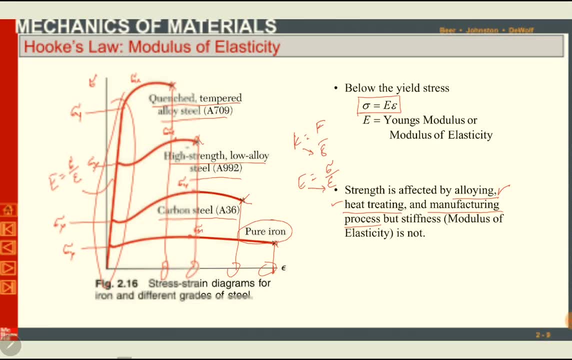 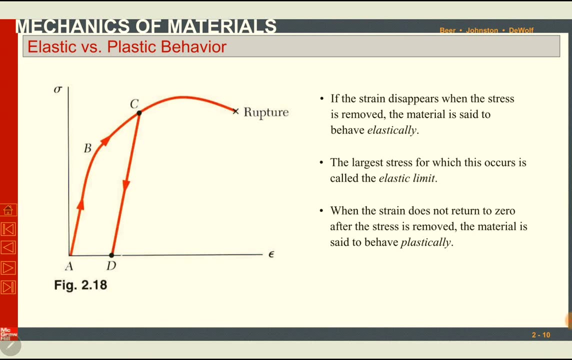 Cannot be changed Using alloying, Heat treatment Or manufacturing processes, But strength can be changed. Even strain can be changed. So next topic is Elastic versus plastic behavior. We have discussed in detail that. What is elasticity And what is elastic limit, What is plastic region And what is plastic behavior? 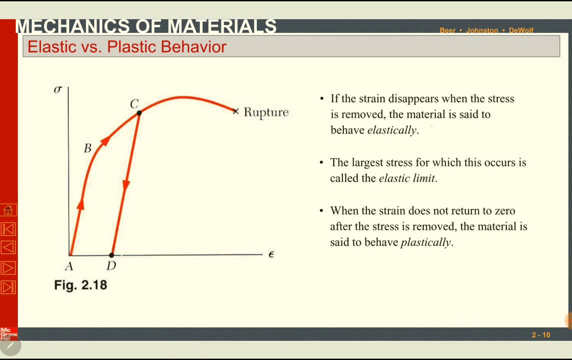 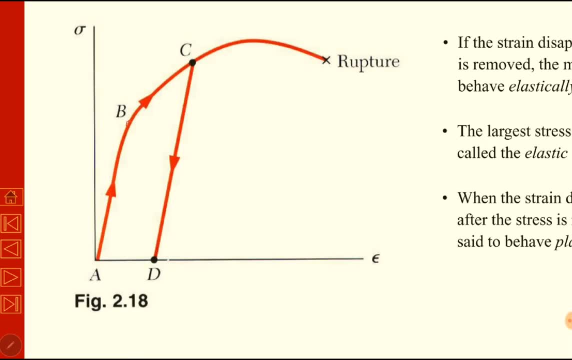 Again, If the strain disappears, When stress is removed, The material is said to behave elastically. For example, In this stress-strain diagram Before point B: If we remove the load, The material will return to Its original position And it will behave elastically. This behavior is called elastic behavior. 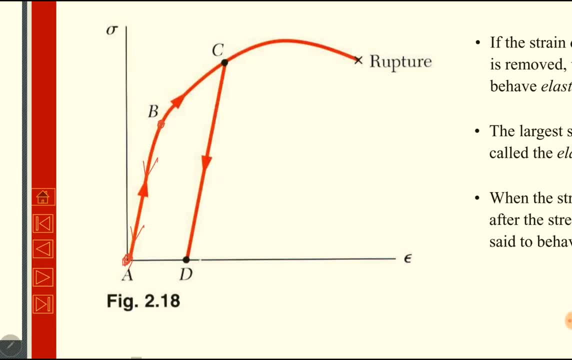 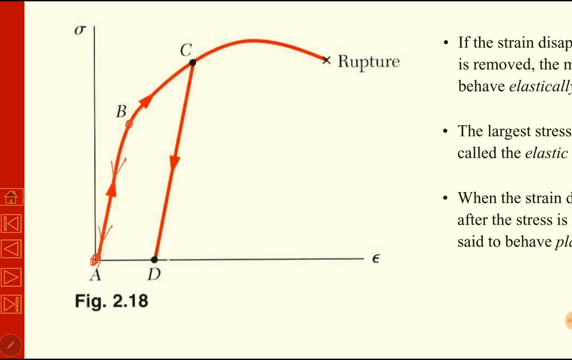 Largest stress for which this occurs Is called elastic limit. So this point B Here Below which The material will return to its original position After removing the load, This point is called elastic limit. We also call it yield limit Or yield strength, When the strain does not return to zero. 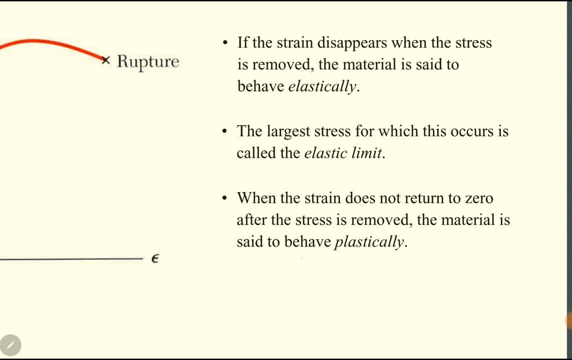 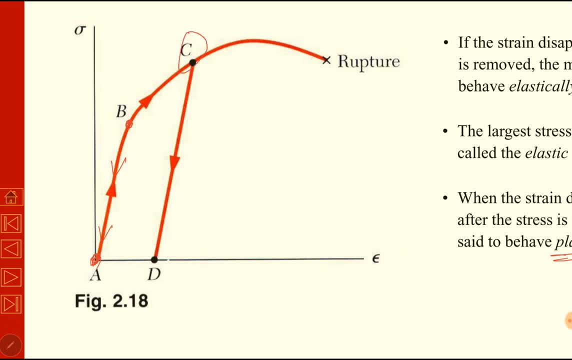 After the stress is removed, The material is said to behave elastically Beyond this point B At any point, For example at point C, If we remove the load, This material will return to point D. At point D, Strain is not zero. This strain is not zero. We can see that on the horizontal axis. 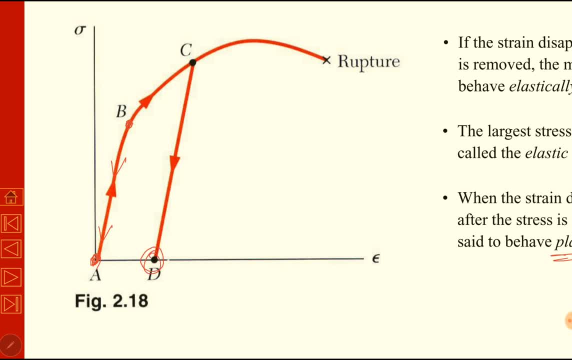 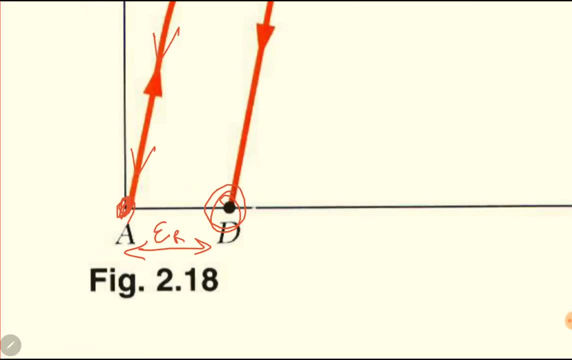 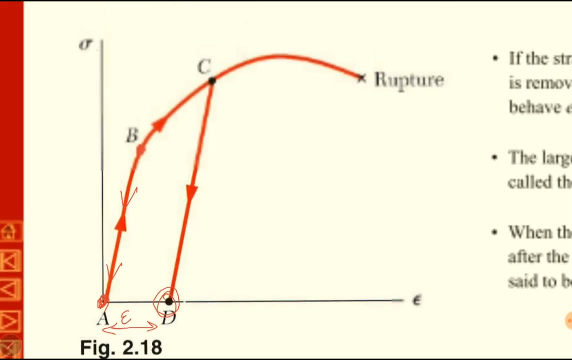 There is Some strain at point D. This much strain, This Permanent strain, Is called residual strain. There is no stress at this point. At point B, Sigma is zero, Because sigma lies at the vertical axis And point D is on the horizontal axis. So at point D, Sigma is zero. 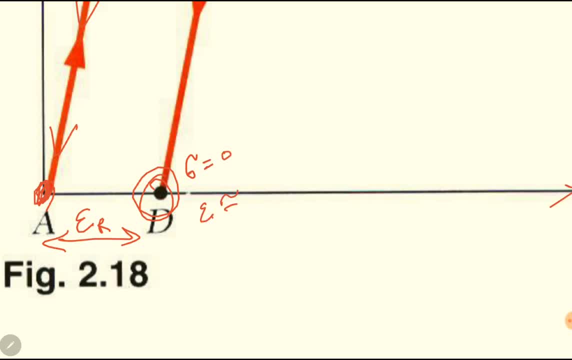 There is no stress, But there is No strain. But there is strain. actually There is permanent deformation. If there is strain, It means there is deformation. So in the absence of stress, If there is strain, That strain is actually permanent strain. This strain exists without external load, Without stress. 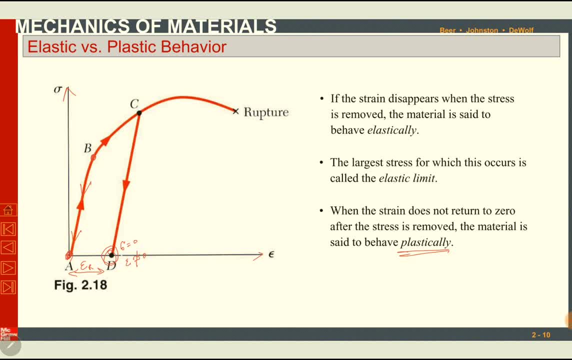 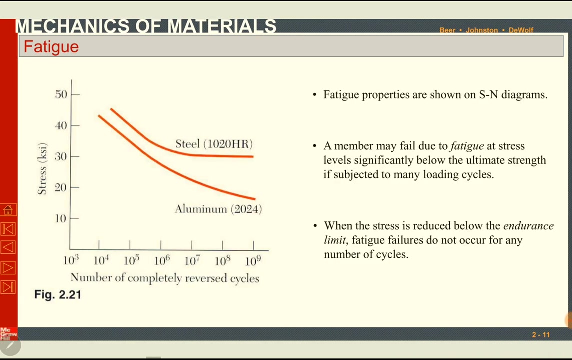 So such kind of material Is called to behave plastically And this region After point B, Tail point Ultimate, This is plastic region And the behaviour of the material is called Plastic behaviour, But before point B The behaviour is called Elastic behaviour. Okay, Our next topic is Fatigue. 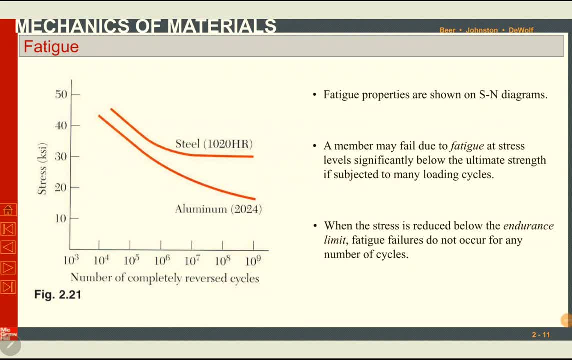 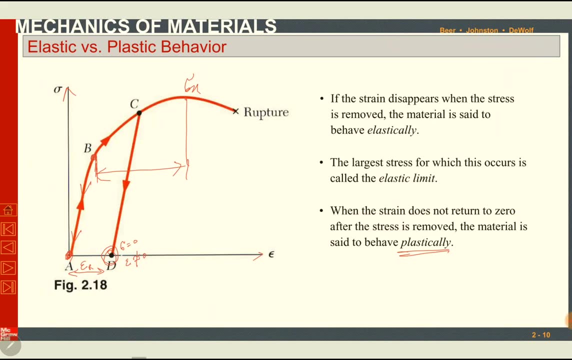 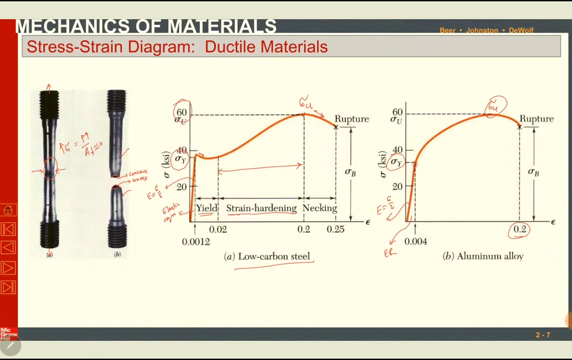 Fatigue is actually Failure of a material Under Cyclic loading, Under repeated load. Previously we have discussed Failure, Behaviour of a material Or behaviour of a material Under static loading. The stress-strain diagram Discussed earlier was Behaviour of a material under static load: Static tensile or static compressive load. 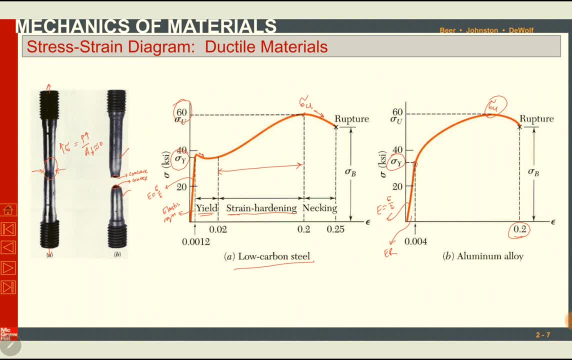 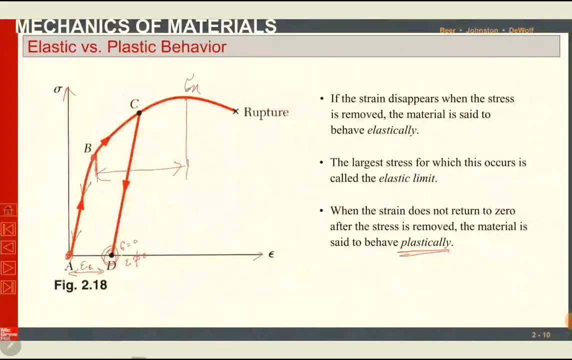 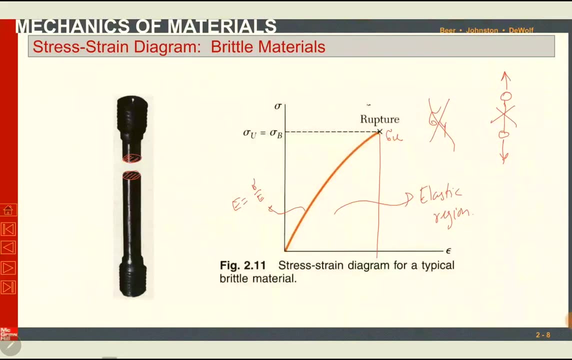 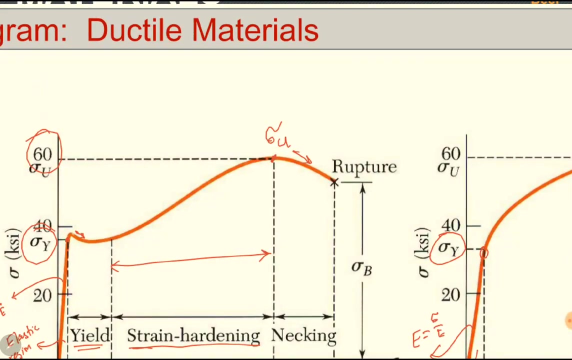 But if the load is not static, If it is repeated, If it is cyclic, Then the behaviour will be different At different number of cycles. The material may fail At different Values of stress. Under Under normal loading, Normal static load, A material Fractures Or permanently Fails at two different 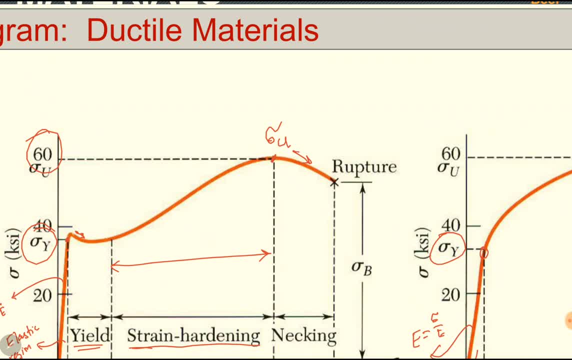 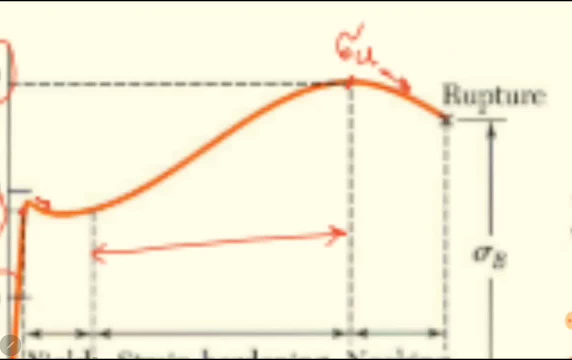 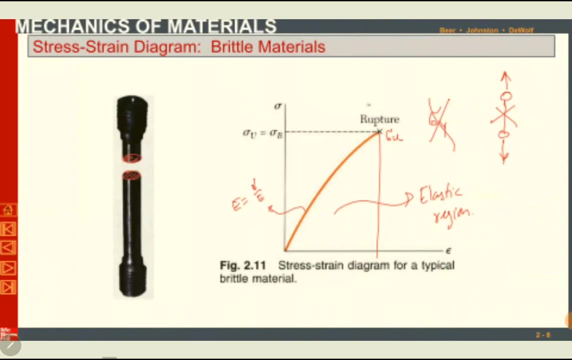 Permanently deforms At two different values of stress. It permanently Deforms at Yield strength Or sigma y, Yield stress, And It fractures after Ultimate strength. Similarly, a brittle material will fracture After ultimate strength. If the load is below the ultimate stress, The brittle material will not fail. 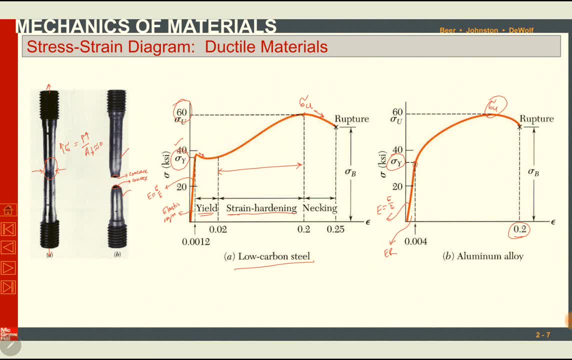 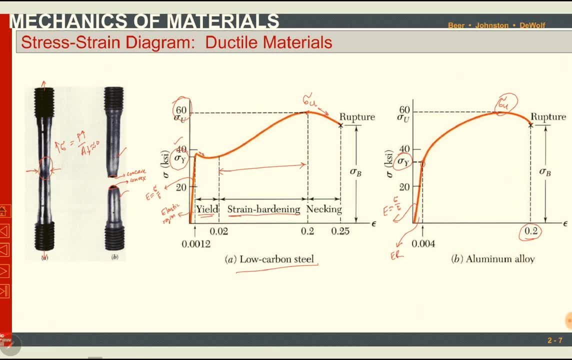 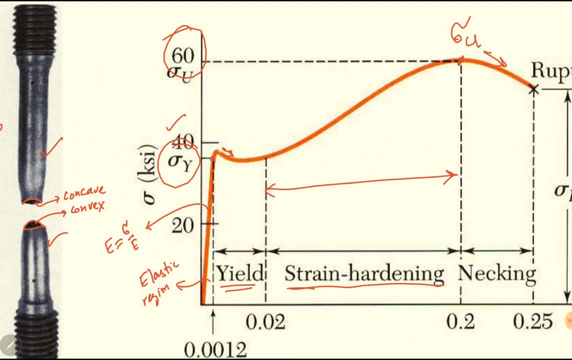 And if the load is below the yield limit Of a ductile material, The material will not deform permanently. But sometimes a material may fail Even before the yield stress. A ductile material may fail Or even may fracture Before this yield stress. It may fracture somewhere In this region. 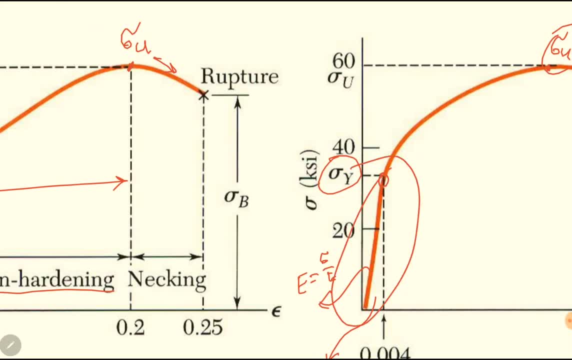 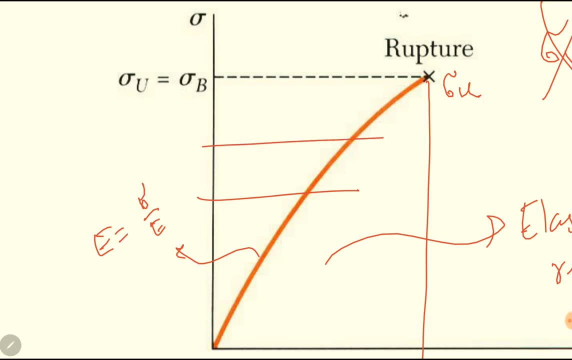 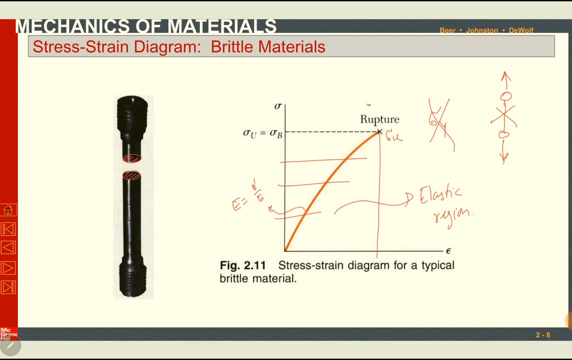 In this elastic region, Here Or a brittle material may fail Before, Before ultimate stress, Somewhere, here Or here Or here, At lower values of stress. This is only possible If the load is not static, If the load is repeated. So such kind of Failure is called fatigue failure. 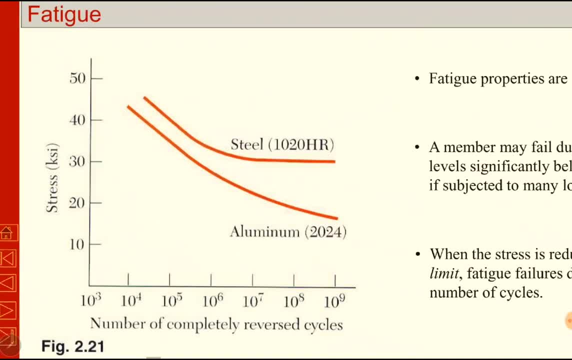 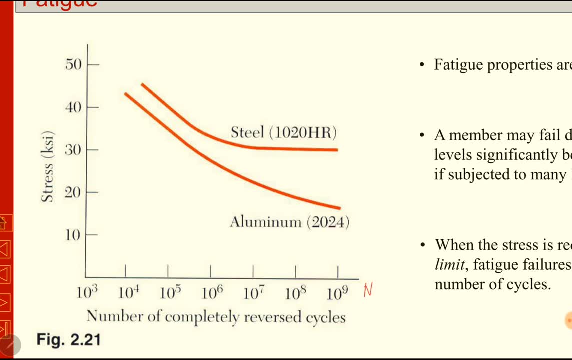 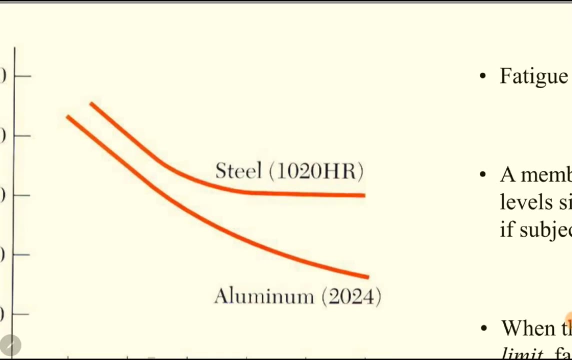 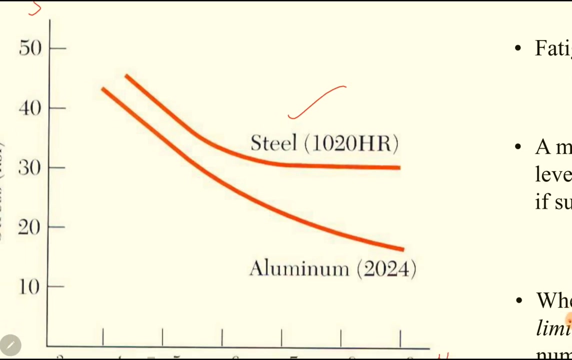 Here is a Diagram given Between Stress And the number of cycles of the load. The horizontal axis Shows number of cycles of load And the vertical axis Is stress. So you can see, For example, This curve Is for steel 1020 Grade of steel. This grade of steel. 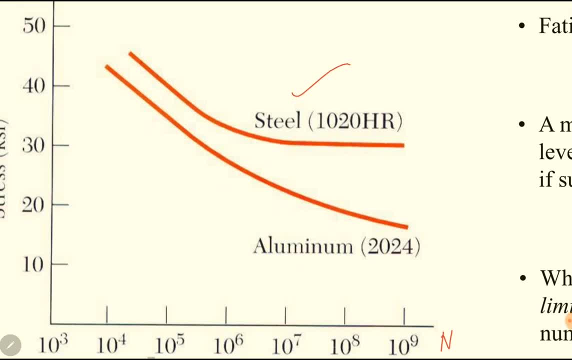 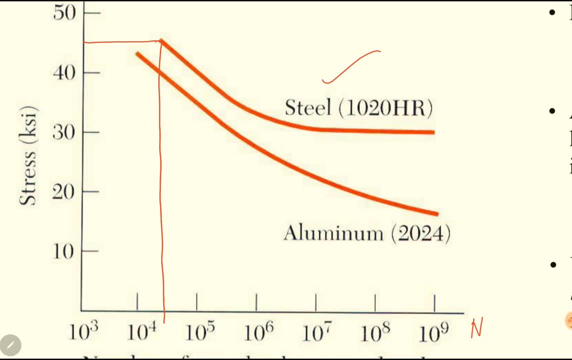 May fail at Somewhere Near 50 KSI, Around 45 KSI. It may fail At number of loading cycle Somewhere between 10 power 4 and 10 power 5. Similarly, It will fail At 40 KSI of stress, At about 10 power 5. 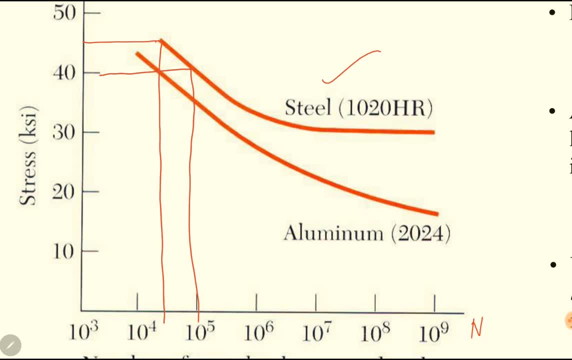 Number of loads. Number of loads. So this is not a static load. In static, Under static load, The number of cycles are: The number of cycles is just single one Equal to one. But If the number of cycles are About 10, power 5 For steel 1020. 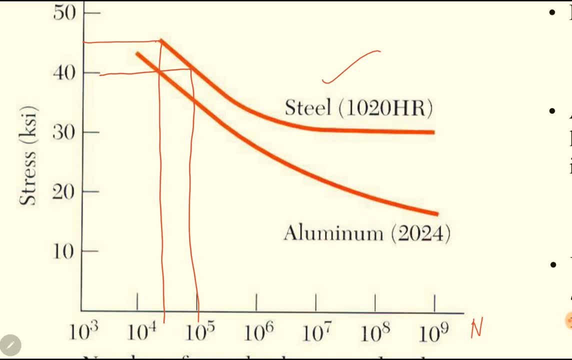 It may fail At even 40 KSI Of stress. So As soon as we increase The number of loads of the cycle, We can see that the material will fail At even Lower values of Stress. So the stress At which a material fails Is inversely proportional to the 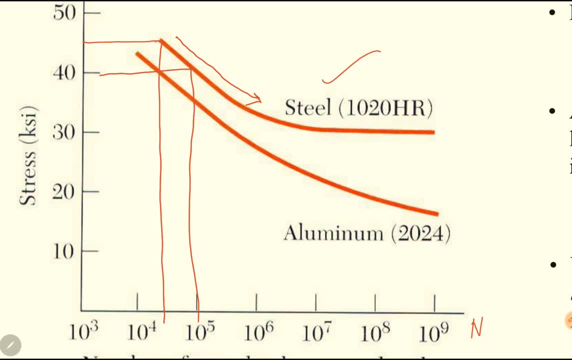 Number of loading cycles. At higher number of loading cycles, The material will fail At even lower values of stress. This value of stress Will be Even Lesser than the Yield strength Of the material for ductile Materials And it will be lower than the ultimate For Britten materials. 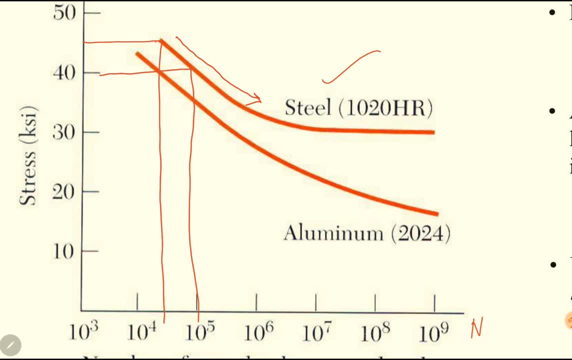 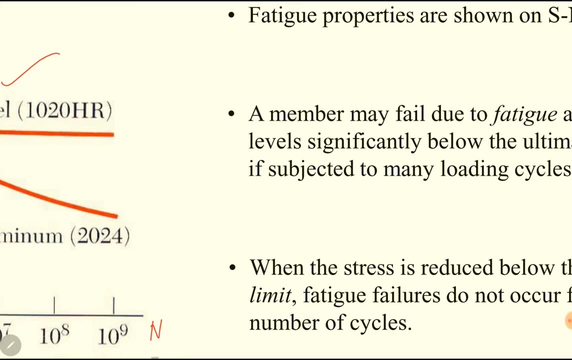 Because Britten materials do not Undergo yielding, So Fatigue failure Is even Dangerous. Material may fail Below At a stress level, Below the defined strength, Below the defined static strength of the Material. Ok, So A member may fail Due to fatigue At a stress level Significantly below the ultimate strength. 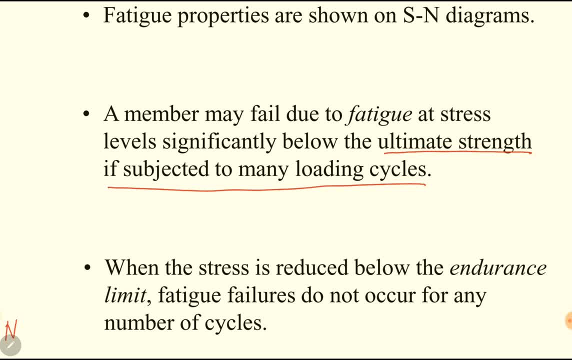 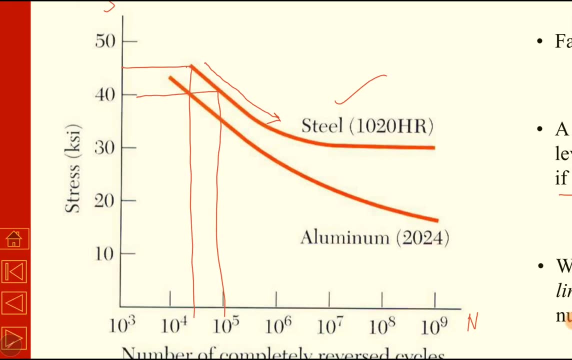 If subjected to many loading cycles Below the ultimate strength, It can be even below the Yield strength For a ductile material At a very high number of loading cycles. Ok, So At higher number of loading cycles, Thus Failure stress is low. Then, If we look at this curve, 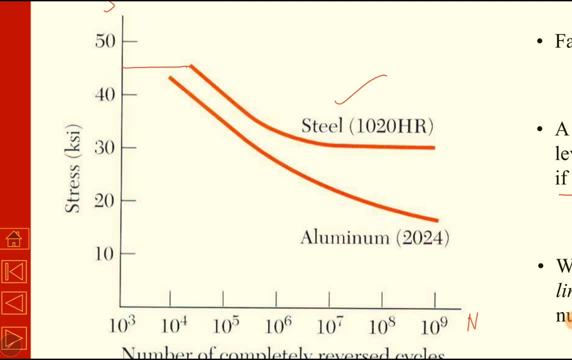 This SN curve Between stress and number of cycles. We can see that This curve Has got flattened horizontally At some level, For example At 30 KSI. It has flattened At around 10 power 7. Number of cycles After this: For any number of cycles Above 10 power 7. 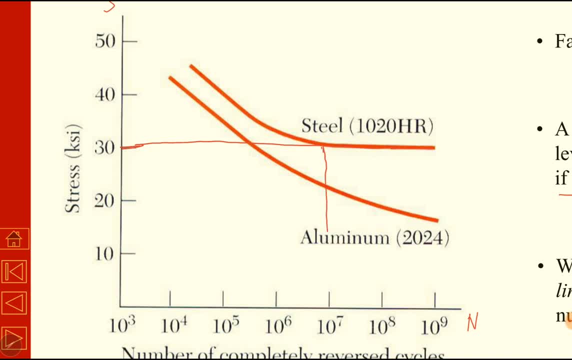 Number of cycles After this: For any number of cycles Above 10 power 7. Number of cycles After this: For any number of cycles Above 10 power 7. Number of cycles Above 10 power 7. For example, At 10 power 8 Or 10 power 9. 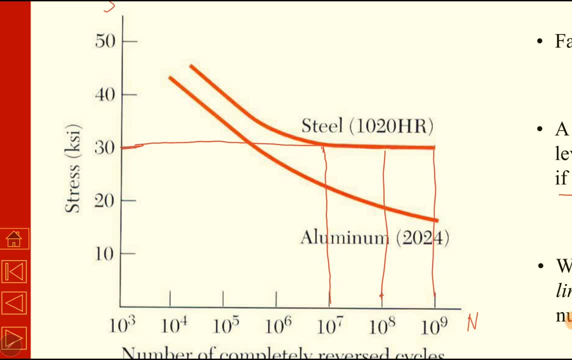 The failure stress is The same. It is 30 KSI For this specific material of steel. So This 30 KSI Is actually The endurance limit Of this material If the Stress is Below 30 KSI, If it is Like 20 KSI. So This line: 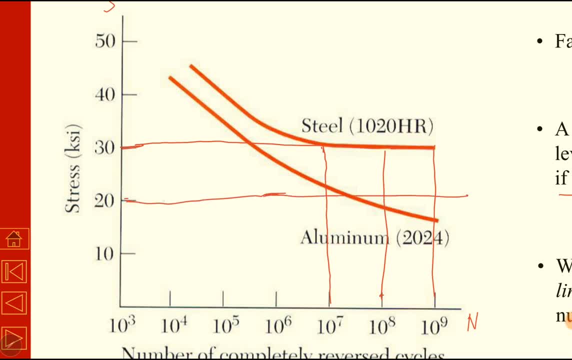 This horizontal line Is Below 30 KSI. So This horizontal line Of 20 KSI, Of 20 KSI, Stress Does not touch This curve Of steel SN curve Of steel 1020. It means Steel 1020 Is safe For Safe At any Value of stress. 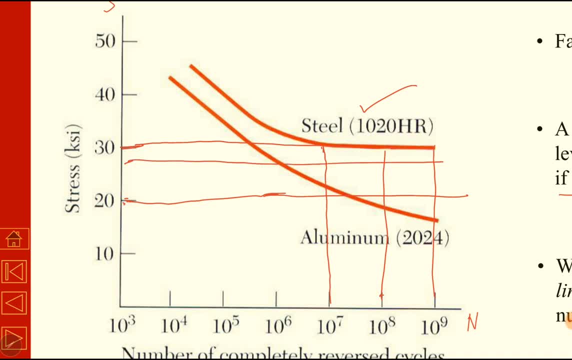 Below 30 KSI. Any value of stress Below 30 KSI Does not touch This curve For any number of Loading cycles. So 30 KSI Is the fatigue Strength Of this material Or endurance Strength Of this material. Endurance Strength Or fatigue Strength Is the value. 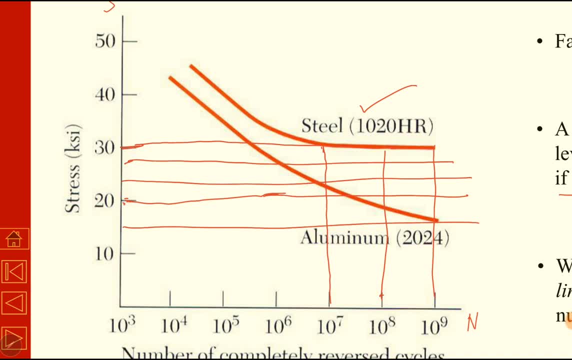 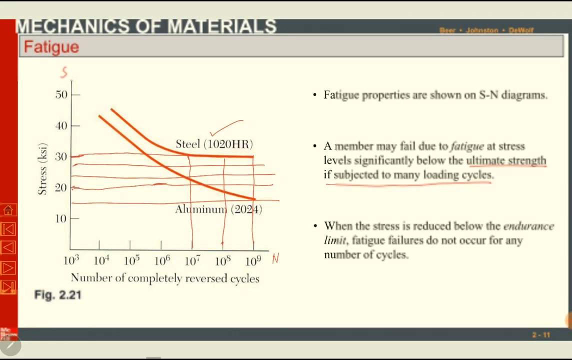 Of stress Below Which A material Will never fail Under fatigue Loading For any Number Of loading Cycles. So Endurance Limit Is a Very Important Parameter For fatigue Loading. So For fatigue Loading, Endurance Limit Is an Important Parameter, But We Will Not Discuss Fatigue The Topic. 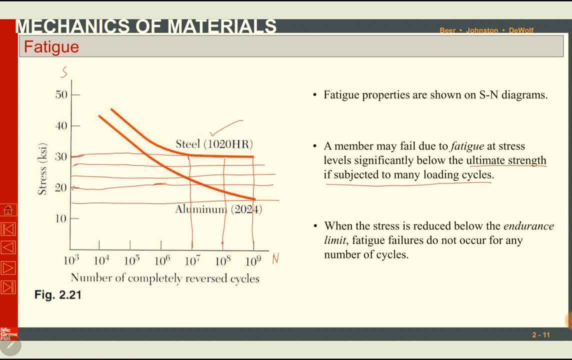 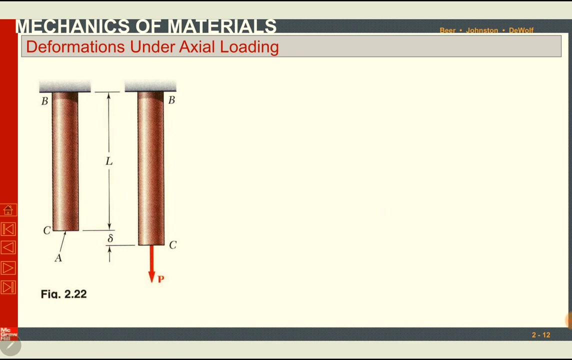 Of Fatigue In This Course In Detail For Introduction Purpose. This Slide Was For The Material Of Stress, And The Material Of Stress Is The Value Of Stress Below Which Material Will Not Fail For Any Number Of Loading Cycles. Theoretically It Is Under Axial Loading. 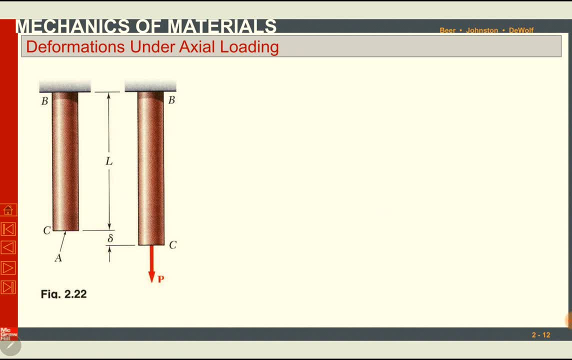 So Whenever We Apply Again, We Are Back To The Static Load, Normal Load. Whenever We Apply Normal Load, The Material Deforms The Length Of The Material In Elastic Limit. If A Material Is Not Deformed Plastically Within The Elastic Limit, We Can Use Hooks Law, Which Is: 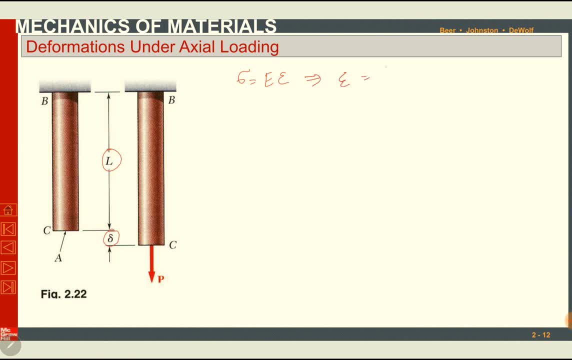 Sigma Is Equal To E Into Strain. Or We Can Write P Over A Because It Is Normal Load. So We Can Write P Over A Divided By E. Sigma Has Been Replaced With P Over A. We Can Write As Deformation Is Equal To Pl Over. 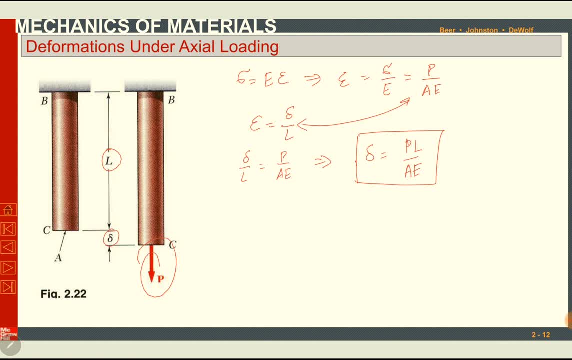 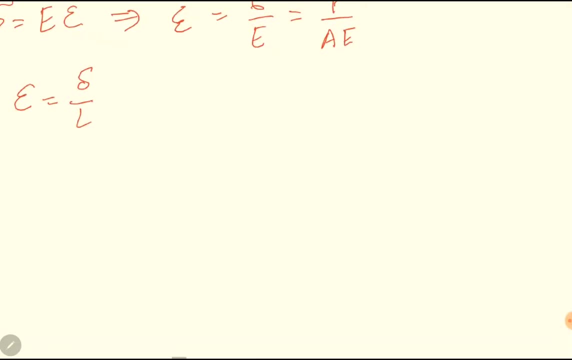 A, E. So Deformation Of Any Bar Can Be Calculated Using This Expression: Load Into Length Divided By Cross Section Area. P, Length And Area Is Geometry. Load, Geometry And Material. Material Property Here Is E, So Deformation Depends Upon These Three Parameters. Load, So One Of 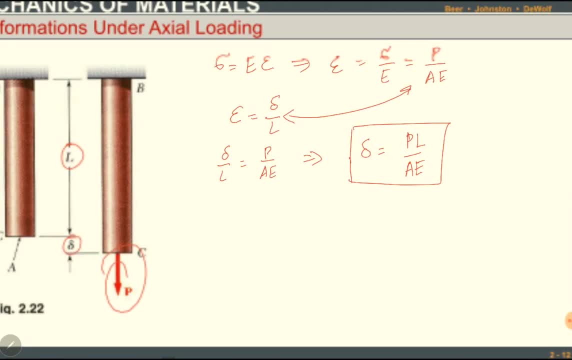 Them Is Changing. So We, For Example, We Have A Bar Where Area Is Consistently Changing. Here The Cross Section Area Is A 1. Here Cross Section Area Is A 1, 2, 3, 4, 5, 6, 7, 8, 9. 10, 11, 12, 13, 14, 15, 16, 17, 18, 19, 20, 21, 22, 23, 24, 25, 26, 27, 28, 28, 29, 30, 31, 32, 33, 34. 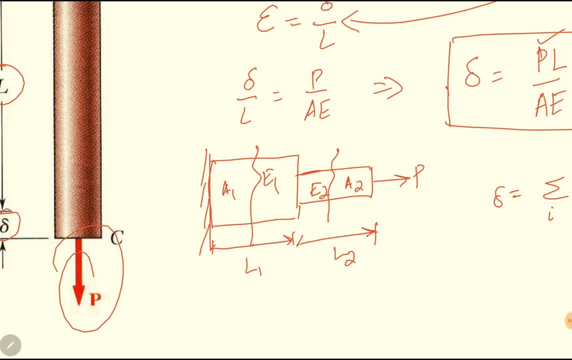 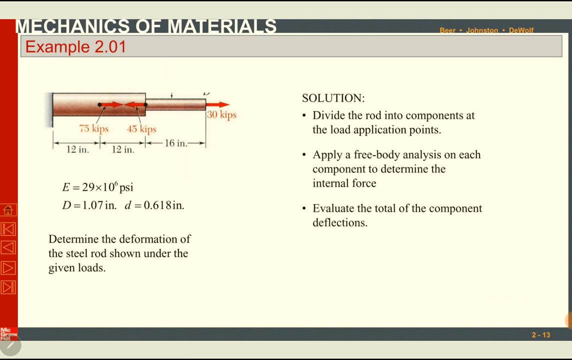 35, 36, 37, 38, 39, 40, 41, 42, 43, 44, 45, 46, 47, 48, 49, 50, 51, 52, 53, 53, 54, 55, 56, 57, 58, 59. 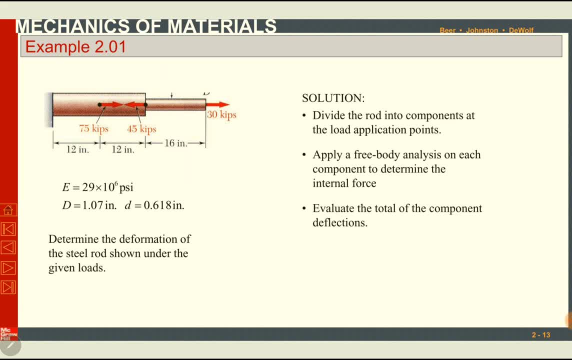 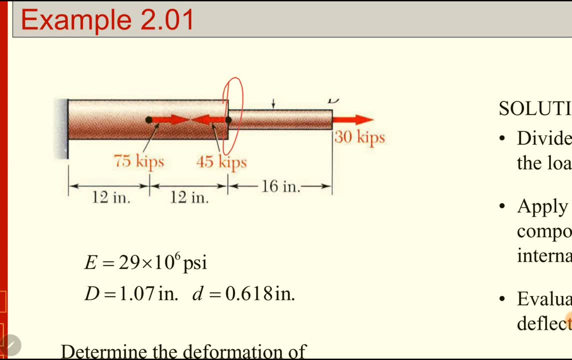 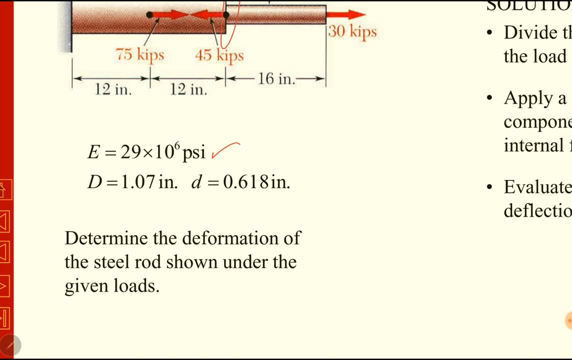 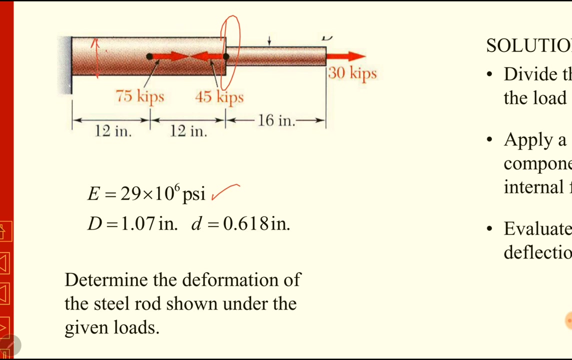 60, 61, 62, 63, 63, 64, 65, 66, 67, 68, 69, 69, 70, 71, 72, 73, 74, 75, 76, 77, 78, 79, 80, 81, 82, 83. 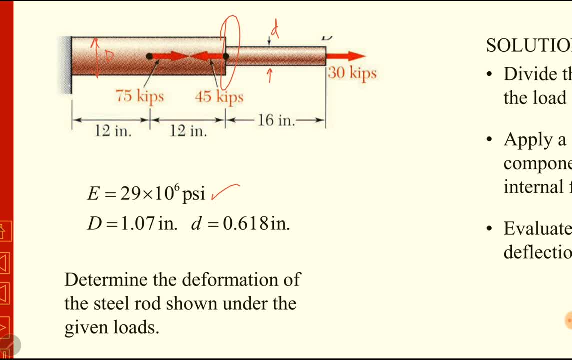 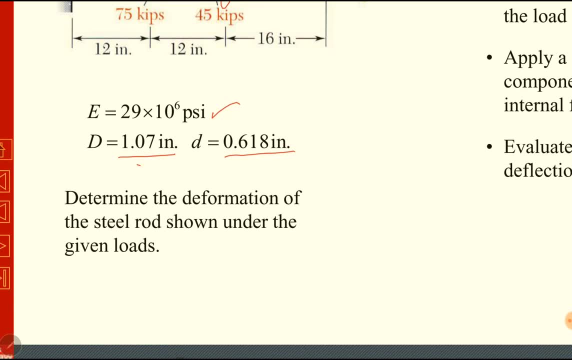 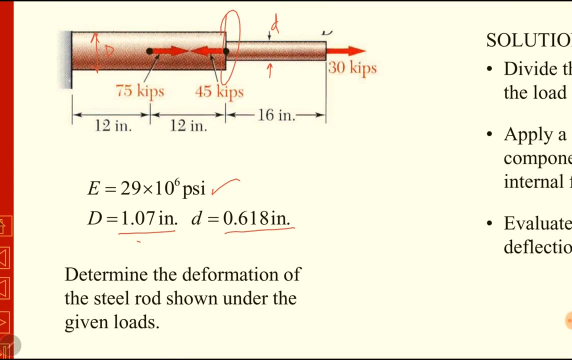 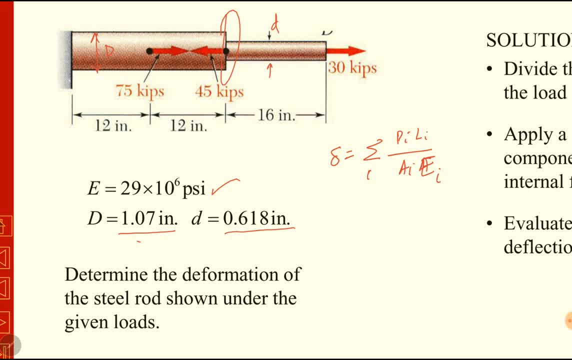 0 0 0 0 0 0 0. wherever the load changes or wherever the area changes or wherever the material changes along the length. Along the length, we will change this load wherever the area changes or wherever the material changes or wherever the material changes. 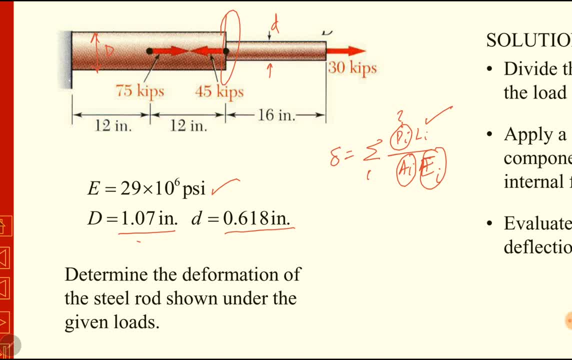 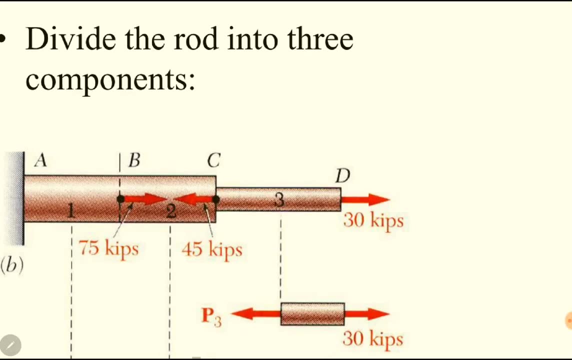 So in this case material is constant, It is same, But area is changing and similarly load is changing at three different points. so we usually start from the free end at the free end. Here I will see ABCD at point A. it is fixed at point B. 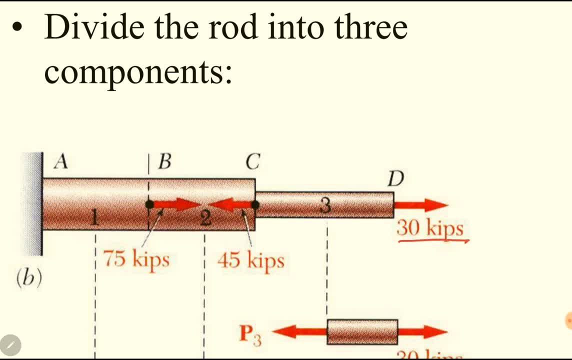 It is free. at free end there is a 30 kilo pounds force. at point C There is a point 45 kilo pounds force and at point B this 75 kilo pounds of force Area is also changing from. at point C We will start at D. at D We have 30 kilo pounds force. 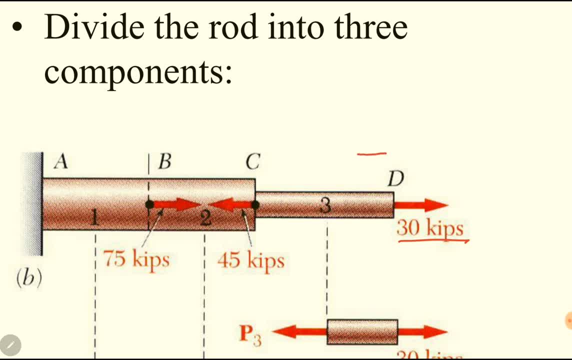 Going from the free end towards the fixed end Area changes at point C. So before that we will section this Bar. Then at C, area changes as well as the load changes. again, Going from C towards B Area is constant but load changes at B, So we will section the. 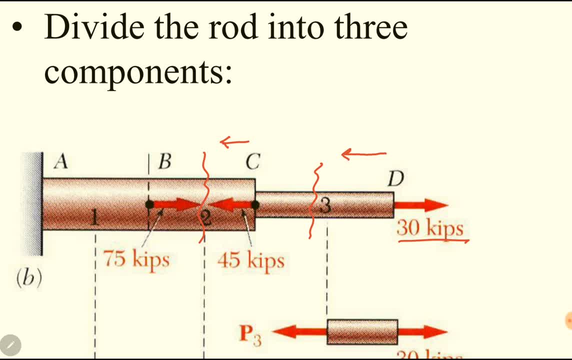 Bar between B and C. again, going from B till a, area is constant, But at point A it is fixed. so it fixed and we have reaction forces. It will be a reaction force here. again, We will section it between A and B. We will section the bar between 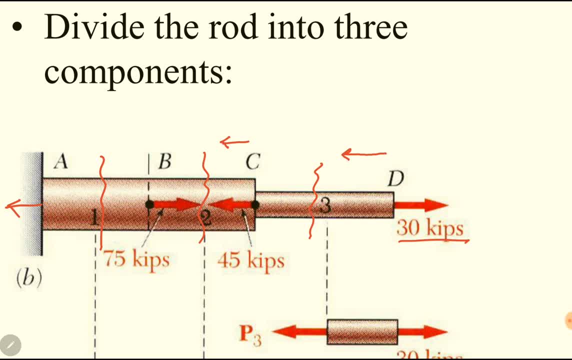 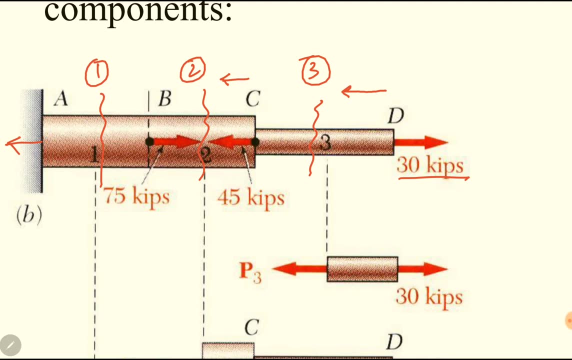 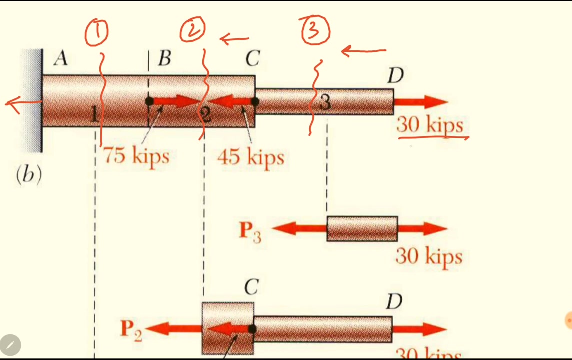 Two points: wherever the load changes are the area changes are the material changes. So we have total three sections: section one, two and three. we will draw individually individual free wide body diagrams At each section. if we section this beam, this bar at point at section three, So we will draw its free body time diagram here at point D. 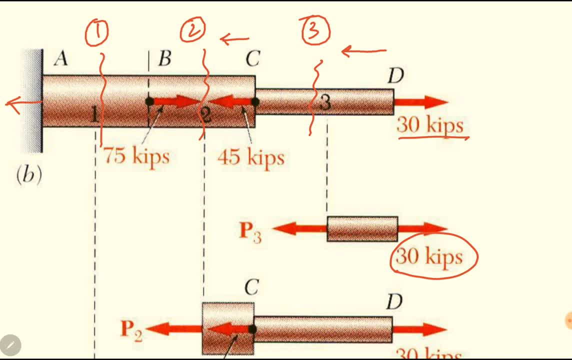 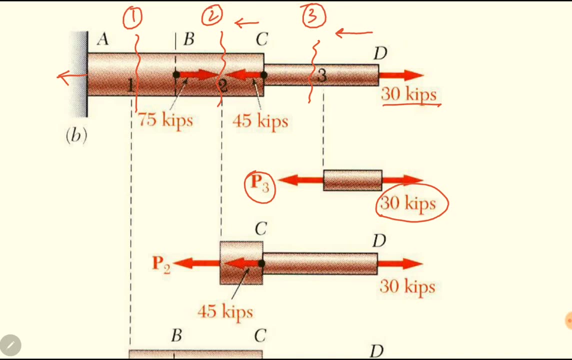 We have 30 kilo pounds of force and at sections Three, where we have sectioned it, there must be a reaction force and we are calling it P3. similarly, at section two, we have drawn a free body diagram. whatever is on the Right side of it, you can also draw it and draw the left side of it. 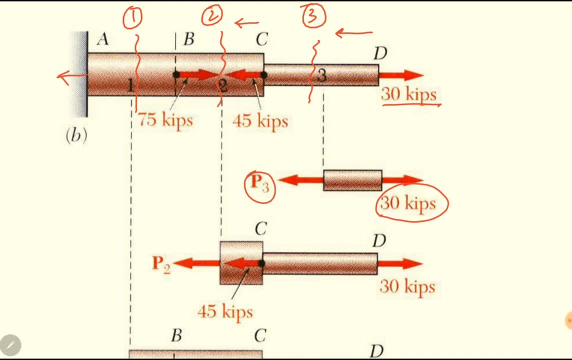 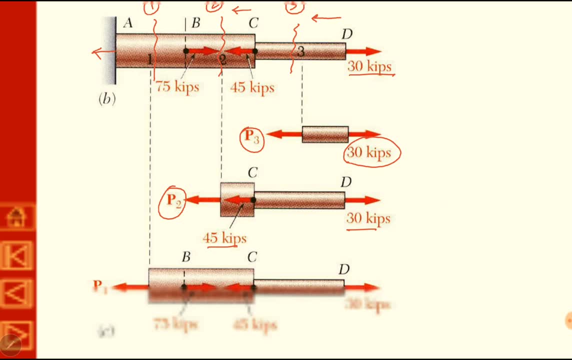 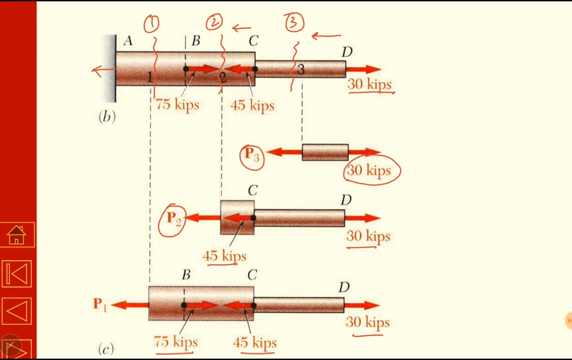 But whichever you follow. so at section two we have a reaction force. all of the other forces are given similarly. If we section it at point, at at one, so all the forces on the right side are Given forces, known forces, and at section one we have a reaction force which is unknown. 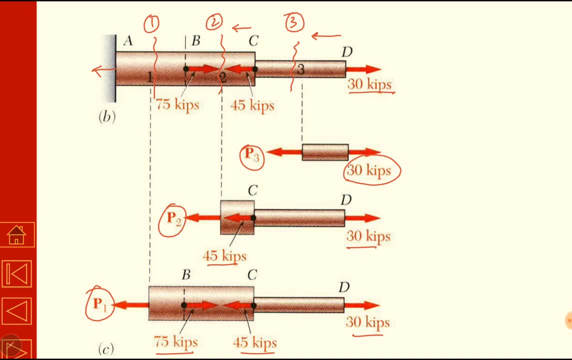 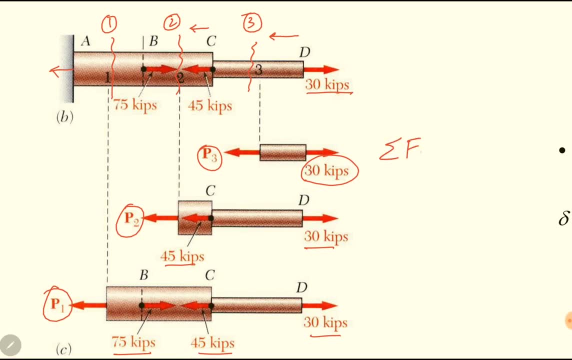 So we have three reaction forces- P1, P2 and P3- in three different sections- section one, two and three- we can find these forces. Summation of forces is equal to zero. So for this section three, P3 minus 30 is equal to zero, so P3 is equal to. 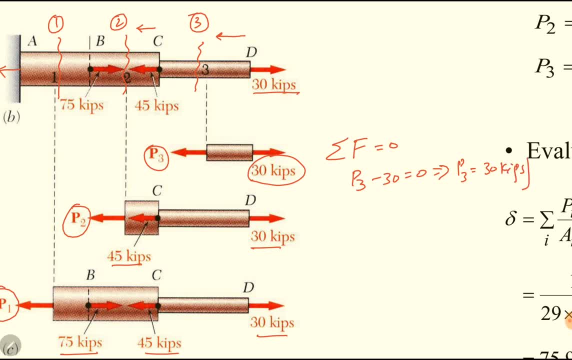 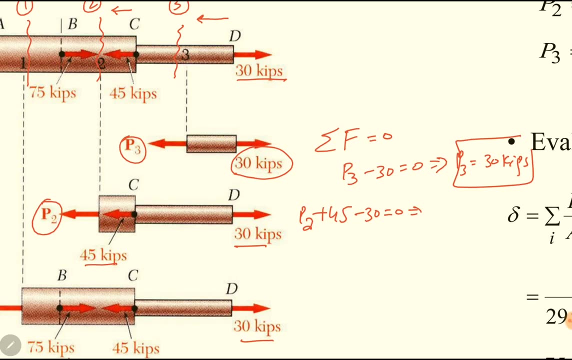 30 kilo pounds. Similarly, for section two, P2 plus 45 Minus 30 is equal to zero. the forces in same direction will have same sign. In the opposite direction they will have different size. so P2 Will be equal to minus 15 kilo pounds. similarly we can find P3. 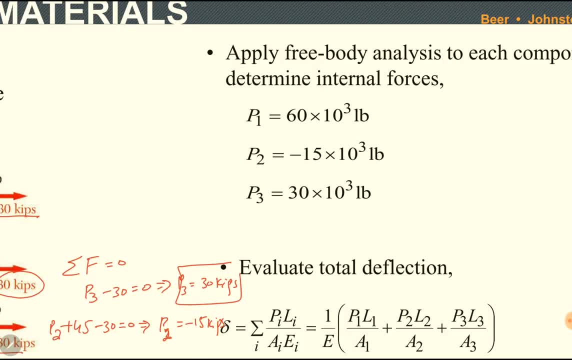 So P2, P3 and P4 have been calculated. P1 is 60 kilo pounds, or 16 to 10 power 3 pounds. p2 is minus 15 kilo pounds and p3 is 30 kilo pounds. okay, now we know p1, p2. 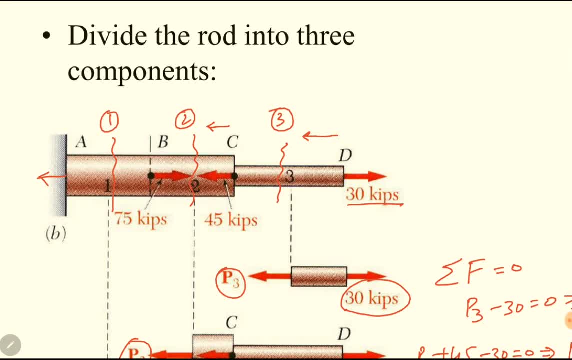 and p3, a1, a2 and a3. section 1 has a diameter, capital d- given to us. section 2 also has the same diameter, so a1 and a2 will be same. section 3 has a smaller diameter, small d it is also given to us. so from diameter we can find areas a1 and a2. both are same pi by 4. 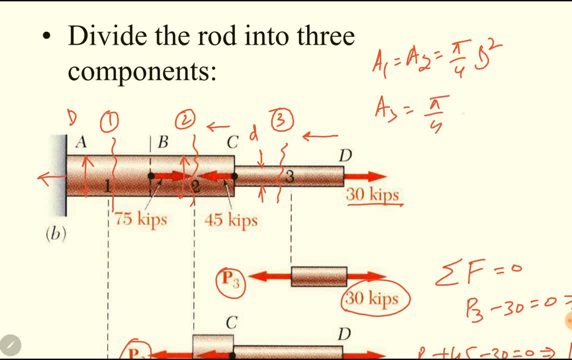 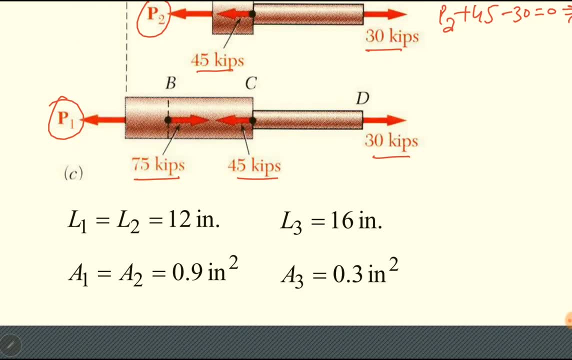 capital d square and a3 is pi by 4 small d square. capital d and small d are given to us, so we can calculate a1 and a2 and a3. a1 is a1 and a2. both are 0.9 square inch and a3 is 0.3 square inch. 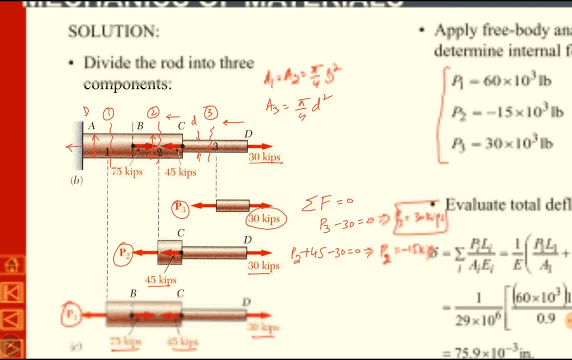 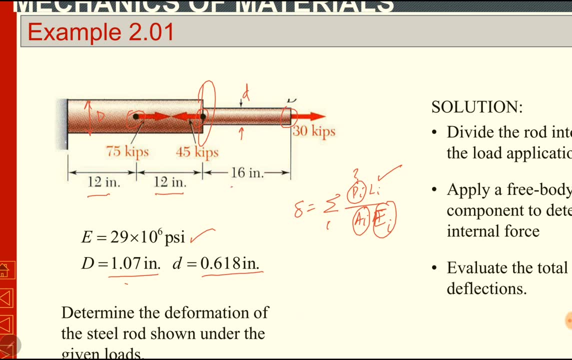 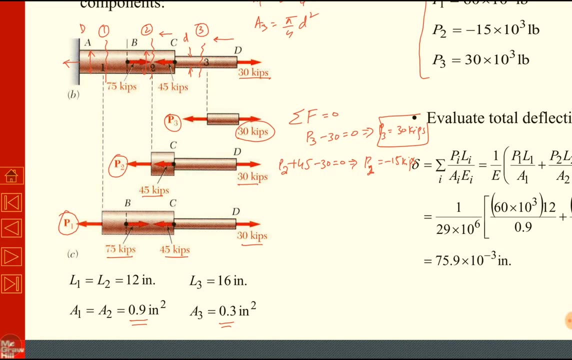 l1, l2 and L3 are given to us already in the given statement. L1 is 12 inches, L2 is 12 inches and L3 is 16 inches length. L is the length between the two points where we have those two points between which we have sectioned the bar. so L1 and L2, both are given to us as 12 inches. 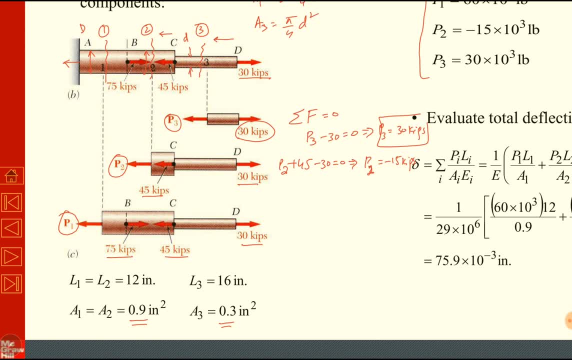 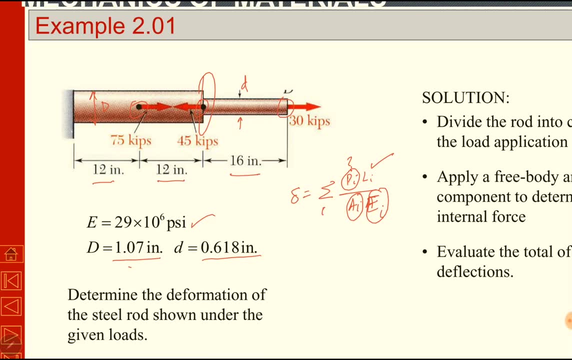 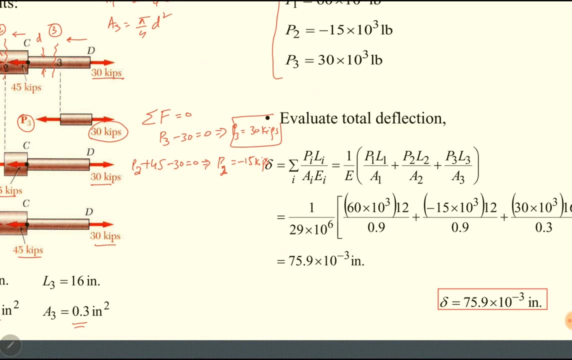 and L3 is given to us as 16 inches. E is same for all of the sections. material is same: E1, E2 and E3. all of them are simply 29 into 10 power, 6 psi. it is given to us in the problem. 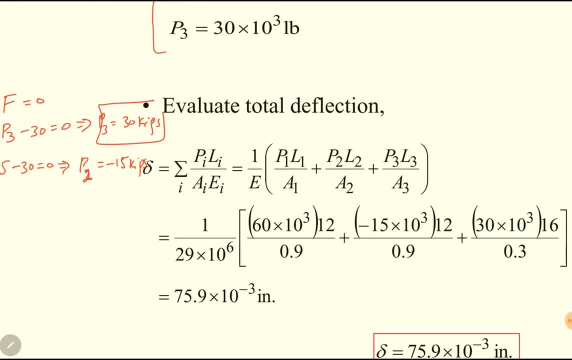 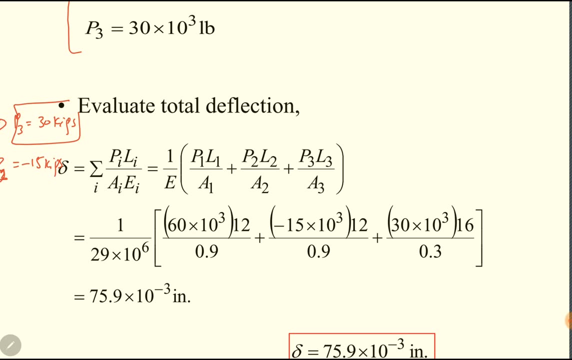 so net deformation is P1, L1 over A1, E1, P2, L2 over A2, E2 plus P3, L3 over A3, E3, E is common because E is constant, So we can put the values here and after calculations delta, our deformation is 75.9 into 10 power. 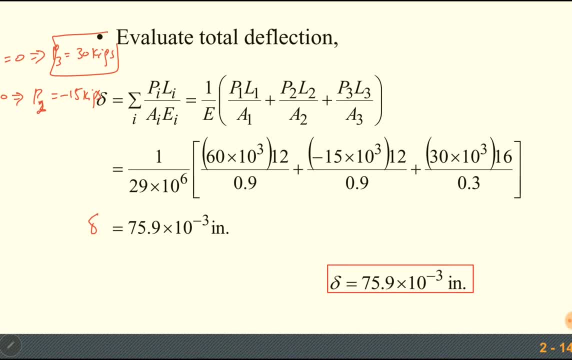 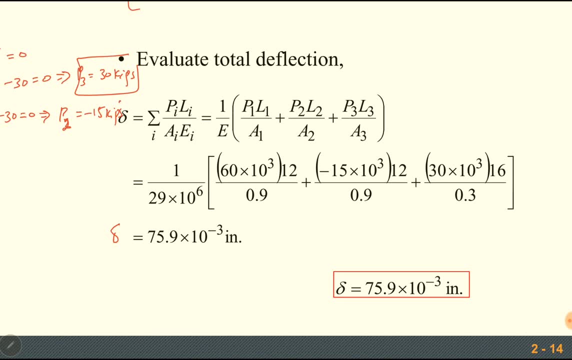 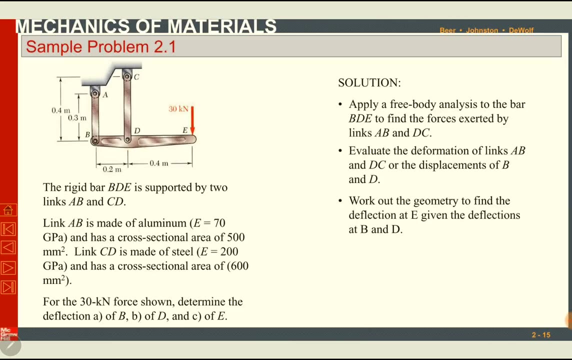 minus 3 inches. this was required in the problem and we have calculated. this is very simple. you have to use this expression: del is equal to summation of PILIAI EI. moving next, we have another sample problem, Problem 2.1 from the textbook. the rigid bar BDE is supported by two links, AB and CD. so 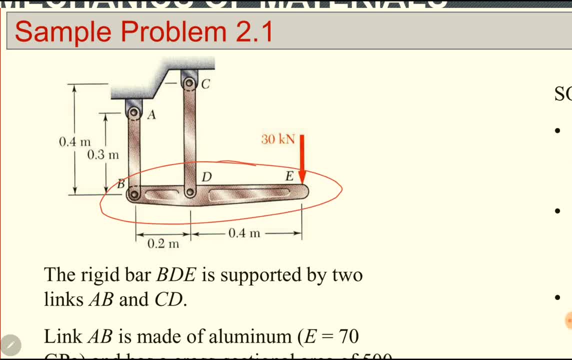 here is a rigid bar. it cannot be deformed, it is rigid and it is supported with two links: AB and CD. now, the AB and CD are not specified as rigid, so it means they are deformable. they are not rigid. we can find deformation in AB and CD. what is required? 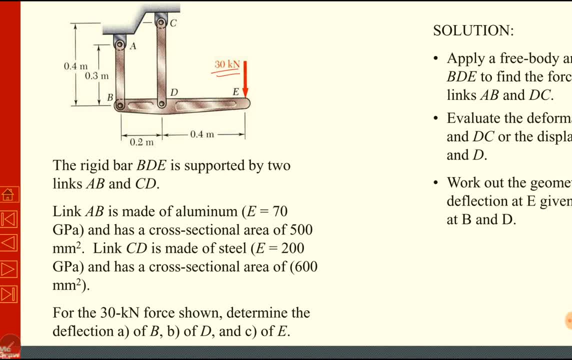 Okay, So we have a load of 30 kilonewton at point E link. AB is made of aluminum and E modulus of elasticity is 70 gigapascal. so if there is a value of E for a material, it means it is deformable material. it is not rigid, AB is not rigid and AB has a cross sectional. 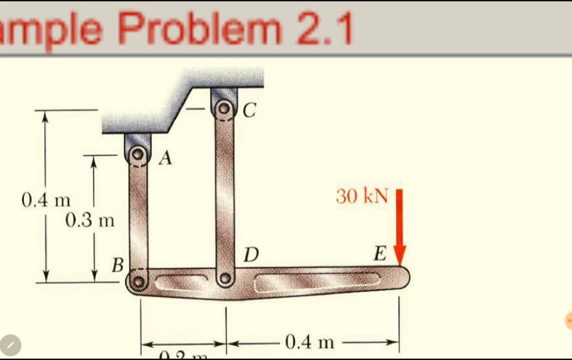 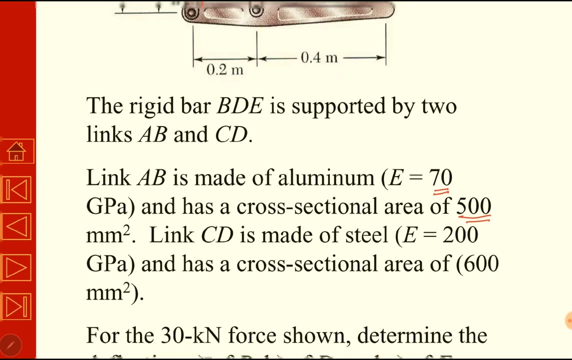 area of 500 meters square. so in the third dimension, which is not visible to us in this diagram, this bar is an area. Okay, Okay, Okay, Okay, Okay. So we have a cross sectional area of 600 millimeter square. link CD is also made of. it is made. 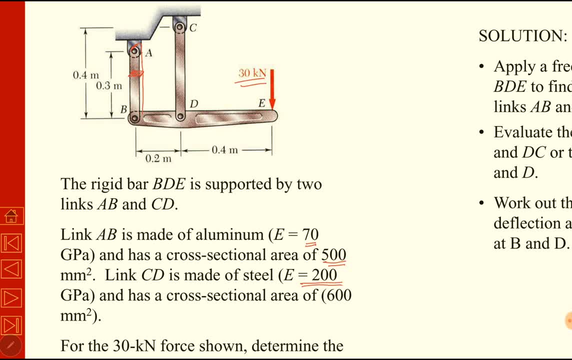 of steel and modulus of elasticity of steel is given to us, 200 gigapascal and it has a cross sectional area of 600 millimeter square. so area for both the bars is given. modulus of elasticity E for both the bars is given and length of both the bars is known. AB is 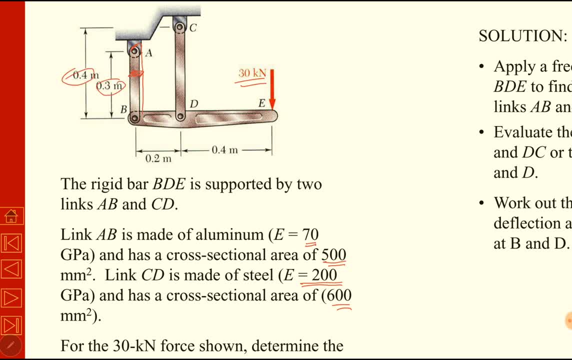 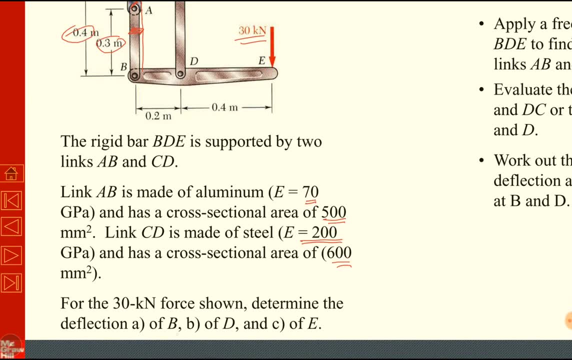 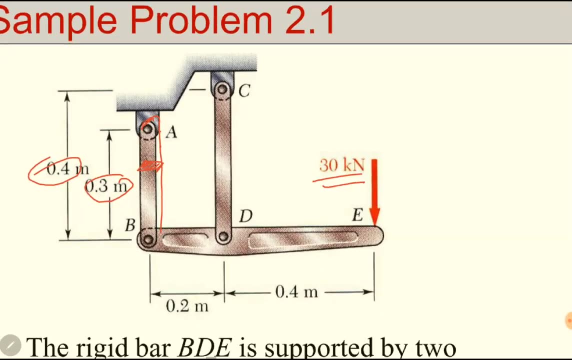 0.3 meter And CD is 0.4 meters. What is required under this load of 30 kilonewton force? determine the deflection in B, D and E. deflection means how much they have moved. it is fixed. both the bars are fixed at the. 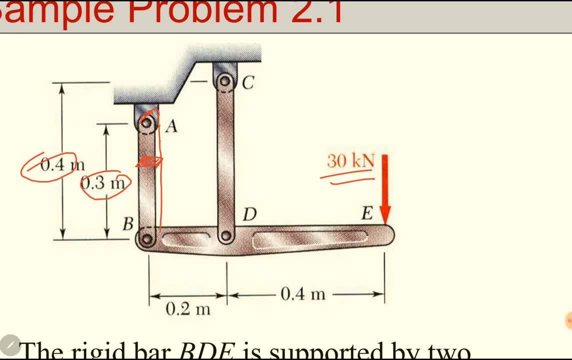 top ends and the bar AB is fixed at A and bar CD is fixed at C, so at the fixed end they cannot move, But at the other end, At And B and D, they can either come down or they can move up, either coming down or moving up. 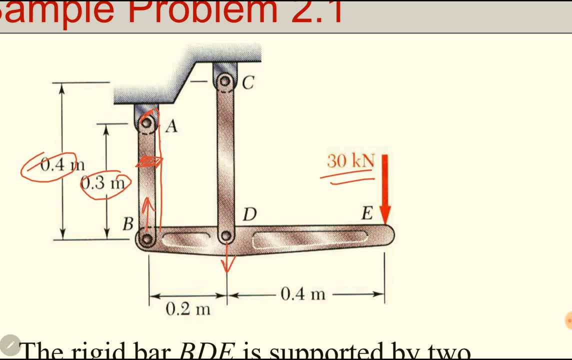 whatever it is. So we will first find either they are in tension or compression. either both of them are can be in tension, or both of them can be in compression, or one of them can be in tension or other one in compression. So the amount this point B moves towards A or moves away from A. 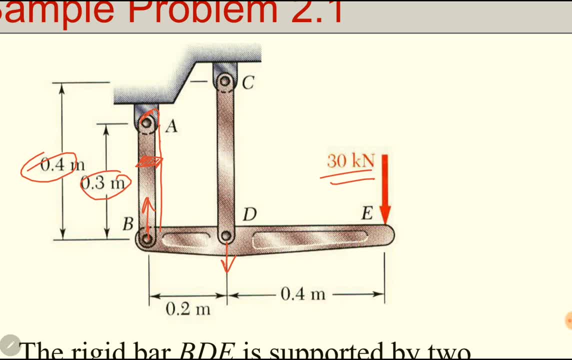 Okay, It is the deformation in this bar AB. similarly, the amount the point B moves towards C or away from C, it will be deformation in the rod in the bar CD. So simply, we have to find deformation in bar AB and deformation in bar CD. it will be the 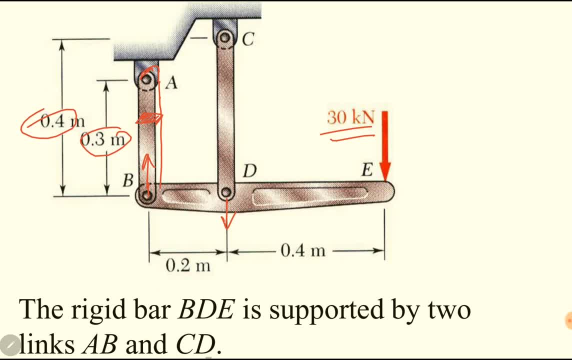 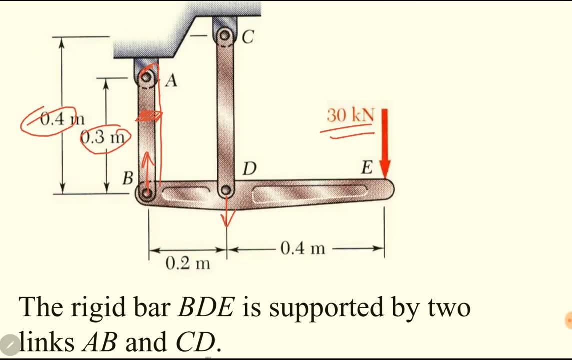 displacement of point B and points D respectively. And again we have to find deformation, deflection, in point E as well. so how much this point E moves, We will find it later. We will find it later on using trigonometry. so first we will find del AB, which will be: 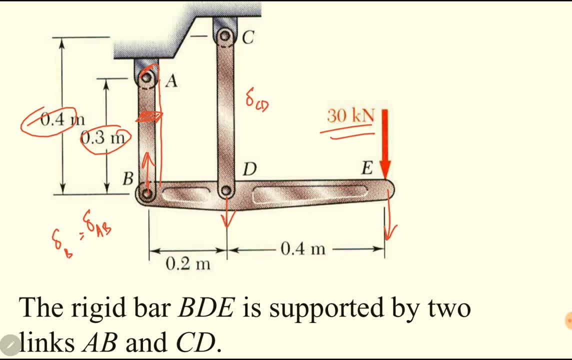 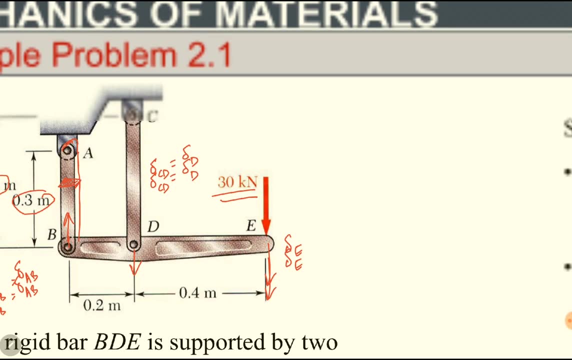 deflection in point B Del CD. deformation in rod CD will be equal to deflection of point D. and from these two values how we find deflection of point E? we will use trigonometry. So let us see how we can do, because there is no deformable bar attached to point E. so 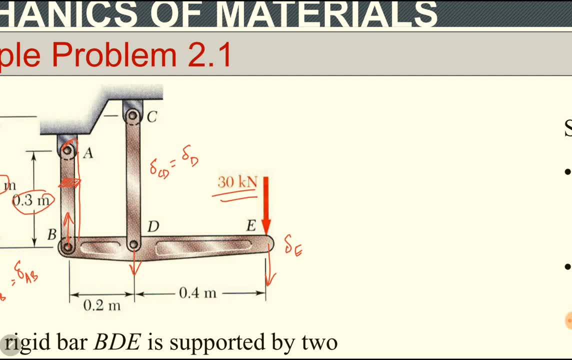 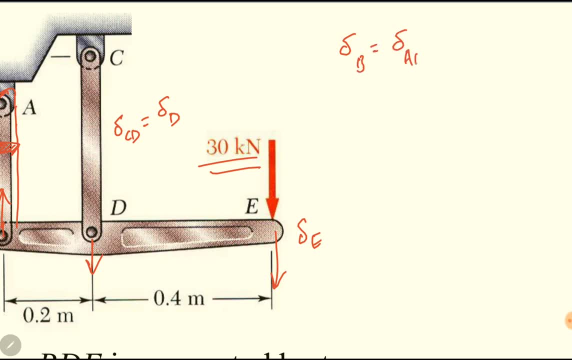 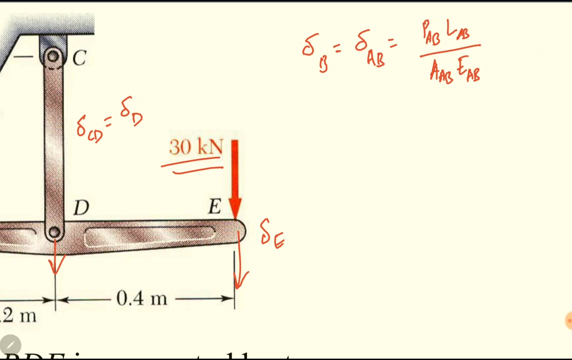 we cannot, We will use this deformation formula. okay, deformation in point A in rod AB del B will be equal to force in AB, length of AB divided by area of AB and E of AB. Length of AB is known to us, which is 0.3 meter. area of AB is given to us in the problem statement. 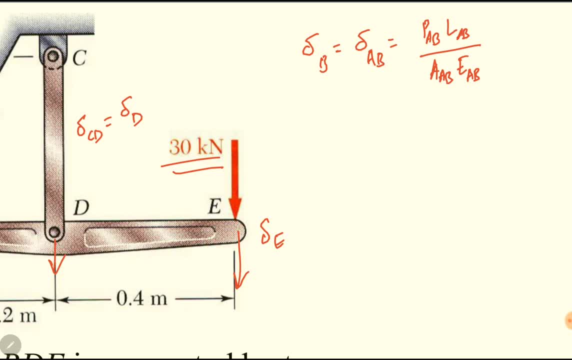 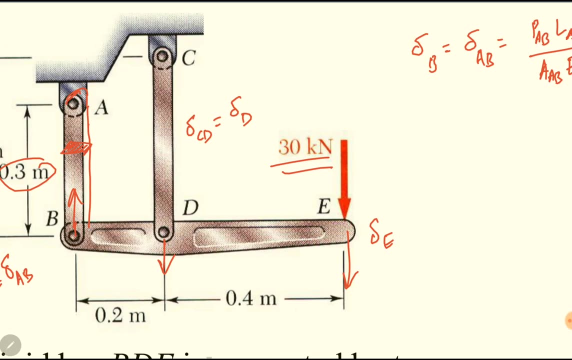 E Modulus of elasticity of AB, Aluminum, is given to us. Okay, So we have to find force in AB, PAB. similarly for CD. we know all of the other parameters. we know we need to know PCD. so the load in AB and CD can be found using equations of: 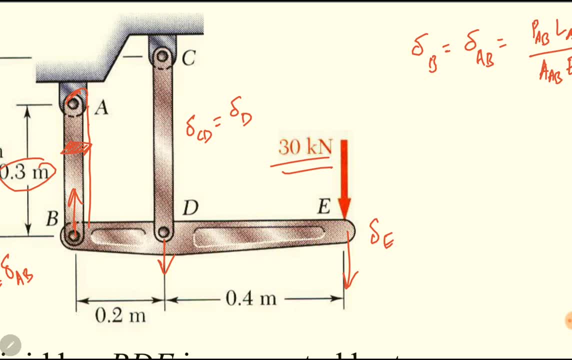 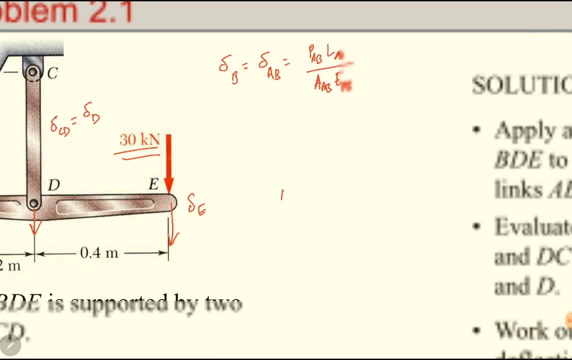 statics, laws of statics. first we will draw a free body diagram of this rigid bar BDE. the free body diagram of rigid bar BDE can be drawn like: at point E We have a downward force of 30 kilo Newton. at point D and B we are assuming that there. 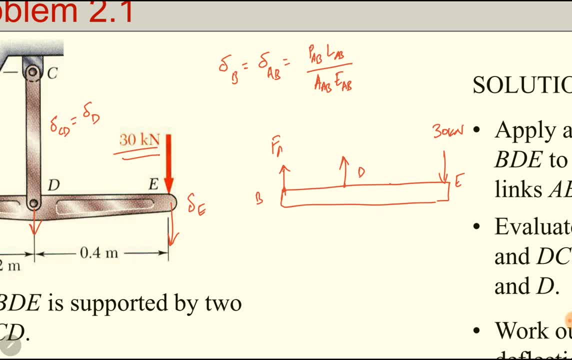 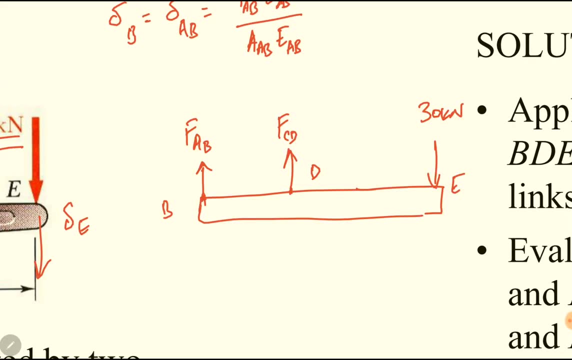 are two reaction forces: FAB or PAB, and FCD or PCD. whatever you represent it, however, you represent it. Okay, Okay, Okay, Okay, Okay, Okay. So we have two arrows upward. they are away from the bar BDE, so away from the bar BDE. 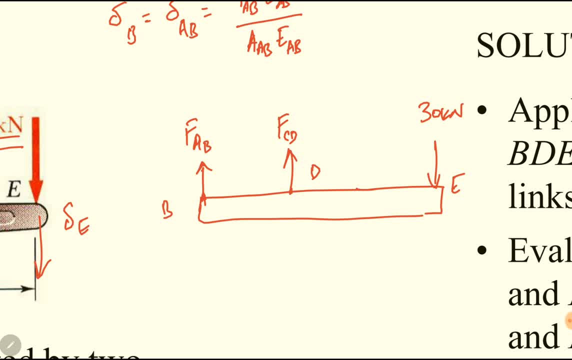 means I am assuming that both of these forces are tensile. this is my assumption. if my assumption is wrong, so after calculation the numerical values will be in the negative, with negative sign. if the sign of the force is positive, it means our assumptions were correct. So initially I have assumed that both these forces are tensile. 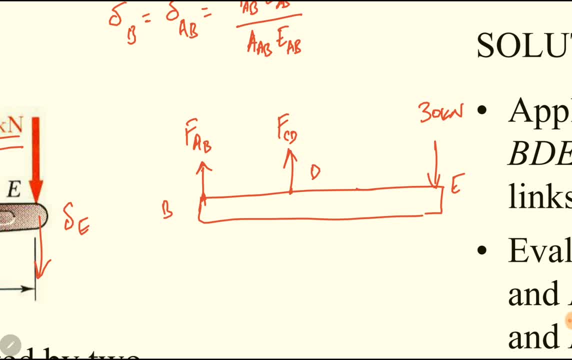 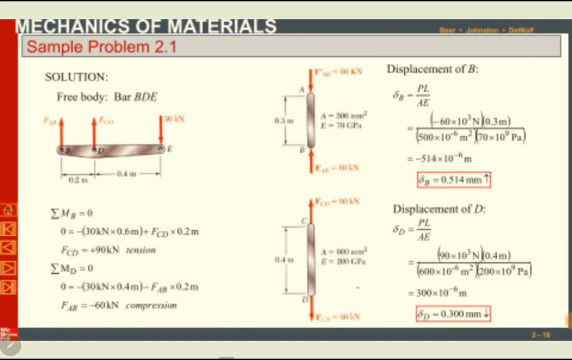 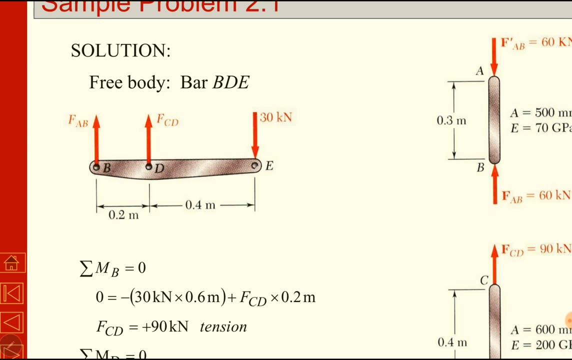 They are away from the body. here we can use equations of statics because we know these lengths. here it is okay. there are two unknowns, FAB and FCD. so two unknowns can be calculated using equations of equilibrium. Okay, Okay, Okay. 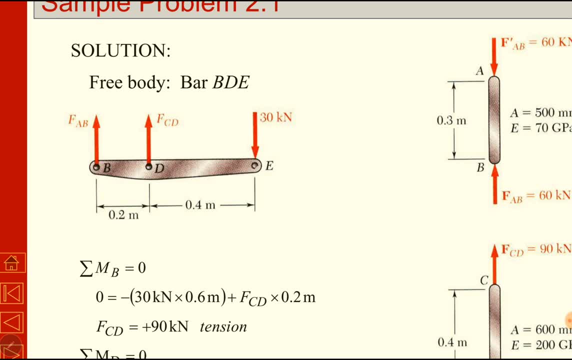 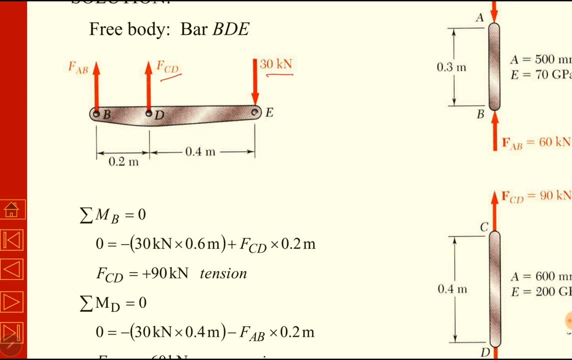 Okay, Okay, from point B, which is 0.2 plus 0.4, it is 0.6, so Fcd becomes 90 kilonewton with a positive value. so positive value means the direction I have assumed here. it is correct. it is under tension. 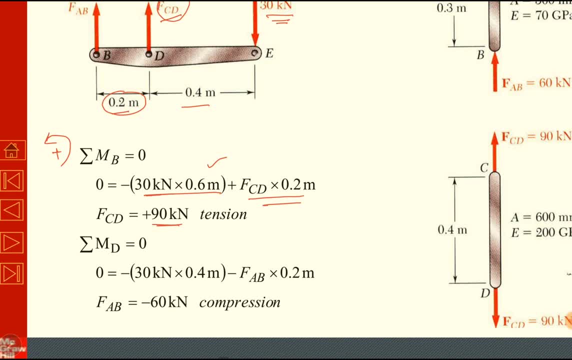 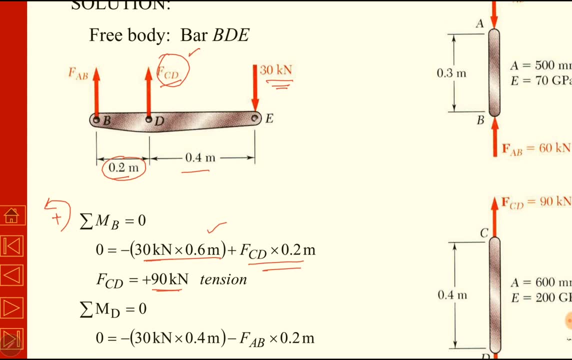 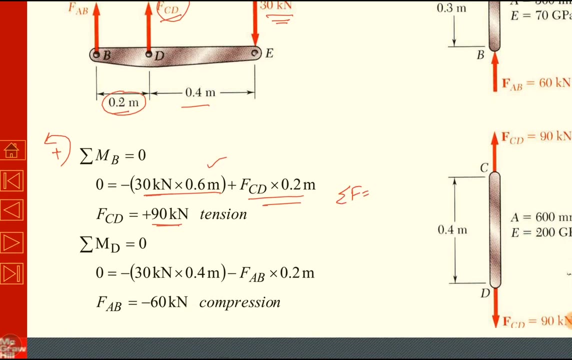 the bar cd is under tension, okay. similarly, it is under tension because I have assumed it under tension and the value is positive value of the force. so it means my assumption is correct. summation of forces is equal to zero. I can write it as: Fcd plus FAB minus 30 is equal to zero, or? 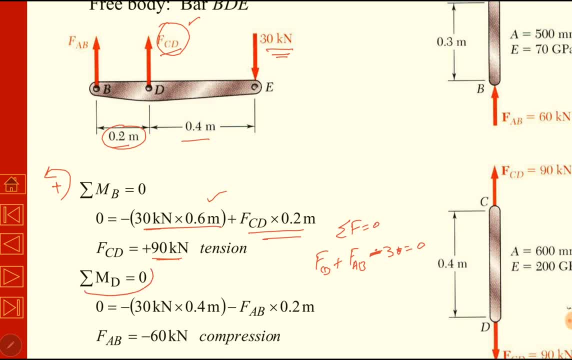 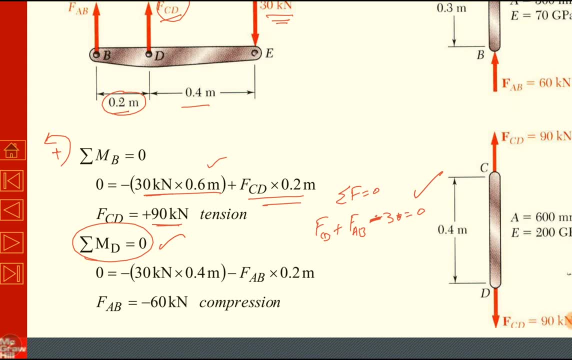 I can use. alternatively, I can use summation of moments at point D. you can either use this expression or this expression. take some of all the moments at point D and you can calculate FAB, and it comes out to be minus 60 kilonewton. 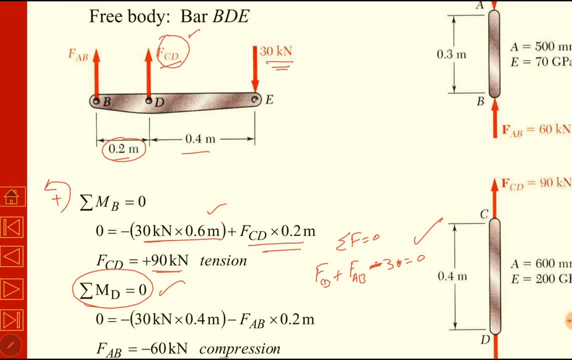 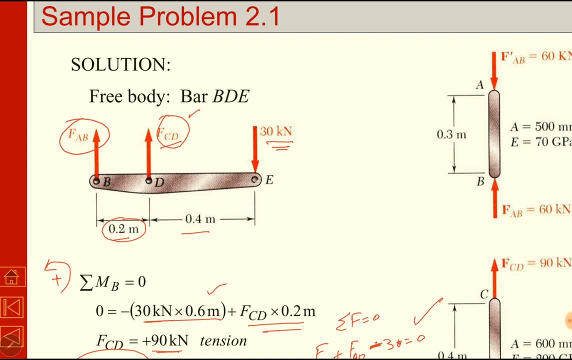 if you want to use this expression, you can use this expression. you can use this expression if it is minus 60 kilonewton. the negative sign means this direction, which I have assumed. it is incorrect. we have to change the direction. I have assumed FAB as a tensile force away from 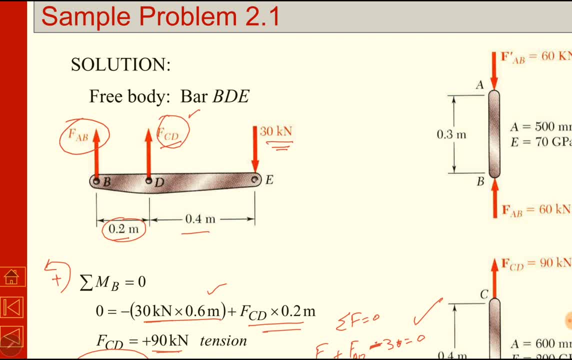 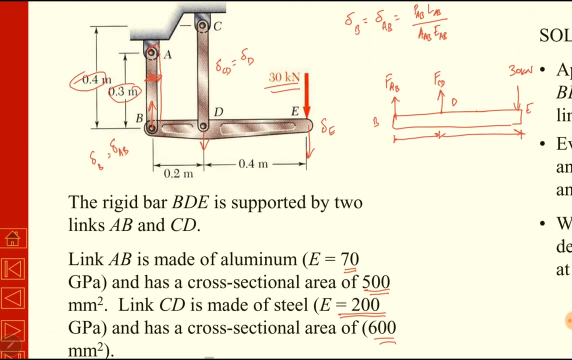 this rod, so it means it is wrong. it should be a compressive one. okay, some students usually get confused that this force AB is towards the, now the new direction which is defined here. it is compressive, so it is towards the, this bar, this rigid bar. so it means some of the students think it means it is towards the bars. 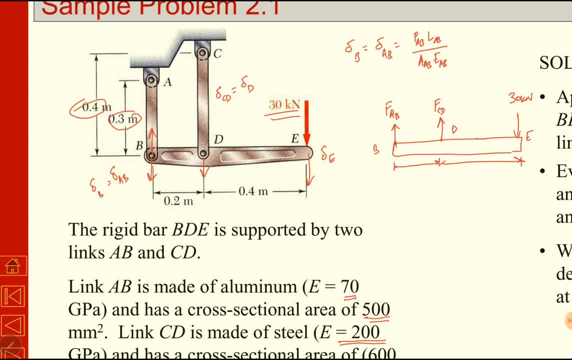 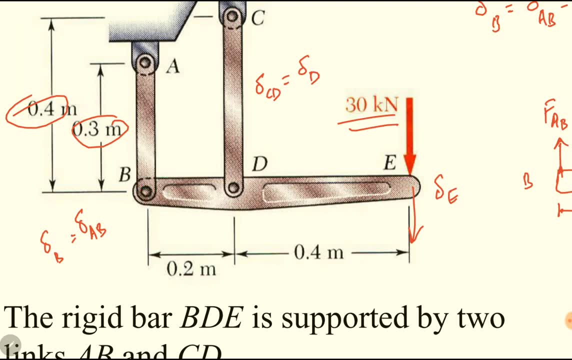 so the force is downward. it is not correct. compression means if the bar, if the bar AB is under compression, so it is applying a compressive force on this rigid bar. in response, the rigid bar will apply a compressive force on the rod AB or the bar AB. similarly, if a 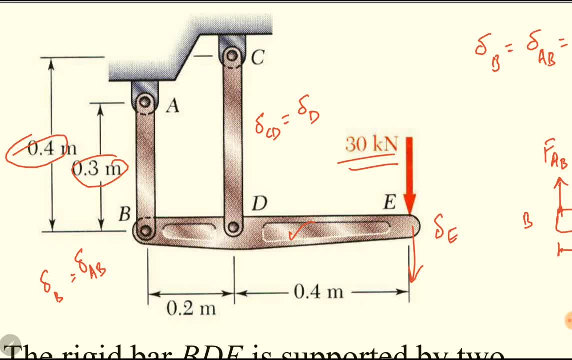 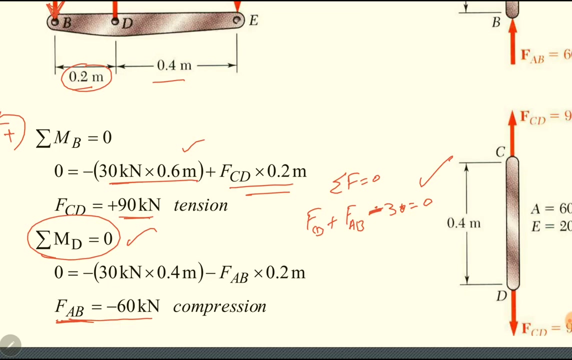 The rod CD or the bar CD is under tension, it is applying a tensile force on the rigid bar BDE and the rigid bar BDE is applying a reaction force as a tensile force on rod CD. So FCD is in 90 kilo Newton tension. if AB is in compression it is minus 60 kilo Newton. 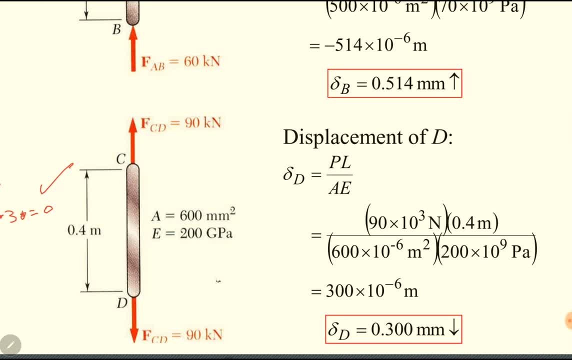 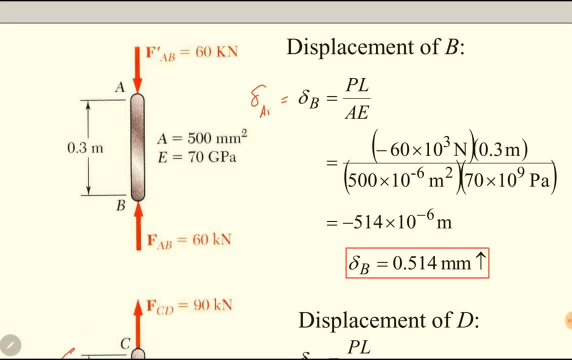 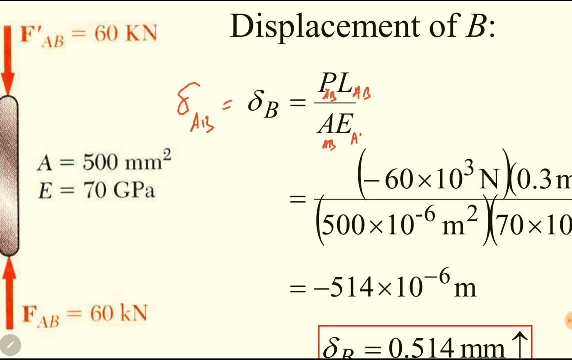 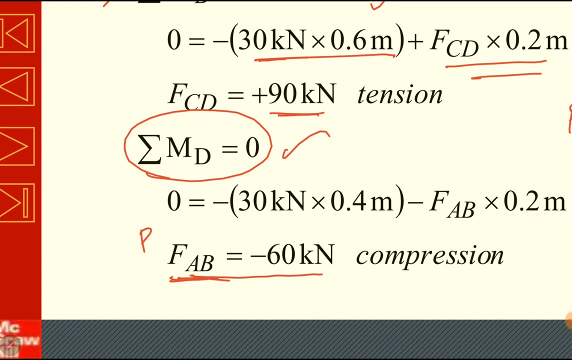 Now we know both the forces. already We have this expression: del B or del AB is equal to PAB or FAB. length of AB, area of AB, E of AB. this PAB is force in AB which we have calculated here is FAB. We should have used here PAB actually. okay. 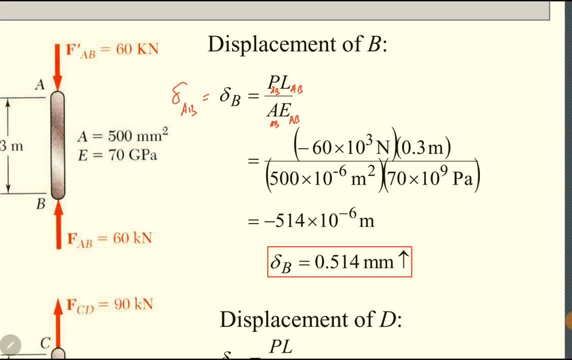 So by putting all the values- length, area and E were already Known to us- P has been calculated as minus 60 kilo Newton, minus 16 to 10 power 3 Newton. So the value value comes out to be minus 5, 1, 4 into 10 power minus 6 meters. 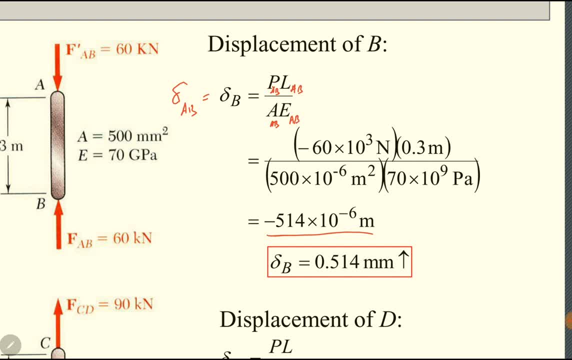 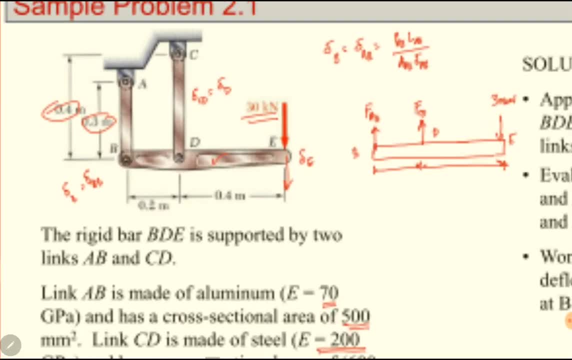 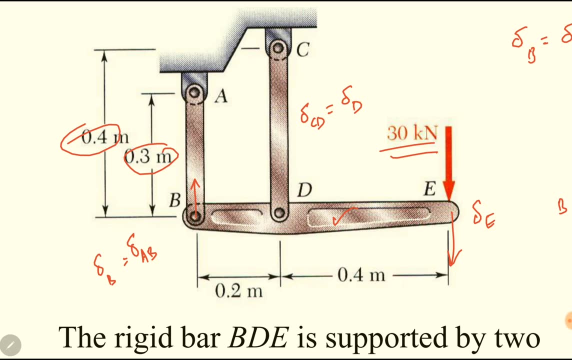 minus 5, 1, 4 into 10. power minus 6 means This rod if the bar AB is under compression. If the bar AB is under compression, it means this point B will move towards a compression means the length decreases, So it will move towards a fixed point. 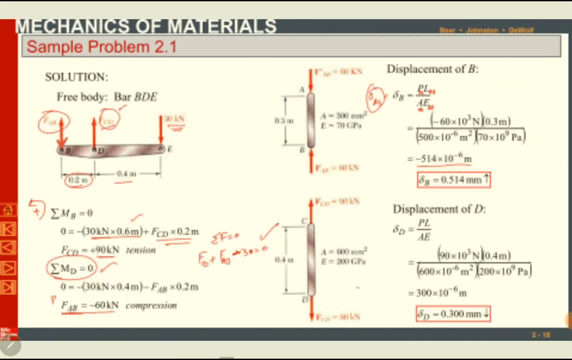 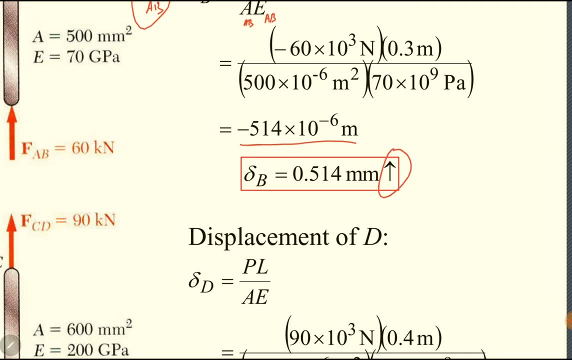 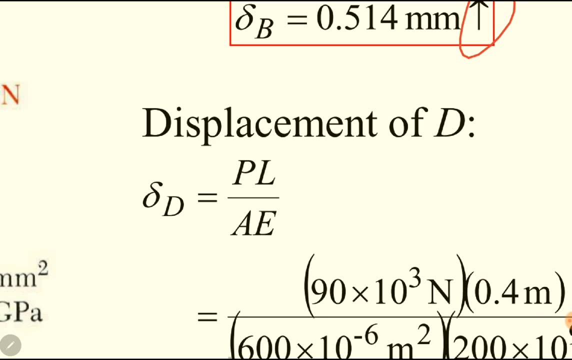 So it is moving upward. actually, Point B, We're here. we have mentioned here 0.5 and 4 millimeter deformation upward. the put sign, similarly del D, is actually deformation in rod. in bar CD It will be CD or F CD, length of CD, area of CD and E of CD. by putting all the values 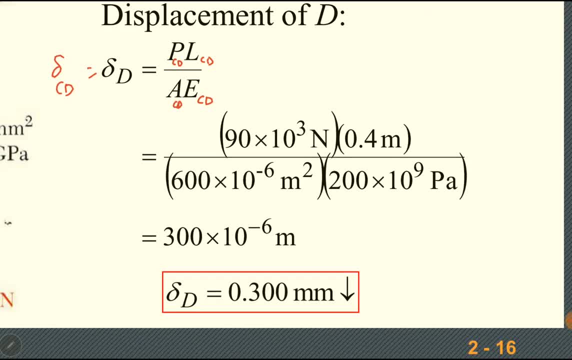 Length area and E were already known to us. P has been calculated recently as 19 to 10 power 3 Newton. By putting all the values del D becomes 13 to 10 power minus 6 meters. It is positive. It means There are. the bar. CD is under tension. 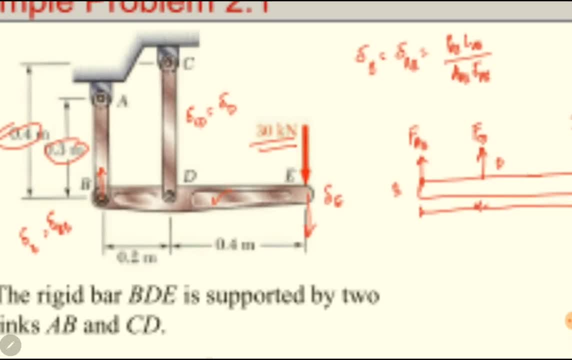 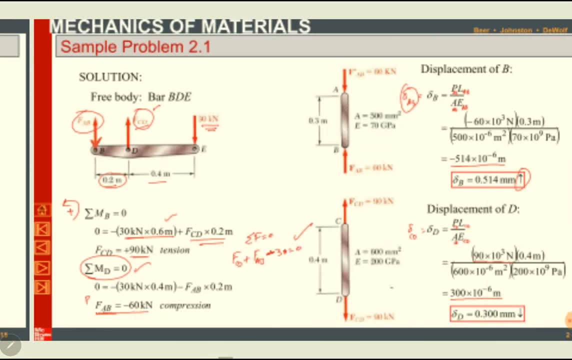 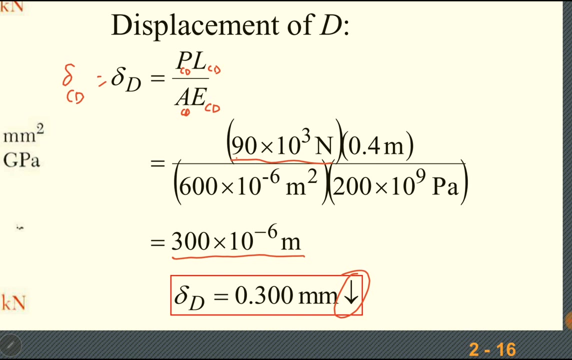 If the bar CD is under tension, It means this point D will move away from point C, the fixed end, So it will come downwards. So here we have shown a downward sign. So now we know that how much the point B has moved upward and how much. 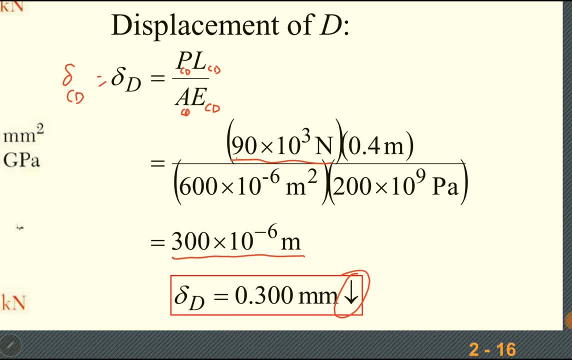 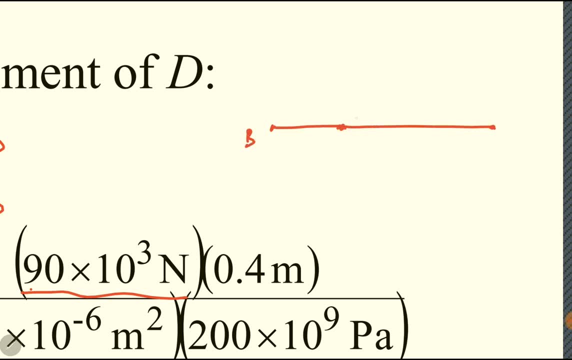 The point: D has moved downward. Okay, initially B, D and E Is like this: it is horizontal. B has moved upward, D has moved downward. It is rigid. So this is Delta B, This is: B has moved to B dash, D has moved to D dash. here Delta D and E will come down, E dash. 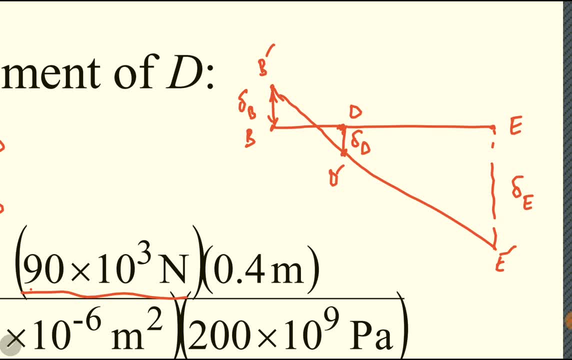 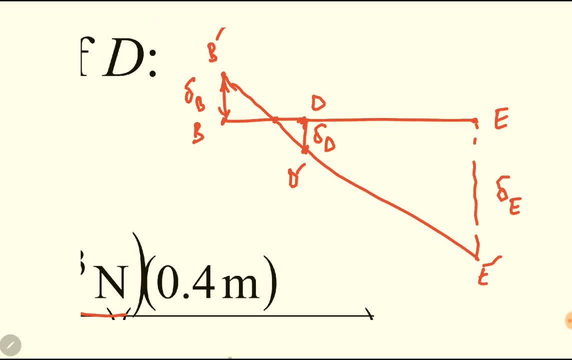 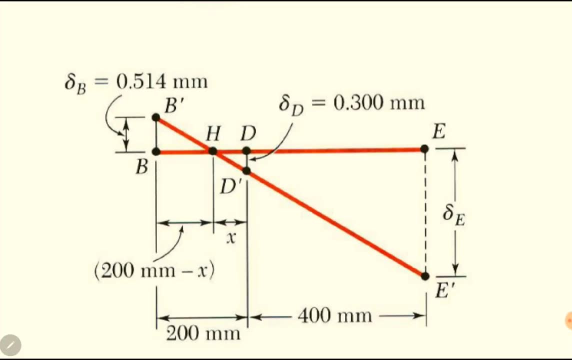 This Delta E you have to calculate. in the third part of the problem We can use trigonometry because we have three similar triangles here. if I call it Is point H, here it is drawn, here This intersection point is point H. We have three triangles, triangle. 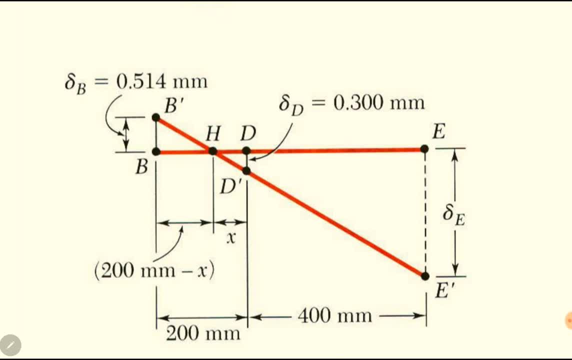 H BB dash, triangle HDD dash and triangle HBB dash. These three triangles are similar triangles because their corresponding angles are equal. So we know from trigonometry that if this, if two triangles are similar, the ratio of their corresponding sides will be same. We do not know this, the location of point H, So let us call it. 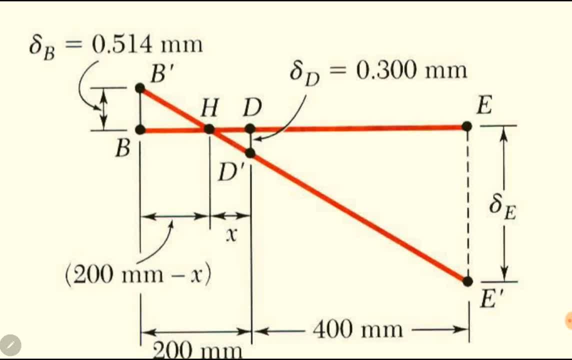 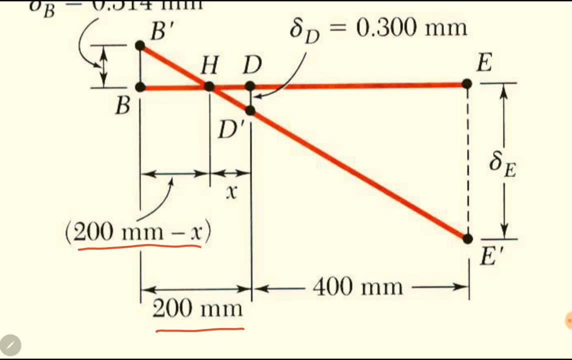 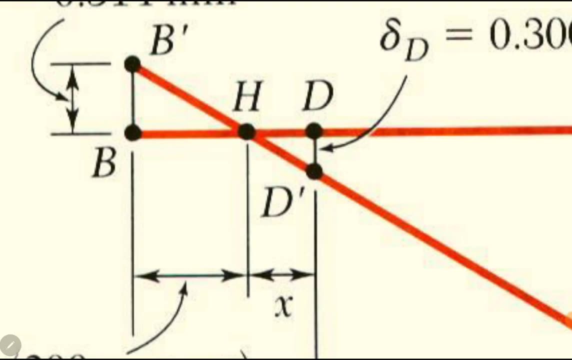 X. HD length is X, so BD is given to us already in the problem. It is 200 mm, So this remaining length will be 200 minus X. So let us find X first. So from these two triangles, HBB dash and HDD dash, They are similar triangles. 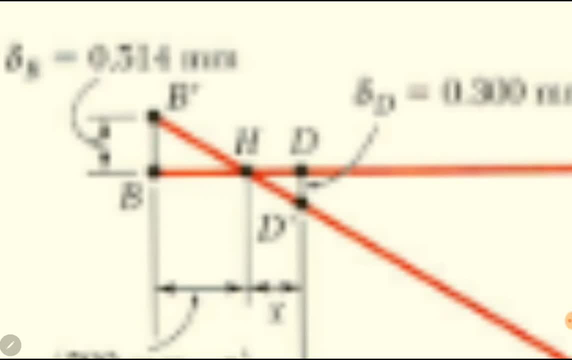 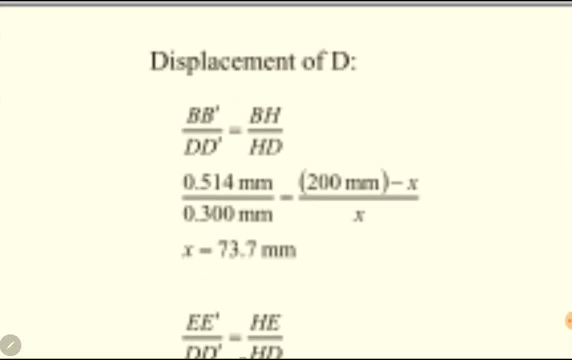 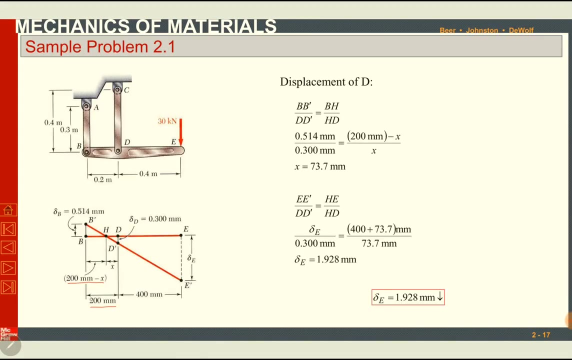 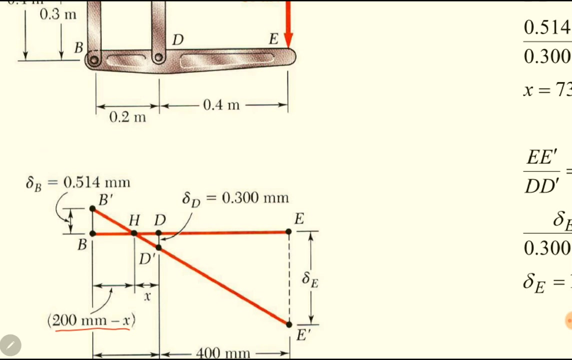 So we can find this length H if we get. if we use the ratio of their corresponding sides, Ratio of the corresponding sides will be equal. BB dash divided by DD dash will be equal to BH divided by DH or HD. So the given values are: BB dash is equal to Delta B and DD dash is equal to Delta D. 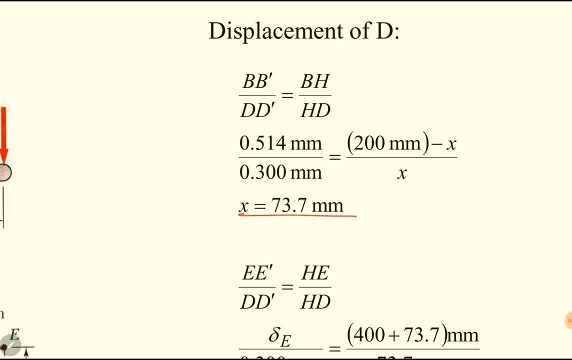 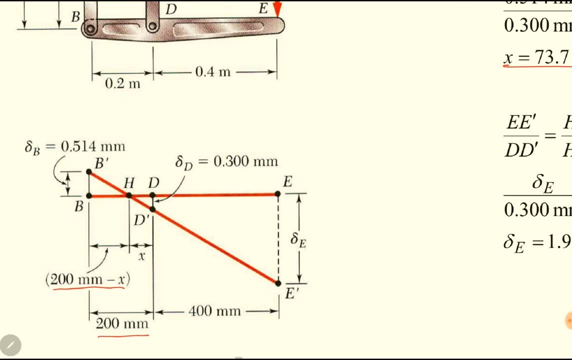 We can simply put the values here and we can find X- Now the X is known to us. So we can compare the two triangles, HDD dash- Now the length X is known to us- HDD dash and HEE dash, from these two triangles, using the ratios of the 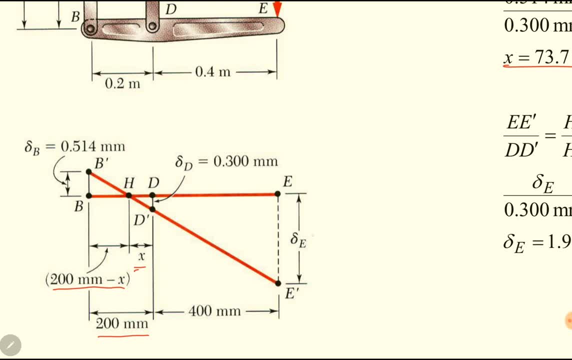 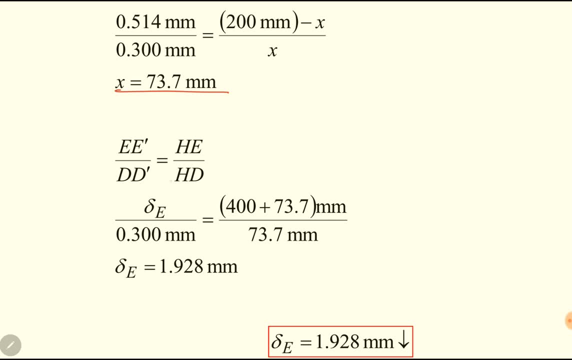 corresponding sides. We can use this side as well. We can find Delta E. This is unknown to us. So EE dash divided by DD dash is equal to HE divided by HD. You know the trigonometry very well from the From your previous mathematics courses. 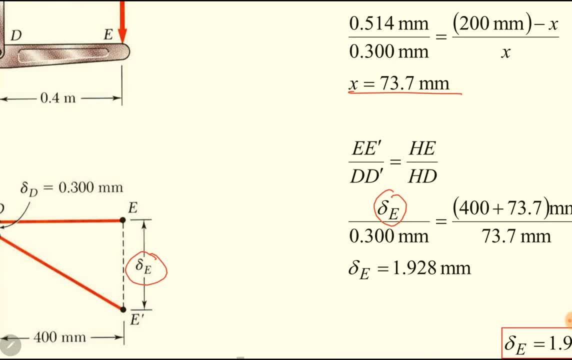 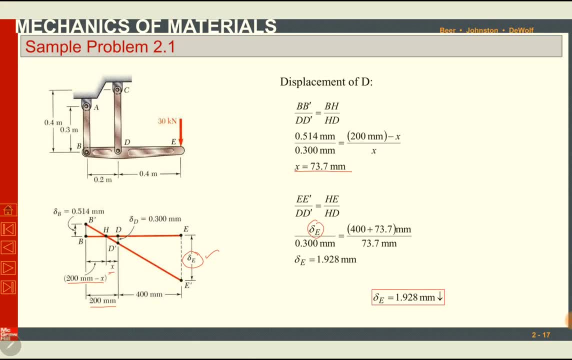 So you can find. EE dash is actually equal to Delta E, this one. All of the other values are known to us, So Delta E can be calculated as 1.928 millimeters and E has moved downward, So we have shown a downward sign here. Okay, so we were required to find. 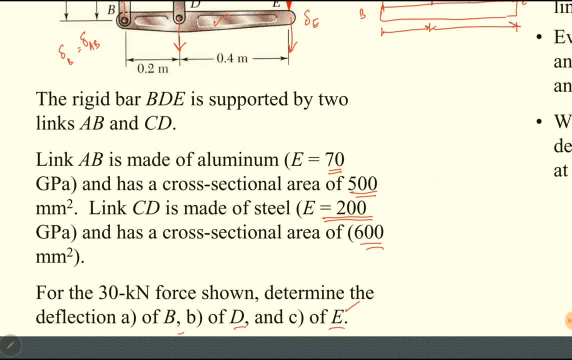 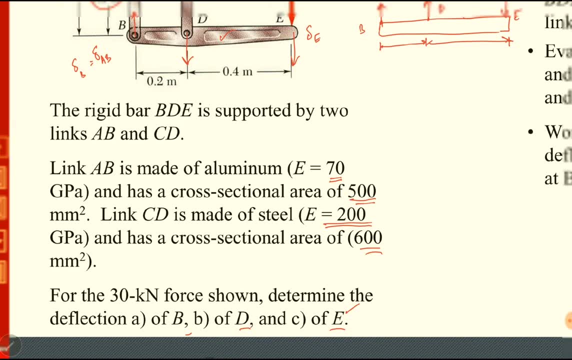 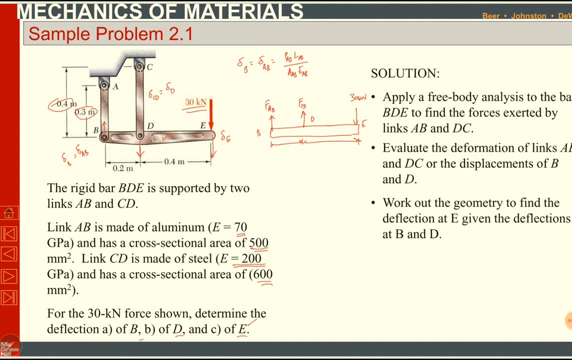 deflections of point B, D and E. Deflection of B is actually due to deformation in rod bar AB, deflection of D is due to deformation in rod CD and deflection of E is actually the due to the rotation of the rigid bar BDE And we have calculated it through trigonometry. I hope the concept is clear to you. I 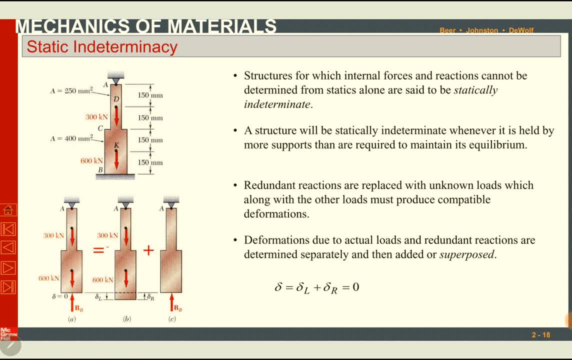 Will move forward. the next topic is static indeterminacy. What is indeterminacy? something that cannot be solved and cannot be determined. So static indeterminacy means something that cannot be solved using equations of statics. equations of statics are equations of equilibrium in two dimensions. we have 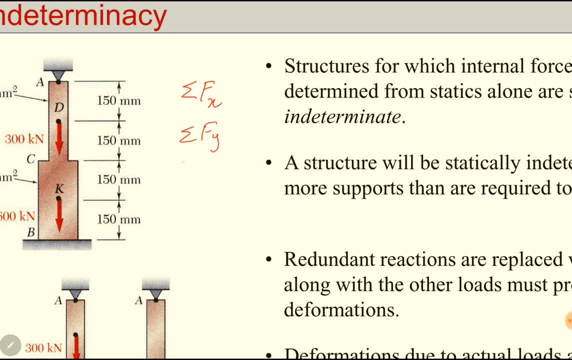 three equations of equilibria: Summation of forces in horizontal direction is equal to zero, summation of forces in vertical direction is equal to 0 And summation of moment in the plane, in the true dimensional plane, is 0. Okay, so, using these three equations, we can only find three unknowns. 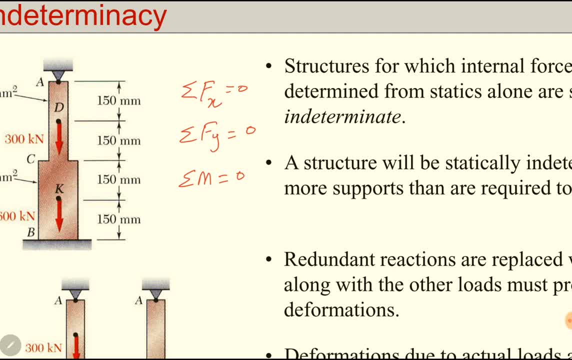 We cannot find four unknowns using three equations. So if the number of unknown reaction forces in a problem is more than number of equations, we cannot solve it using equations of equilibrium or equations of statics. so such kind of problem is called statically indeterminate problem. for 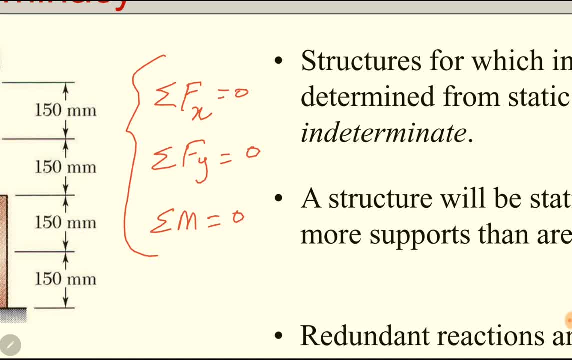 these two. remember that for these equations, from these three equations, we can find three unknowns, but one of them should be in the horizontal direction and the other two can be in any other two directions. one force can be in horizontal, two can be in the vertical, or one can be in the vertical, two can be in. 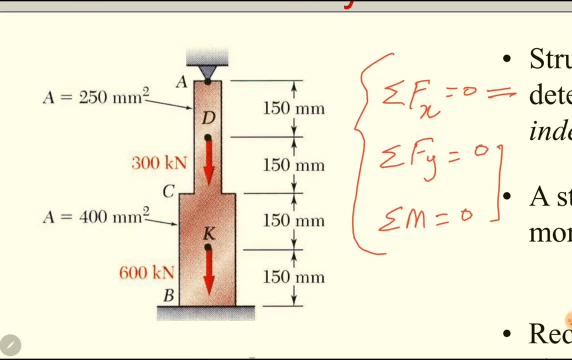 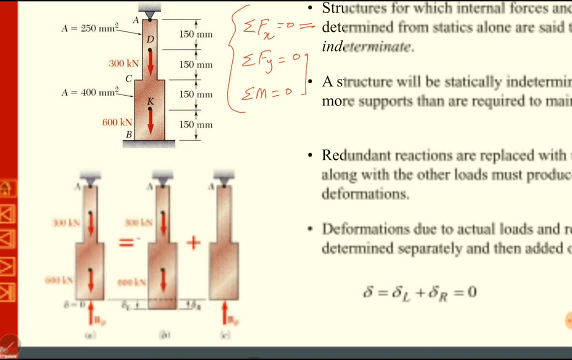 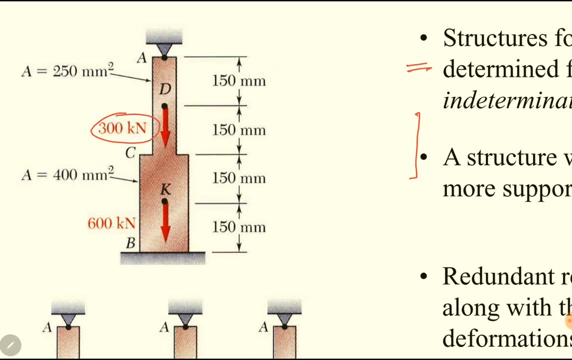 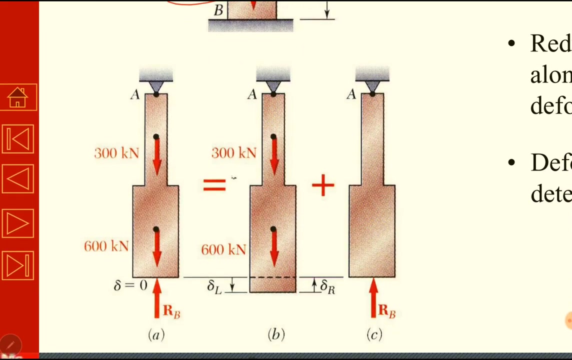 the horizontal, we cannot find all the forces in one direction. okay, now, here this problem is given to us. two forces are known: 30 kilonewton, 300 kilonewton and 600 kilonewton. if we draw a free body diagram here, here is the free. 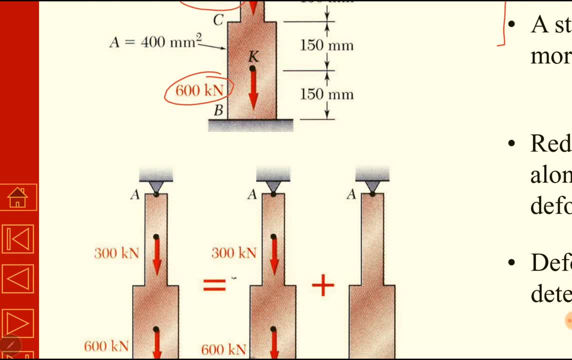 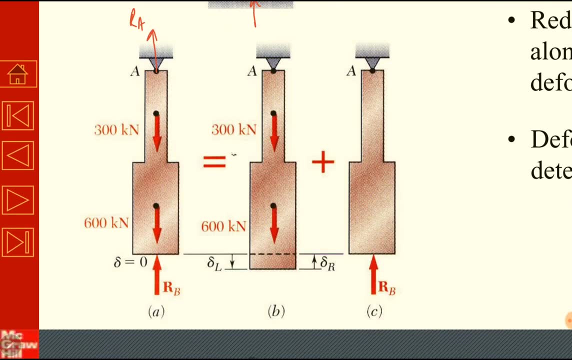 body diagram. there will be one reaction force at point A, R, A and one reaction force at B, where it is resting R, B. so there are two unknown reaction forces. we cannot use equation of forces in horizontal direction. because there is no force in horizontal direction, we cannot use this expression. 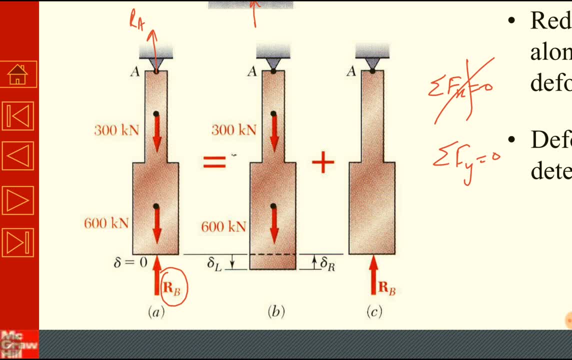 we can use this expression. okay, both unknown forces are in vertical direction, one of the expressions. we cannot use this expression because there is no moment. all these forces, all of the three given forces and reaction forces, are in a single direction, single line of action. so if the forces are in a single line of action, in the same line of action, they 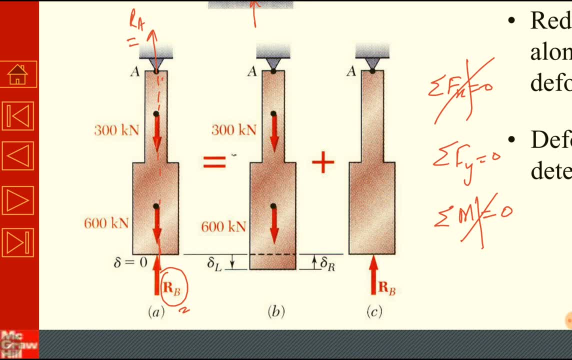 cannot produce any moment, so we cannot use the equation of moment for moment. we need to have offset distance between the two forces, so there is no offset distance, so we cannot use equation of moments. we have only one equation of equilibrium, but we have two unknowns, R A and R B. so this problem is statically. 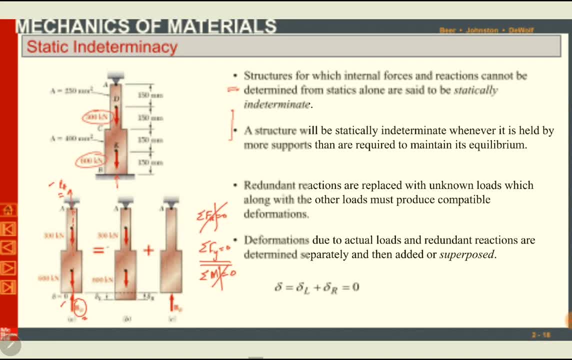 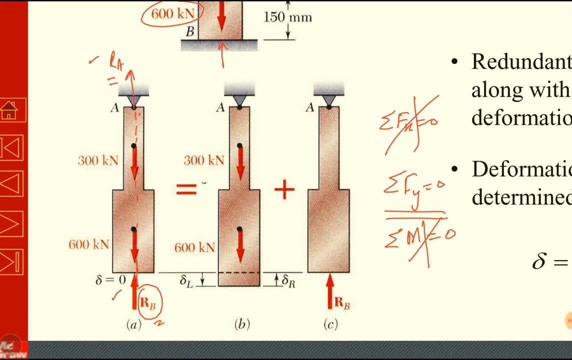 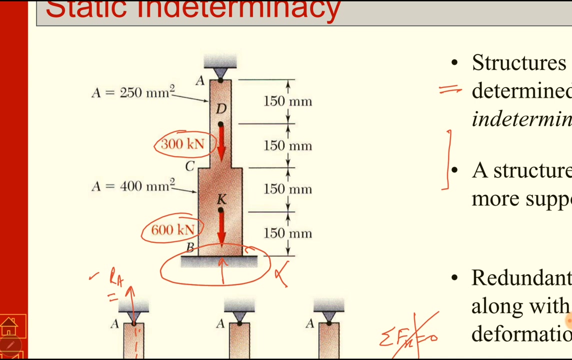 indeterminate now what we can do here. one of these two reaction forces, R A and R B, is a redundant reaction. redundant means we do not need that reaction force to keep the body in equilibrium. even if this- there was no support at point B, this body was still in equilibrium due to the support at point A, or even if there was. 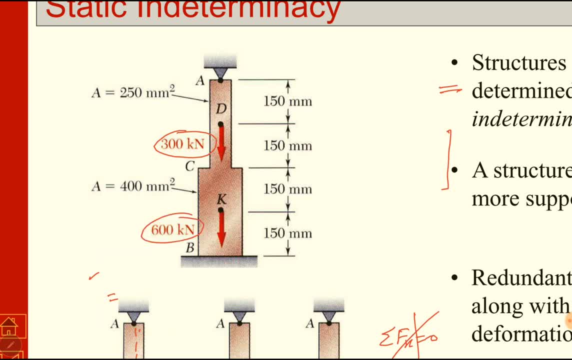 reaction force. or if there was a support at point B but there was no support at point A, still the body would have been in equilibrium because the support at point B. so one of these reaction forces is redundant reaction. it depends upon us. whichever we call redundant, okay. so we will denote one or nominate one of. 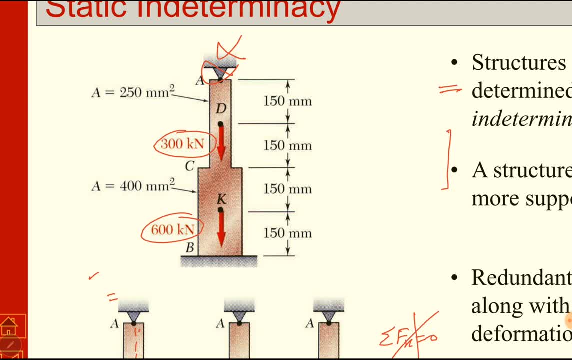 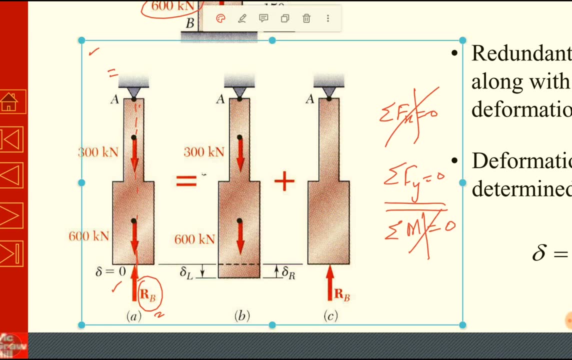 the reaction force as redundant reaction and then we will treat that reaction as a load. reaction is actually internal, but we will keep. we will treat it as a external load. okay, how we will do: first we will remove the redundant reaction. in this case, what we have done, we have removed this redundant reaction in the 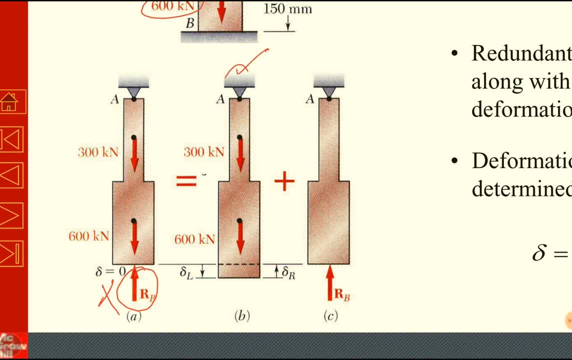 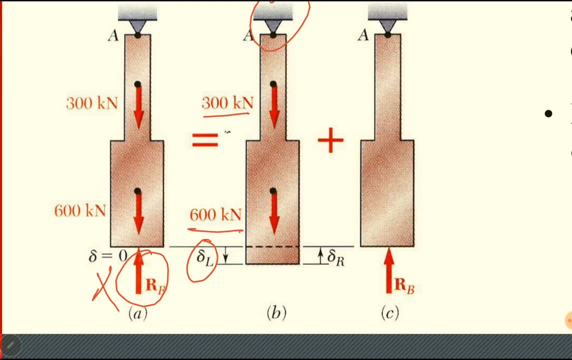 first part. there is only one reaction at point a. there is no reaction at point B. so the applied forces of 300 kilometer and 600 kilometer it will elongate. naturally it will not be relaxed in the envelope. so we have changed the reaction, this body downward and there will be a deformation of delta L because we have removed the reaction. 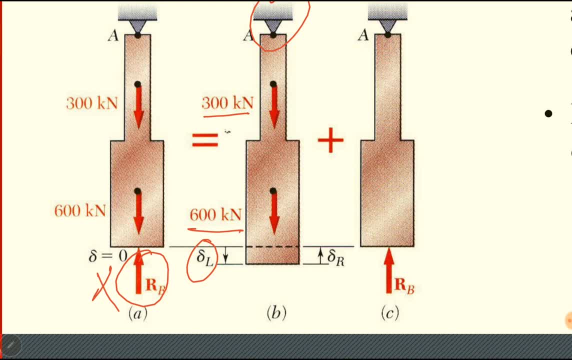 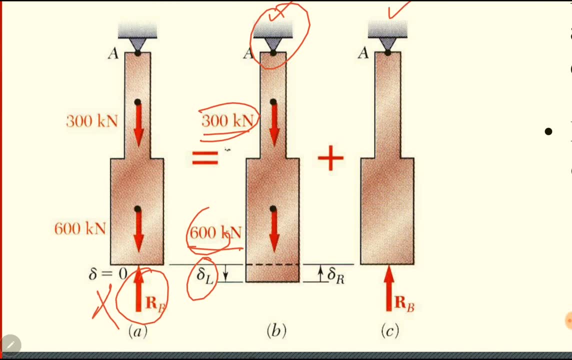 at point P. in the next step we will remove the applied loads of 300kN and 600kN. in this case we have removed the applied loads and we have applied the redundant reaction, which was previously removed in the previous step. we have applied it as a load now. so this redundant 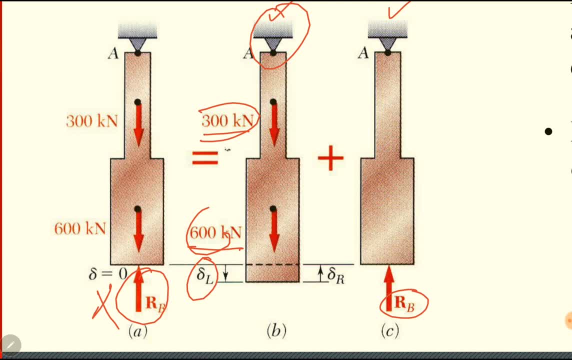 reaction is a compressive load in this case, and it is pushing back the this body and it is pushing it back and this compressive deformation is delta R. there are two deformation: one deformation due to the applied loads- 300 and 600kN- and the other one is due to the redundant reaction. 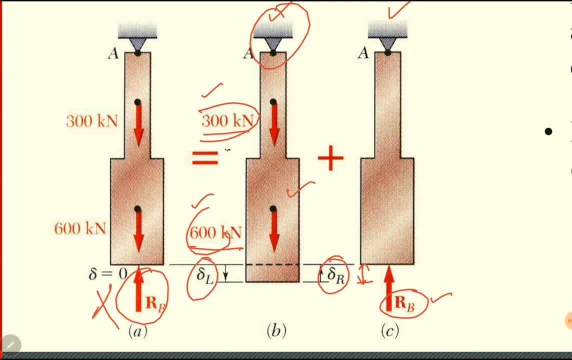 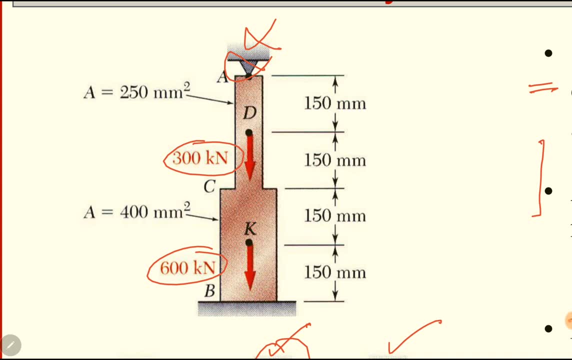 which is a compressive one, delta R. These two deformations are equal But opposite, because at the end this body has no deformation, it is fixed. at both ends there is the net deformation is zero. so the sum of these two deformations del L and del, 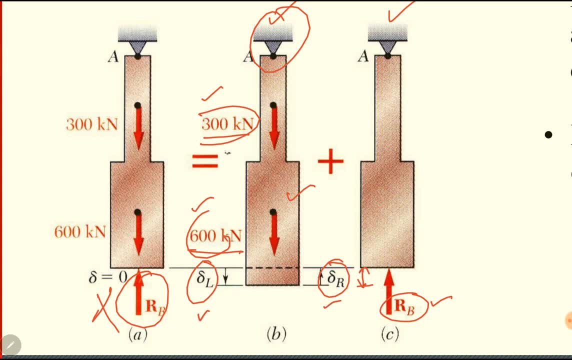 R is zero. in some other case it can be a positive number. if the given deformation is not zero, it should be given in the problem either it is a positive deformation or it is a negative deformation. currently there is no deformation, so summation of del L and del R is zero. 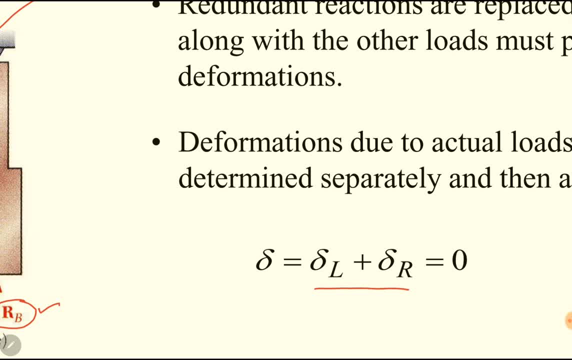 Net deformation is zero. so we have got an extra equation. previously we had only one equation: summation of forces is equal to zero in vertical direction. now we have another equation: del L plus del R is equal to zero. so using these two equations we can now find two unknowns. so now the problem. 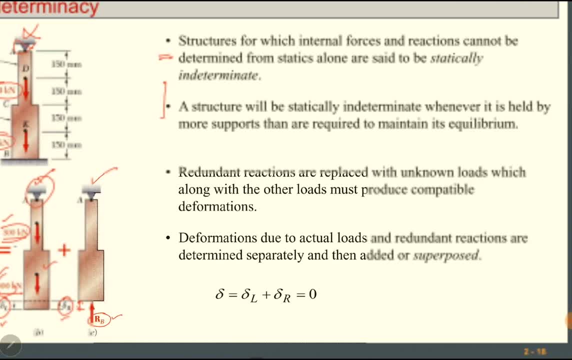 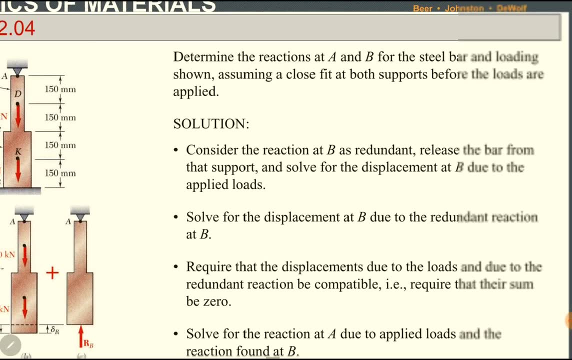 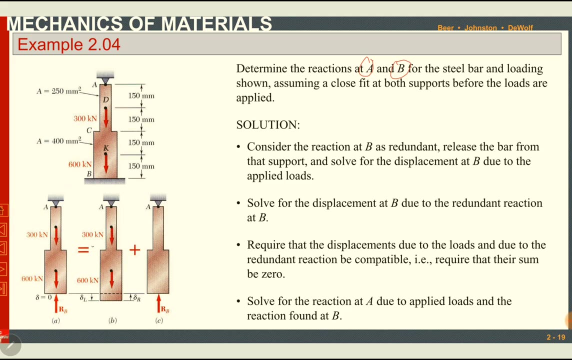 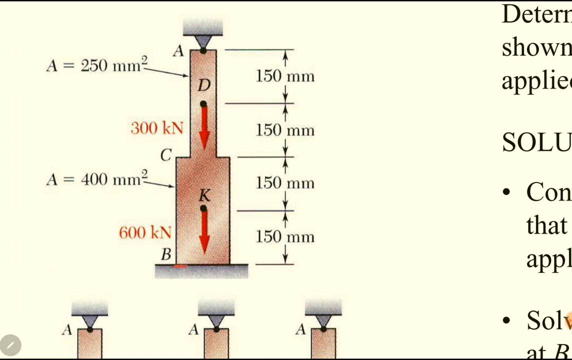 can be solved. okay, we will solve this problem on the next slide. the same problem, example two: points zero four. determine the reactions at point A and B for the steel bar and loading shown. assume a close fit at both supports before the loads are applied. close fit means this body is touched with. 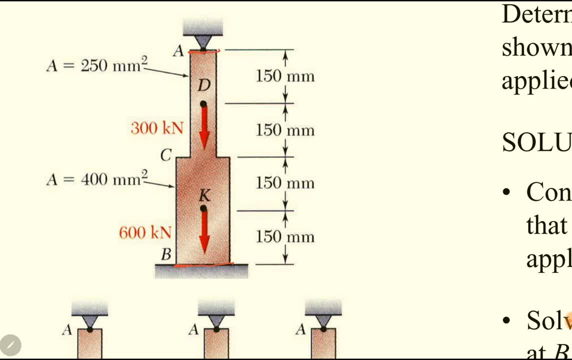 the support at A and it is already pinned at B. close fit means there can be no deformation, there is no space for the deformation. okay, so net deformation is zero, close fit. If there is no close fit, the deformation, the net deformation, will be given in the statement of the. 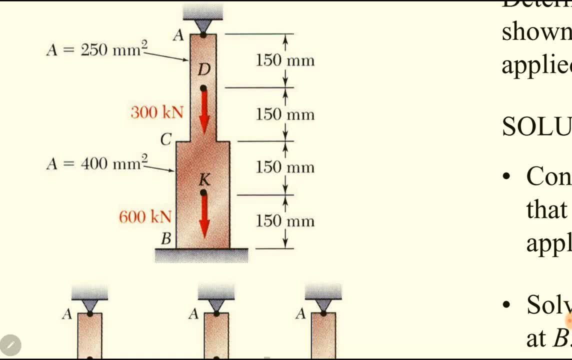 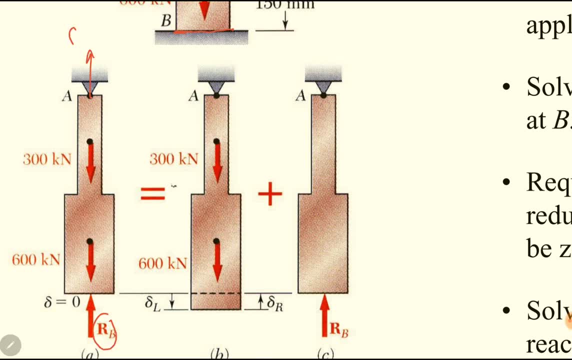 problem. it can be a positive deformation or negative. okay, now we have two reaction forces, as discussed earlier: R B and R A. we cannot solve it using equations of statics, so what we will do? we will treat this R B as an external load. first, we will remove this R B and we will find del L due. 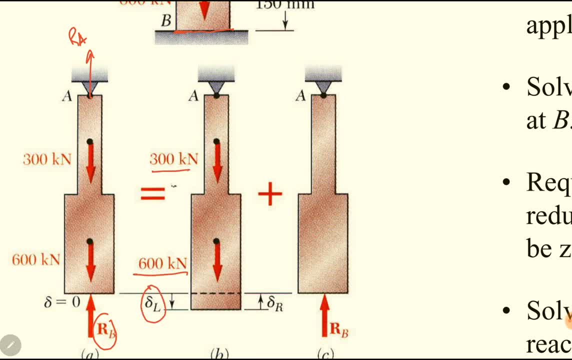 to the applied loads of 300 kilonewton and 600 kilonewton and then we will remove the two loads. in the first case we will find del L. in the second case, we will remove the applied loads 300 and 600 kilonewtons and we will apply R B as a compressive force and to find del R. okay, in the first case. 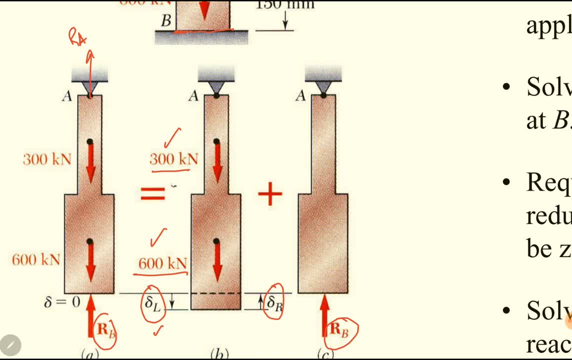 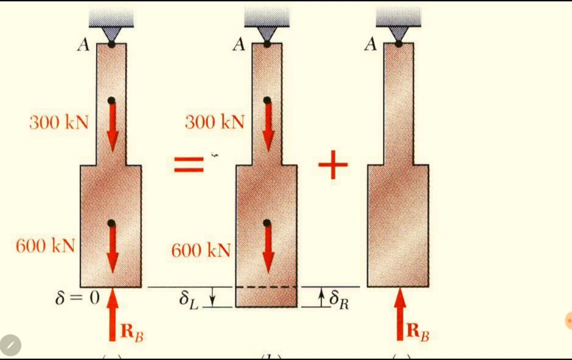 and okay, after that we will add the two deformations del L and del R and we will keep the addition, the sum equal to zero. to get an extra equation, okay, in the first case we have to know the force in each section, area of each section and 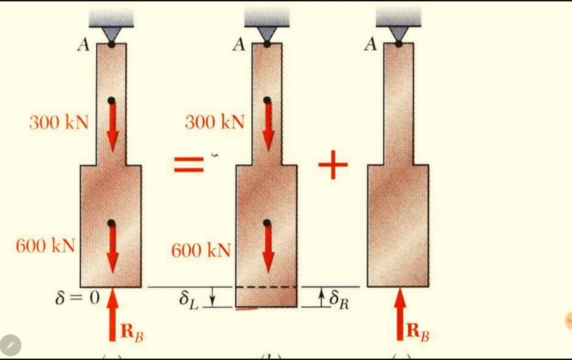 length of each section, starting from the free end. from this end there's no force on the free surface. as we move upward, the force comes here. so between these two points we will section the beam, the the bar. then, moving from here upward, the area changes. at this point so we will section the bar wherever the load changes, where the area. 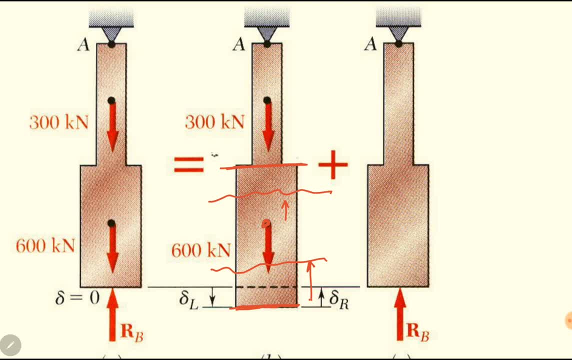 changes. we have to section this bar again. moving upward, the areas same, but the load changes at a point. so we will Section again. and from here upward, at the Fixed point till till the fixed point, we have to Section again. so we have section one, two, three and four. similarly, for this diagram there is a. 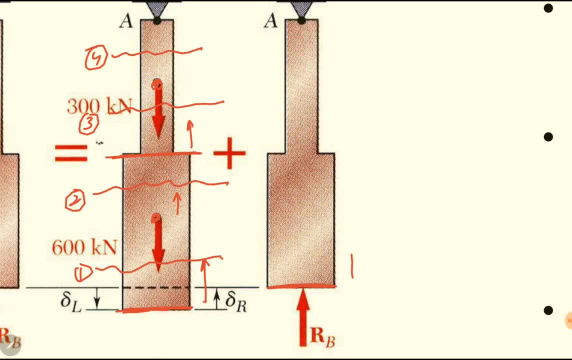 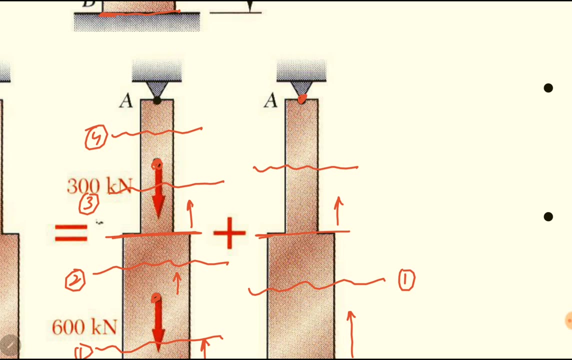 load at the free end. as we move upward, load is constant but the area changes here. so we will section it here, section one. and then, moving upward again, there is no load but the area is constant. load will change are the new load is a reaction force here, so we will section it. okay, we have four sections in the 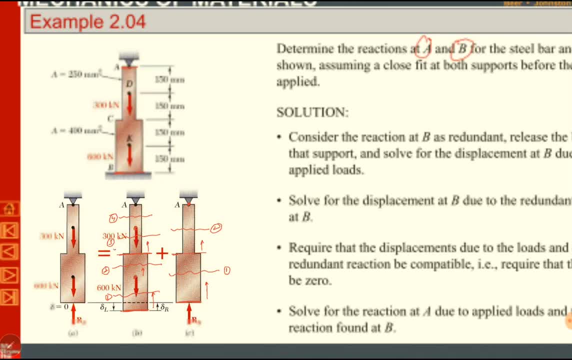 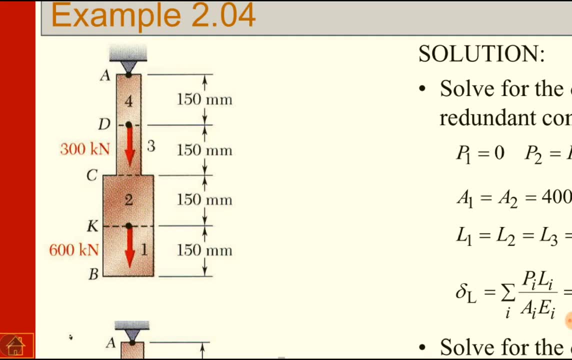 first case, two sections. in the second case we will solve the two cases individually and then the sum will be equal to sum of the deformations will be equal to zero. for section one, the length is 150 mm. load is zero. if I draw this section one, this one, there is no load at the free end. so at the section point, if 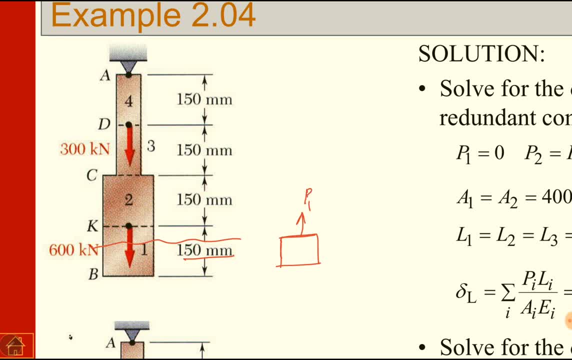 I call a F1 reaction force. wherever we cut, we have to apply a reaction force. the summation of forces is equal to zero, since there is no other force. so this P one does not exist. actually it is zero if I section it here and I draw it like: 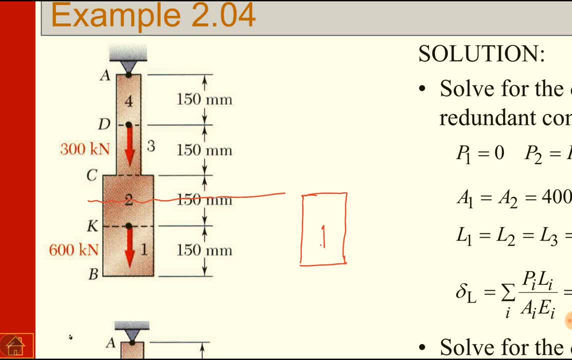 this: there is a force, at point K, 600 kilo Newtons, and there is a reaction force, P to summation of forces are equal to zero. so P2 is 600 kilo Newton and it is tensile because the sin will be positive. similarly, if I section it here in three at section 3, and I draw a free body, 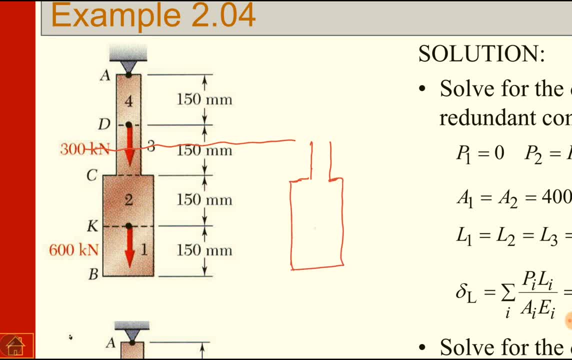 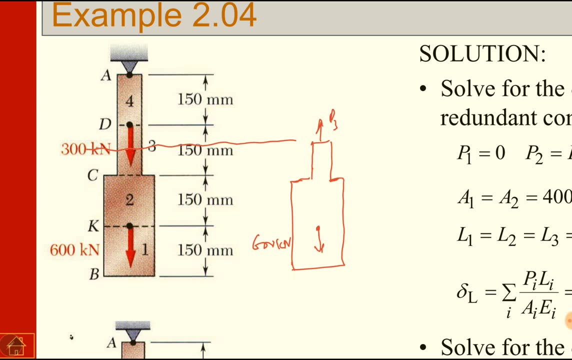 diagram. at point K there is a force of 600 kilo Newton's and at section 3 there is P 3, so P 3 is again equal to 600 kilo Newton's. there is no other force. and if I, if I section the body at 4 and draw a free body diagram, there is a force at point K. 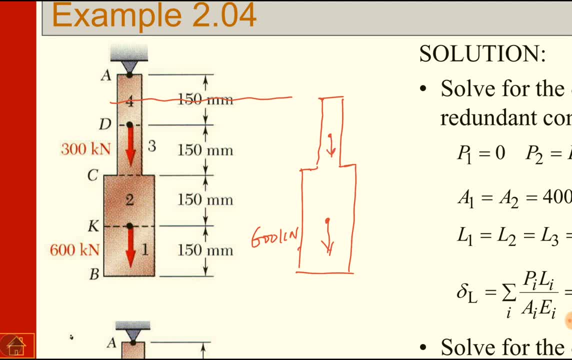 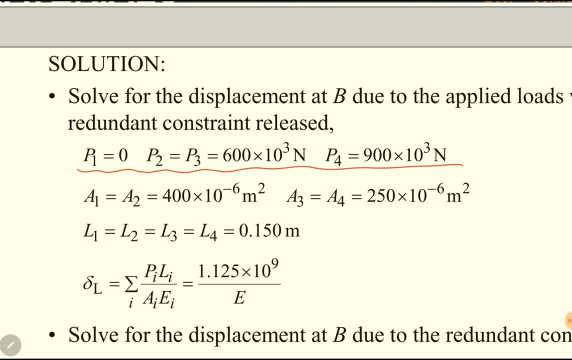 and then there is another force at point D. Now, if the point D is included in the free body diagram, here is P4, so summation of forces is equal to 0 and P4 becomes 900 kN. So P1, P2, P3 and P4 are known in the first diagram. A1 and A2 are given in the problem. 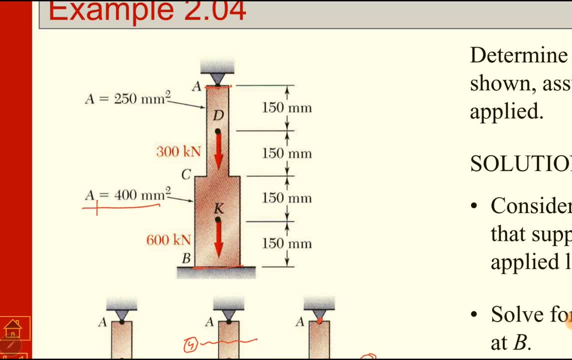 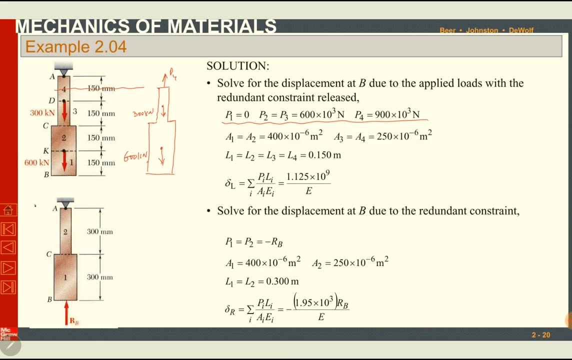 This problem is given A1, this is A1, A2, A1, A2, this is section 1, section 2, they both are same. Similarly, A3 and A4 is same 250 mm square. A1 and A2 are given A3 and 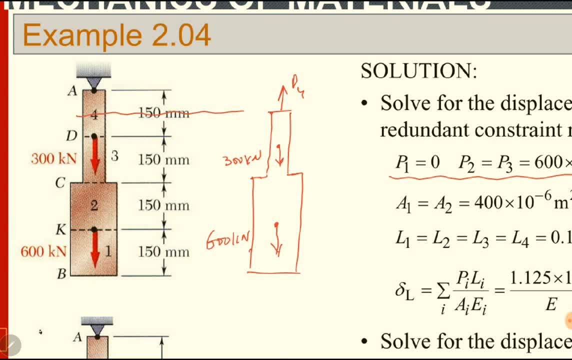 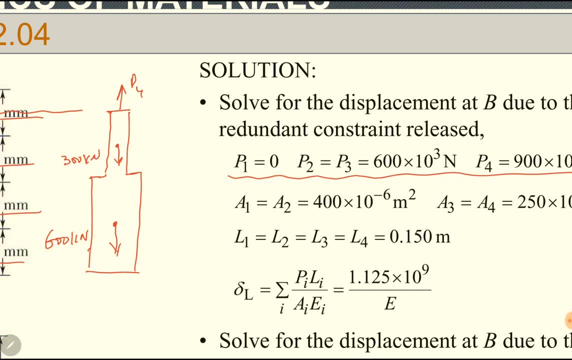 A4 are given. L1, L2, L3 are given. L2, L3 and L4 are also given. This is L1, L2, L3 and all of them are equal to 150 mm. E is same throughout. it is not known to us in this problem, so we will use it as E Summation. 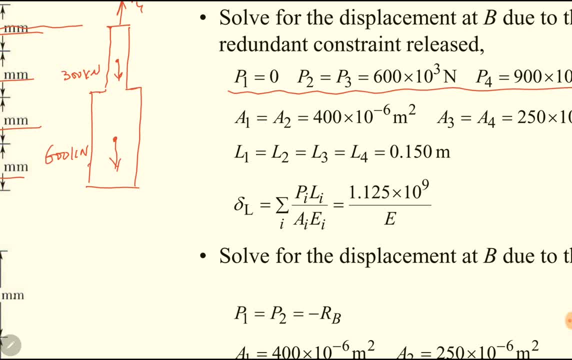 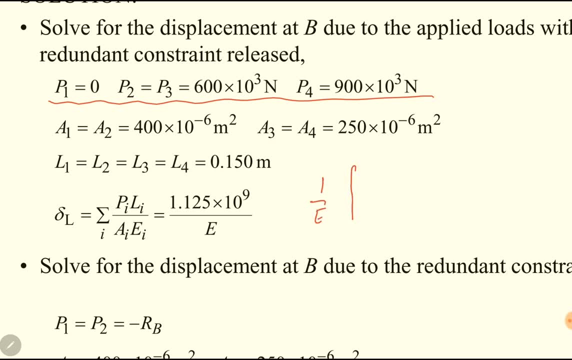 of. we will use this equation of summation. so del L is equal to PILIAIEI. it will be like 1 over E. E is constant. Remember that if any of the load is negative, we have to use it as negative. the deformation: 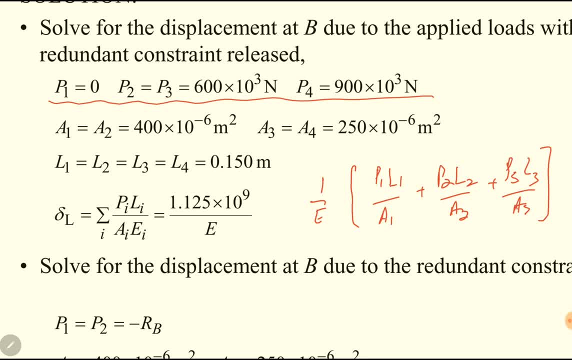 will be compressive and it will be subtracted from the net deformation. So we have got del: L is equal to 1.125 into 10, power 9 divided by E. Similarly, from the next diagram- here we will section it between point B and C, Because this is PILIAIEI it. 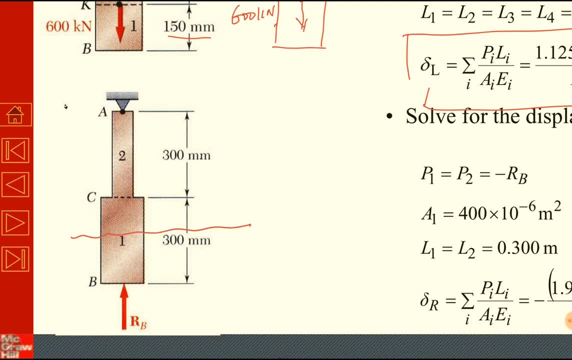 will be like 1 over E. Similarly, from the next diagram here we will section it between point B and C, Because there is no load but there is change of area at point C. So here is RB and here will be P1, because RB is compressive. so I have denoted P1 as compressive and P1 for this case is equal. 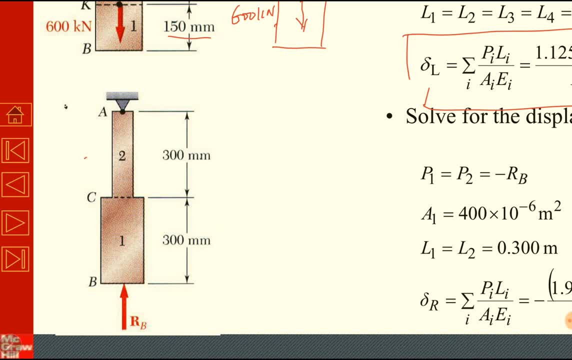 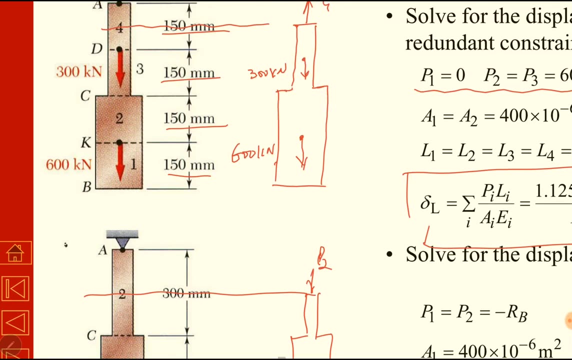 to RB. Similarly, if I section it at 2, so P2 will be compressive again. So we will section it at 2.. P1 is equal to RB. it is compressive. Remember that this P1 and P2 in this section. they are not the same as P1 and P2 in the previous. 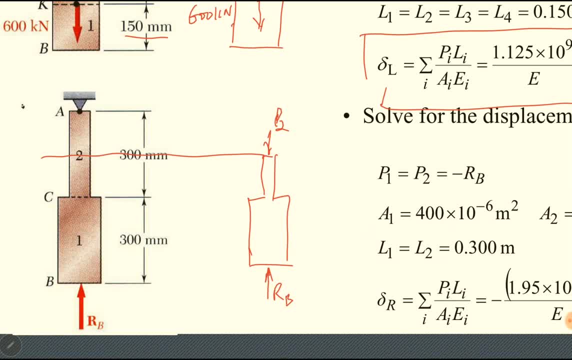 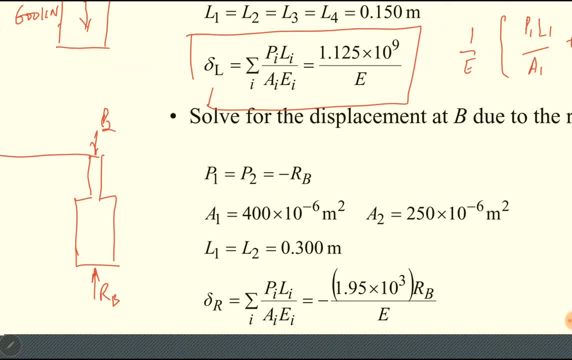 section. if you are getting confused with it, you can denote them with section 5 and 6, P5 and P6.. Anyways, the P1 and P2. both are equal to minus RB, actually, which is compressive A1 and A2,. 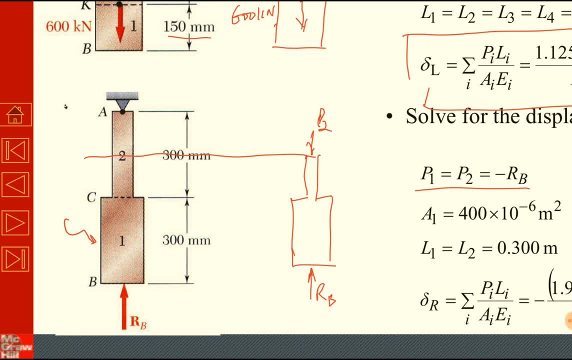 now we have two areas only. we have two sections actually. So first section area is A1. This is P1 and P2. only A1 and A2. they are known to us from the statement of the problem. Similarly, L1 in this case. 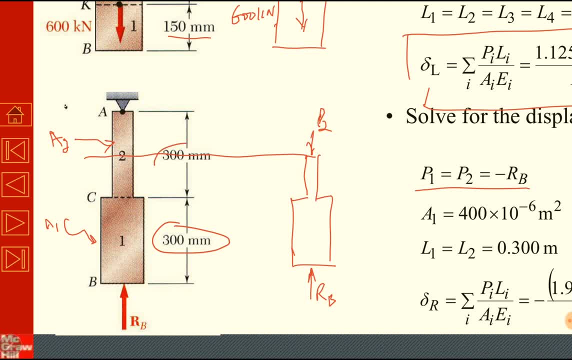 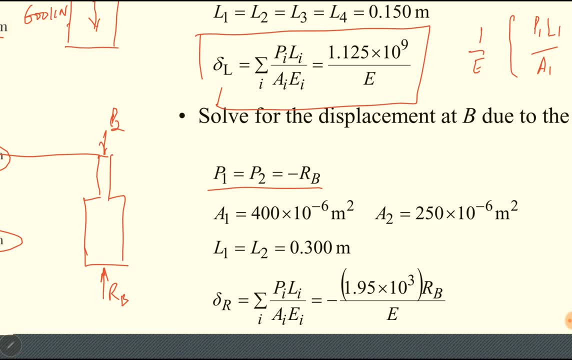 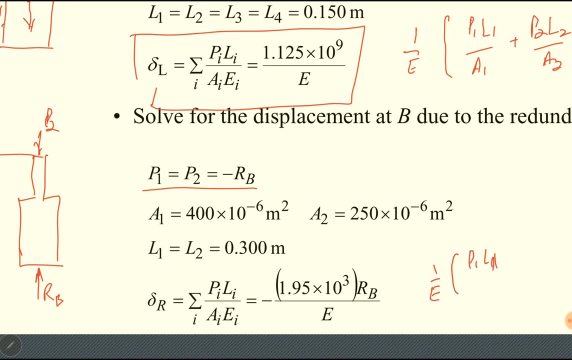 is length of this whole section between B and C, and L2 is between C and A. both are 300 mm. each are 0.3 meters. Now summation in this case is 1 over E into P1, L1 divided by A1, plus P2, L2 divided by A2.. So del R becomes minus 1.95 into 10, power 3 multiplied by RB. 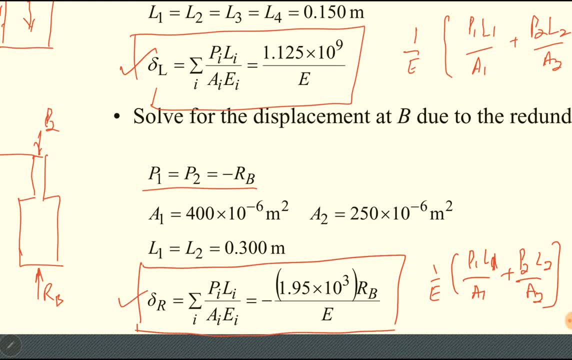 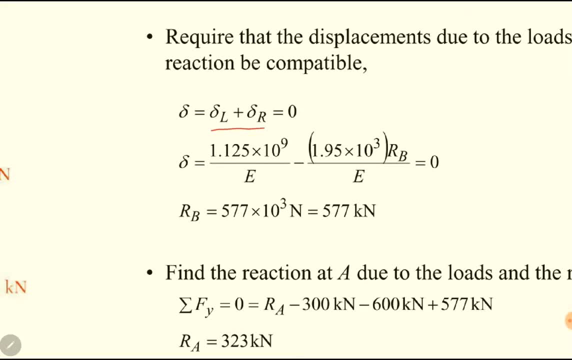 divided by E, Now we have 2 deformations del L and del R. sum of them should be equal to 0.. So del L plus del R, the sum of them is equal to 0. there is only 1 unknown. if we 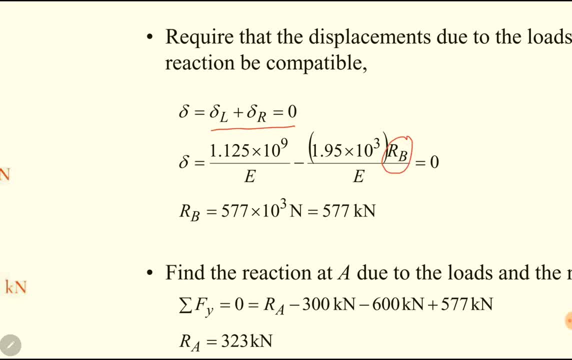 put the values there is unknown RBA, So del L plus del R we have only 1 unknown. if we put the values there is unknown RBA, okay, we can keep E as constant. the ratio is equal to 0, so E cannot be equal to 0. 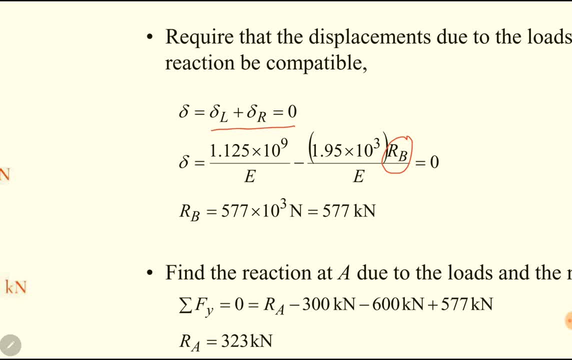 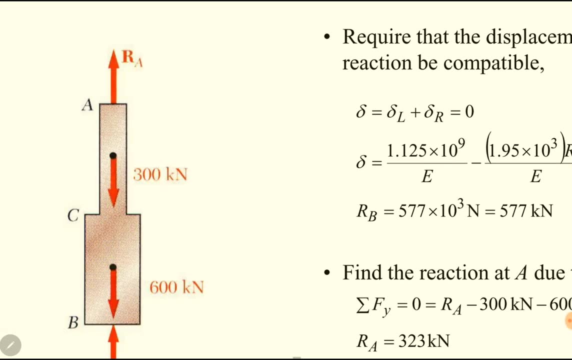 and because it is divided by E and E is a material property, so it definitely. it is not equal to 0. so RB has been calculated: it is 577 into 10 power minus 3 Newton's, or 577 kilo Newton's. now the RB is known to us. if RB is known to us, 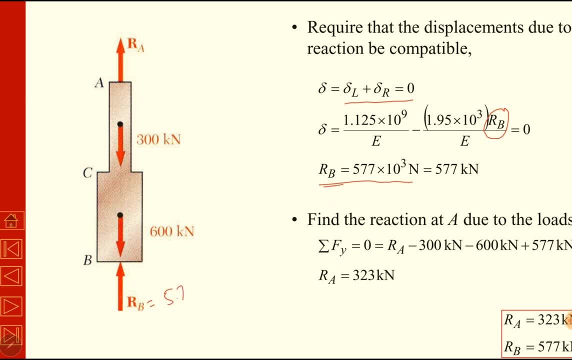 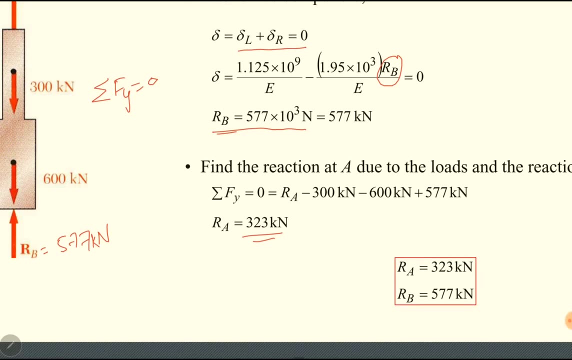 from this diagram if RB is known, so there's only one unknown, and we can find it using equations of equilibrium. now it is statically determinate. summation of FY is equal to 0, so FY will be 323, put all the values, 323 kilo Newton's. so we 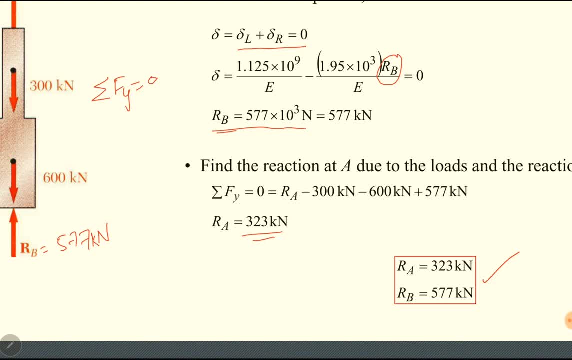 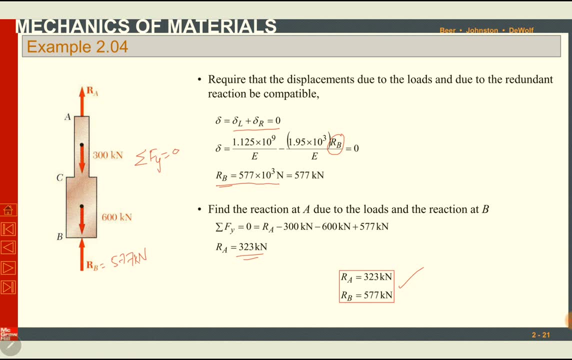 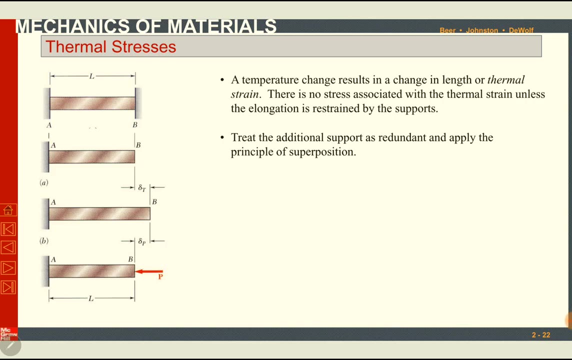 have calculated both the reaction forces, RA and RB. okay, I hope the concepts are clear and if there is any questions you can ask me through email make. the next topic is thermal stresses. as evident from its name, thermal stress is due to a thermal change and due to 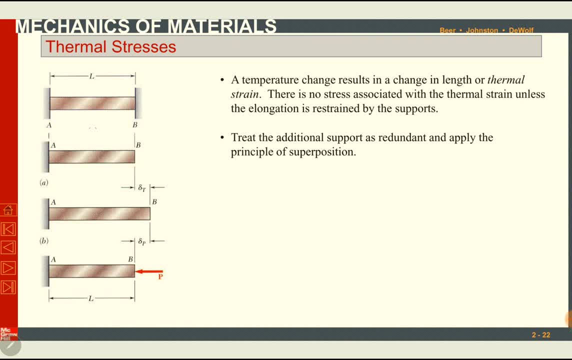 increase or decrease in temperature. due to increase in temperature materials usually expand, and due to decrease in temperature the materials contract. this expansion in the length of volume and contraction is deformation, and dividing that deformation by the, by the initial length, is a normal strain. so as soon as the material expand or contract, there is a 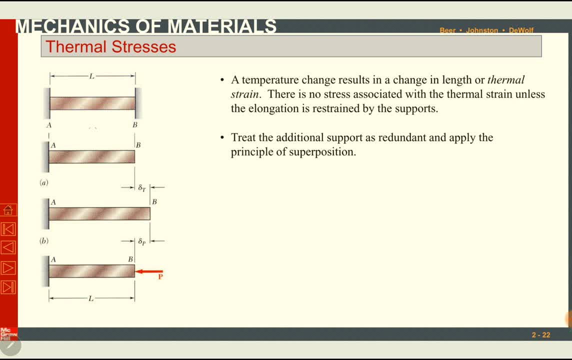 normal strain, tensile strain or compression strain, which is called thermal strain because it is due to the change in temperature. the material is allowed to expand freely or contract freely due to a change in temperature, so it will have a thermal strain, but there will be no thermal stress, because there 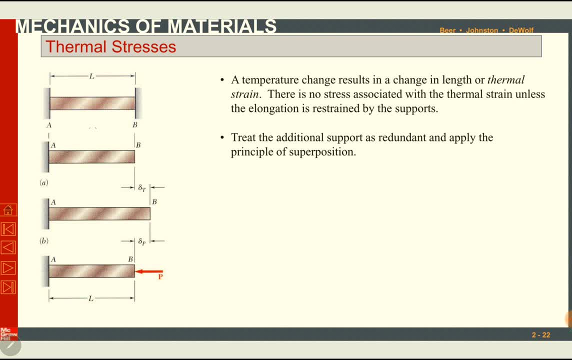 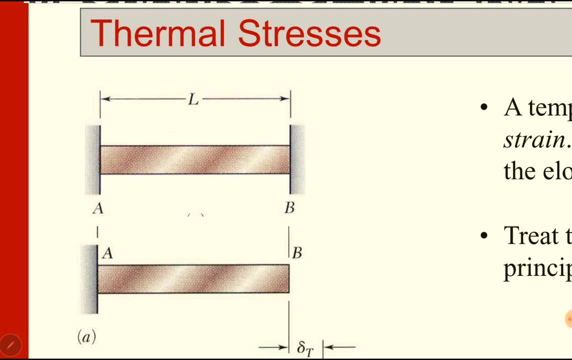 is no restriction. it is expanding or contracting freely. so in order to have a thermal stress, we need to stop that thermal expansion or thermal contraction. just like this figure, a member has been constrained from the two ends and A and B. if there is a thermal change, if the temperature 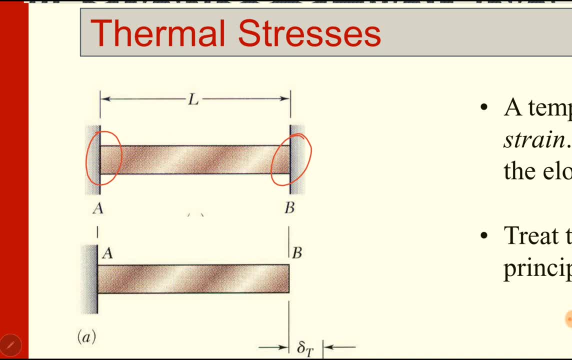 increases. this bar cannot expand in the horizontal direction, so there will be a thermal stress in the horizontal direction, but there will be no thermal strain because we have stopped that expansion. similarly, if we stop a contraction, there will be a. there will be no thermal strain again and there will 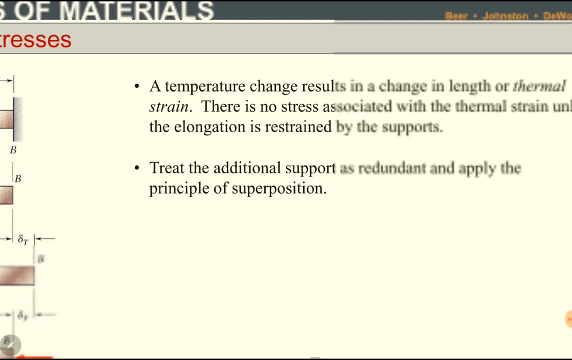 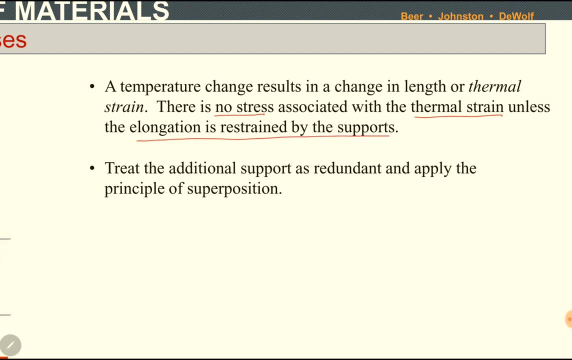 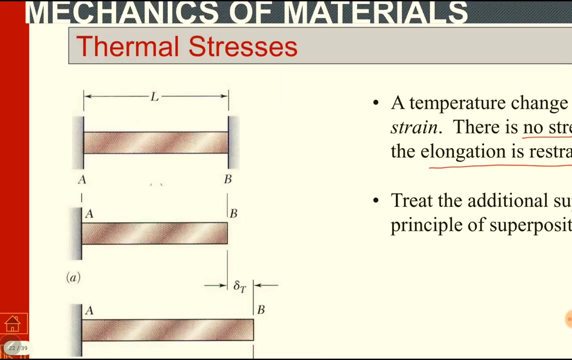 be thermal stress. so there is no stress associated with the thermal strain unless elongation is restrained by the supports. so we have to stop the free expansion and free contraction due to temperature change in order to have thermal stress again. a problem of thermal stress is like a statically indeterminate problem we we can see in 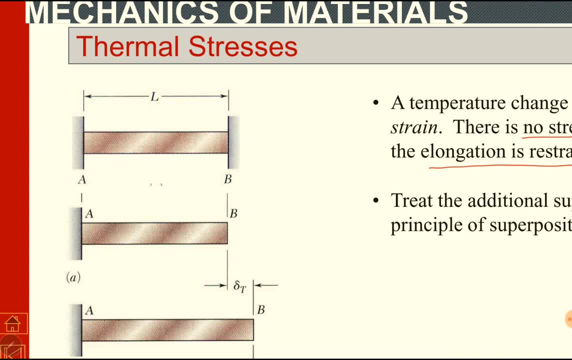 this diagram and the bar is constrained or restricted from both ends. there are reaction forces on both ends and the number of forces on both ends are of. reaction forces are more than number of equilibrium equations and the problem is statically indeterminate. there will be two unknown reaction. 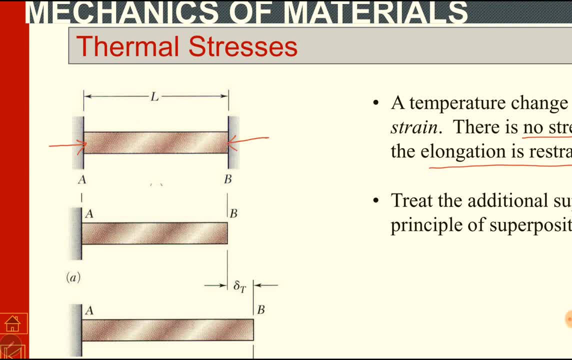 forces at the end. these two constraints are applying a compressive. if the temperature is increasing, for example, the bar will try to expand and the two constraints at the end will try to compress back, compress it back to the original length. so there is a compressive force at two ends. this these- 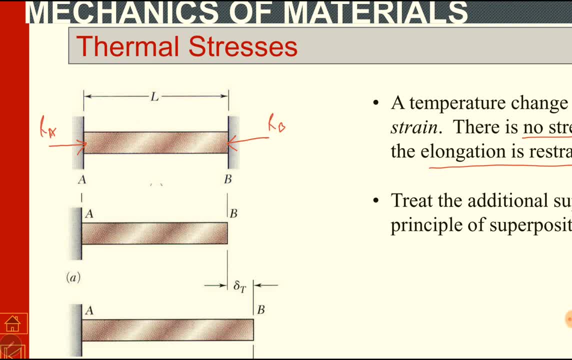 two compressive forces are A and R. B are unknown because they are two, so we cannot find it using summation of forces in X direction. we have only one equation in this case and using this equilibrium equation we cannot solve this problem. we cannot calculate these two reaction. 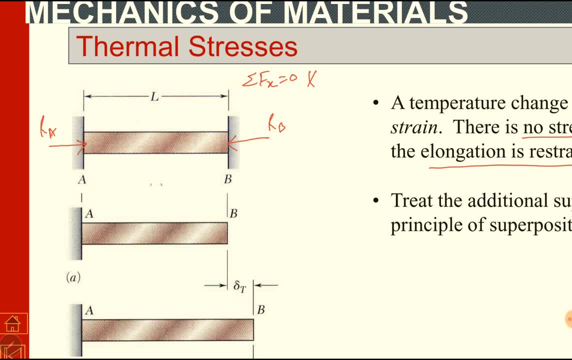 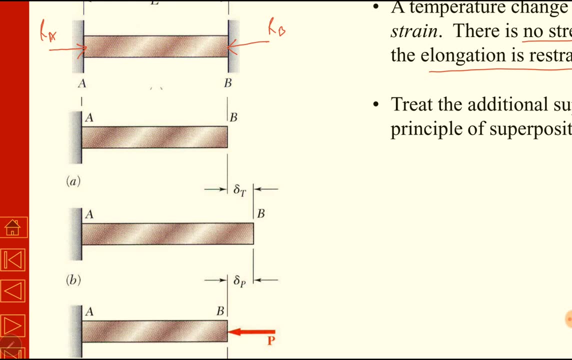 forces. so what we have to do, just like the previous topic, we will consider one of the reaction as a redundant reaction. for example, the R B is redundant reaction. so we have removed this redundant reaction from B and we have left the bar expand freely in the horizontal direction from the end B. so 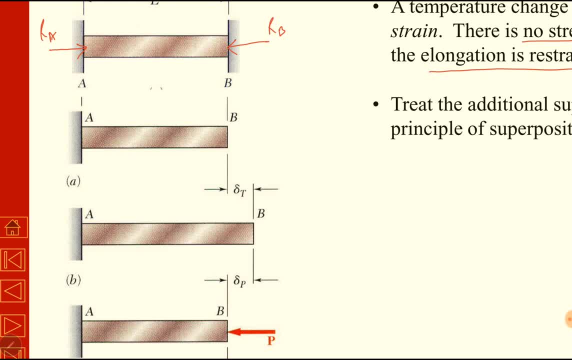 under an increase in temperature it will expand by an amount of Delta T, thermal deformation. this Delta T will be equal to alpha Delta T L. alpha is coefficient of thermal expansion, delta T is the change in temperature and L is its initial length. now what we do after calculating this Delta T: change in temperature, a change in 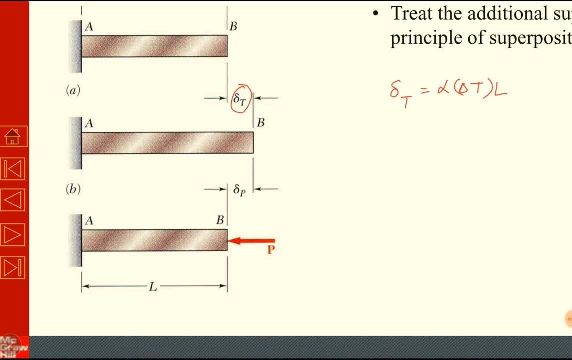 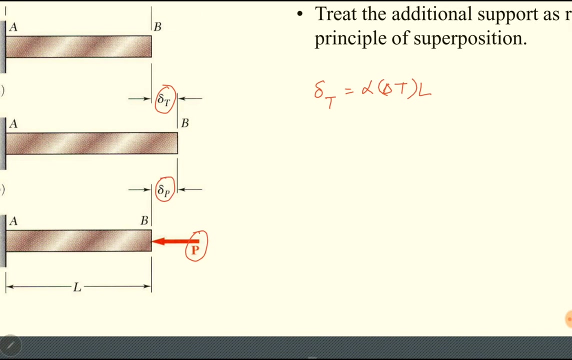 length due to temperature, deformation due to temperature. what we do? we have to apply the redundant reaction as a force, the compressive force P in the next step, and this compressive force will compress the bar AB again to its original length L. this compression is del P, which is due to the force, and previously we have 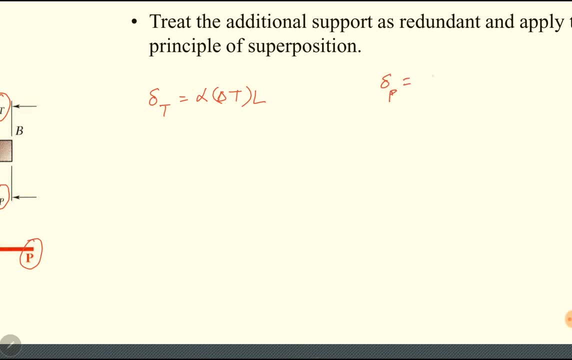 studied that deformation due to force is equal to PL over AE. in the beginning of this chapter we have derived this expression. so this deformation del P is due to the applied force P, which was actually due to the reaction at point B, and this delta T is deformation due to thermal change, due to 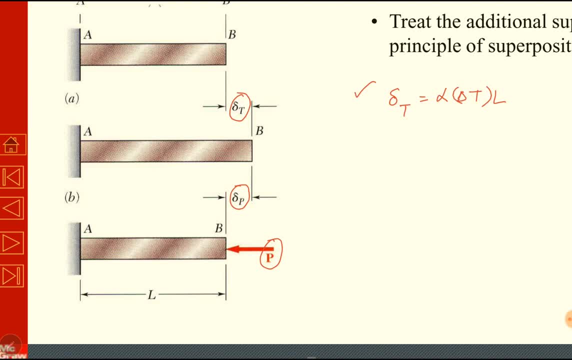 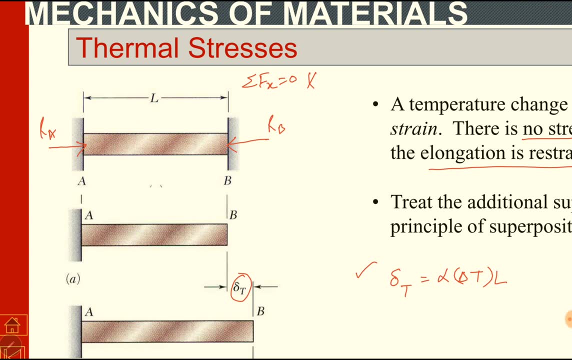 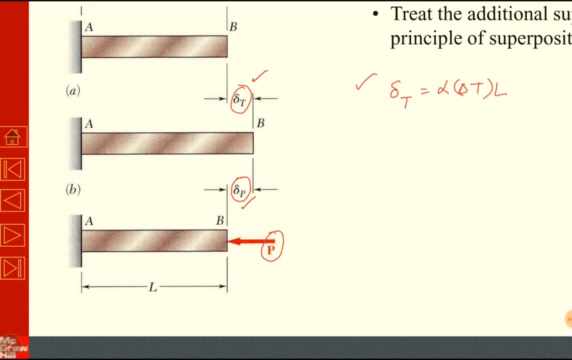 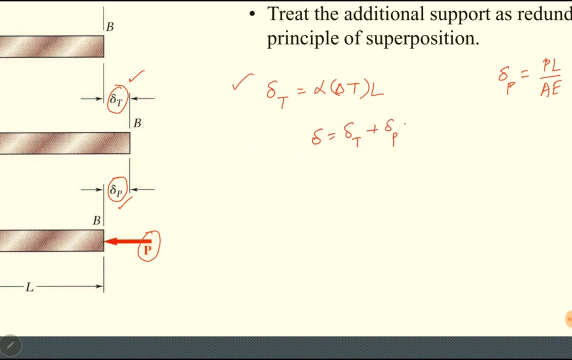 temperature. now, at the end, we know that there is no increase or decrease in the length of the bar. the net deformation is zero because it is fixed from both ends. so sum of these two deformations, del T and del P, must be equal to zero. the net deformation which is sum of del T plus del P is equal. 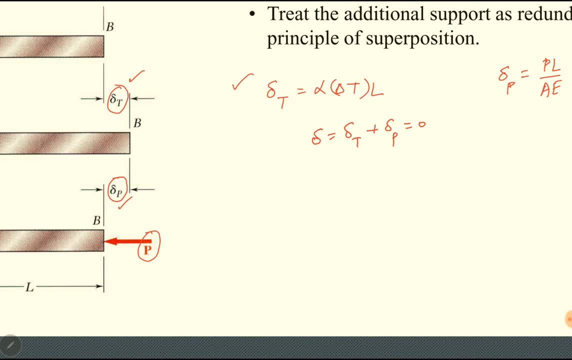 to zero. so by inserting the expressions del, T is equal to alpha, Delta T, L, alpha plus del P is equal to PL. over AE is equal to zero. so we can calculate force from here. P is equal to minus AE, alpha, Delta, T. negative sign means this force is. 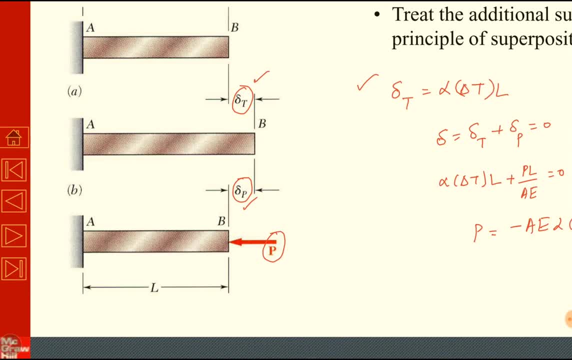 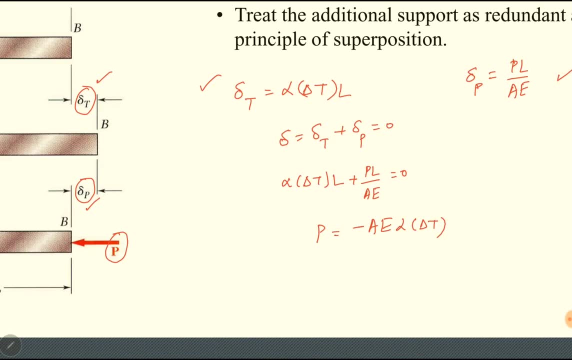 compressive, which is definitely a compressive force. it is trying to stop our expansion, so it must be a compressive force. this compressive force is equal to minus area into modulus of elasticity, into coefficient of thermal expansion, into change in temperature. del T is the net change in temperature if we 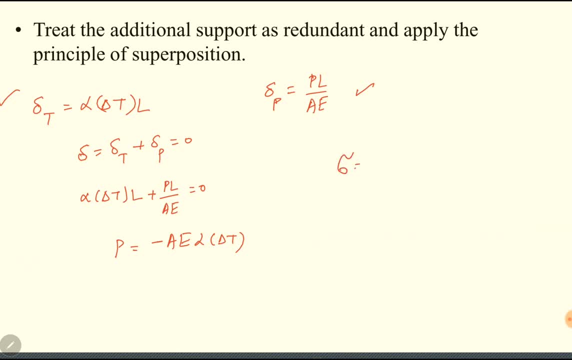 divide this force by area so we can find thermal stress which is equal to force divided it is a kind of normal stress, so it is equal to P over A. by dividing this force, P over area, so we will get minus E, alpha del T. this is thermal stress which is compressive in the nature against. 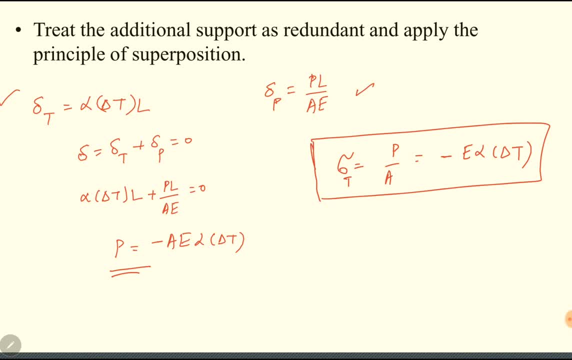 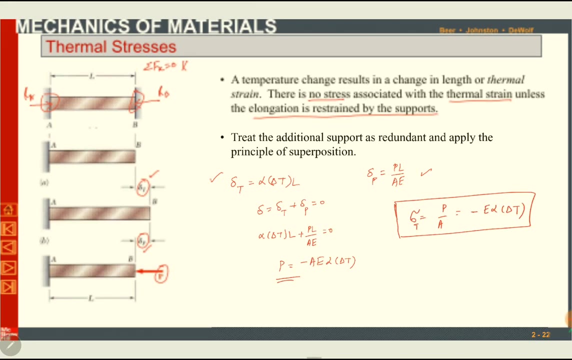 thermal expansion against an increase in temperature. similarly, the same expression will can be derived for a tensile force against a thermal compression. there will be no negative sign. the expression will be similar. okay, so we can calculate thermal stresses in the same way, just like we have done. we 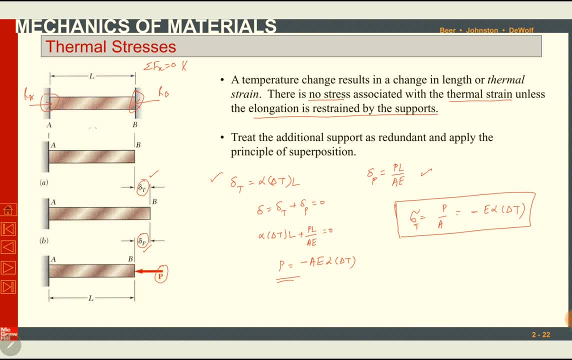 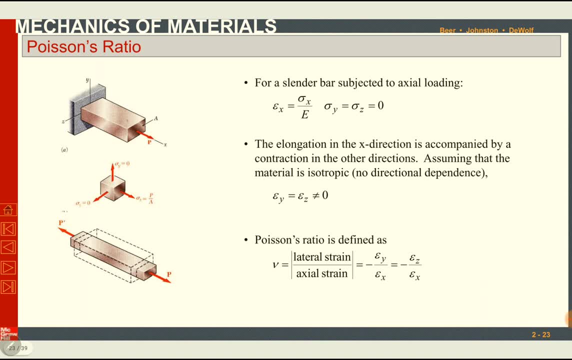 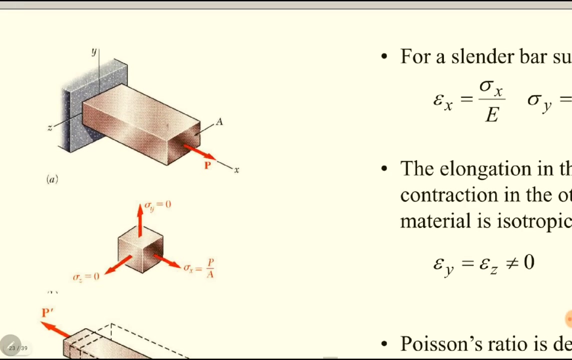 have followed a procedure for statically indeterminate problems. well, the next topic is poisons ratio. it is a very important parameter, poisons ratio. it is defined for ductile materials. really, a slender bar is shown in the diagram and force is being applied in the horizontal direction, X direction, so there will be stress in the 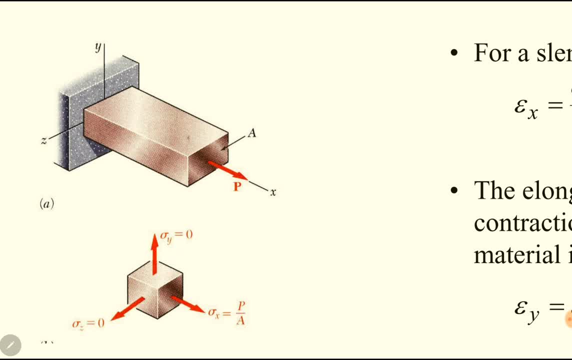 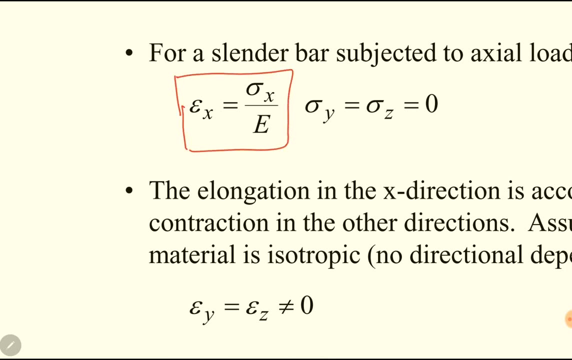 extraction and strain. in the extraction there is no stress or no force in the y and z direction. so initially we think like there is no deformation or no strain in the y and z direction. we just defined strain in the x direction is sigma X over e. this is Hooke's law. we are 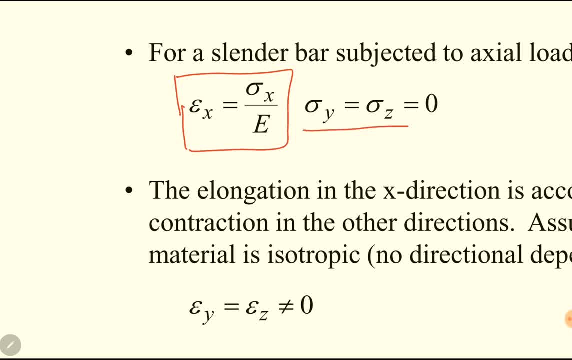 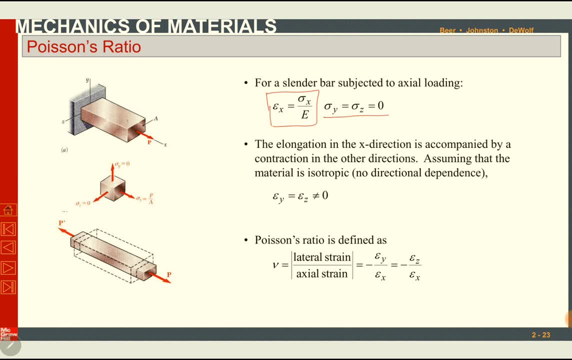 just discussing about elastic deformation. only. there is no stress in the y and z direction because there is no force in the y and z direction. ok, the elongation in the x direction is accompanied by a contraction in the other two directions, assuming that the material is isotropic. isotropic means there is no directional. 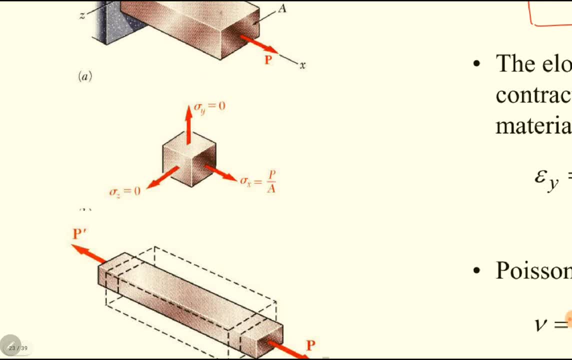 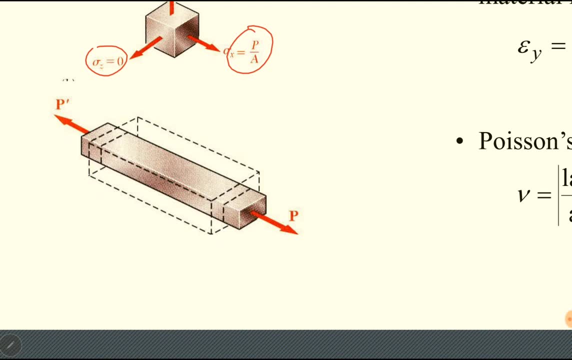 dependent property. so the stress in the X direction. there is no stress in the Y and Z direction, but due to the expansion in the X direction, there will be contraction in the Y and Z directions. this is this property is a property of deformable materials, ductile materials specifically. so remember that whenever 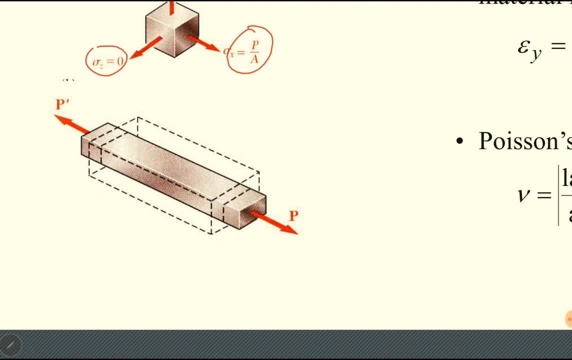 we apply or whenever we deform a material, one of the three directions it will have, it will experience an opposite formation in the other two directions. if the deformation in x direction, the applied deformation, is tensile, so there will be compression in the Y and Z direction, and if the 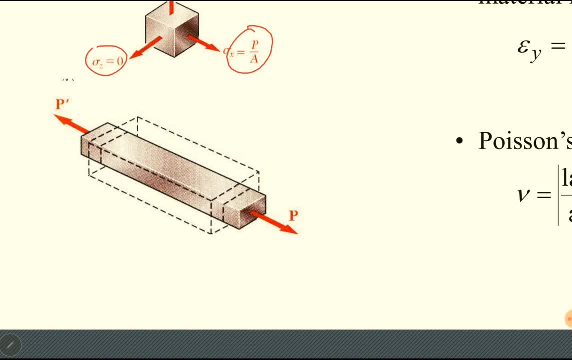 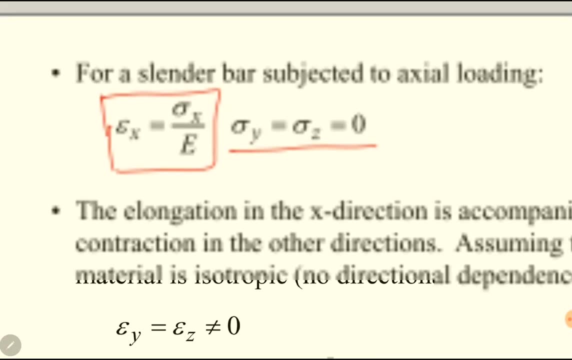 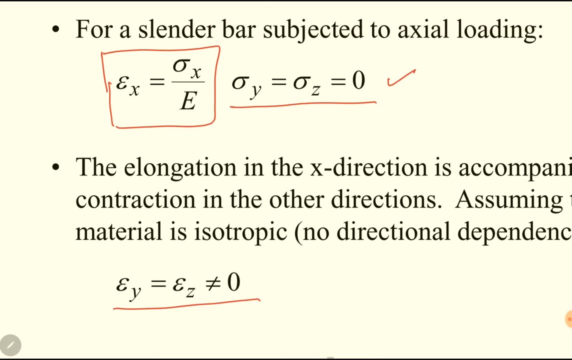 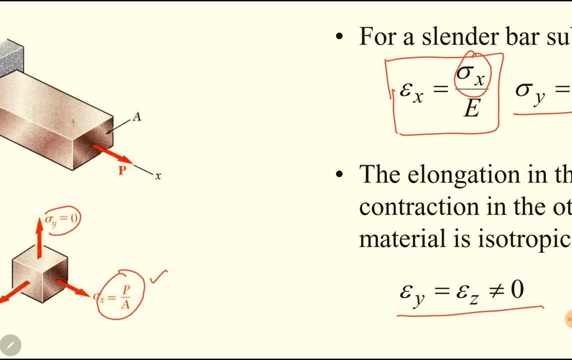 applied deformation in the x direction is compressive, so there will be tension in the Y and Z directions. so there is zero stress in the Y and Z direction. but there is not a zero strain in the y and z direction due to the stress in the x-direction. Sigma X, which is equal to p over a, due to the stress in x-direction. 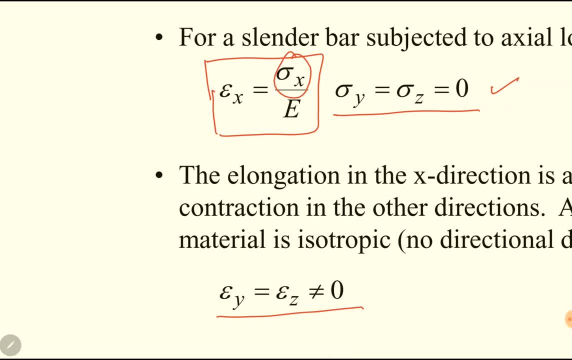 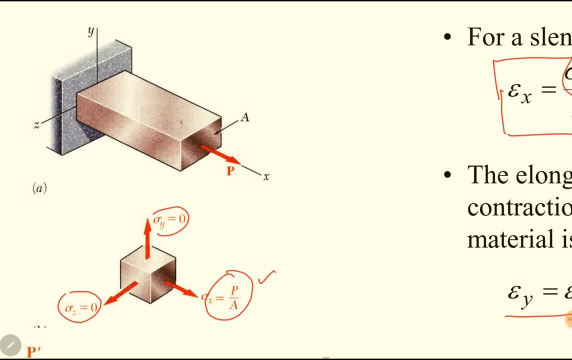 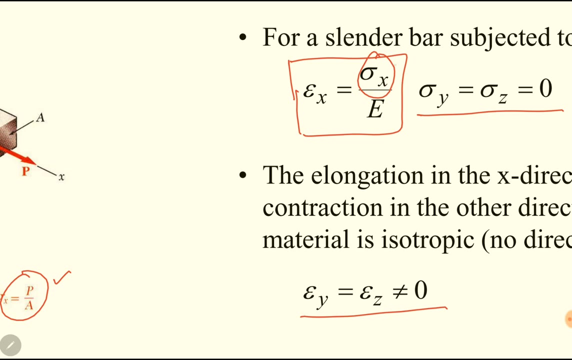 there is strain in the y and z direction, so we call this strain as lateral strain. the stress, the strain in the axial direction or the direction of force is called axial strain and the strain in the other two directions is called lateral strain. so this strain- epsilon y and epsilon z- due to the stress in x-direction. 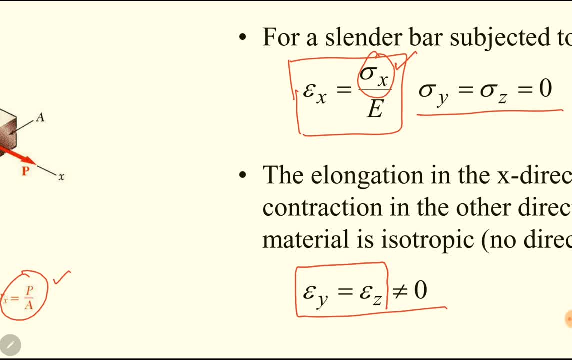 will be same. epsilon y and epsilon z are. strain in the y and strain in the z direction will be same. the compression in the y and z direction- not the compression, actually the compressive strain in the y and z direction will be same and it will not be equal to zero. so we here, we define: 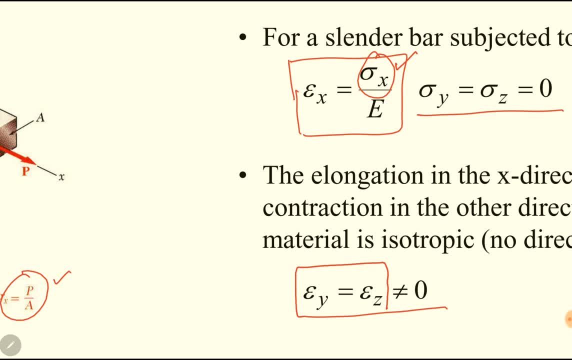 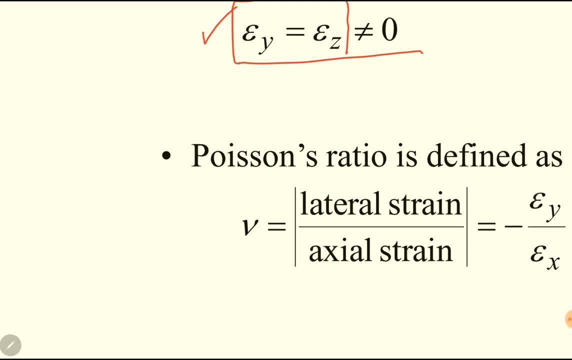 a a new parameter and which is called Poisson's ratio. it is a ratio of two strains: the lateral strain divided by the axial strain. the lateral strain which has been produced due to the axial strain. the lateral strain divided by the axial strain. axial strain is produced directly due to the axial load and 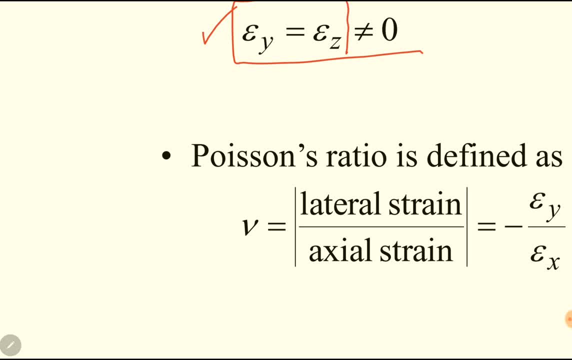 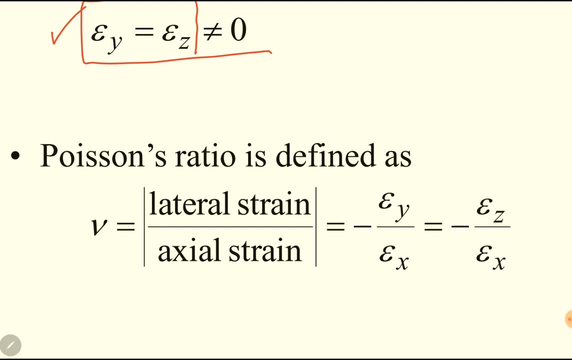 lateral strain is a result of the axial strain. these two will always be in the opposite direction. if the axial strain is tensile, the lateral strain will be compressive, and if the axial strain is compressive, the lateral strain will be tensile. okay, so this Poisson's ratio must be a positive number. that is why we 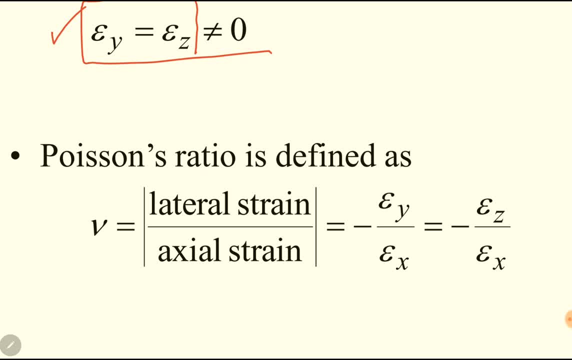 have kept it in the two vertical lines, absolute lines, and one of the lateral or axial strain must be compressive. if the axial strain is tensile, lateral will be compressive. if the lateral strain is tensile, axial strain will be compressive. so one of them will be negative. so the total 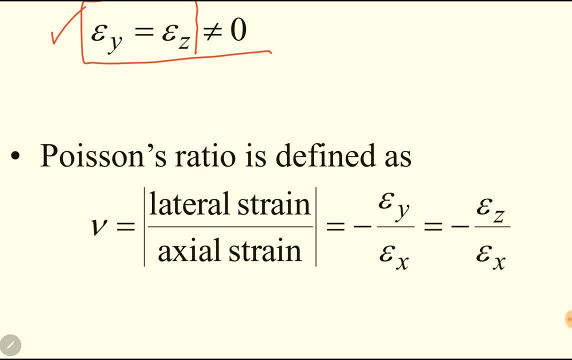 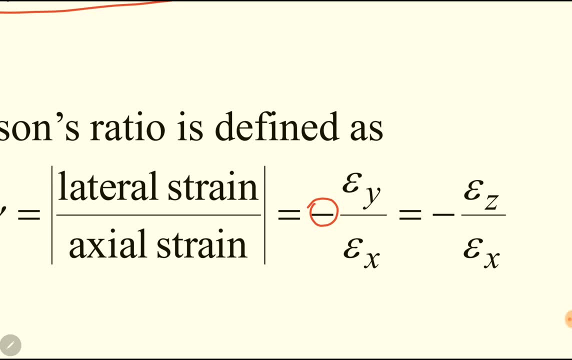 number, the total ratio, comes out to be negative. so that is why we are multiplying it with a negative sign, so that the total becomes, or the net value becomes, positive. one of the epsilon Y are epsilon X will be negative compressive. so by multiplying that negative with a negative sign, it will be. 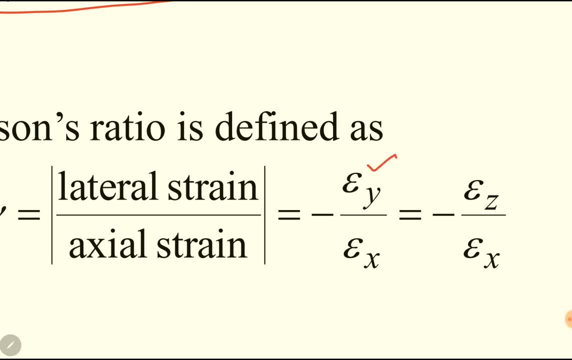 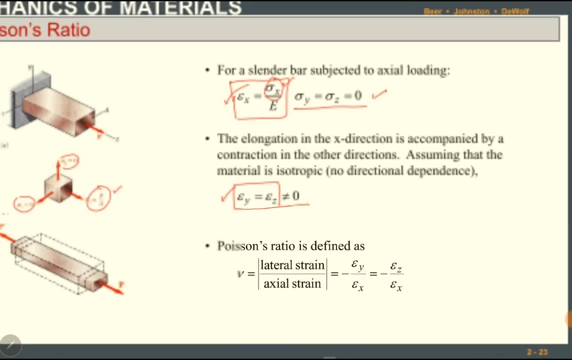 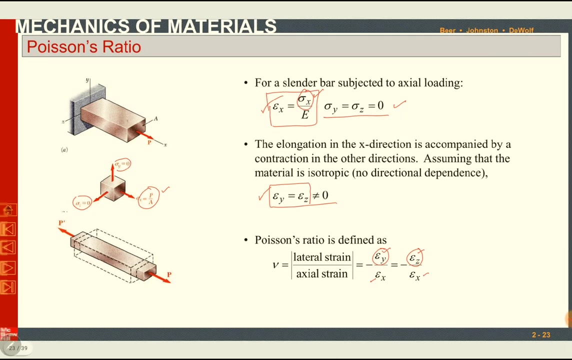 positive. similarly, strain in Y divided by strain X are strain in Z divided by strain X, ratio will be same because this number, strain in Y and strain in Z, these two strains are same. okay, so we will use this Poisson's ratio, this concept, in our upcoming topics. this is a very important topic. okay, now we 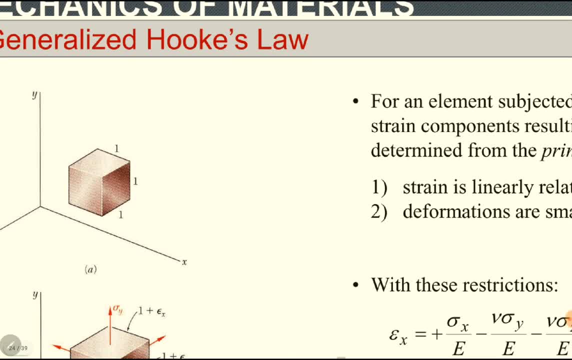 are going to use it. previously we have discussed that due to stress in the axial direction- one of the axial direction, for example, in the X direction, there will be stress P over A and there will be strain in the joint draw of A and there will be strain in the joint draw of B. 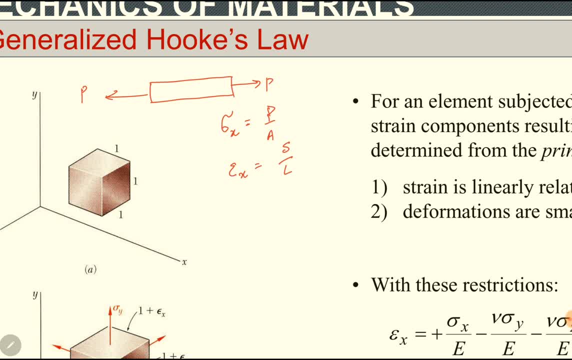 and there is strain over L. okay now, in the X direction there is strain due to the force in Y direction as well as to the force in Z direction. if there is force in Z direction and Y direction, there will be strain in the XXL as well. doツ 도 Ģ LORD. the Hook's law was defined for single direction only, for example, stri诊 modified by a single direction only, for example, strain in the general direction. Are거든요 is the human contact. so if your distance remains carefuly dependent, then أو by any ability to μέ souha inteiro். 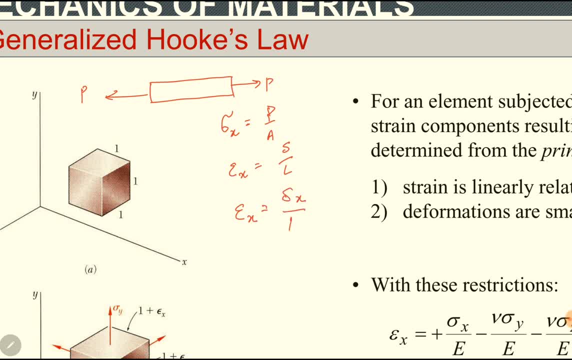 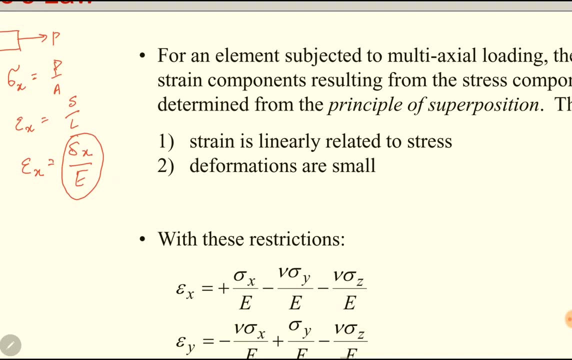 strain in x direction is equal to stress in x direction divided by modulus of elasticity. this component of strain is only due to the force or the stress in the x direction, but there will be contribution of forces in the y and z directions as well. so we can write it like this: the strain in 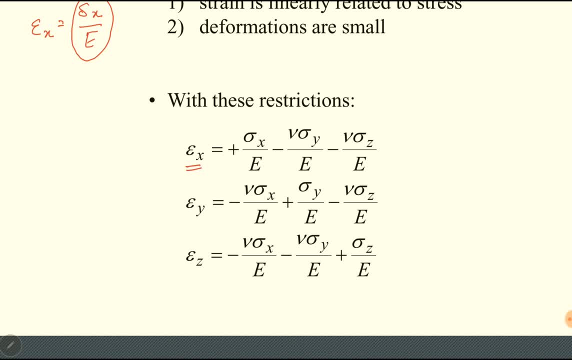 the x direction is due to three components of loads or three, three components of stress. due to the stress in x direction, it is sigma x to whatever e, minus due to the strain in y direction. so it will be a multiple of poisons ratio, which has been defined in the previous topic, minus the 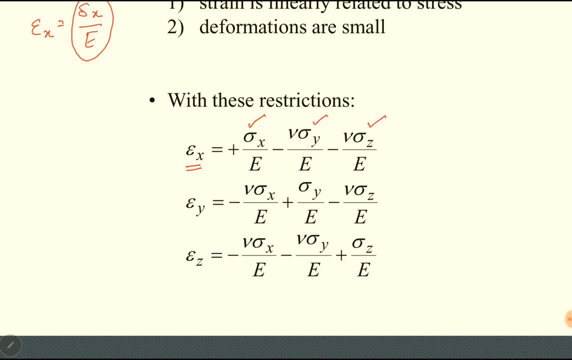 strain due to Z stress. stress in the Z direction it will again will be multiplied with the poisons ratio. so the negative sign means this deformation. deformation will be in the opposite direction. ok, so Similarly, strain in Y is because of the stress in Y direction, minus the stress in X direction, minus the stress in Z direction. 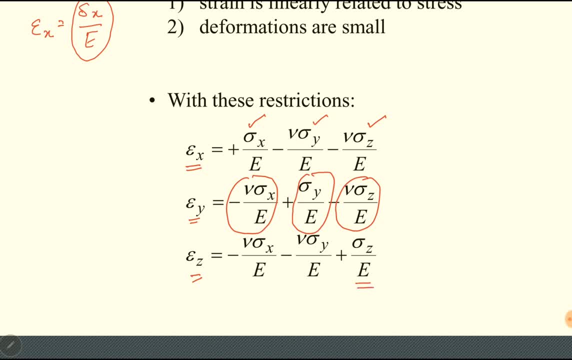 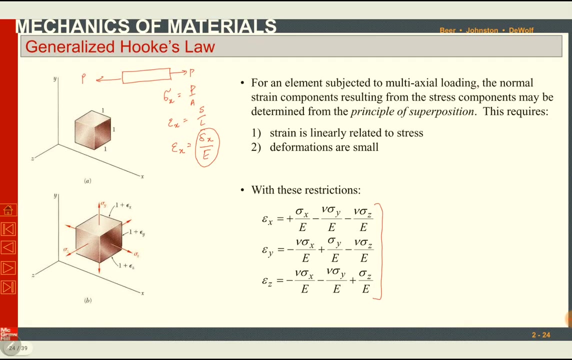 Similarly, strain in Z direction is due to stress in Z direction minus the stress in Y direction, minus the stress in X direction. So these three expressions are actually Hooke's law in three dimensions. It is called generalized Hooke's law. So now, from now onwards, if we want to calculate components of strain in the three dimensions, or one of the three dimensions, X, Y and Z, 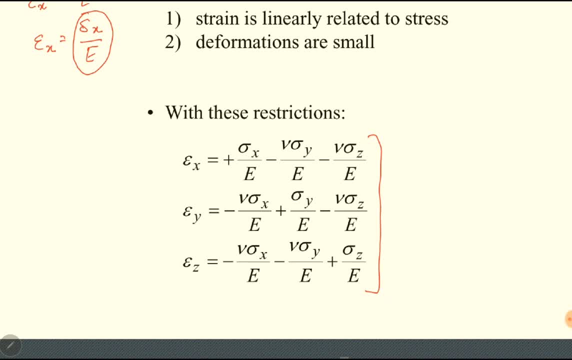 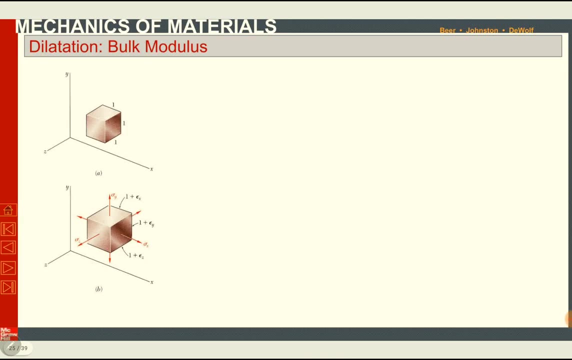 we need to use Poisson's ratio and the three-dimensional stresses- normal stresses, sigma X, sigma Y and sigma Z- to calculate each component of the strain. We will use it in our next topic, which is dilatation or bulk modulus. 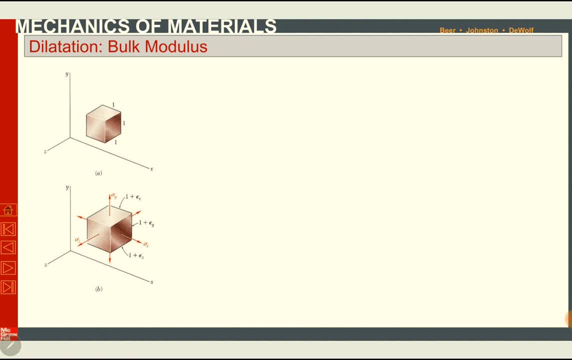 Again, bulk modulus is another. It is a very important concept, Bulk modulus or dilatation. Dilatation is actually resistance against volumetric change, resistance against volumetric strain, Just like the Young's modulus or modulus of elasticity is resistance against normal strain. 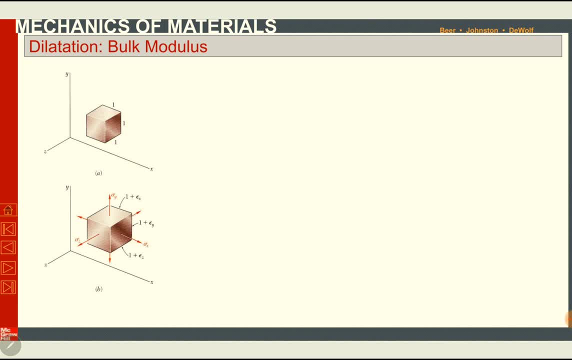 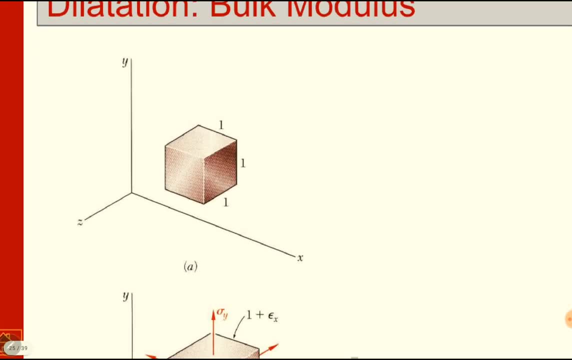 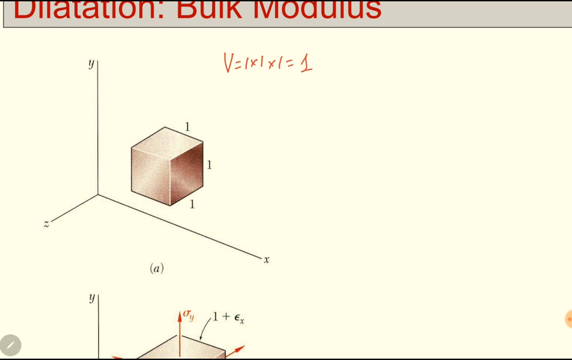 So, similarly, dilatation is resistance against volumetric strain When we are making a decrease in volume but change in volume. here we will have a cube with the sides Each, with each side having unit length one. The net volume will be one into one into one. 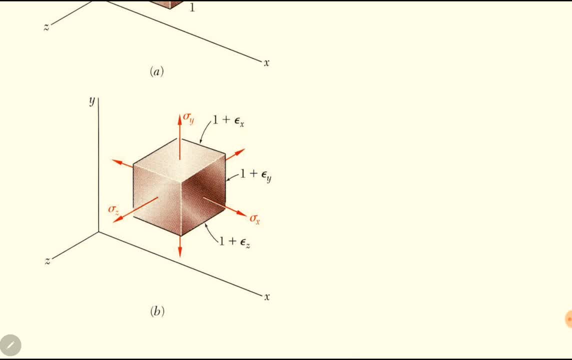 Which is one again: unit volume. OK, After applying stresses in the three directions- Sigma X, Sigma Y and Sigma Z- The change in volume are the net volume. The change in volume are the net volume In the Museum. the length of the new sides will be 1 plus epsilon x, 1 plus epsilon y and 1 plus epsilon z. 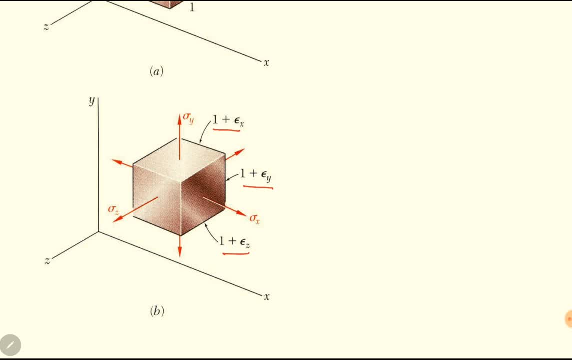 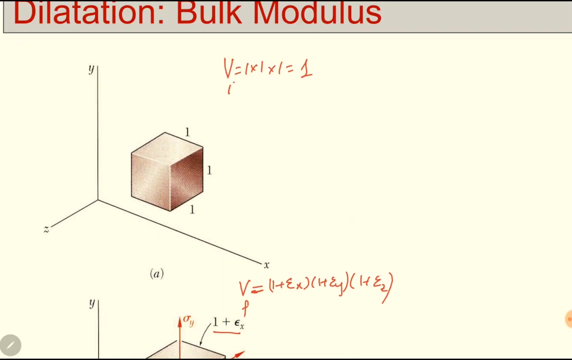 epsilon x, epsilon y and epsilon z are the change in length. ok, so the new volume in this case is 1 plus epsilon x multiplied by 1, plus epsilon y, multiplied by 1 plus epsilon z. so the final volume minus initial volume is the change in volume. 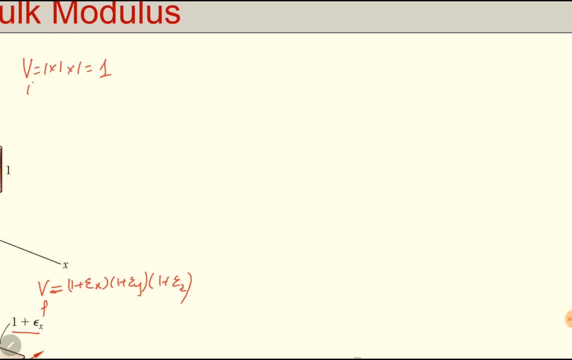 ok, the change in volume is equal to the final volume minus the initial volume. so, after simplifying this expression by multiplying the different terms, some terms will have product of different strains, because epsilon x, epsilon y and epsilon z, these are very small numbers, so their products, product of two of the strains or three of the strains, will be a very, very small number. 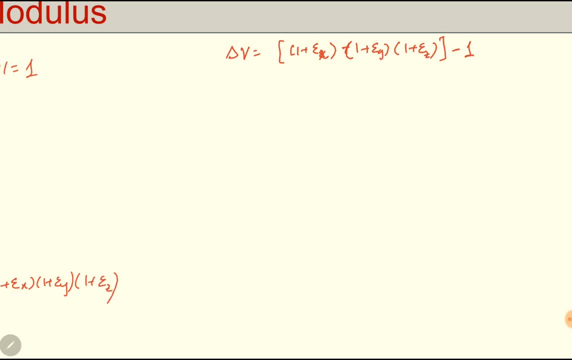 so we will neglect those terms involving product of two or three strains. so, by simplifying it, the net volume will be: I will keep only the significant terms: 1 plus epsilon x plus epsilon y plus epsilon z. I have neglected the terms involving the product of the strains. 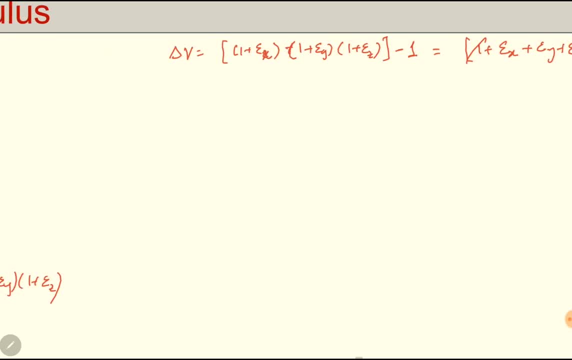 so 1 and minus 1 can be cancelled out. so net change in volume is equal to epsilon x plus epsilon y plus epsilon z. ok, this is change in volume. so dilatation which is denoted with small e: it is equal to the change in volume per unit original volume. 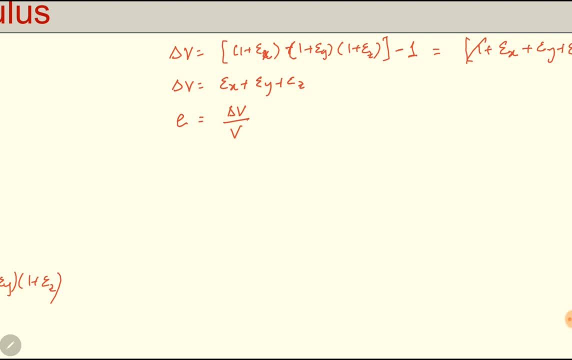 this is volumetric strain. actually, dilatation is volumetric strain and bulk modulus is resistance to the volumetric change, resistance to the change in volume. previously I stated that dilatation is the resistance to the change in volume, which is wrong. dilatation is actually change in volume per unit. original volume. 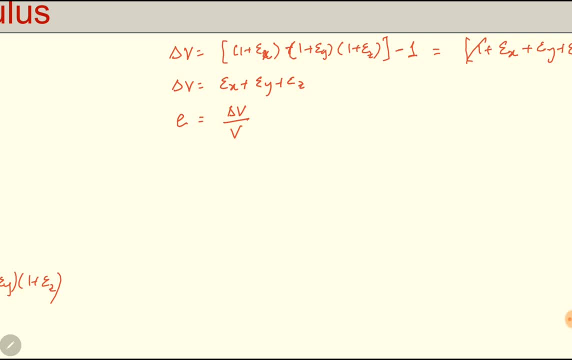 dilatation is actually volumetric strain. bulk modulus is the resistance to volumetric change, so please remember it. I have corrected my statement. bulk modulus is resistance to the volumetric strain and dilatation is actually the volumetric strain. ok, so it is equal to change in volume per unit. original volume. 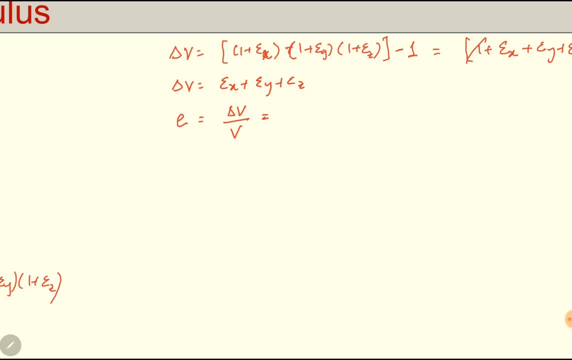 So it is equal to change in volume per unit original volume. So change in volume is here epsilon x plus epsilon y plus epsilon z And original volume, which is initial volume. it is equal to 1 in this case. So anything divided by 1 will be the same. 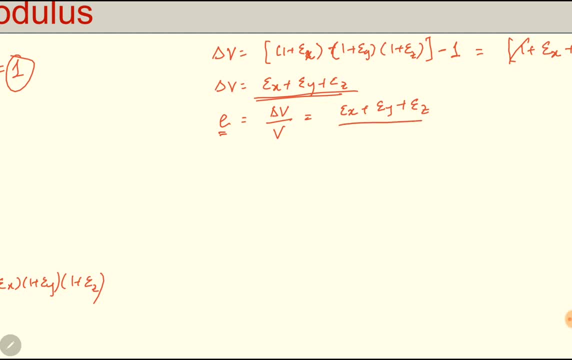 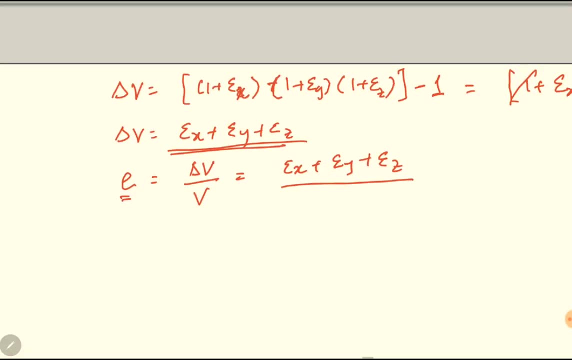 So E is equal to dilatation, is equal to epsilon x plus epsilon y plus epsilon z, Sum of the strains in the three directions. Now, if we put expressions of strains from the previous slide, from the generalized Hooke's law, 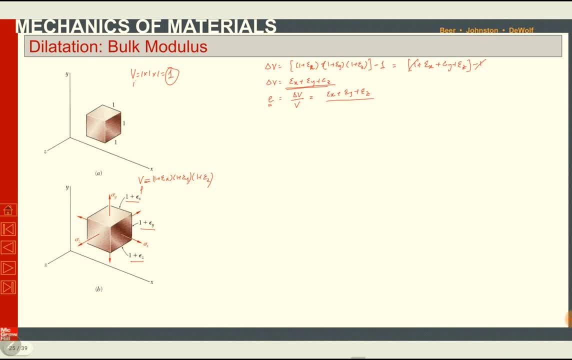 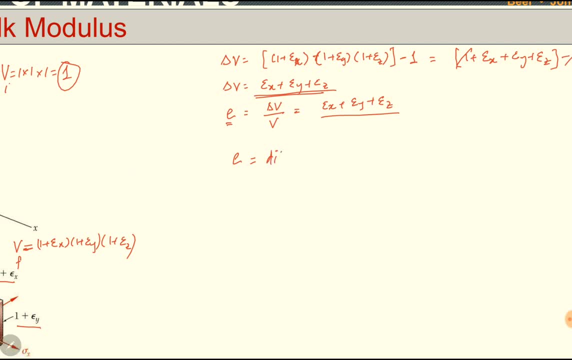 by putting the strains in terms of stresses. we can simplify this expression and dilatation, or the volumetric change, will be equal to small. e is actually. dilatation is equal to sum of the strains. And if we put the expressions of strains from the previous slide, 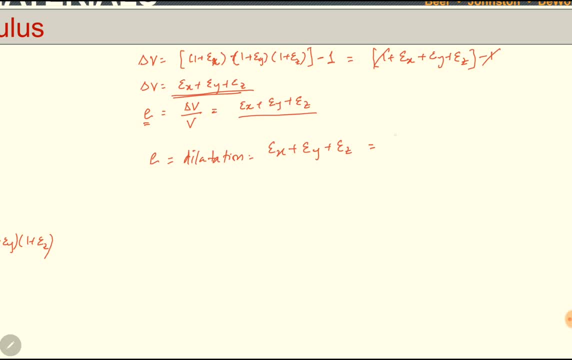 from the generalized Hooke's law, so it will be 1 minus 2 nu divided by E. I have skipped the simplification terms. You can do it or you can see it in the textbook- any of the textbooks related to mechanics of material. 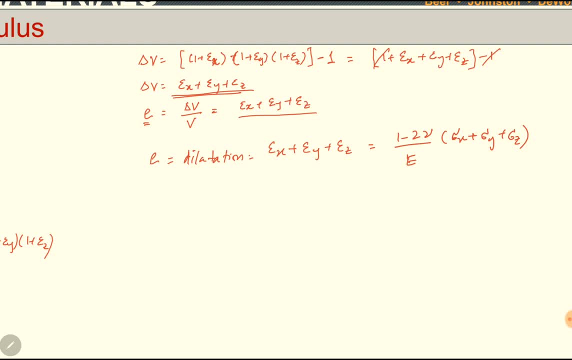 So the dilatation or the volumetric strain or the change in volume per unit original volume is actually sum of the three dimensional normal strains, are it is equal to 1 minus 2 nu. So nu divided by E, multiplied by sum of the three normal stresses. 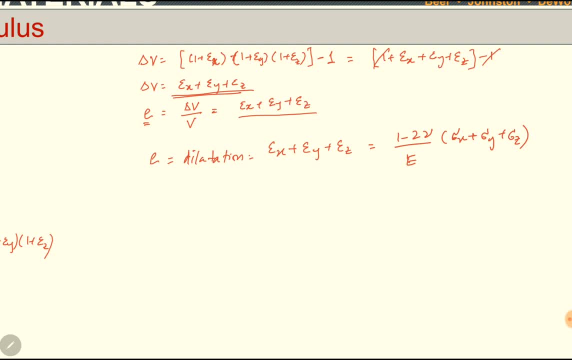 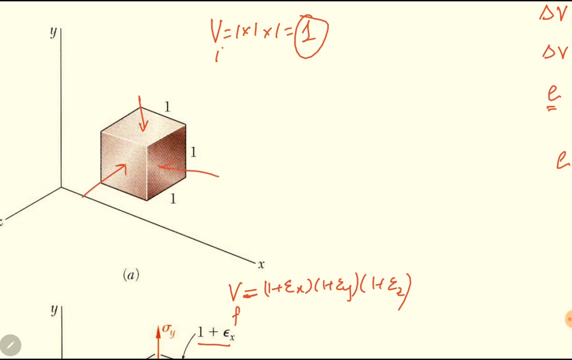 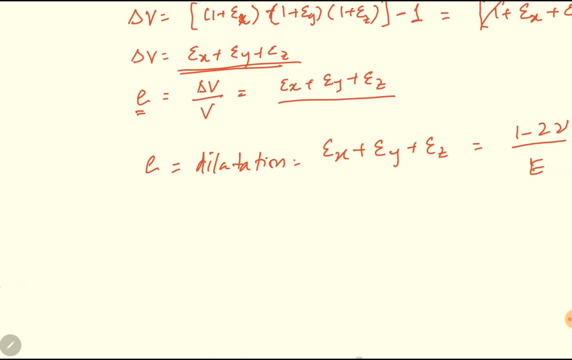 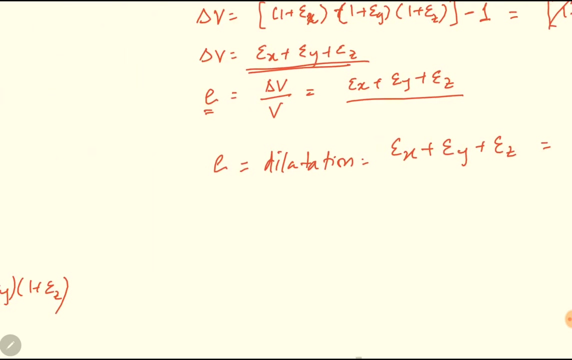 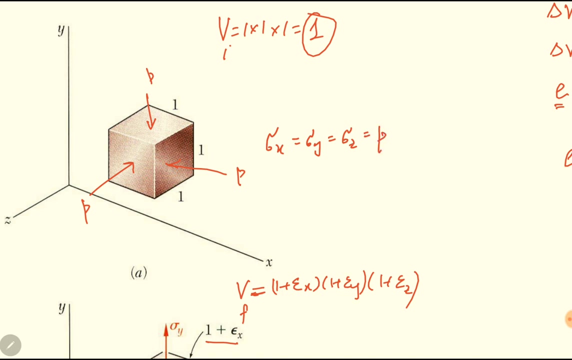 Okay, now if we assume that a body or a cube, it is under a uniform hydrostatic pressure. Uniform hydrostatic pressure means the cube is under the same amount of pressure from the three sides Hydrostatic pressure. Okay, so the stresses in the three dimensions, three directions, sigma x, sigma y and sigma z in this case, are all equal to the pressure. 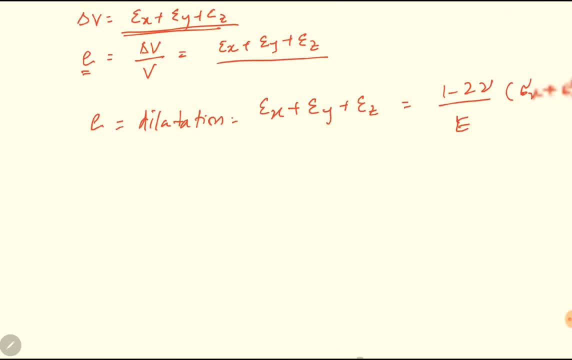 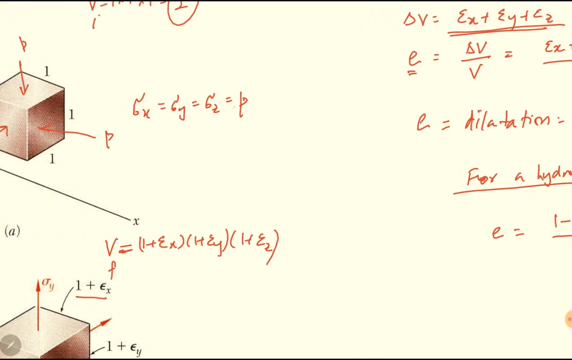 So I want to use this specific case for a hydrostatic pressure case. Okay, for this case the dilatation is equal to 1 minus 2 nu divided by E into sum of the three. sorry, this is minus P, because hydrostatic pressure is compressive. 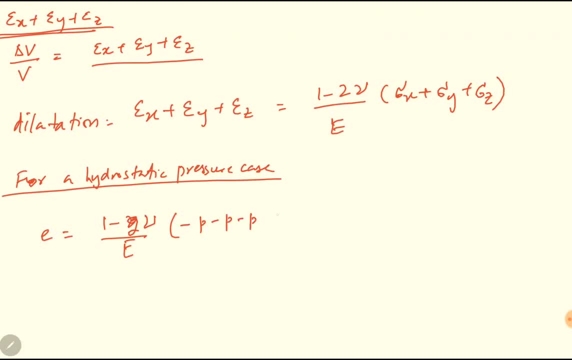 So minus P, minus P, minus P. So it becomes minus 3P into 1 minus 2 nu over E. I can further simplify it as minus P divided by E over 3 into 1 minus 2 nu. 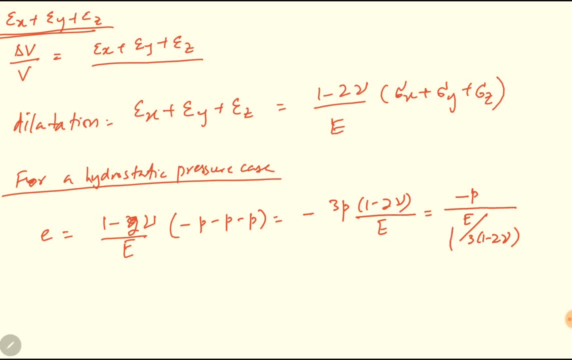 Okay, so this term E. Okay, so this term E. E divided by 3 into 1 minus 2 nu. this is actually a constant. All the terms are constant, so I can replace it with constant K. This K is actually equal to E divided by 3 into 1 minus 2 nu. 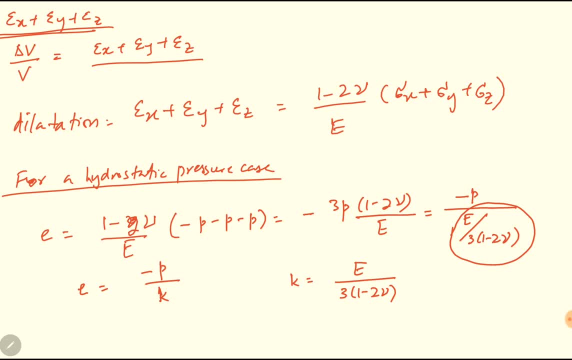 This K is bulk modulus. This is bulk modulus and this bulk modulus is actually inversely proportional to dilatation E. The lower the bulk modulus, the higher will be dilatation. So bulk modulus is a material property. If a material has lower bulk modulus, it will experience more dilatation, more volumetric strength under pressure. 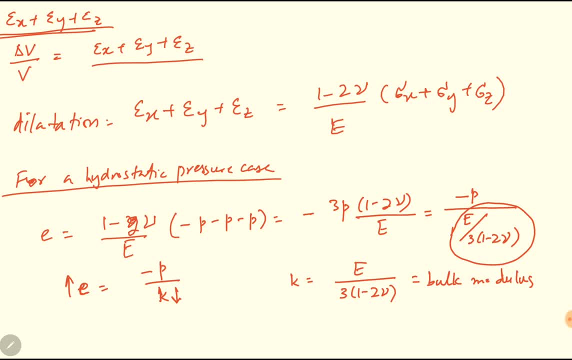 And if a material has higher bulk modulus it will have lower volumetric strength. It will experience lower volumetric strength against the same amount of pressure. So it is actually a resistance to volumetric strain or dilatation or change in volume. 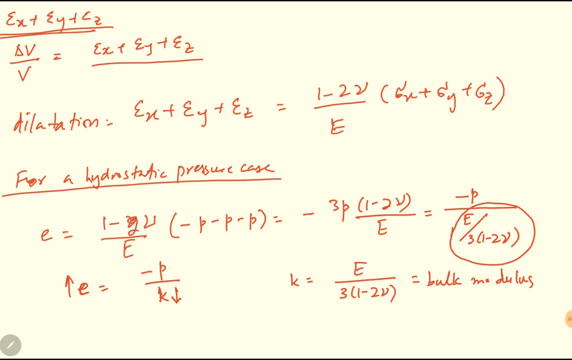 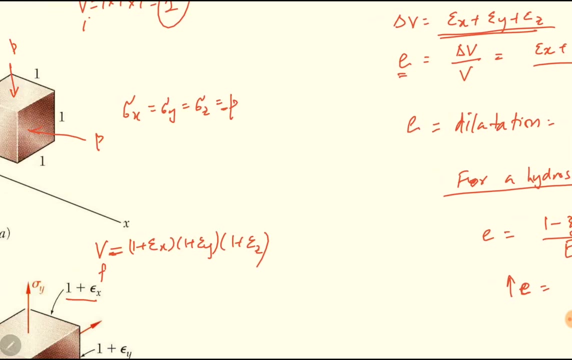 Bulk modulus is a resistance to change in volume or dilatation. Okay, in this case we have derived this expression of bulk modulus for a compressive stress or compressive pressure case. In case of compressive pressure, the dilatation must be negative. 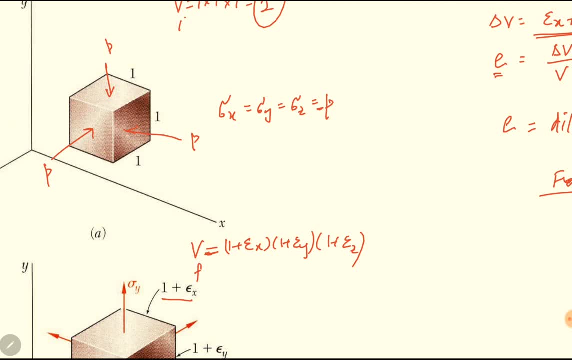 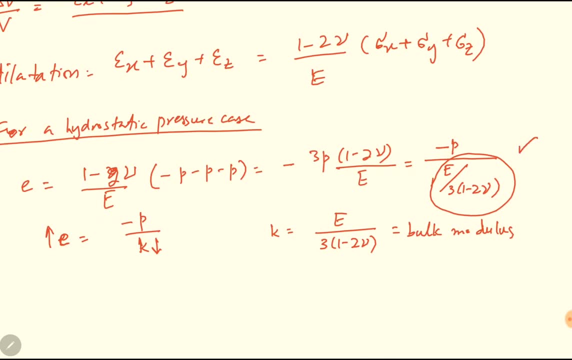 The change in volume must be negative. It means this expression for E: it must yield a negative number. Here is a negative sign with the pressure It means the value of K, This E divided by 3, into 1 minus 2 nu. 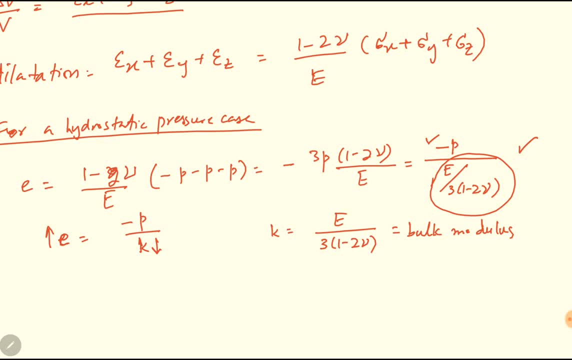 1 minus nu must be a positive number, so that the net value of E is negative. So for K to be positive, it is equal to E over 3 into 1 minus 2 nu. This ratio should be a positive number. 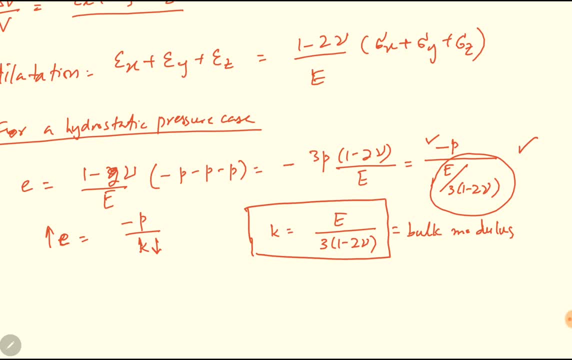 If this is a positive number, E is already positive. It means 1 minus 2. nu should be positive. Okay, if this should be positive, it means nu should be greater than, or 2, nu should be less than 1.. Or you can say nu should be less than 1 by 2.. 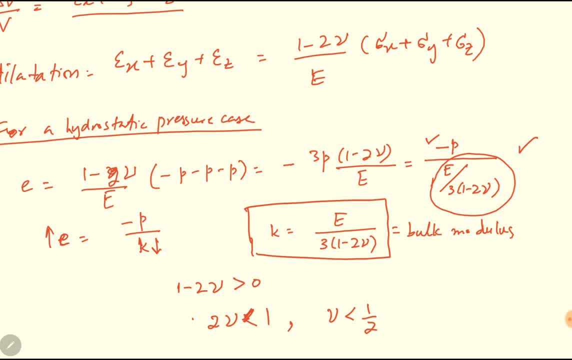 So Poisson's ratio should be less than 1 by 2.. It cannot be greater than for any material. This is a derived fact That Poisson's ratio cannot be 1 by 2 or 0.5.. The value of Poisson's ratio will always be less than 0.5.. 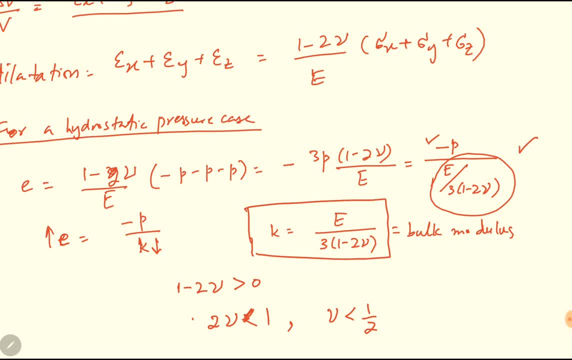 It has no unit because it is a ratio between two similar quantities, between two strains, And it can also be not less than 0. Remember that Poisson's ratio cannot be less than 0. It cannot be a negative number. Previously I have told you that. 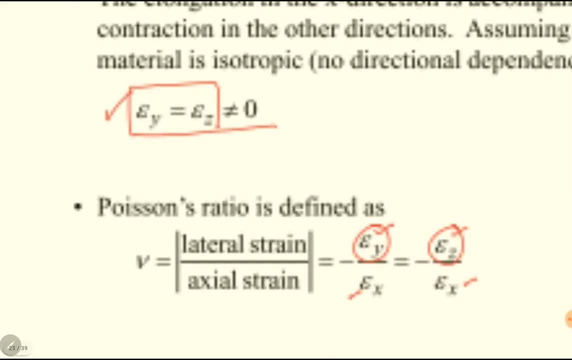 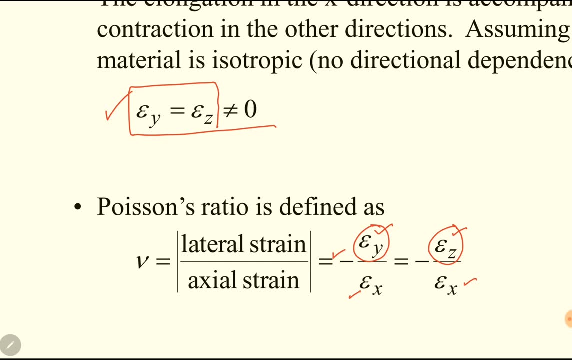 Poisson's ratio must be a positive number. We have intentionally kept a negative sign in the expression, this negative sign, so that the ratio of two strains, one of them, must be a compressive strain, so that the ratio becomes positive. So Poisson's ratio cannot be a negative number. 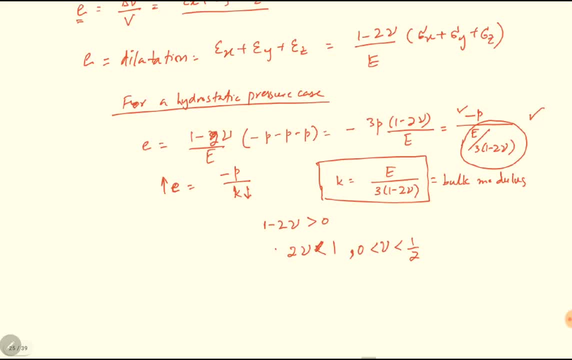 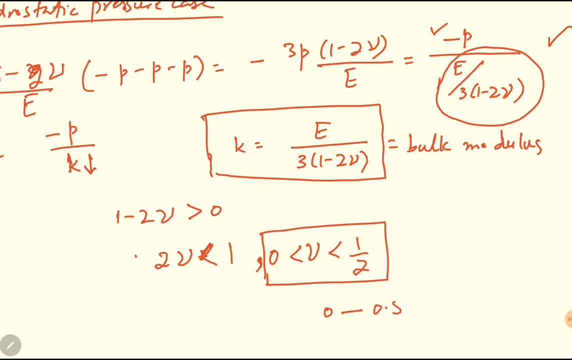 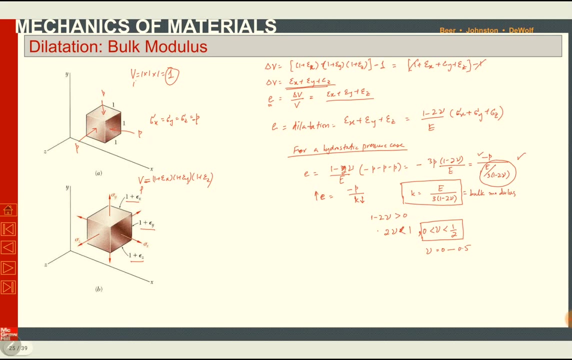 So it should be greater than 0.. It should be less than 0.5.. So Poisson's ratio is something between 0 to 0.5.. It is different for different materials, So we have studied about Poisson's ratio. 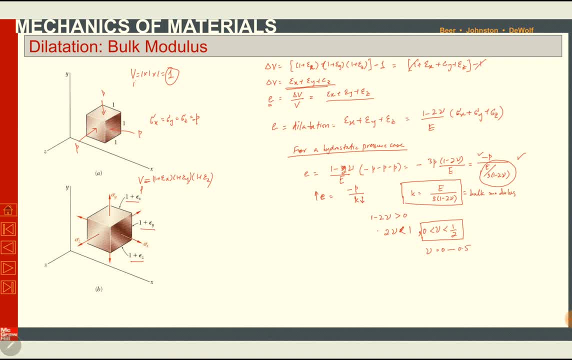 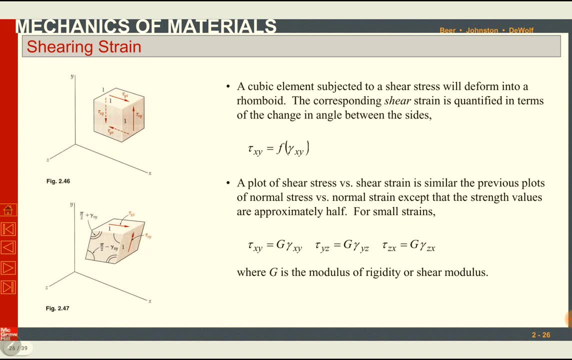 And then bulk modulus. these two are two important constants which will be used in the subject of mechanics of material. Bulk modulus can also be used in fluid mechanics, in your concept of fluid mechanics. Okay, So again, our next topic is shearing strain. 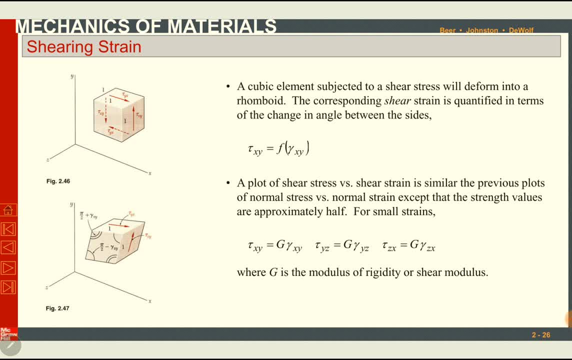 Previously we have discussed about normal strain. Normal strain is actually change in length. either tension or compression, increase in length or decrease in length. So what is shear strain? Shear strain is actually change in shape. The angles of the sides are changed. 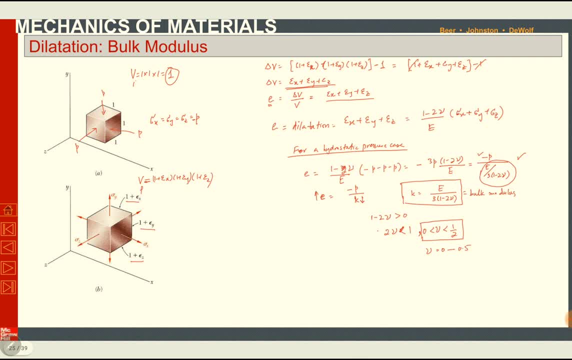 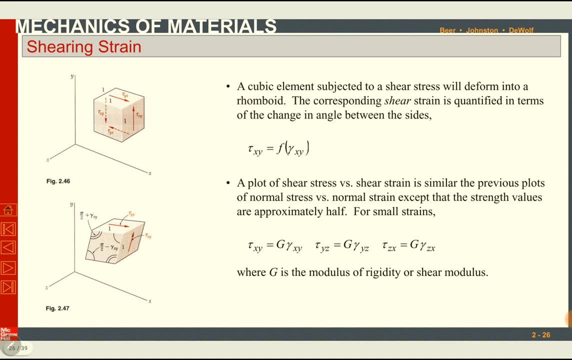 In case of normal strain, the lengths of the sides of a cube are increased or decreased, But in case of shearing strain the angles are changed, So cubic elements subjected to a shear stress will deform into a rhomboid And the corresponding shear strain is quantified. 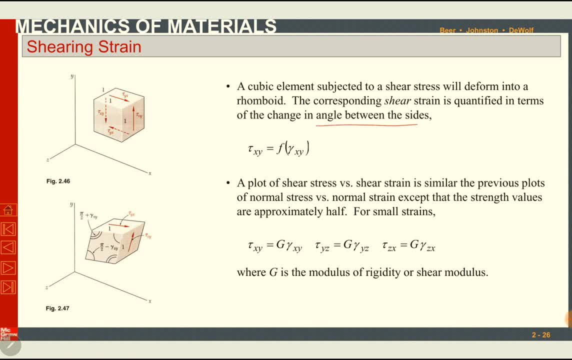 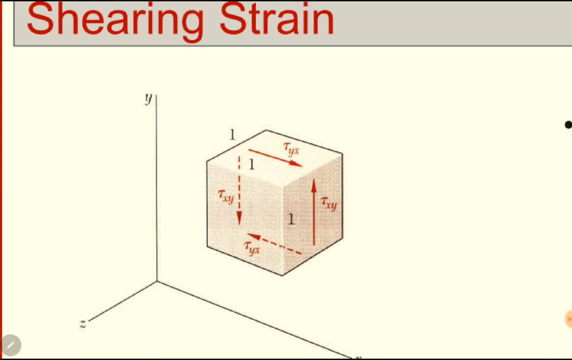 in terms of the change in angle between the two sides. So shear strain usually have a unit of radiance because it is change in angle. So here you can see, shear strains have been applied. shear forces have been applied on the sides of a cube. 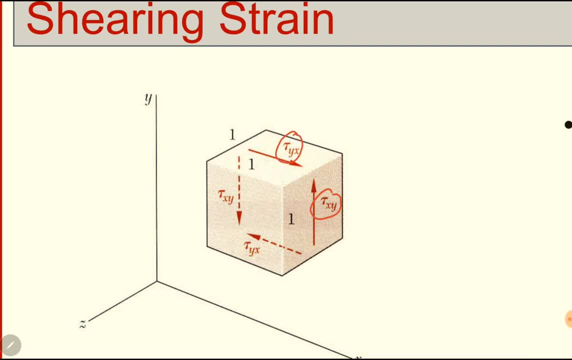 You can see tau and tau. They are both same in magnitude. Directions are different. Here is tau and tau, So these two forces will just change the angle of this edge. Similarly, these two forces will change the angle of this edge. 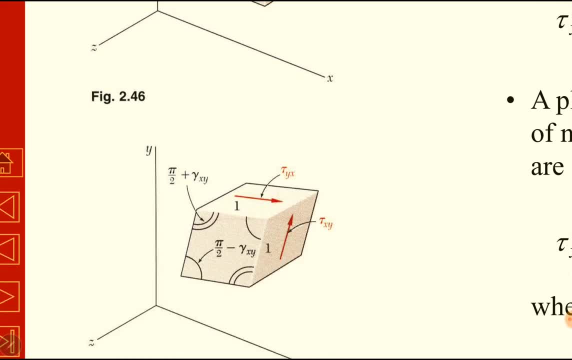 So you can see change in angle at the edges, The adjacent sides. So at the two sides the angles will increase. At the two edges the angles will increase and the other two edges angles will decrease. So you can see, initially all angles were. 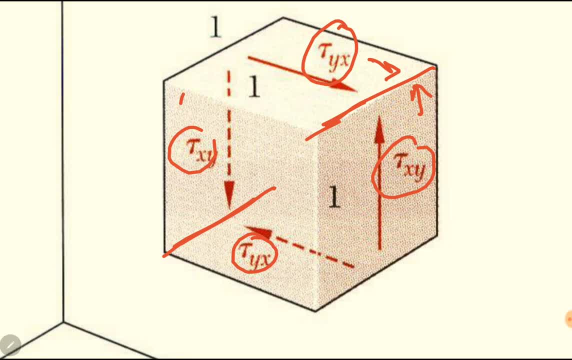 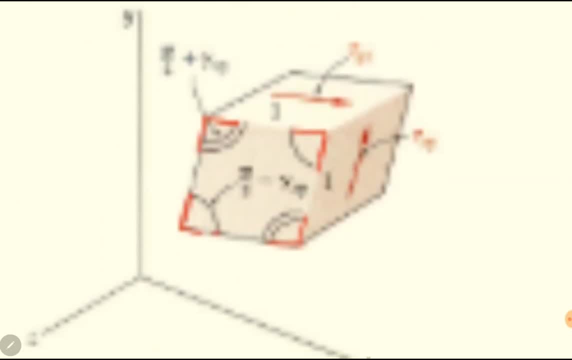 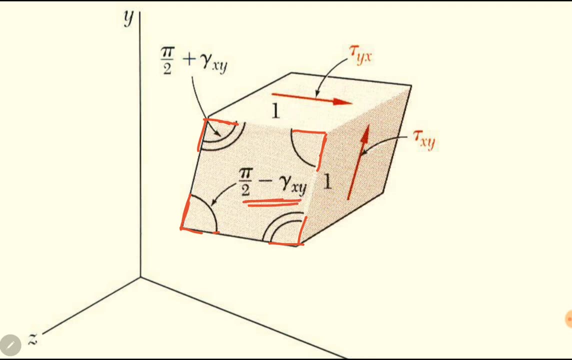 in this cube all the angles were 90 degree Angles between adjacent sides, But now you can see two of them are 90 minus specific number gamma And two of them are 90 plus gamma. This gamma xy is actually shear strain. 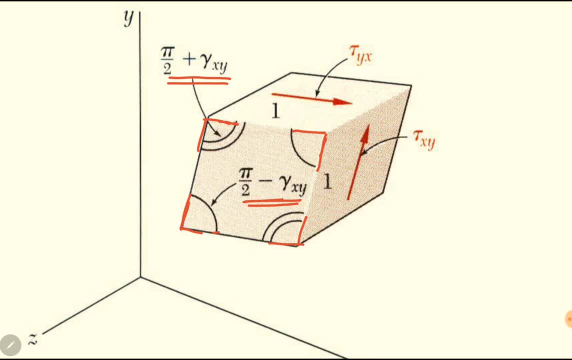 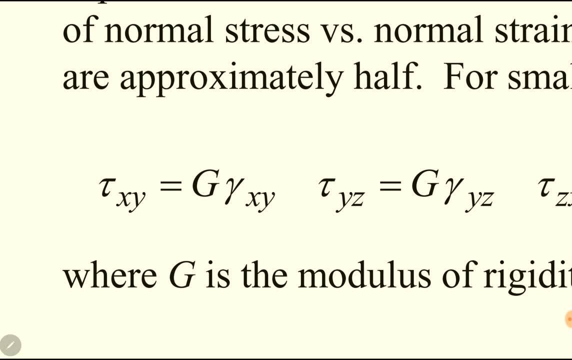 It will be measured in radiance, So shear strain gamma. it can be written in this form, using Hooke's law. like previously we have used Hooke's law, which is equal to, which is written as normal stress is equal to e into normal strain. 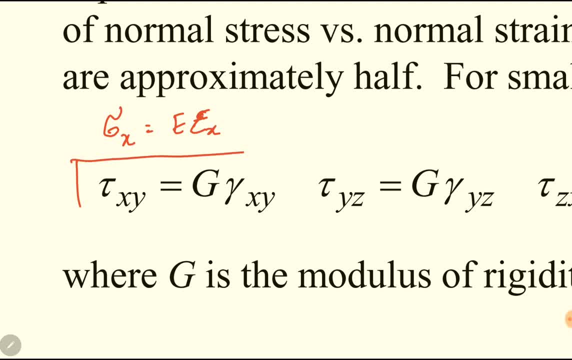 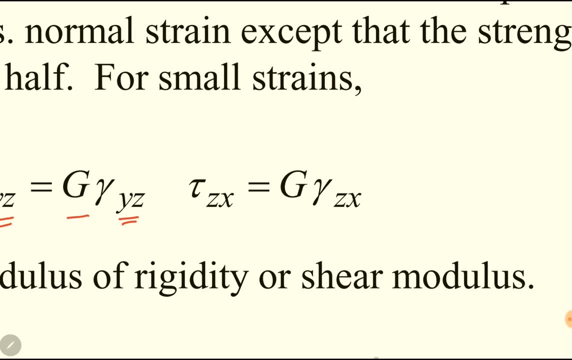 So, in terms of shear stress and shear strain, Hooke's law can be written as: shear stress is equal to g, which is modulus of rigidity, into shear strain in the xy direction. Similarly, shear strain in the yz direction is equal to g into shear strain in the yz direction. 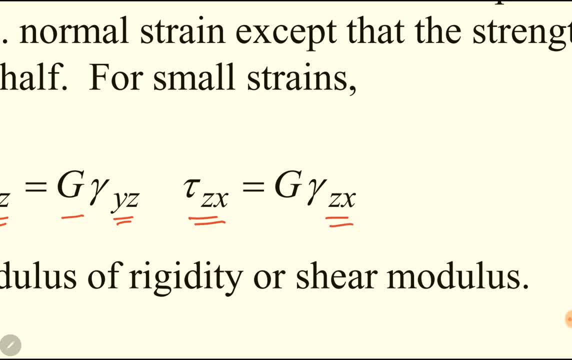 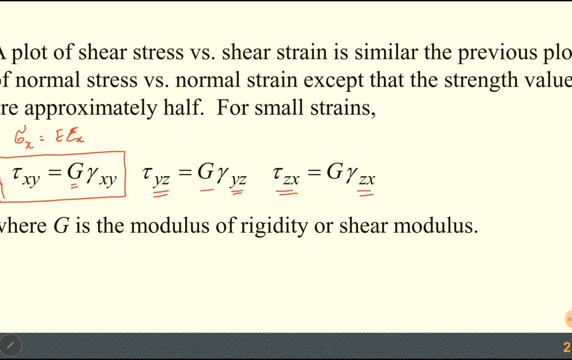 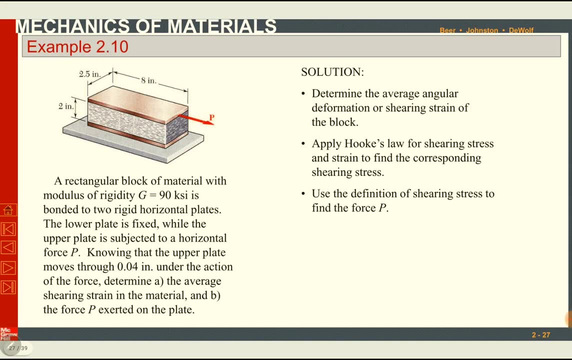 Shear stress in the zx direction is g. shear strain in zx direction, g is modulus of rigidity and it is resistance to the shear strain, Resistance to the change in angles. Here is an example problem upon the topic of shear strain and shear stress. 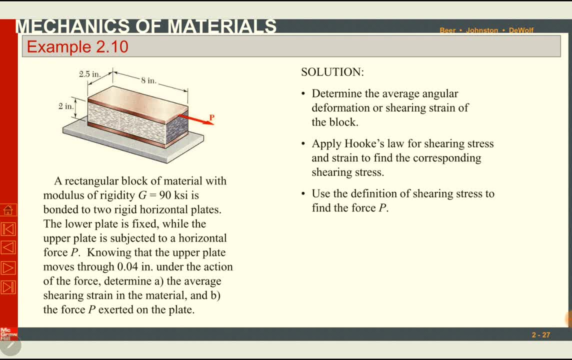 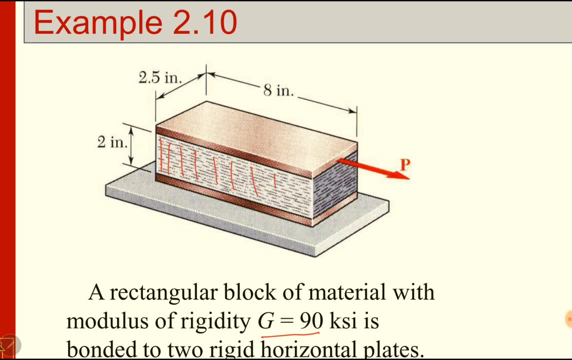 A rectangular block of material with modulus of rigidity g equal to 90 kilo pounds per square inch, ksi is bonded to two rigid horizontal plates. Here you can see a rectangular box. this one the shaded portion in between a top and a bottom plate. rigid plates. 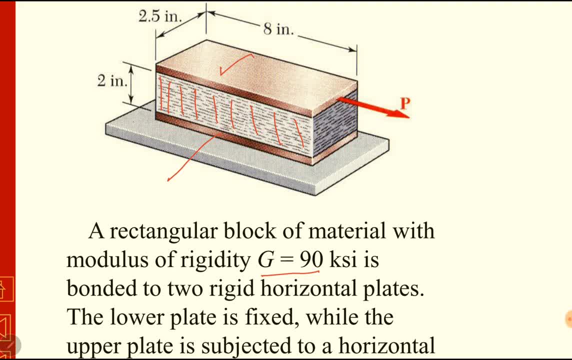 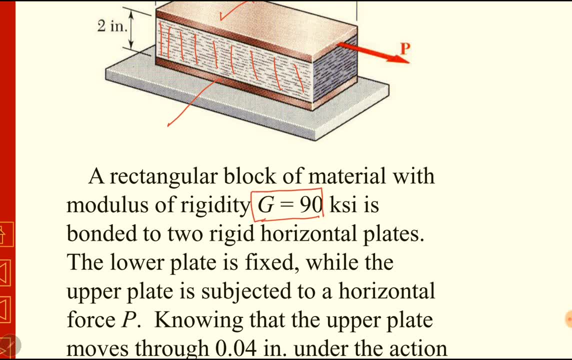 so the top and bottom plate, they are rigid. there will be no change in the shape or change in the length. but the rectangular block has a modulus of rigidity, so it means it can be deformed. it has a modulus of rigidity. rigid materials have infinite. 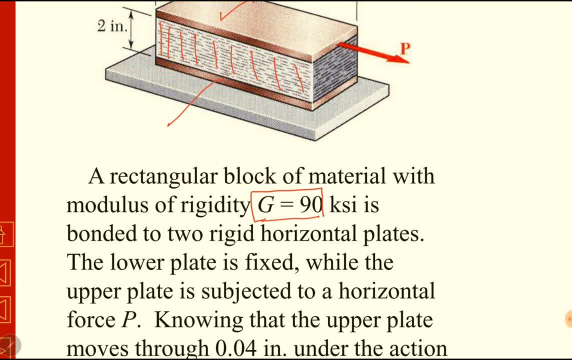 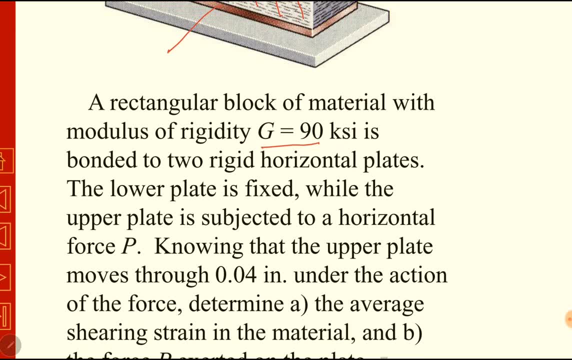 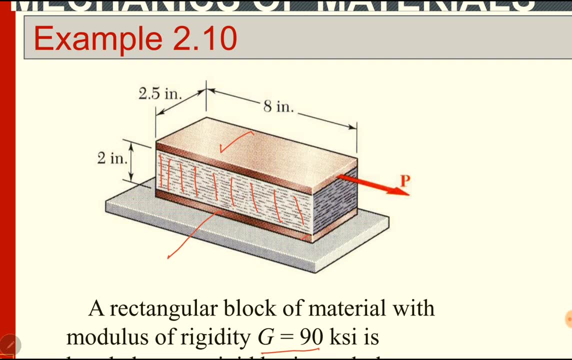 number of models of rigidity, but deformable materials have a positive number of models of rigidity. ok, the lower plate is fixed while the upper plate is subjected to a horizontal force. so this plate, the lower plate, it is fixed with the ground while the upper plate 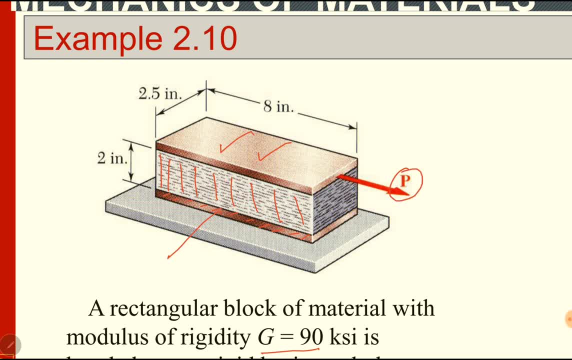 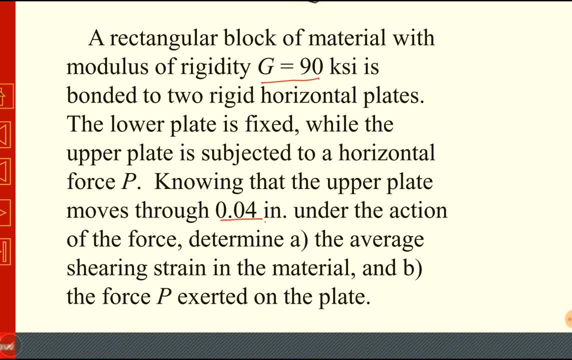 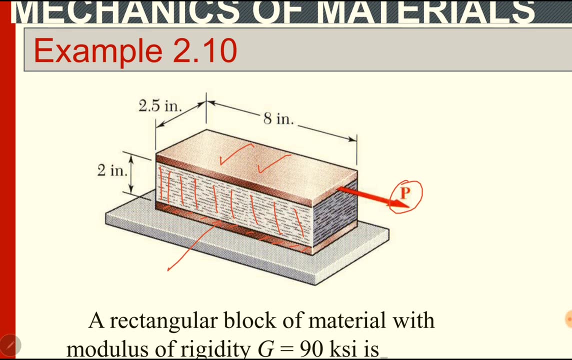 is subjected to a force p. knowing that the upper plate moves through 0.04 inches under the action of the force, determine the average shearing strain in the material and the force exerted on the plate. by applying this force p, the upper plate moves towards. 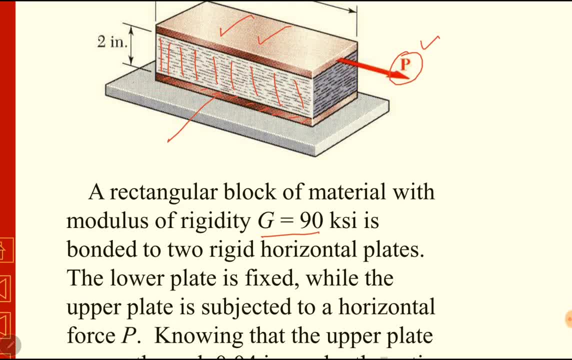 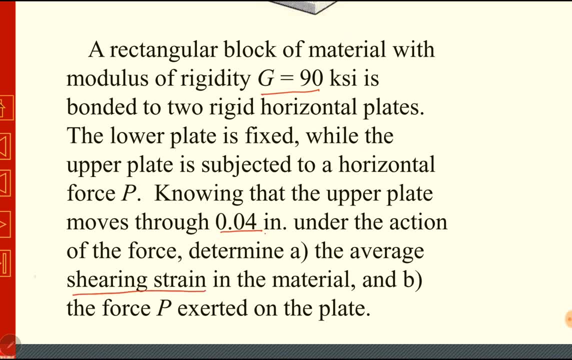 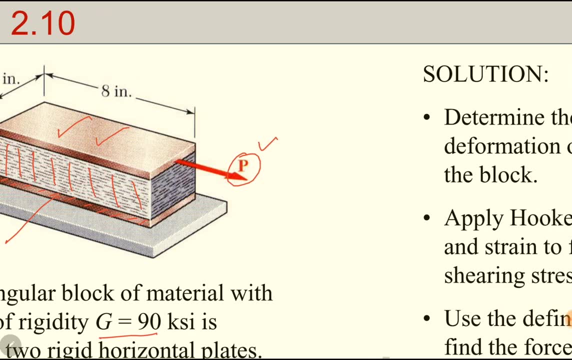 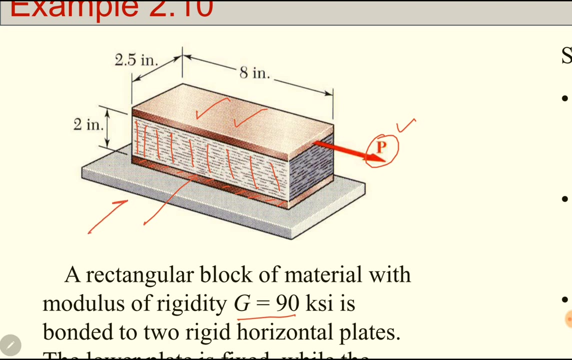 moves in the direction of the force p with a distance of 0.04 inches. we have to find the average shearing strain in the material and the force exerted, p. here I will draw a two dimensional figure by looking from this view, if this is my front view, 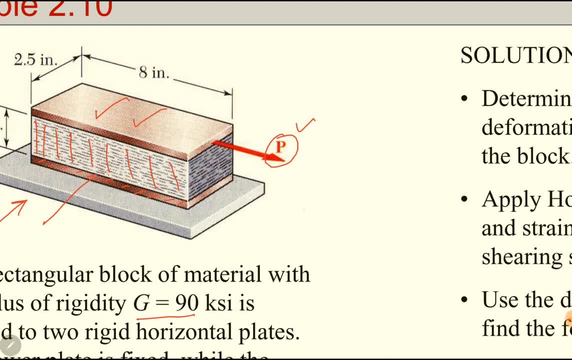 from this direction. I have to draw two dimensional figure here. here is the top plate and here is the bottom plate. the bottom plate is fixed with the ground. it will not move. ok, the top plate is attached to the rectangular block. by applying the force p, the bottom plate is fixed. 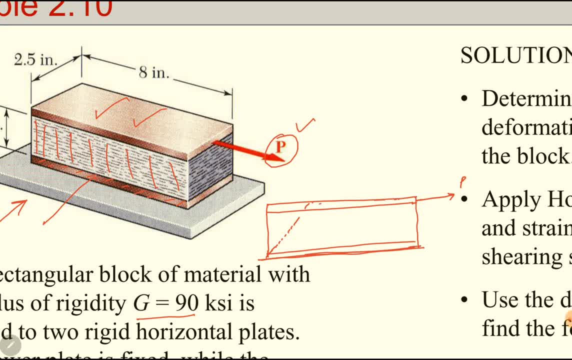 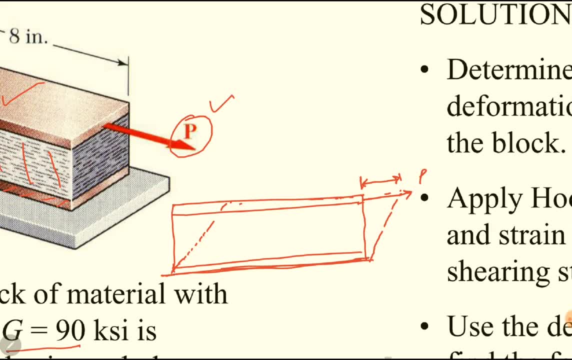 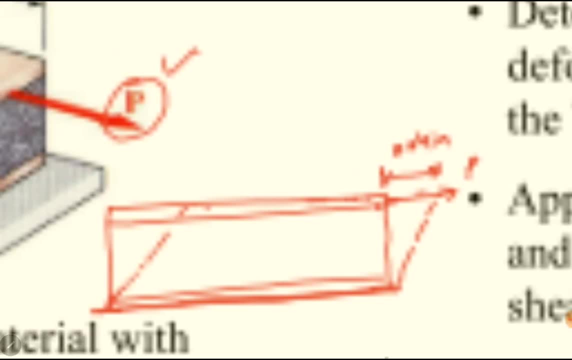 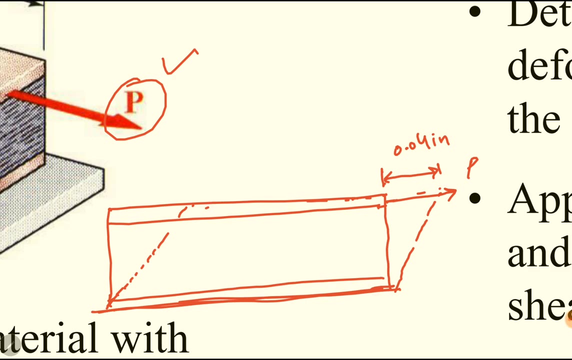 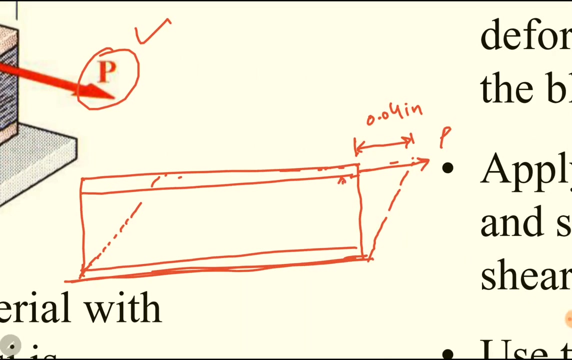 at its position, but top plate will move at its position and with a distance of 0.04 inches. ok, here we can see that a new triangle has been developed. one side of the triangle is 0.04 inch, the height is 2 inches, so you can find. 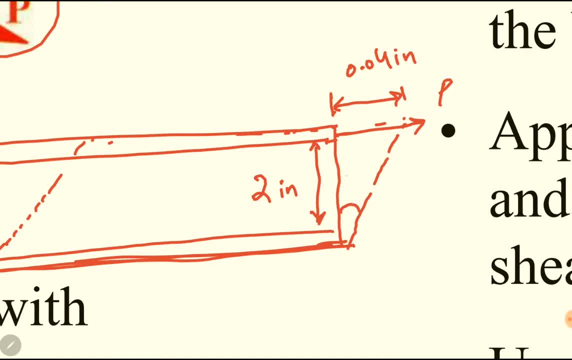 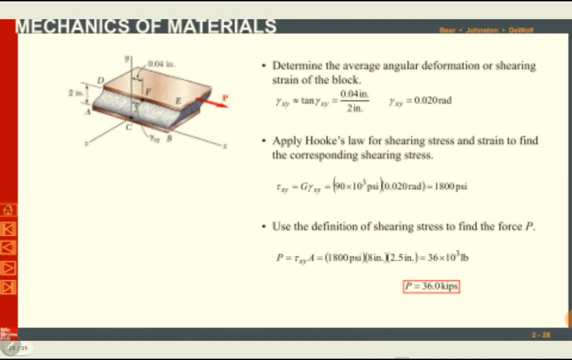 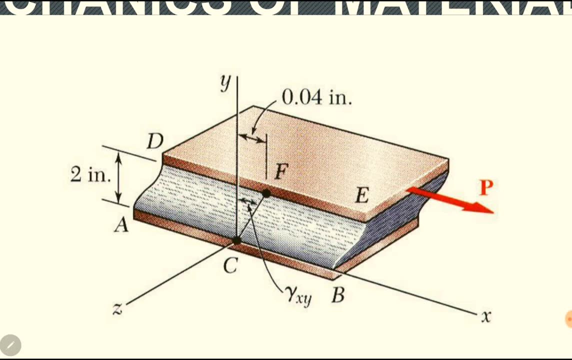 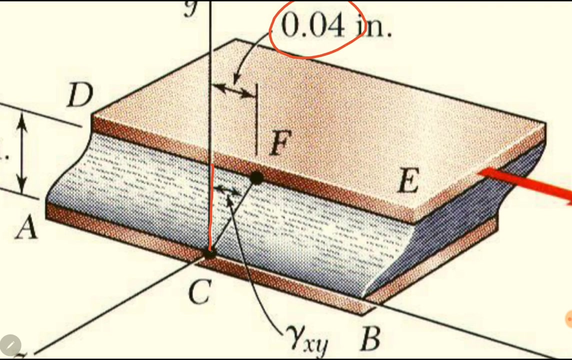 the angle. we will change an angle, this angle gamma. using trigonometry we can find angle gamma. we will find it here. it is like this: you can see: the block has deformed. the bottom plate is fixed. the upper plate has moved in the direction of the force. 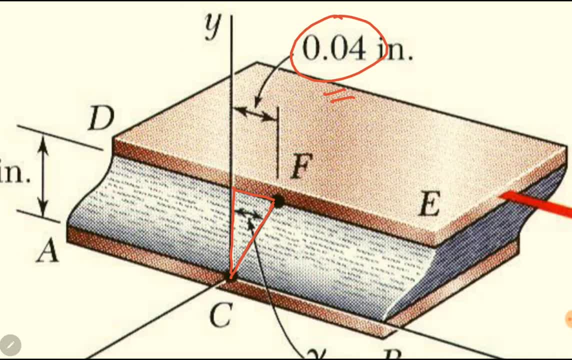 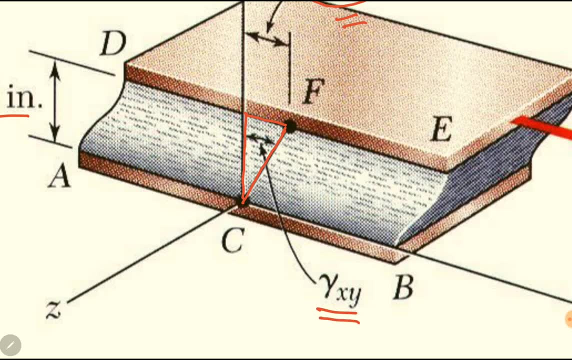 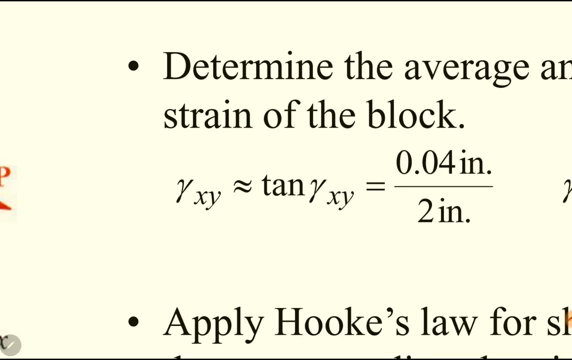 with a distance of 0.04 inch and the other one equal to 2 inches, we have to find this change in angle gamma. so, using trigonometry, gamma is almost equal to tangent of the angle. because this is a small angle, strains are usually small numbers. 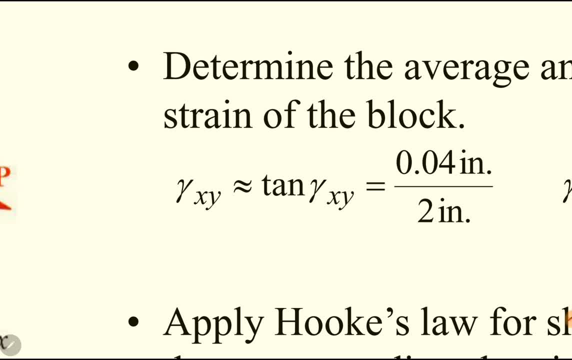 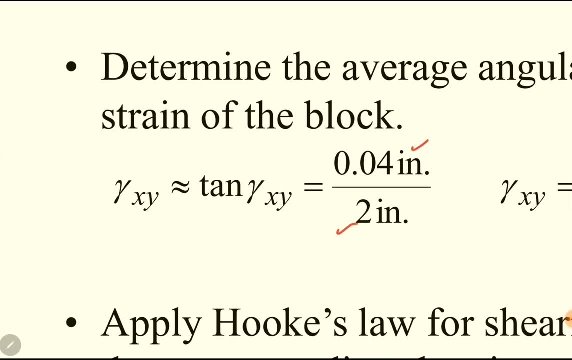 so tangent of small numbers is equal to in radians. remember that tangent of an angle is equal to the value of the angle itself in radians. so tan equal to perpendicular divided by base. in this case perpendicular is 0.04 inch and base is 2 inches. 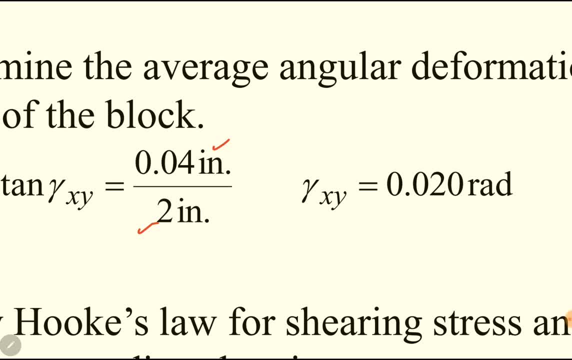 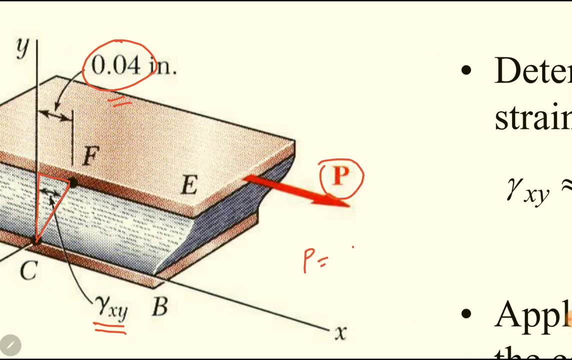 so gamma xy becomes 0.02 radians. the first part was to find volume matrix strain, sorry, the shear strain, and we have calculated it. the second part was to find load p, this force p. so force can be calculated from stress, stress into stress, into area which area? 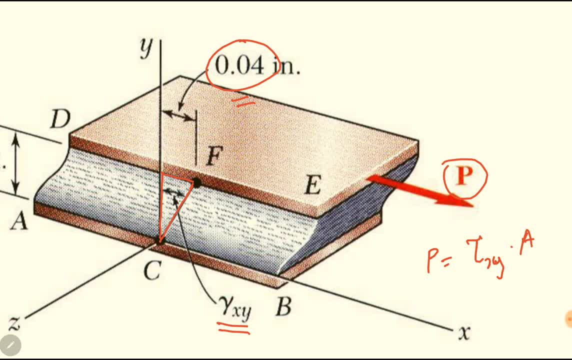 which is going to slide. this area of the plate, or the bottom of the stop plate, is attached with the block. this block, this area is attached with the block and we are applying force on the top plate. the top plate is trying to move in the direction of the force, but since it is bonded to, 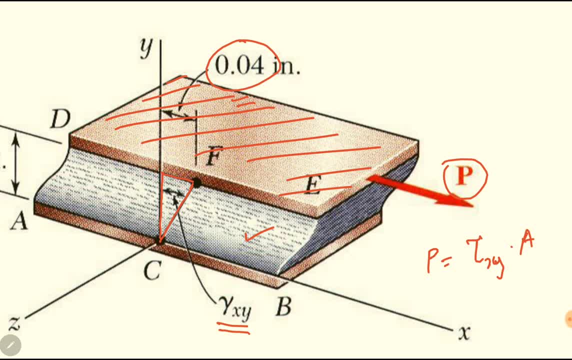 the rectangular block. so due to that bond it is trying to slide. there is a restriction and due to that restriction there will be shear strain in the common area between the top plate and the rectangular block. this area is equal to the top, the top area of the plate. 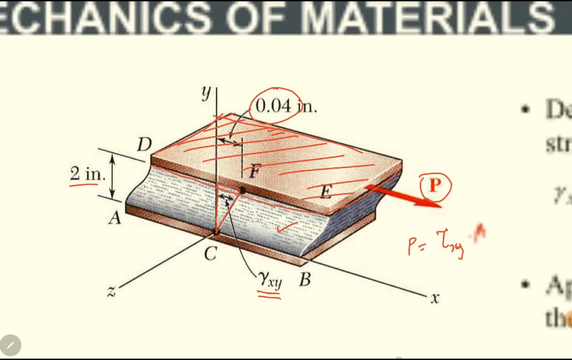 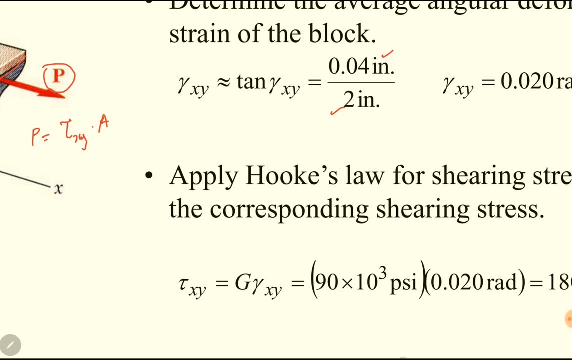 the top area is actually known to us. so we have to find stress first. stress is equal to shear. stress is equal to g into shear strain. g is given to us in the problem statement, which is 90 into 10 power, 3 psi and 90 ksi. 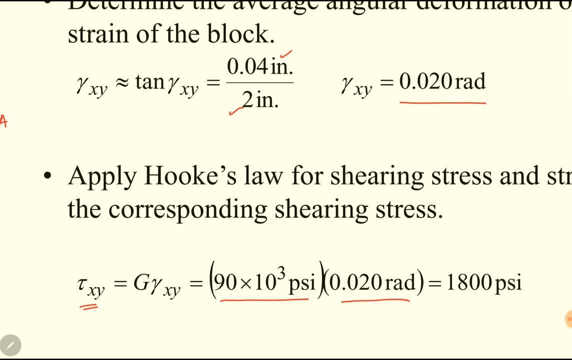 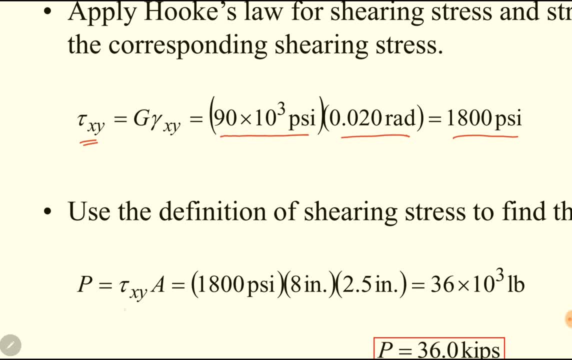 shear strain has already been calculated, which is 80 into 2 radians. so the product becomes shear stress, which is 1800 pounds per square inch. shear stress is known to us, so shear stress into area is load or force. shear stress is 1800 psi already. 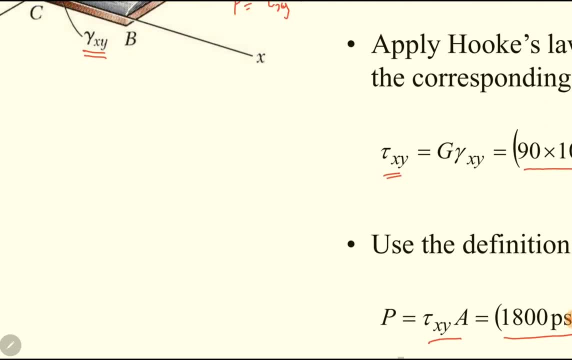 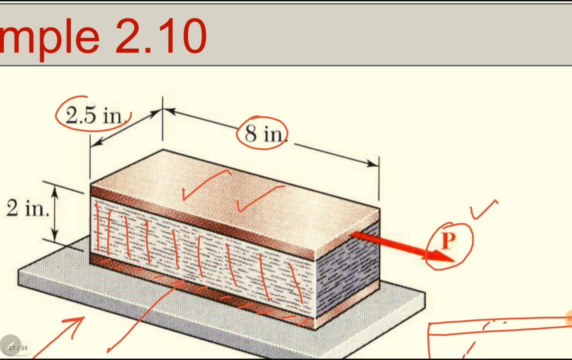 calculated area is 8 into 2.5 inches. it is given to us in the problem statement. here it is: 8 is the length and 2.5 is the width of the top of the plate, which is also a common area between the top plate and the. 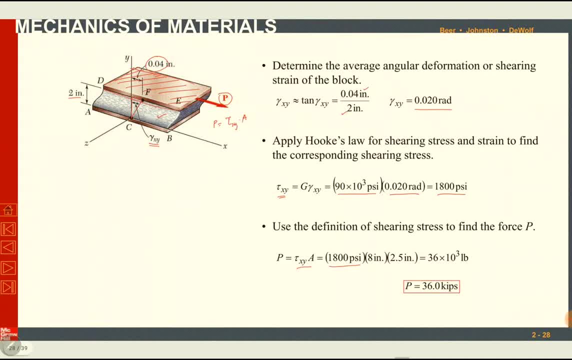 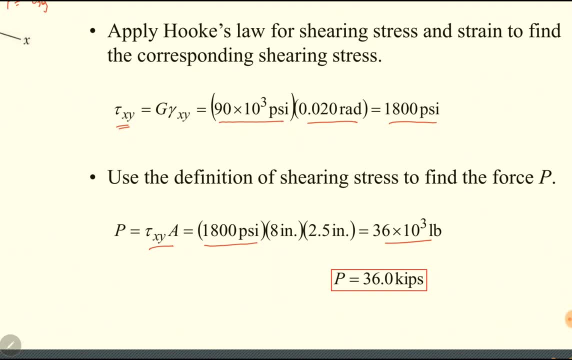 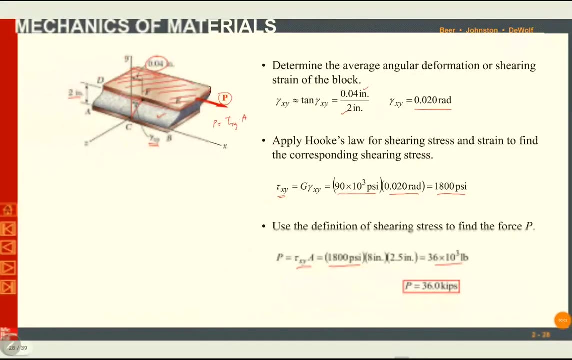 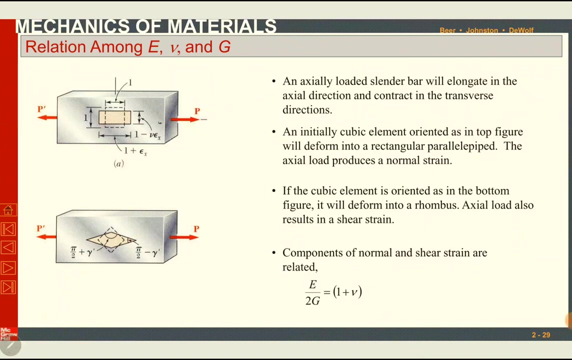 rectangular box, rectangular block. so multiplying the stress with the area, it becomes 36 into 10 power, 3 pounds, 36 kilo pounds. ok, the next topic is relation among e, nu and g. e is modulus of elasticity, nu is Poisson's ratio and g is modulus of rigidity. 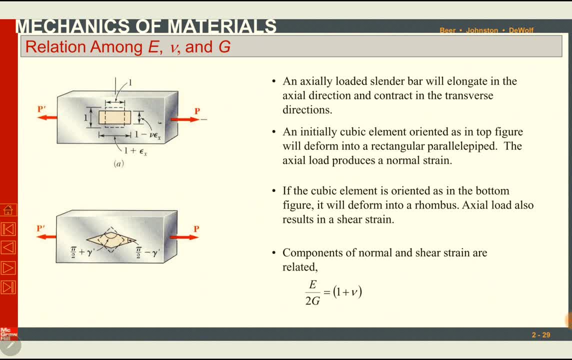 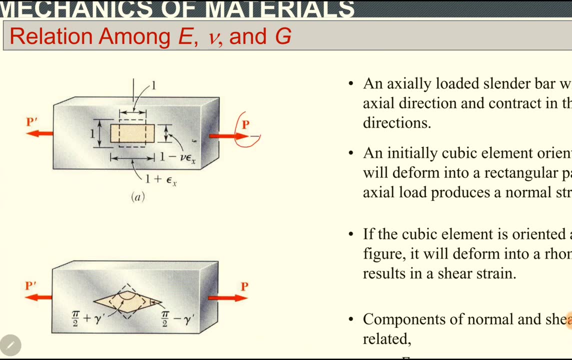 these are three different material properties and they must have a relationship with each other for same material because if we apply axial load on any material, at any bar, for example in the axial direction, there is normal strain in one of the direction, in direction of the force, in particular resist. 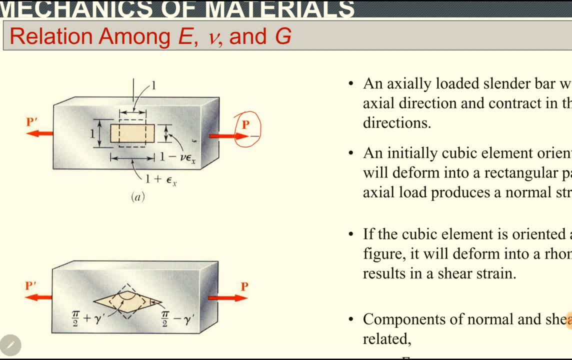 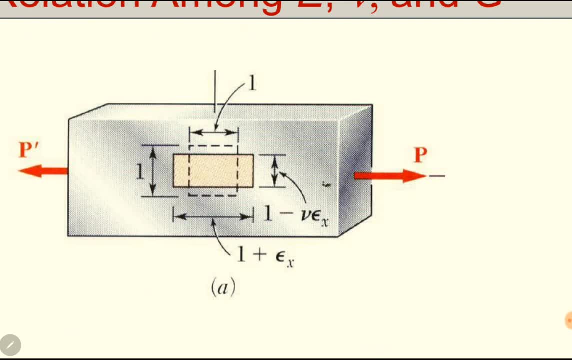 it has stiffness or modulus of elasticity in that direction specifically, but there is a strain in the other direction. you can see here: if the initial length of a marked square is 1 cross, 1 initial length of each side after applying the force in one of the direction. 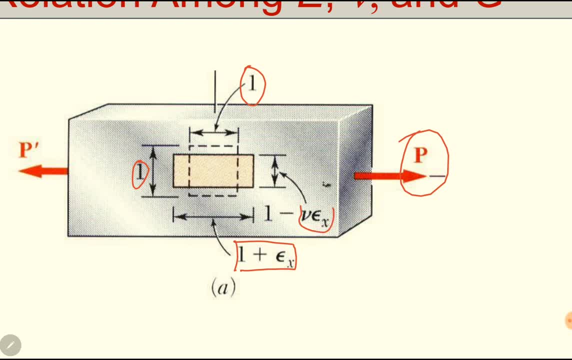 it has increased by epsilon x in the other direction. so this nu has a relationship with normal properties of the material. e is a normal property against normal stress. so modulus of elasticity has a relationship with nu. similarly, if we apply normal stress or normal force on a material, 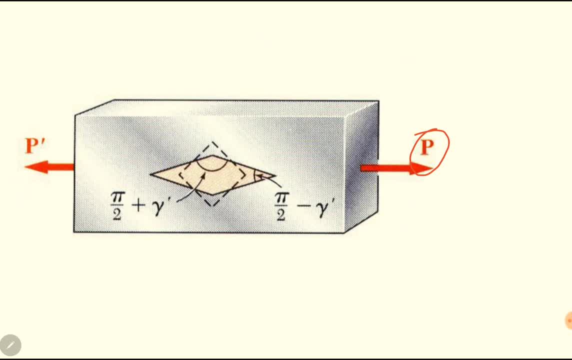 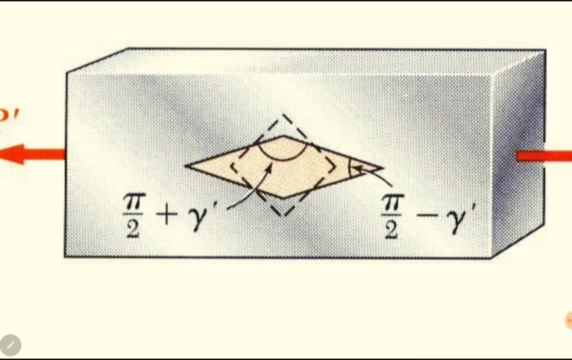 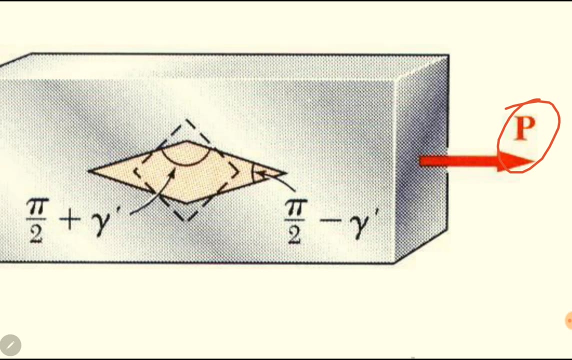 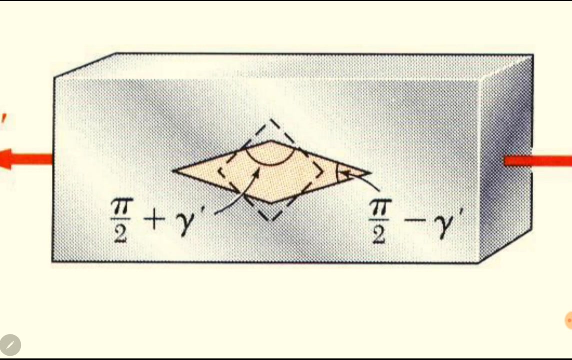 and we mark here a square with the dotted lines shown here. it is on a. it has an angle with the force p or with the direction of the force. so after applying the force you can see that the initial cubic element has been deformed into a rhombite. 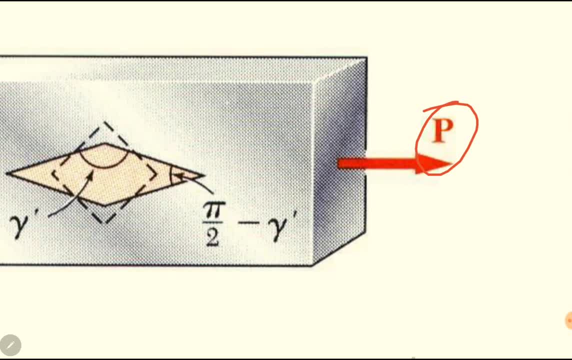 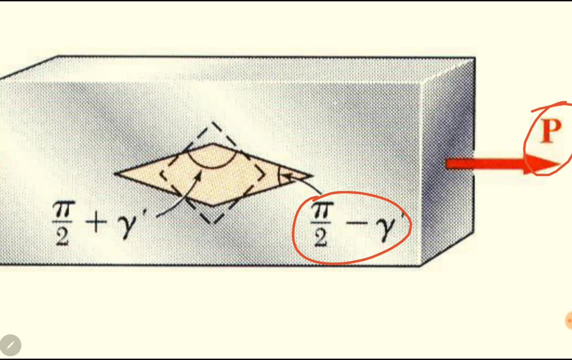 or initial square has been deformed into a parallelogram. so, due to the applied normal force, the angles have been changed, which you are going to study. what is the direction of the plane, or the angle of the plane with the applied force, if it is normal? 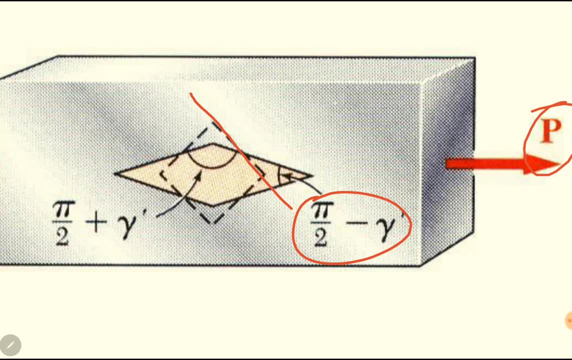 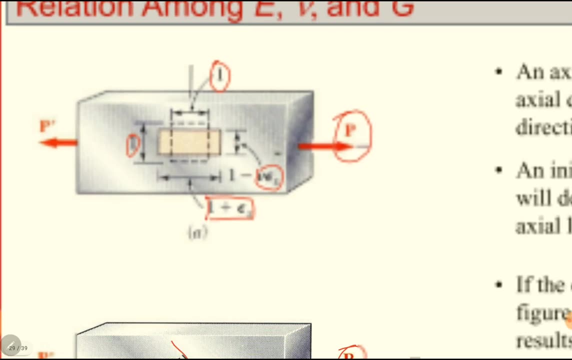 so there will be only normal deformation. if it is not a normal direction, if the angle is not 90 degree, so there will be a shear strain as well. so these normal loads may produce shear strains and similarly, due to the normal load, even the lateral strain may be produced. 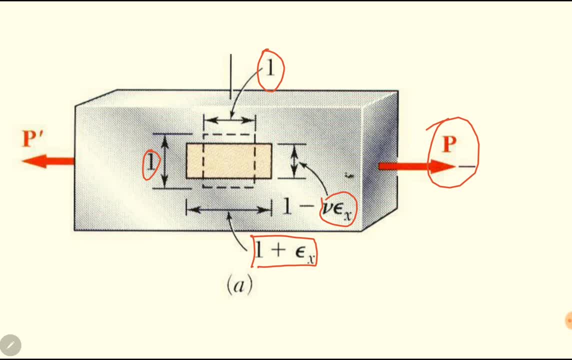 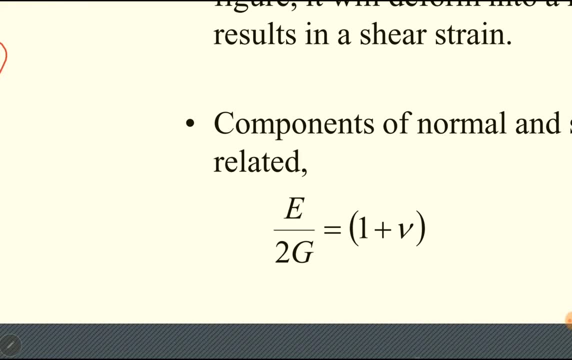 so these properties, the sharing properties, the normal properties and the Poisson ratio- they have some relationship with each other- which has been defined here. e over 2g is equal to 1 plus nu. modulus of elasticity divided by 2 times modulus of rigidity is equal to. 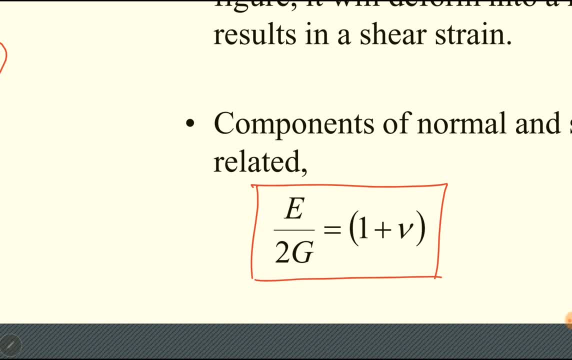 1 plus Poisson's ratio. the derivation of this expression is not necessary. you can go and read it, but I will use this expression in our numerical problems if one of the three parameters- sorry, if two of the three parameters- e, g and nu- are given. 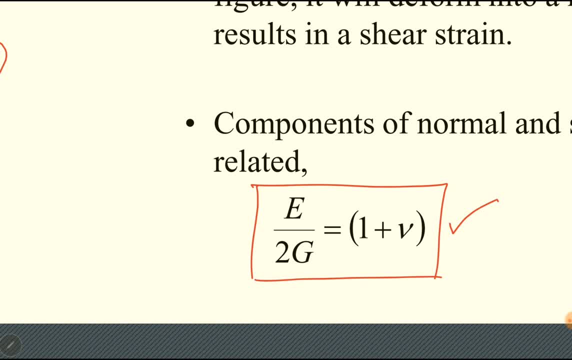 so we can find the third one for a single material. if, for any material, nu is given to us and g is given to us and we need e for some specific calculation, similarly, if any other two of these properties are given, we can find the third one. ok. 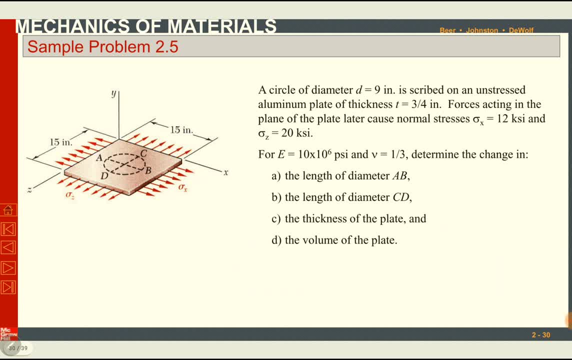 here is the sample problem. sample problem 2.5 from the text book. a circle of diameter 9 inches is inscribed on an unstressed aluminium plate of thickness equal to 3 by 4 inches. force acting in the plane of the plate causes normal stress. 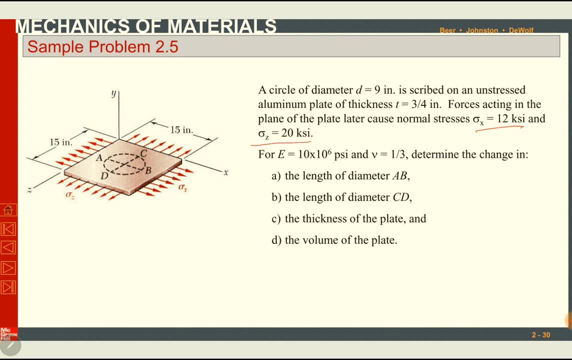 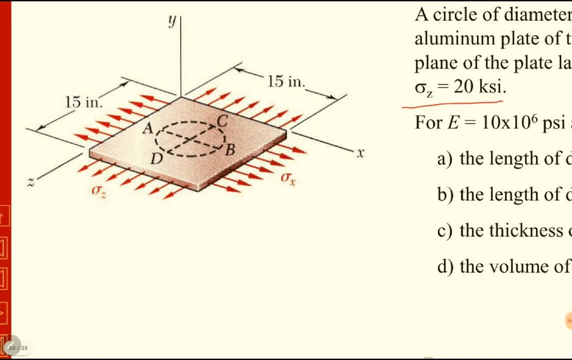 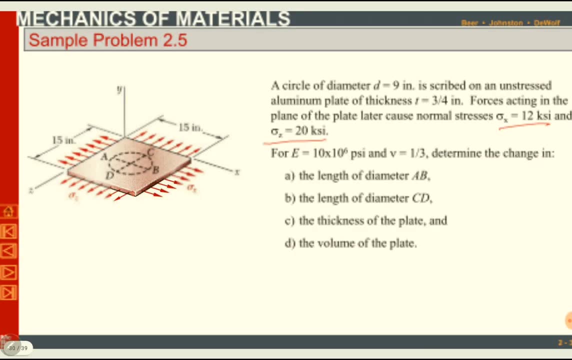 of sigma x equal to 12 ksi and sigma z equal to 20 ksi. ok, here is a thin plate which is a thickness in the third dimension, in the vertical direction, which is equal to 3 by 4 inches. it is, before applying any stress, sigma x and sigma z. 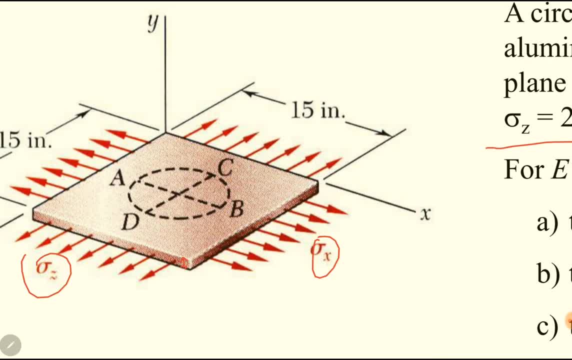 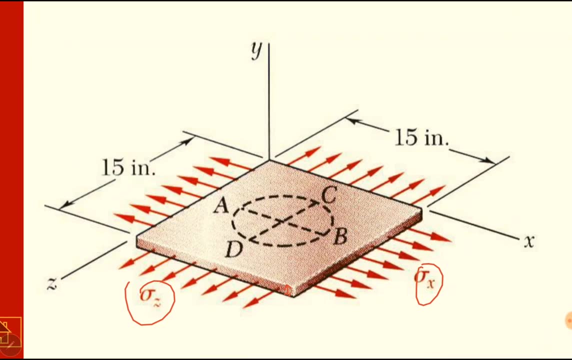 a dotted circle has been inscribed here. you can see it: a, b, c d circle. it is circle, so its diameter a b and diameter c d. both are equal. the diameter of the circle is given to us, which is 9 inches, so a b length and c d length. 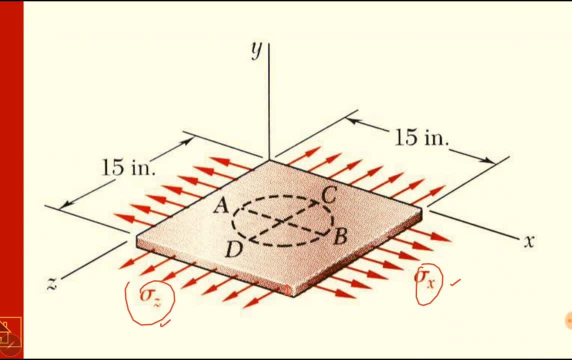 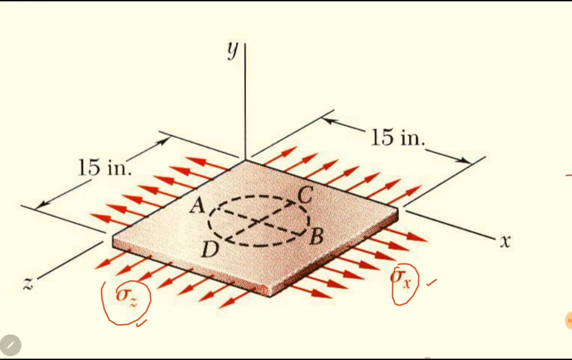 both are 9 each. before the application of sigma x and sigma z. later, after scribing, it has to be determined the team condition in the next second quantity of the applied, also of the compressive, what I've been asked from us to find out to determine the change in. 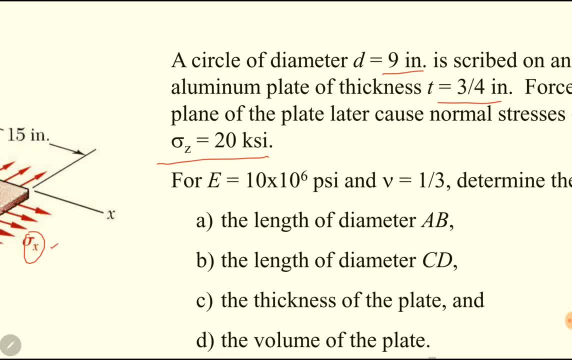 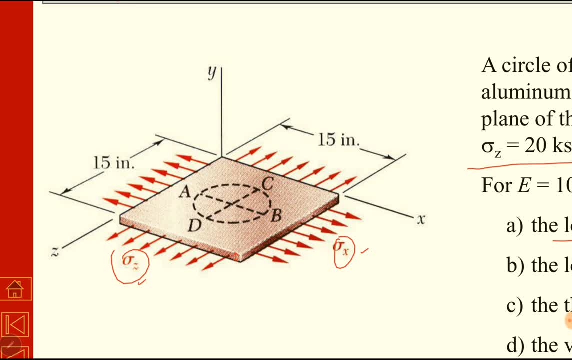 the length of diameter AB. initial diameter AB is nine inches. after application of the Sigma Z and Sigma X, what is the change in AB? either positive or negative. so it is actually a normal strength. initial length of AB is nine inches. we have to just find strain in AB. what is strain in AB? actually, AB is in 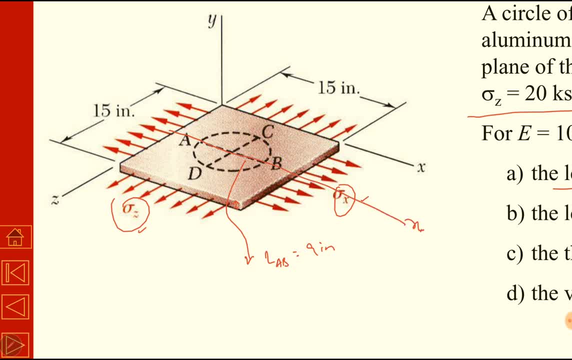 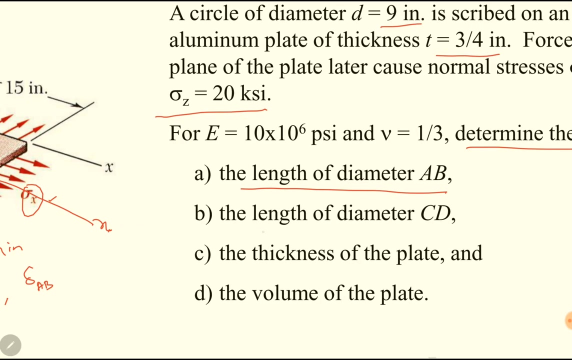 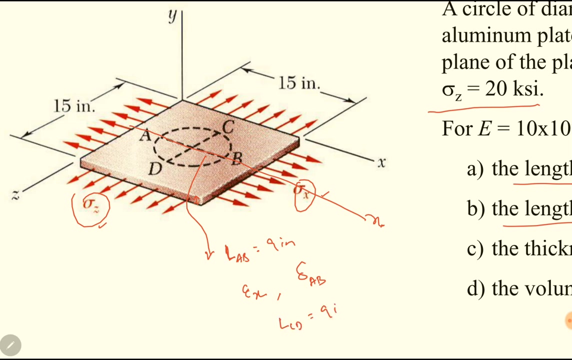 the X direction. so we have to find- first we have to find epsilon X. okay, from this we can find change in AB. if we know the epsilon X, we can, and we know the initial length of AB. so we can find change in AB similarly. second part is change in the length of diameter CD. so initial diameter CD is known to us. 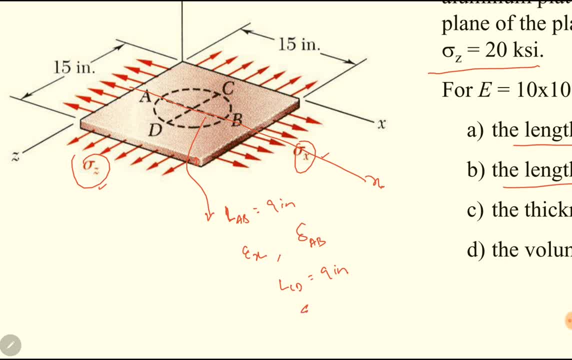 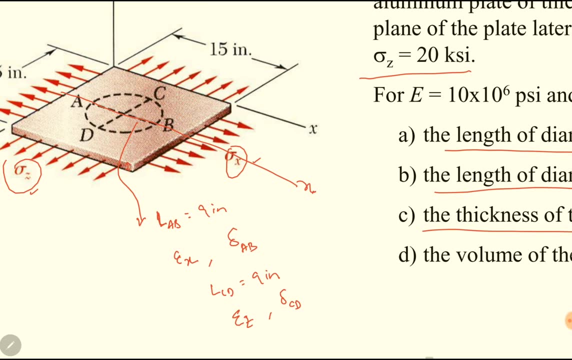 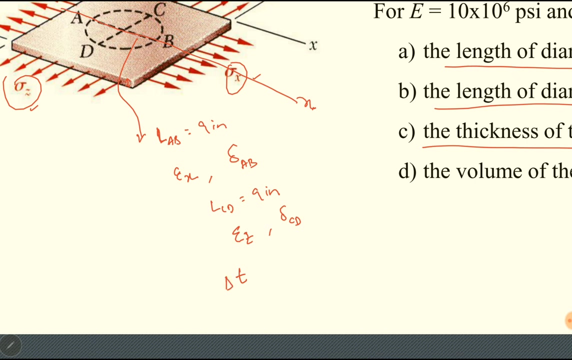 CD is in the Z direction. so we need to know epsilon Z. from this epsilon Z we can find change in diameter CD, because change in length per unit length is equal to strain. then thickness of the plate: thickness is in Y direction. so for this, for change in thickness, we have to find strain in Y direction and initial 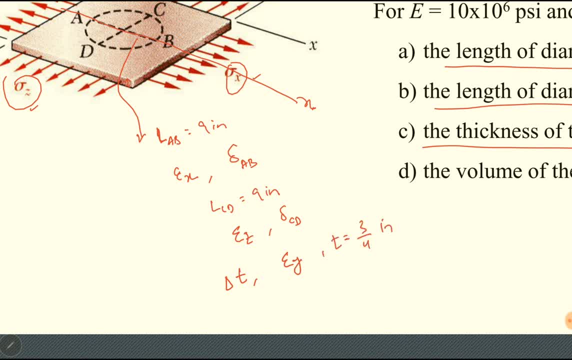 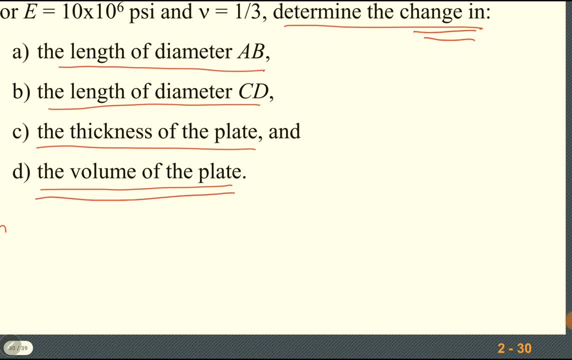 thickness is given to us just three by four inches. and finally change in the volume of the plate. change in the volume of the plate, so volume of the blade. changing volume of the plate is equal to sum of the threeobrails Bank style. epsilon X, epsilon Y, epsilon Z have derived this in our topic of dilatation Ş. but this fraction of a volume of the plate is equal to the volume of the plate. Sum of the thoresal goes to that in aris and how much dwarf we? we have to have this in our topic of dilatation, bringing in where and what structure? toemosu très important to learn and new fields is to bring the anyways of STR difference between szybularization, bacteria, viewer tratick and how many grams. here is three layers ofening Cortesan. 우리가 yi ü this because of. we have derived this in our topic of dilatation, Chrism. this is what is the state of the. 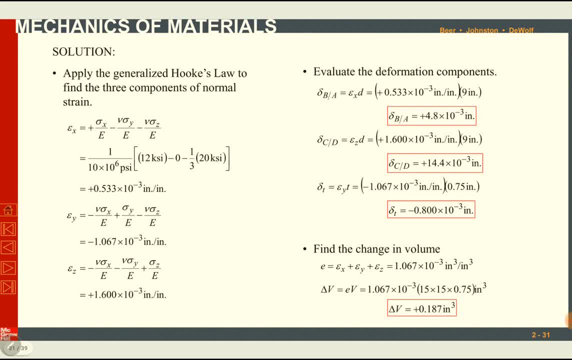 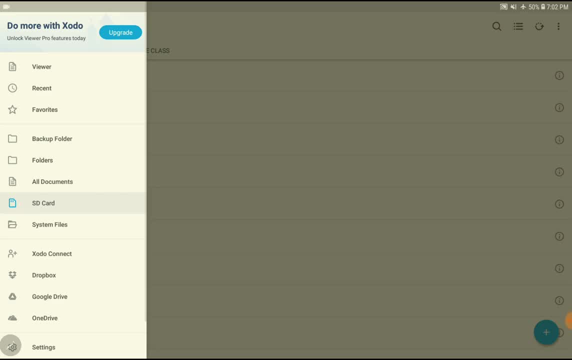 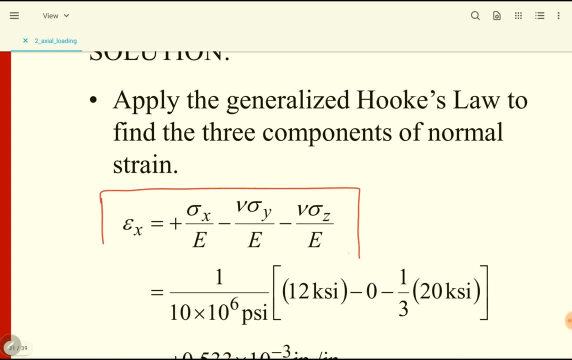 dilatation. so we will move first using generalized Hooke's law. we know the expression of generalized Hooke's law. we can find the three strains epsilon X, epsilon Y and epsilon Z using generalized Hooke's law. Sigma X, Sigma Y and Sigma Z are given to us. Sigma X, Sigma Y and Sigma Z are given to us. Sigma X is 12 KSI. 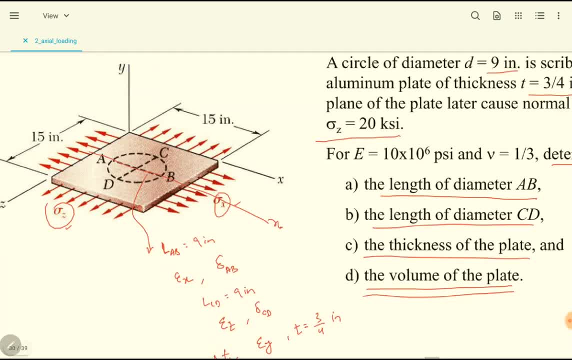 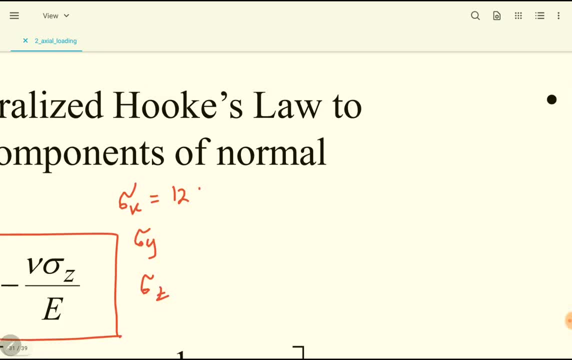 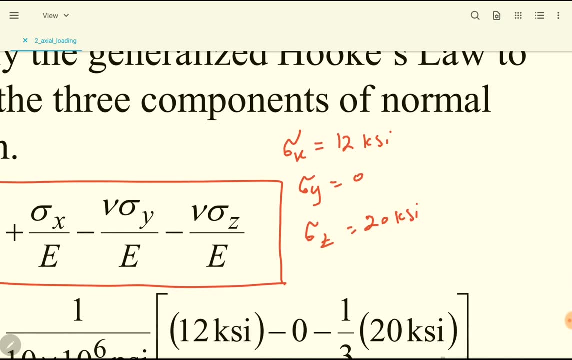 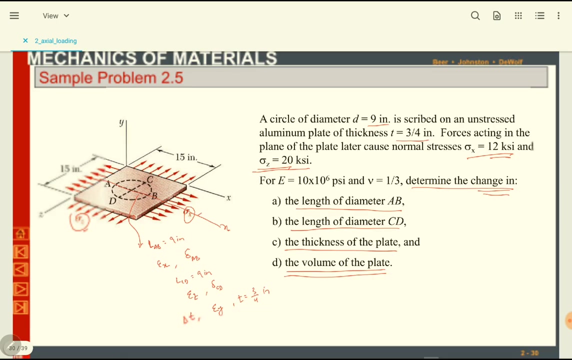 Sigma Z is 20 KSI and there is no stress or force in the Y direction. so Sigma Y is 0, 12 KSI, 0 and 20 KSI. E is given to us and nu is given to us in the statement. E is 10 into 10 power, 6 psi and nu is 1 by 3. so we know all the. 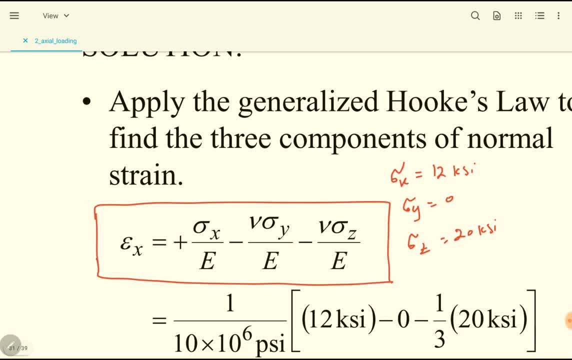 terms on the right side of this expression. so we can find epsilon X. E is 10 into 10, power, 6 psi and nu is 1 by 3. so we know all the terms on the right side of this expression. so we can find epsilon X. 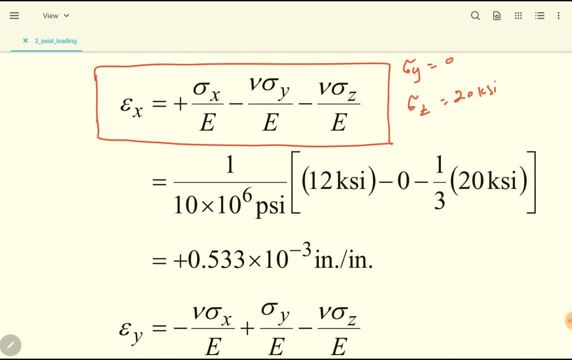 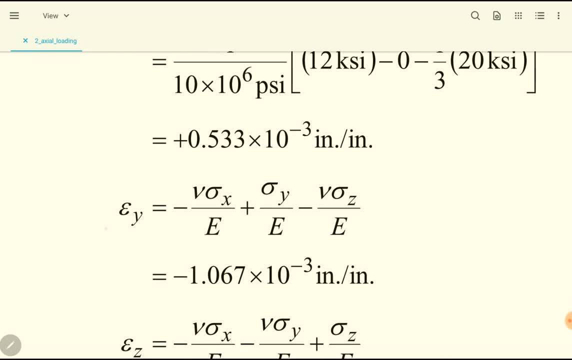 which is 0.533 into 10 power minus 3 inch by inch, means it has no unit strain. which is 0.533 into 10 power minus 3 inch by inch, means it has no unit strain, has no units. similarly, epsilon Y using generalized Hooke's law. we know all the 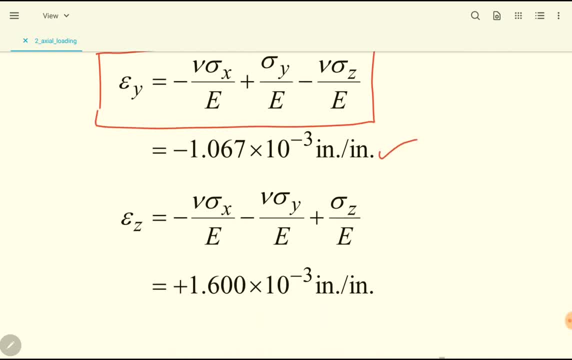 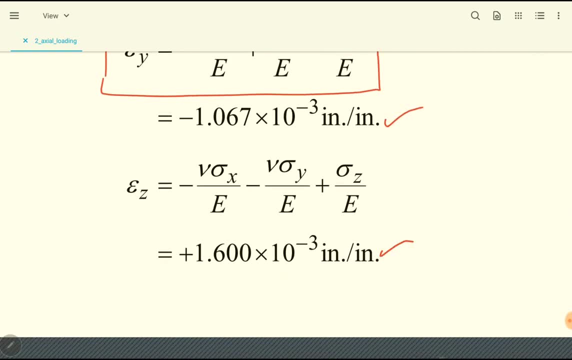 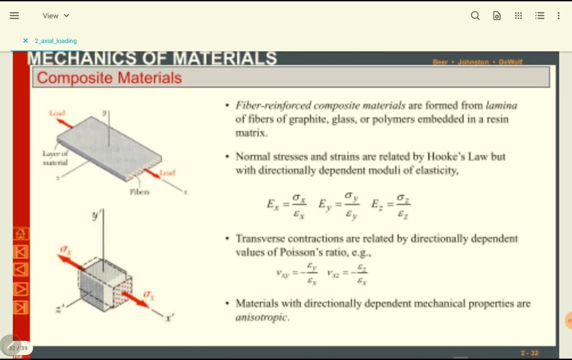 terms on the right side of the expression. so we can find strain in Y direction and similarly stress and strain in Z direction. so you can see strain in X and Z direction are positive but strain in the Y direction is negative because due to the tensile forces in x and z directions there will 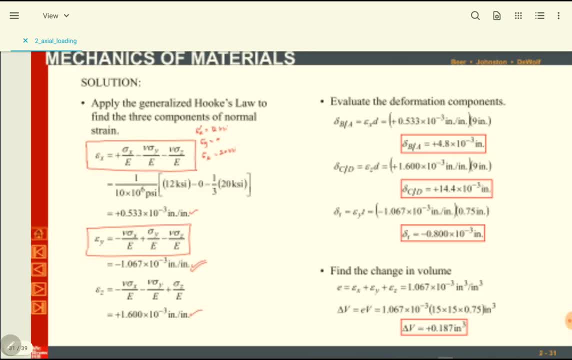 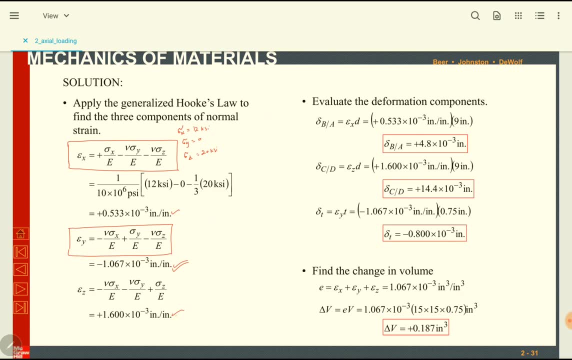 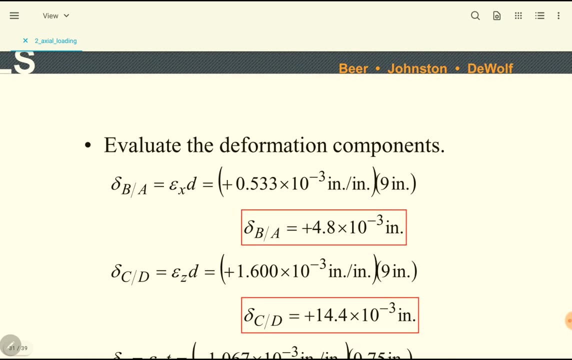 be compression in the y direction. that is why it has a negative sign. so we have found three strands in three directions: x, y and z directions, as discussed earlier. diameter in A B. diameter A B was in x direction, so del A B. delta, or change in length per unit length is equal to strain, so delta. 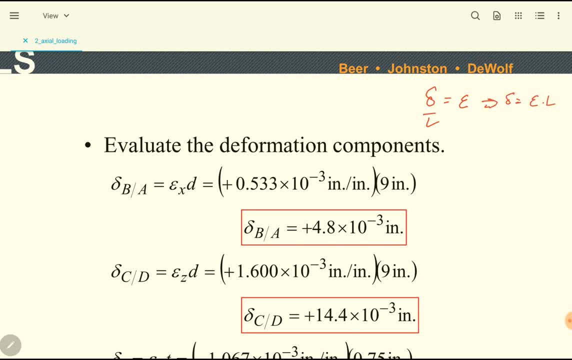 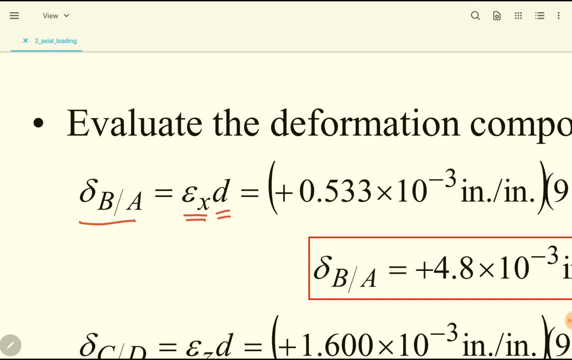 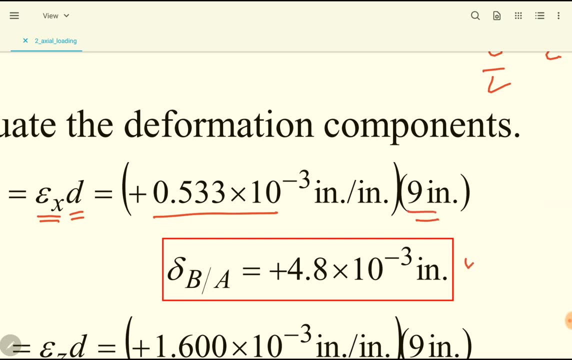 is equal to strain into length. so change in length A B is equal to strain in x direction because A B is in x direction to length of A B, which is diameter. so we know strain in x direction and we know the given diameter. so we can find change in diameter IB, similarly change in diameter. 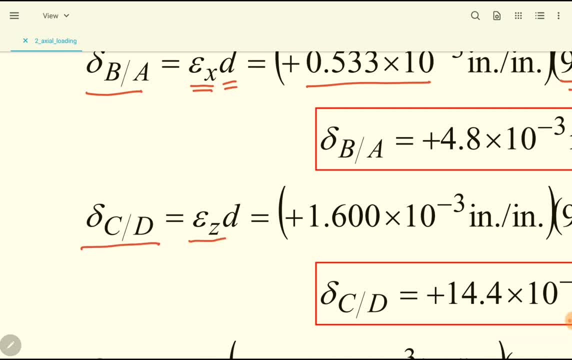 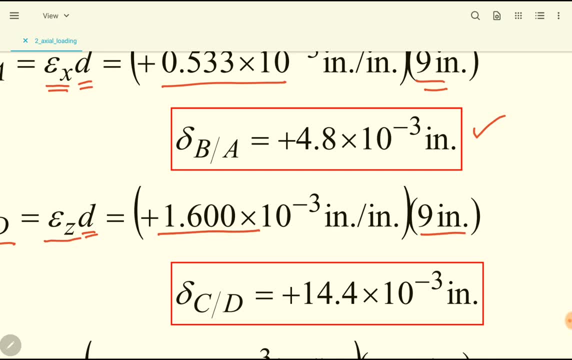 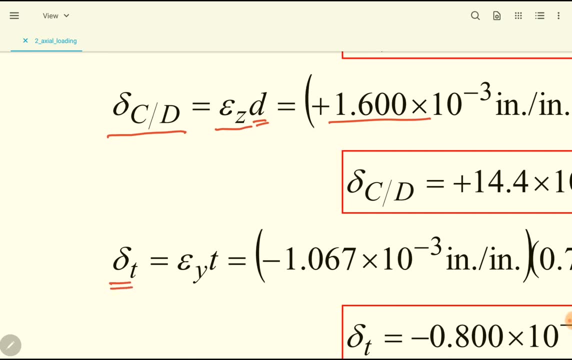 CD is equal to Stan is that direction, because CD is in Z direction and the initial length of diameter, CD, which is D Stan, is known to us. diameter is known to us, so we can find change in CD. similarly, change in the thickness is equal to thickness is in the Y direction. so strain in the Y direction and initial 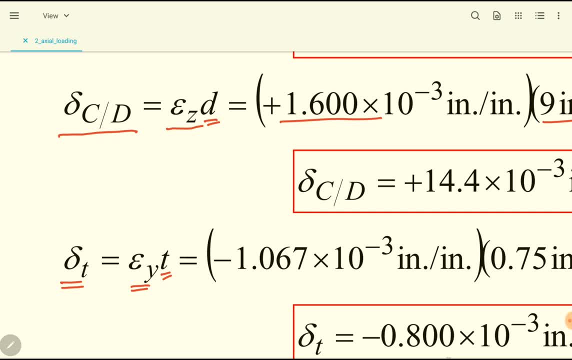 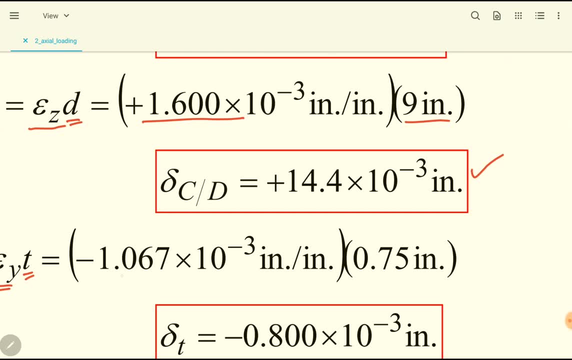 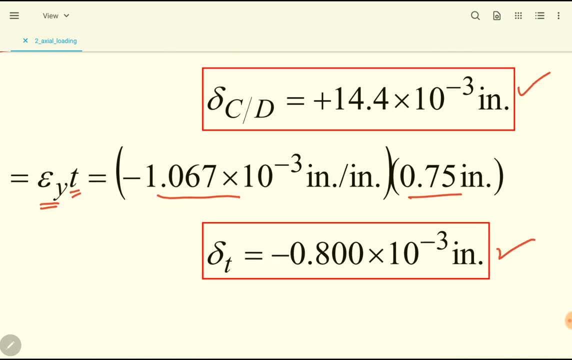 thickness. every change in the length is equal to strain in that direction multiplied by initial length in that direction. so strain in Y direction and initial length and initial thickness, both are known to us. so change in thickness is negative because there was compression in the negative, in the Y. 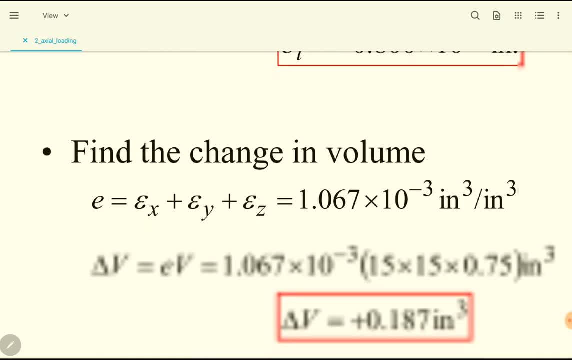 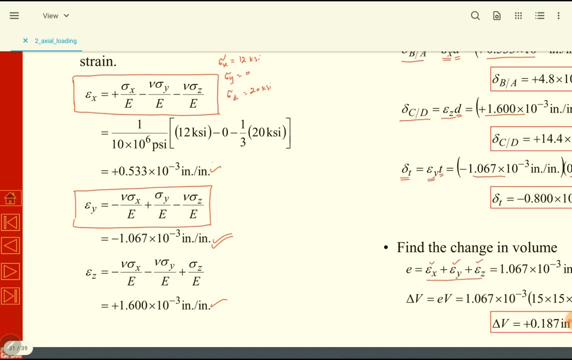 direction and then the net change in volume. as discussed earlier, dilatation is equal to sum of the three volume, sum of the three strains. so by adding epsilon X, epsilon Y and epsilon C, which we have calculated here earlier, you can find dilatation which is one point zero, six, seven into ten power. 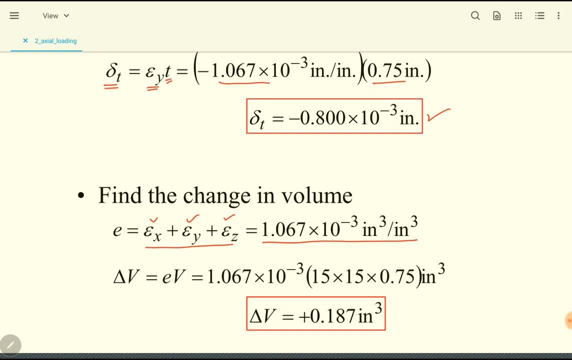 minus three. dilatation is change in volume per unit original volume. the change in volume will be dilatation into initial volume, so dilatation is already calculated here. 1.67 per unit original volume is equal to 1.60 into initial volume, so dilatation is already calculated here. 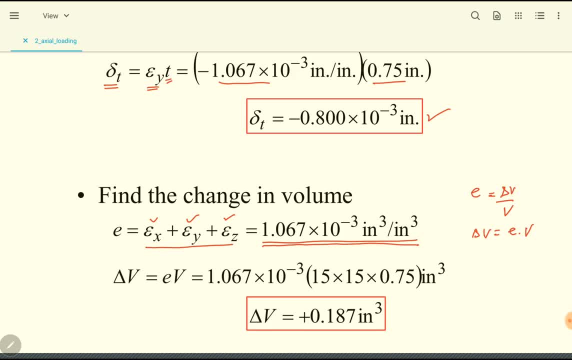 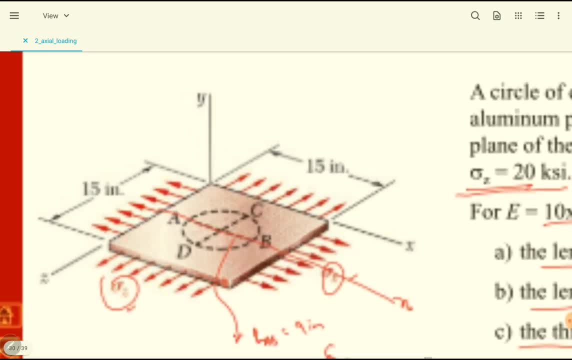 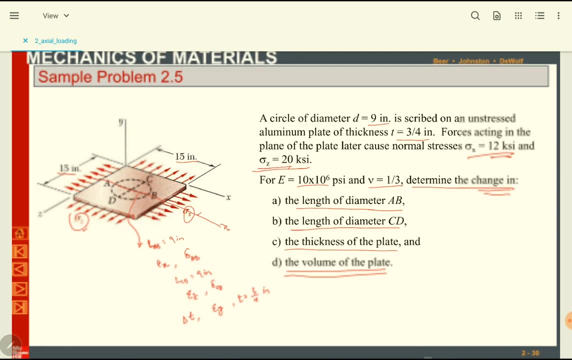 0.067, and initial volume can be calculated by multiplying the side, the lengths of the sides initially, so lengths of the initial sides are 15 inch. 15 inch and thickness. thickness is 3 by 4 inches, so 15 into 15, into 3 by 4 or 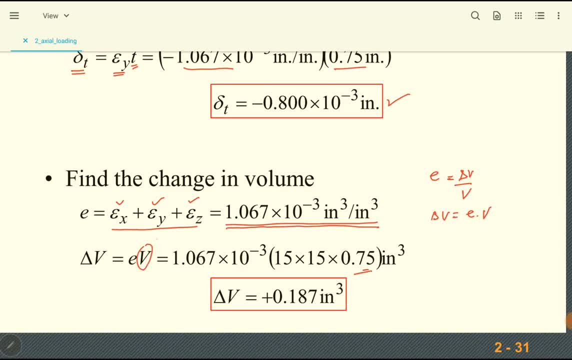 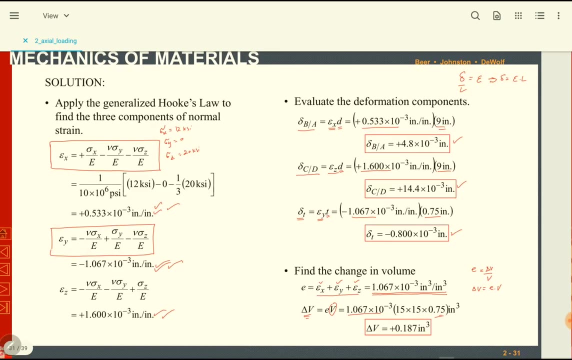 0.75, which is initial value. dilatation is 1.067, so the change in volume is equal to 0.187. so the net change in volume is positive. it is increase in volume, actually okay. the next topic is composite materials. what are composite? 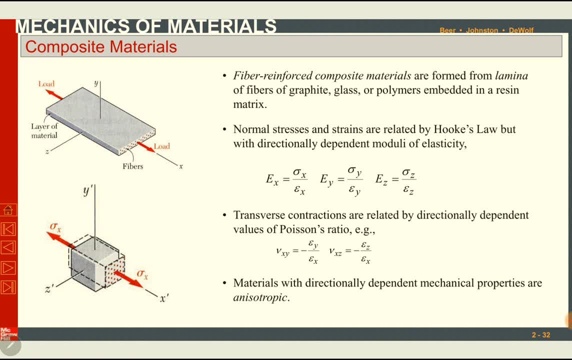 materials. actually composites are combination of more than one type of materials which are physically and chemically distinct. they are not homogeneously mixed. they are isotropic materials. they are homogeneously mixed. they are isotropic materials. they are. there will be directionally dependent properties. the composite materials. 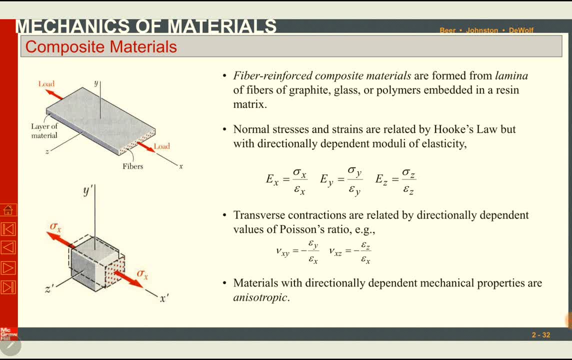 usually have different properties in different directions, in the XY and Z directions. the materials, for example. one of them is reinforcement, the other is matrix. so the reinforcements are mixed into matrix to increase its properties. one of the best example is concrete reinforcement beams and the concrete reinforcement beams. the concrete is a matrix. in the still bothered our 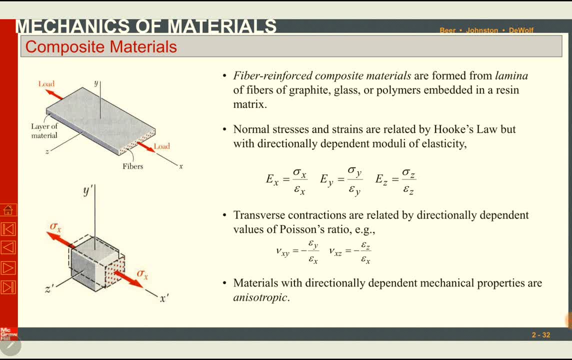 reinforcement are fibers. the serial bars are mixed with concrete to increase its tensile strength, because the concrete concrete itself has a very poor tensile strength in some properties. so composite materials are tailored materials. they are men made. materials which are tailored are which are designed to increase some targeted properties. 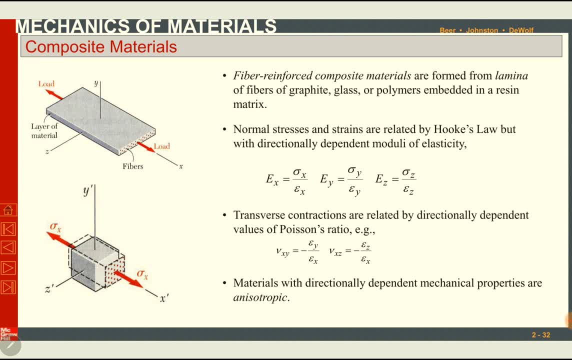 targeted directions. so a composite material which has a reinforcement and a matrix has directional dependent properties. it depends upon the direction of the reinforcement. in a concrete reinforcement beam you can see that the tensile strength in the direction of the steel bars is higher as compared to the 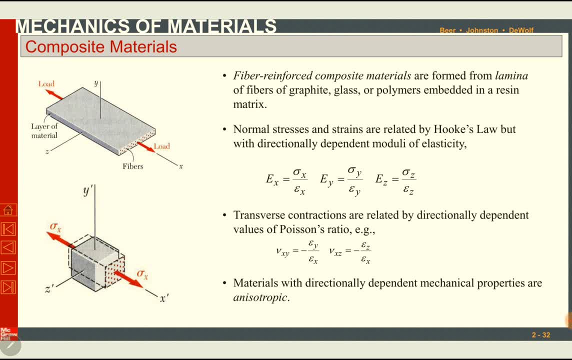 other directions. similarly, one of the famous type of composite material is fiber, reinforced composite materials. we are fibers of different materials are reinforced into matrix matrices. the fibers can be steel. it can made of steel, it can be made of carbon or glass or a natural fiber which are reinforced into. 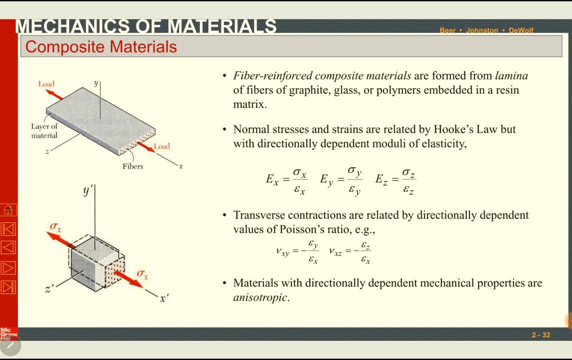 either polymer or matter, metals or ceramics. so fiber reinforced composite materials are formed from lamina of fibers of graphite, glass or polymer embedded into different resonance or matrices either of polymer, metal or ceramics. they have different directions depending upon they have different properties in different directions, depending upon the direction of the fibers or the reinforcement. 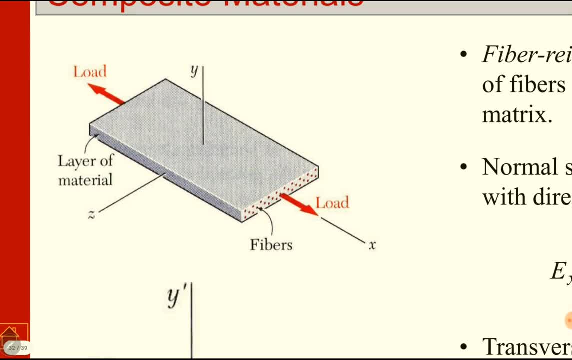 so, for example, here you can see some fibers, you can see the, the fibers in the cross-section, so this material will bear more load in the direction of the fibers here, a direction of the fibers inside this matrix, which are not visible here, so they are made with different layers of the fibers if the same fibers are. 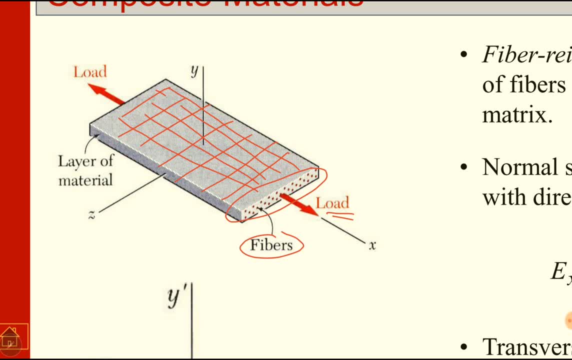 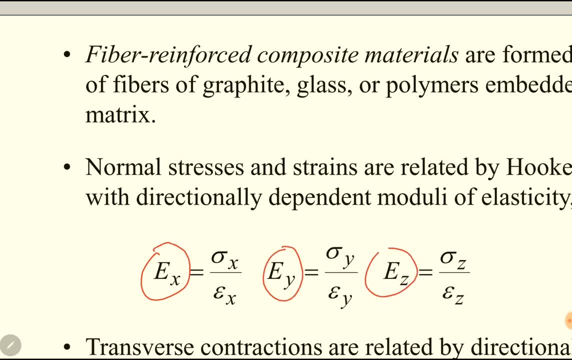 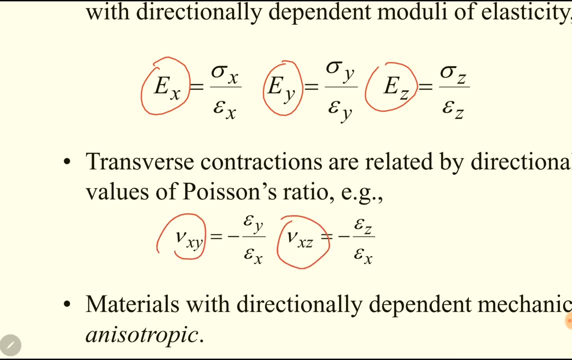 placed with the same density in the other direction, so it will have same properties in the other direction as well. so such kinda materials have different modular elasticity in different directions, in the xy and z directions. similarly different Poisson's ratio in different planes: xy-plane, in xc-plane, similarly yz-plane. so materials with directionally 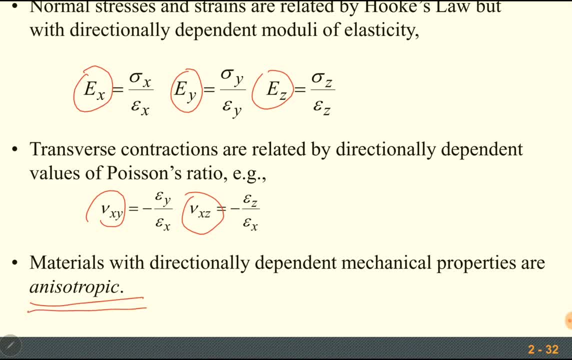 dependent mechanical properties are called anisotropic, so composite materials are just a type of are an example of anisotropic materials. up till now we have discussed all the isotropic materials. so in the future, in some other subject you may discuss or you may study about an isotropic materials as well. 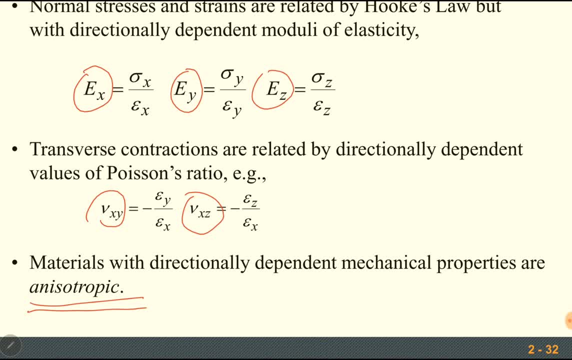 here we have just defined the composite materials. we are not discussing them in detail, but you just need to know that there may be some materials which may have different properties in different directions: different number of E, different models of elasticity in different directions. similarly different Poisson's ratio in different directions. up till now we have studied a single. 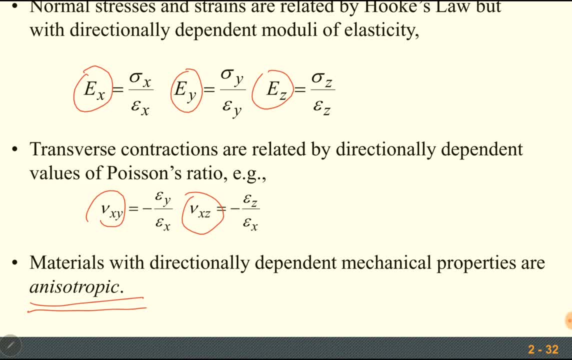 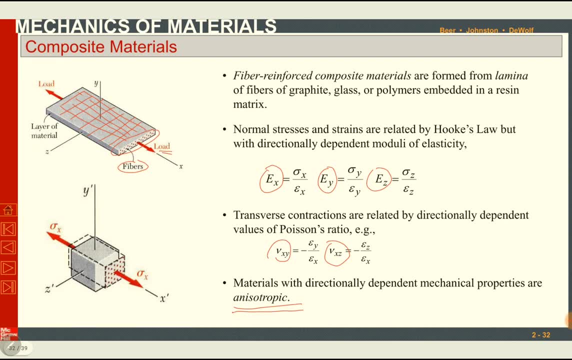 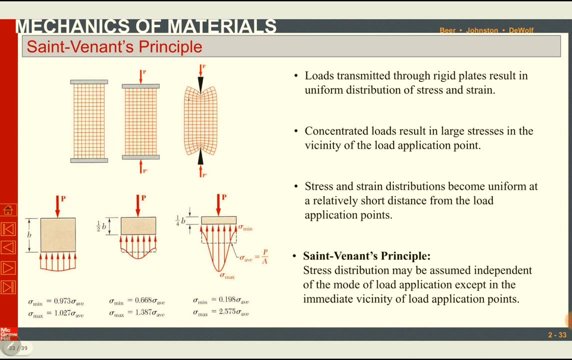 models of elasticity for a single material. similarly, single Poisson's ratio for a single material, because we have discussed isotropic materials. only if we discuss about, or if we study about anisotropic material, there will be different properties in different directions. okay, the next topic, which is: 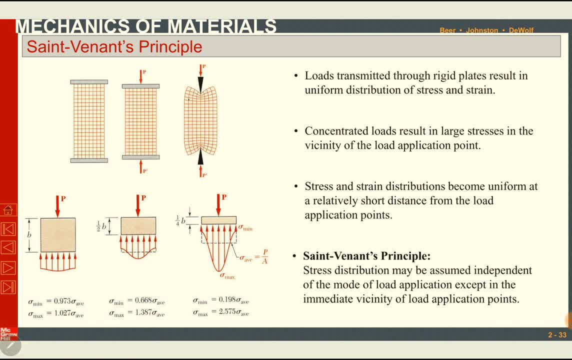 a very important one is the question of how many isotropic materials are there and how many are not, is Saint Manon's principle. it is about stress concentrations. so whenever we apply concentrated forces generally, in reality there is no concentrated force. all forces are distributed over some area. concentrated force is just. 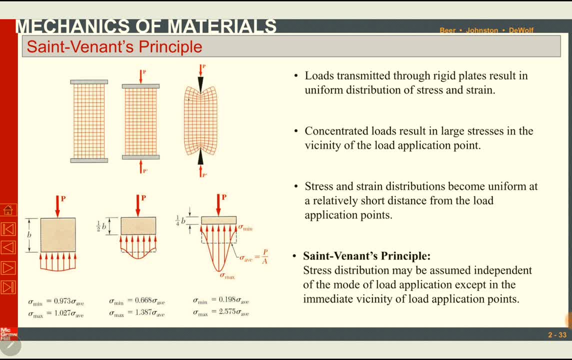 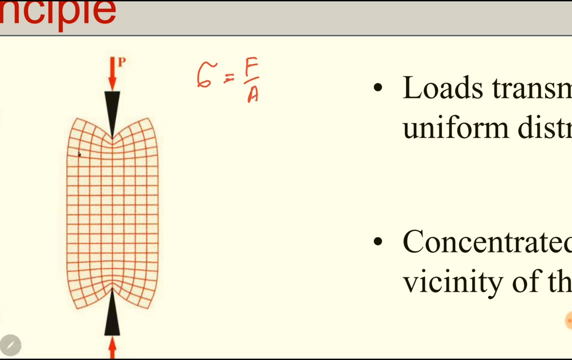 considered to be applied at a specific point and a point has a area equal to zero. so we know that stress is equal to four 뒷 divided by an area. if we consider a force is a concentrated force, it is o to be applied at a point and point has a 0 area. that means the stress must Pf. 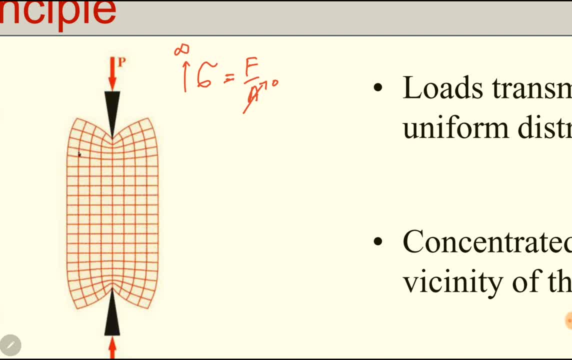 be infinite, don't? no one but? but no material can bear infinite stresses. so it means if you are applying concentrated force on any material, it is theoretically correct, but practically it is not a concentrated force. otherwise it will produce infinite, finite stress in that locality and the material will fail. so concentrated forces do not exist. 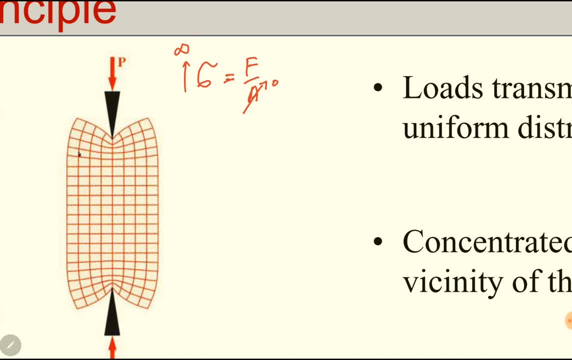 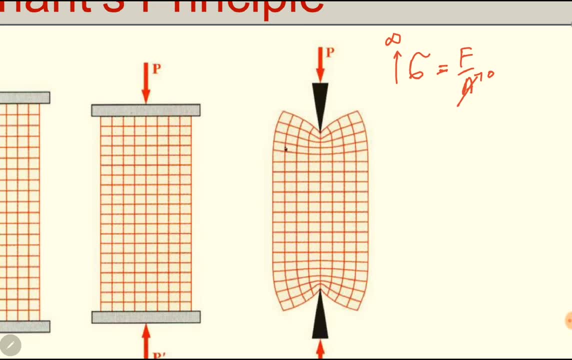 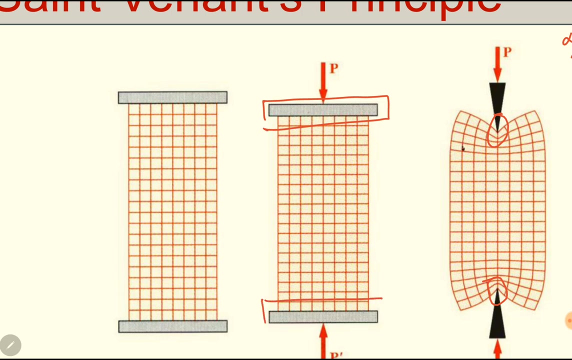 but there may be forces which are applied on very narrow regions. so here are shown some forces. for example, if a concentrated force is applied here, it will produce maximum damage in the vicinity of the point of application of the force. but instead of that, if we place a rigid plate or two rigid plates at the two ends and then we apply concentrated force, 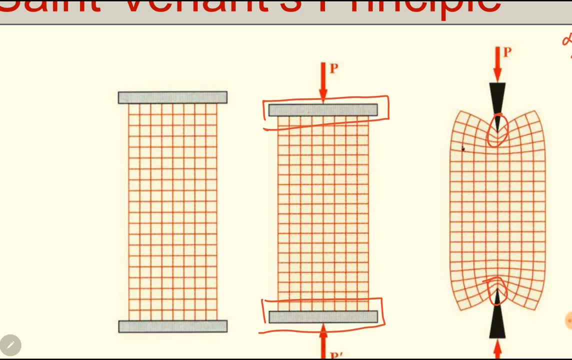 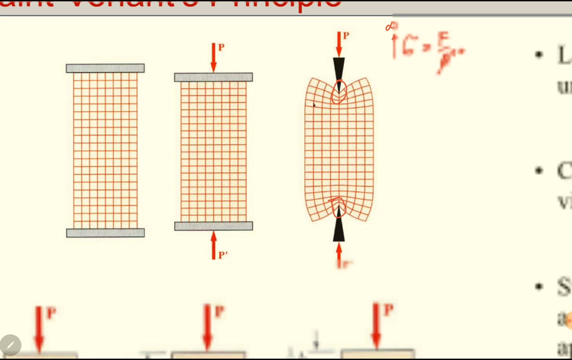 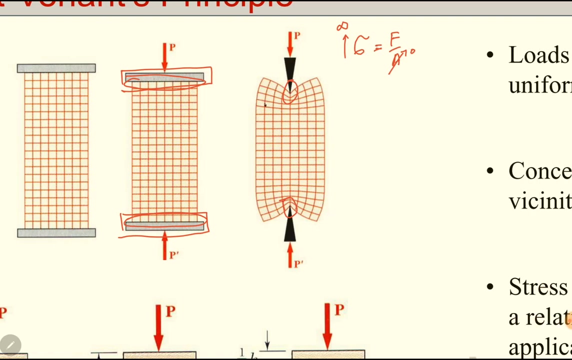 on the rigid plate. the rigid plates or the rigid materials do not undergo any deformation, so it will push or compress the whole surface uniformly. this is an ideal condition. but if there is a concentrated force, the concentrated force will produce stress concentration. similarly, if there are sharp points there will be stress concentrations, so loads transmitted. 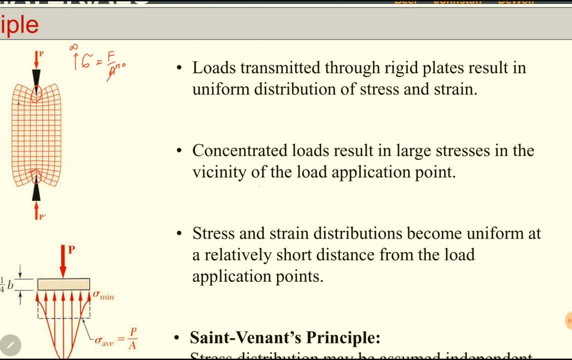 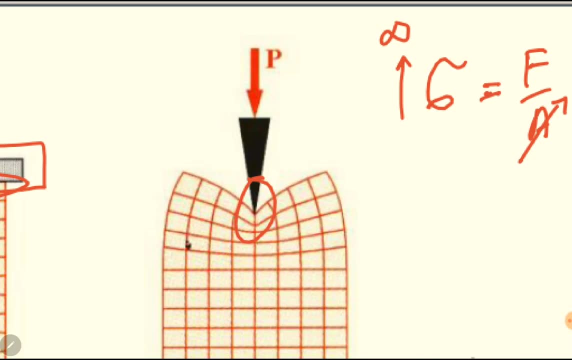 through rigid plates result in uniform distribution of stress and strain, but if there are concentrated loads they result in large stresses in the vicinity of the load application point and stress and strain distribution become uniform at a relatively short distance from the load application point. for example, if we applied concentrated force at a point, so there will 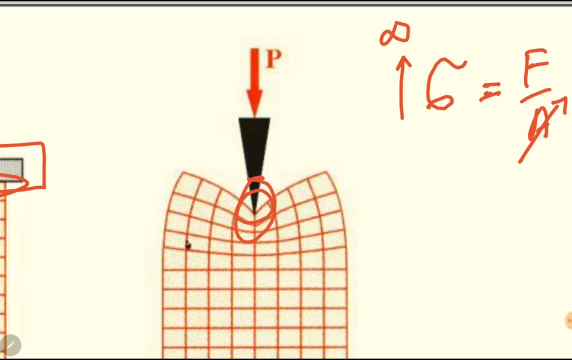 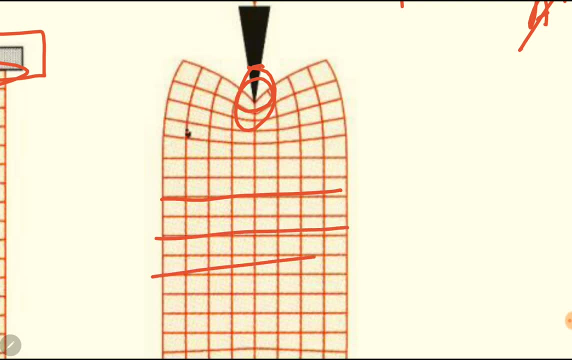 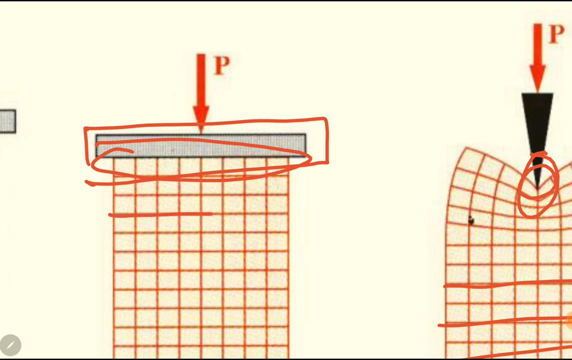 be maximum stress in the vicinity of the load application point As soon as we move away from the load application point, from here or here, or here we go down or we go away from the load application point. so the stress value will tend to be constant with increase in distance from the load application point. but in case of rigid plate, here the stresses 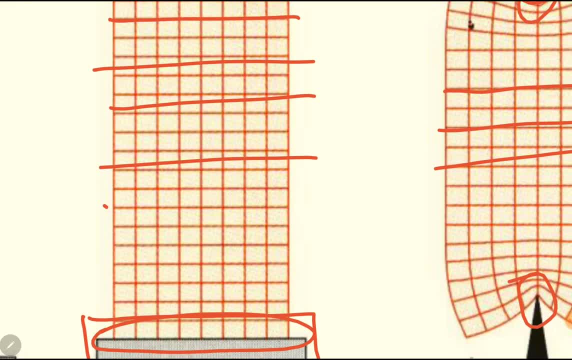 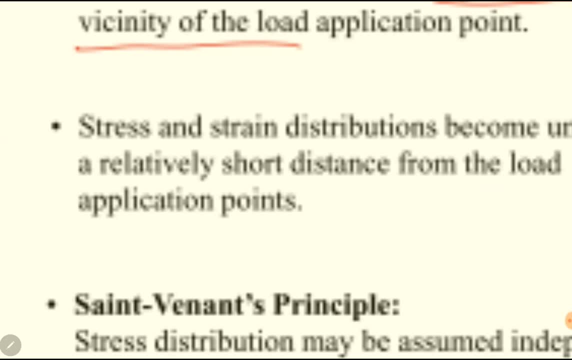 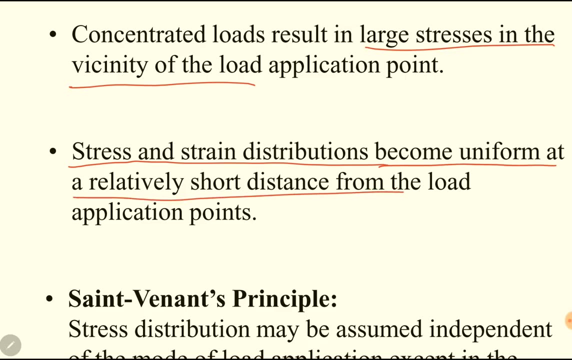 in the cross-section. So if we apply concentrated force on the rigid plate it will push or compress the whole surface uniformly. this is an ideal condition. but if there are sharp points there will be stress concentrations. so loads transmitted through rigid plate result in uniform distribution of stress and strain distribution. 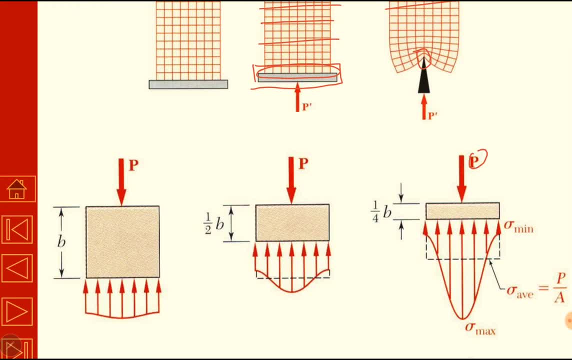 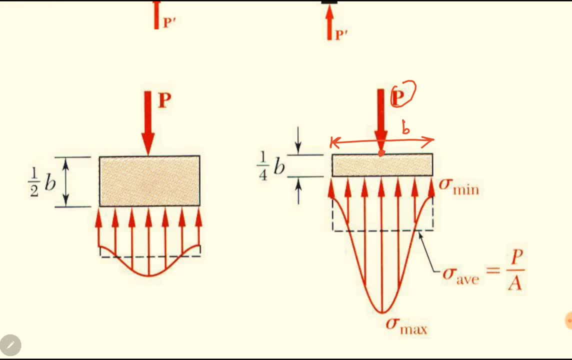 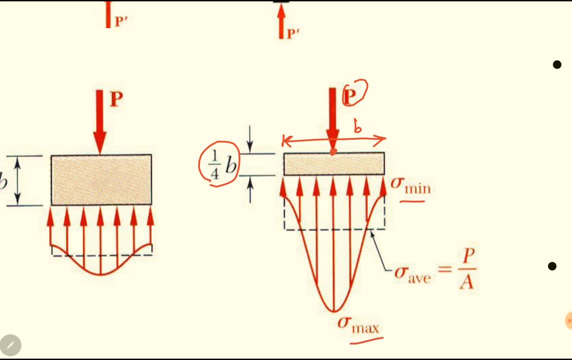 we apply concentrated force as soon as we go away from P. if we apply concentrated force as soon as from the point of application of force P, by a distance of P by 4, so the difference between maximum and minimum stress will be huge stress in the line. 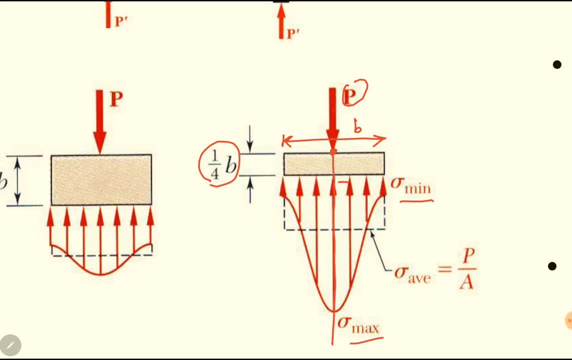 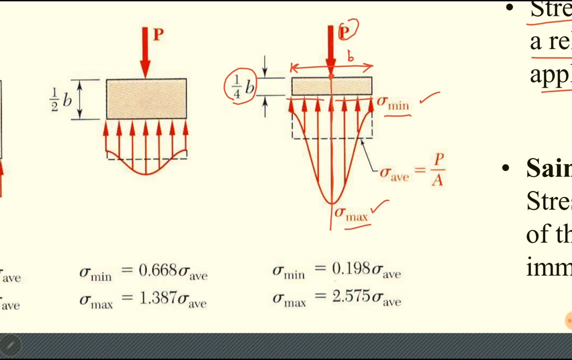 of action of the force will be maximum and the stress away from the line of force will be reduced. so the distance, the difference between this maximum and minimum force is given here. the minimum minimum stress- sorry, the minimum stress is equal to 0.1 and 8 times the average stress and maximum stress is equal to 2.5. 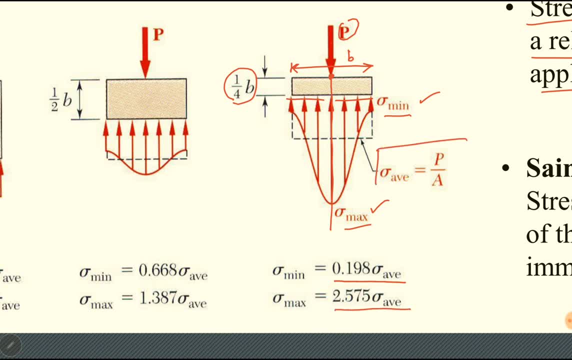 7, 5 times the average stress. what is every stress? it is P over a which we usually calculate, but there is a difference between this minimum and maximum stress. but if we go down or go away by a distance of B, by 2, B is actually width of this plate. 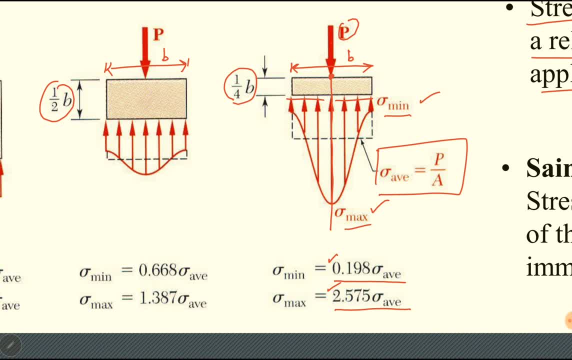 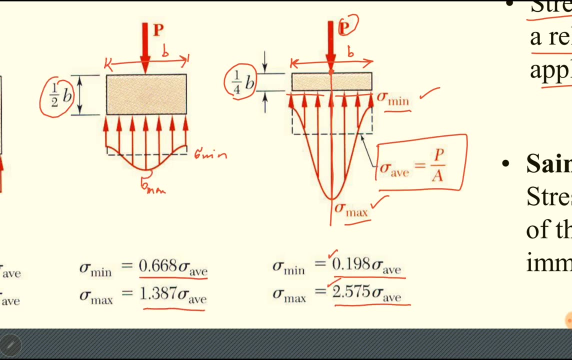 where distance of B by 2 from the point of application or the plane of application of the force. so we can see that the difference between maximum and minimum stress has reduced and the max, the minimum force stress, is equal to 0.6 times the average stress and maximum stress is equal to 0.2- sorry, 1.3 times. 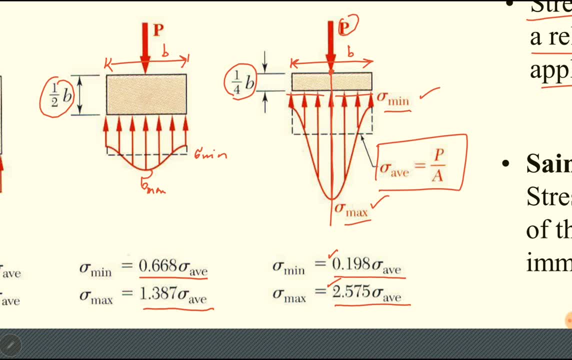 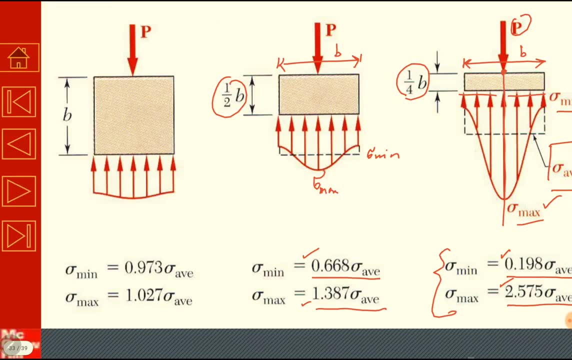 the average stress. so the difference between minimum and maximum has reduced as compared to the previous case. again, if we move further away, at a distance of B which is equal to the width of the plate, distance B from the surface of application of the force, so we can see there is a minimum. difference between maximum and minimum stress. minimum stress is 0.9 times Sigma average and maximum stress is one point zero to seven times Sigma average. this is almost the same. the maximum minimum stress is are almost same. 0.9 and 1 are almost equal. so maximum and minimum stresses. 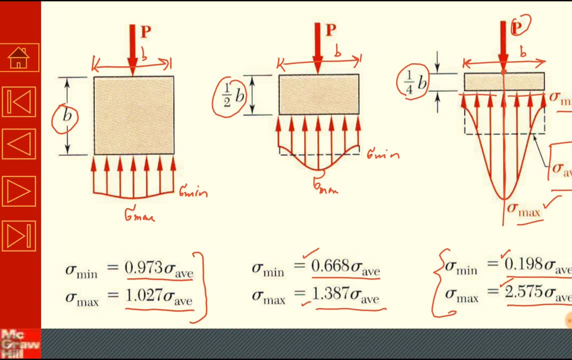 are almost same if we are going away from the point of application of the force. but if, as soon as we move towards the point of application of the force, there will be stress concentration, there will be localized maximum stresses, which is a very important topic. maximum stress at any point are in the vicinity of the 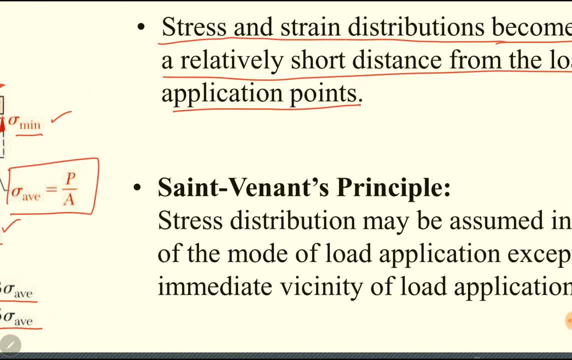 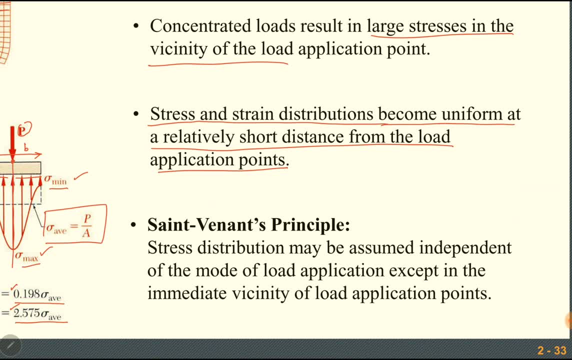 load application point may produce the maximum damage, which we have not discussed until now. we will discuss it in the StVenant's principle or in this specific topic. stress distribution may be assumed independent of the mode of load application, except in the immediate vicinity of the load. 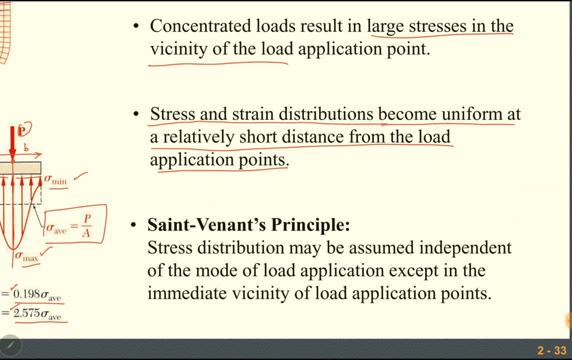 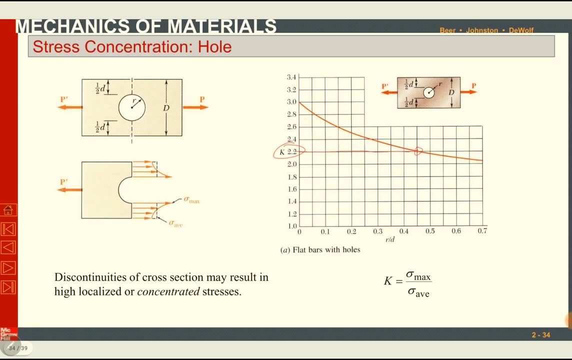 application point. so stress distribution or the intensity of stress is very serious- are very important only in the immediate vicinity of the load application point. ok, have some specific cases. one of the case is a hole in a plate we can see is a hole in the ok. before that we need to know a relationship between maximum. 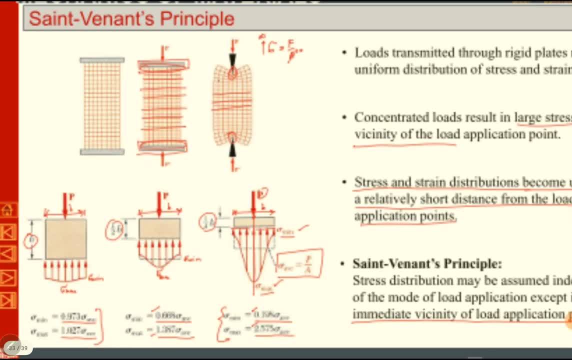 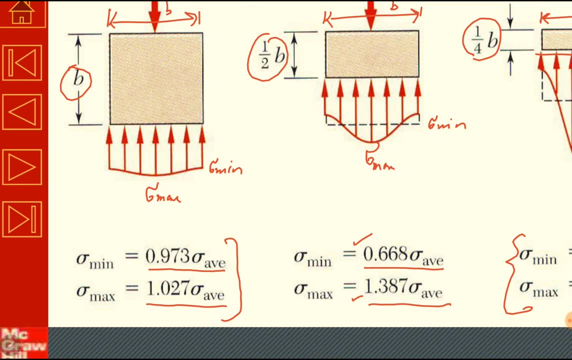 stress and average. previously we have seen there are maximum stresses and minimum stresses. there's a distribution of stress on surfaces, so somewhere it will be maximum in the load facility load application point, near the load application point, and it will be minimum away from the load application point. there is a variation between 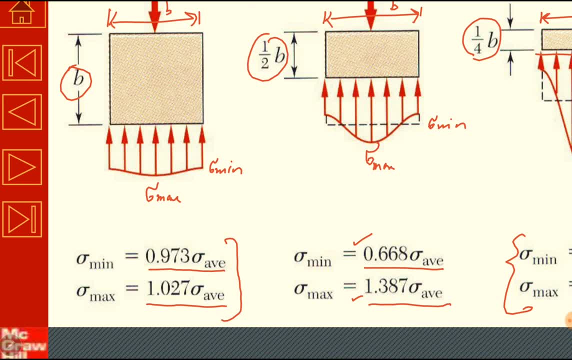 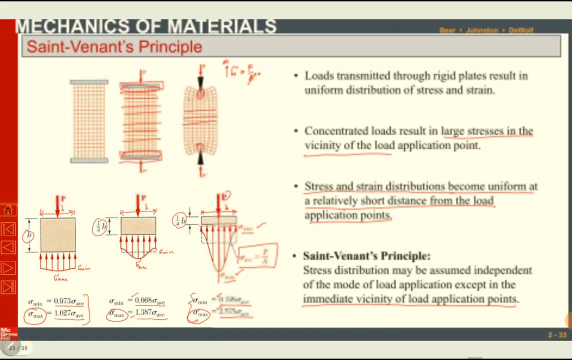 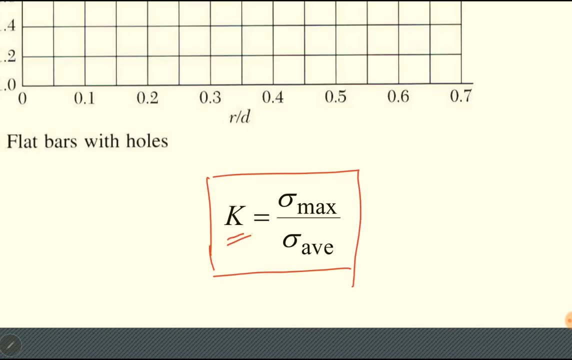 maximum and minimum. so this maximum stress is very important for us, not the minimum one. in each case, maximum stress is important for us. so there's a relationship between average and maximum stress. the ratio of maximum stress to the average stress is called stress concentration factor, K1, K-2, etc. 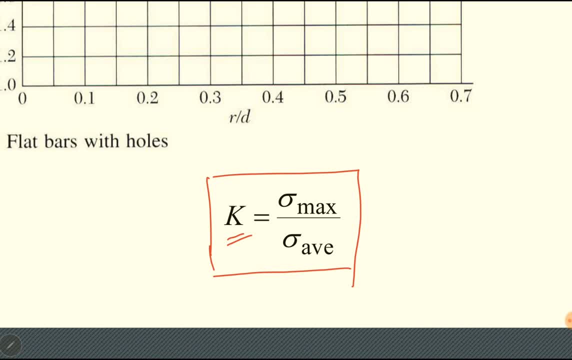 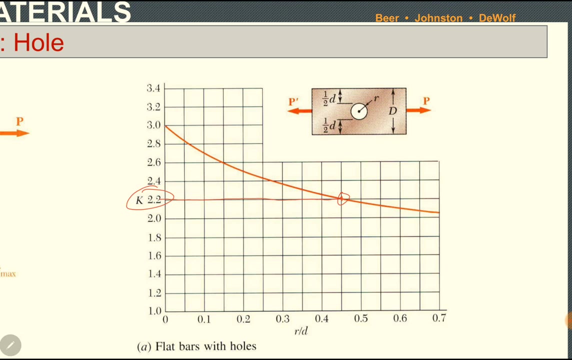 factor K. If the maximum stress is much higher, there will be a higher stress concentration. factor K. In some cases, where the plates or the bodies have irregularities like holes or fillets or sharp points, there will be stress concentrations. there will be maximum stress near the sharp points or the. 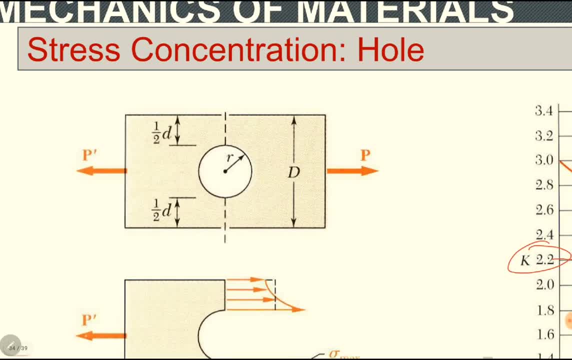 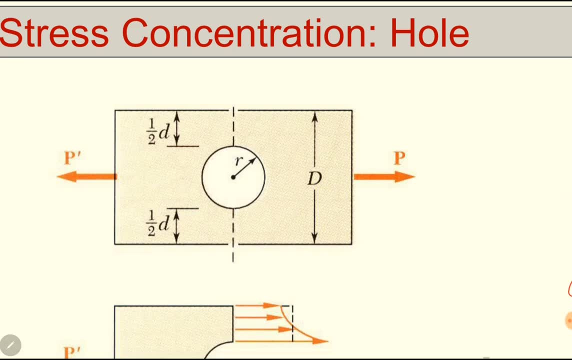 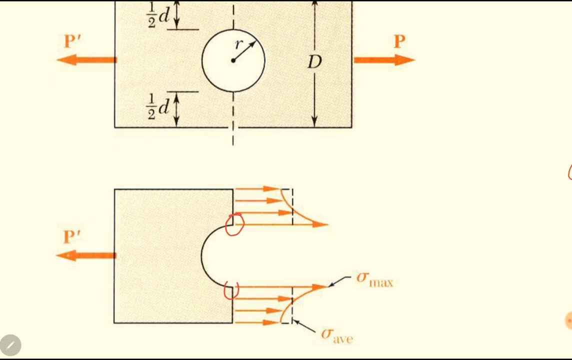 irregularities. So just like that, if a plate has a hole, hole is an irregularity or a flaw, so we can see that around the hole stress will be maximum, and near the hole, like here it will be at this point, at the edge of the hole, stress will be. 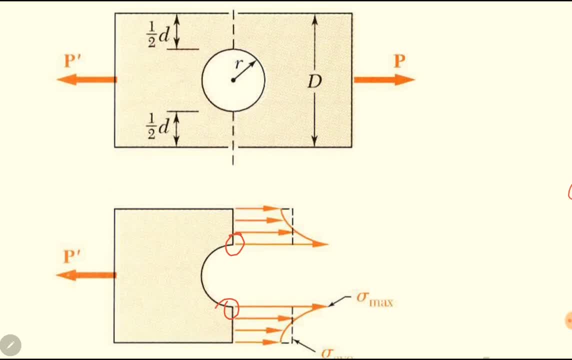 maximum. We have just sectioned this plate and we have seen that stress is maximum at the edge of the hole. As soon as we go away from the edge of the hole, it starts reducing and it will be starts reducing. it will be minimum at the outer edge. 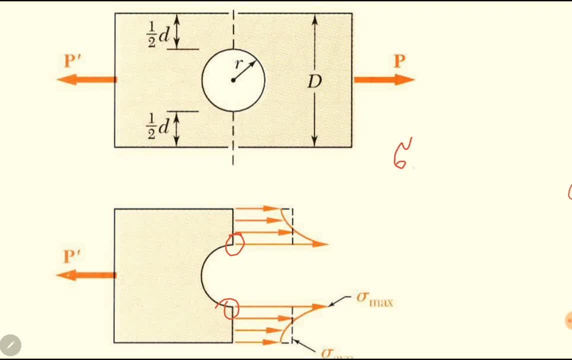 Okay, normal stress or average stress is equal to force divided by area. Force is the externally applied force, and what is area Area is the cross-sectional area. In this case, this cross-sectional area, which is equal to the total, In this case it is equal to width D into thickness in the third dimension. 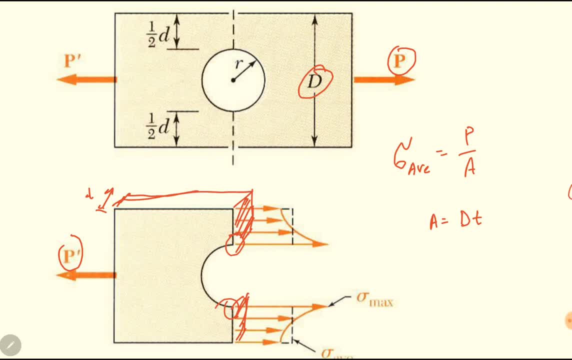 D into T, But if there is a hole, so we have to reduce the diameter of the hole, which is two times radius. we have to reduce the diameter of the whole from the thickness, because the whole thickness is not under the stress, it is only this shaded portion which is under the stress. 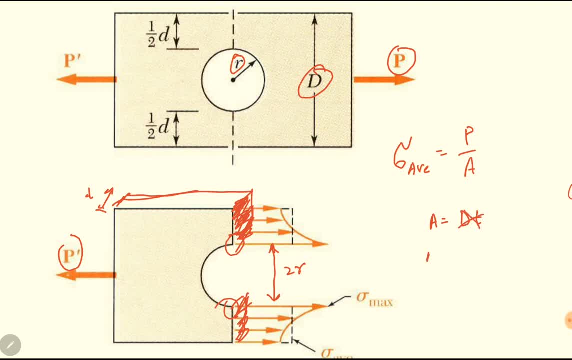 what we have to do. it will be: area will be D minus the diameter of the hole. this capital D is not diameter. capital D is the width of the plate minus diameter is 2R into thickness. this shaded portion is the area under force or under stress. so this area. 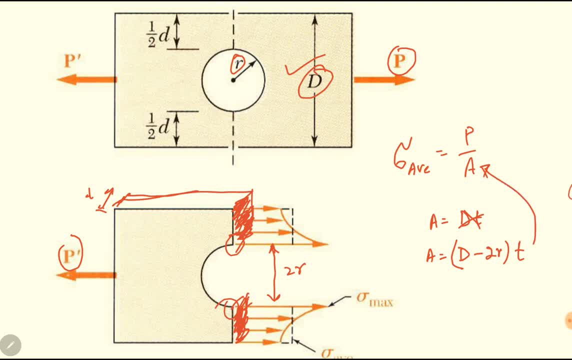 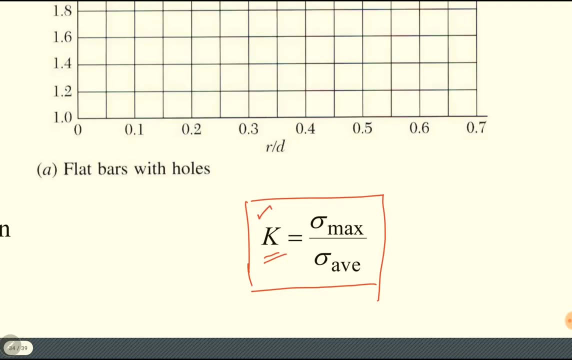 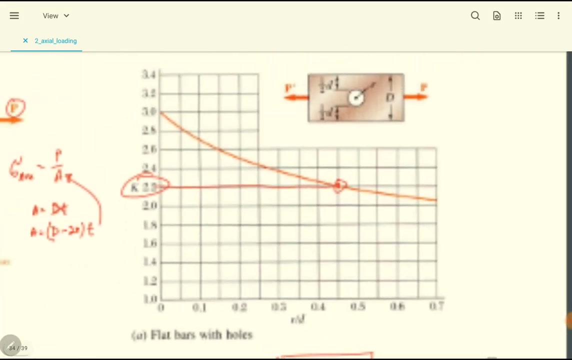 is inserted in this expression P divided by area, so we can find every stress. with this expression, average can be calculated like this: if we know K, so we can find maximum stress. so how can we find K? K can be found from this chart for a plate with a. 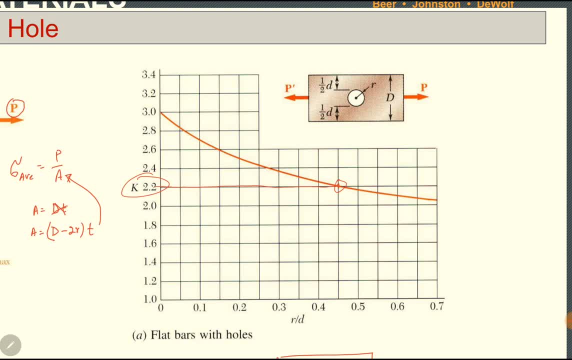 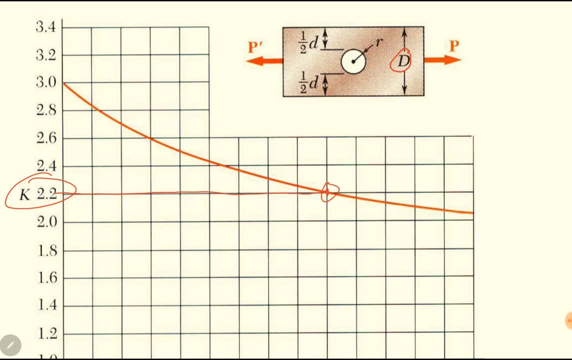 hole in the center. so for a plate with a hole, capital D is, in this case is the width of the plate, R is radius of the hole. small d here, in this case small d, is half of the sorry small d is capital D: width of the plate minus. 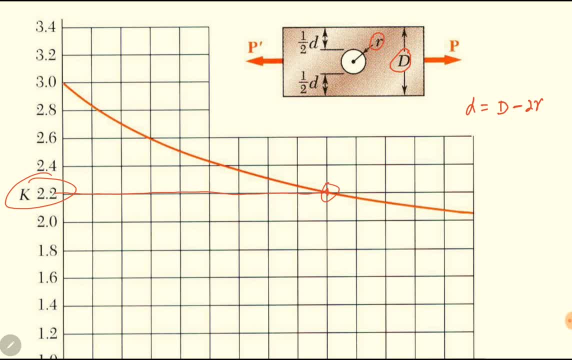 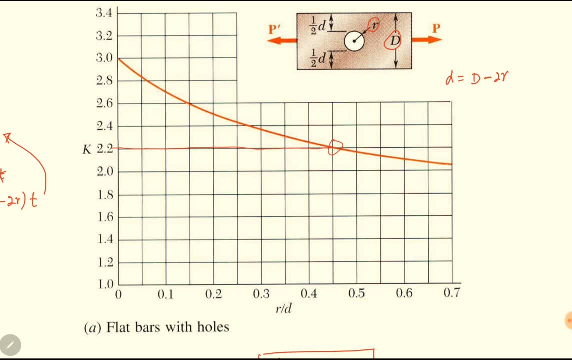 diameter of the hole. OK, so this chart is given to us. in this chart we can find K. K is a geometric property. stress concentration factor is geometric property. it will be different for different geometries, if the value of D, which is width of the plate, or R, which is radius of the whole. 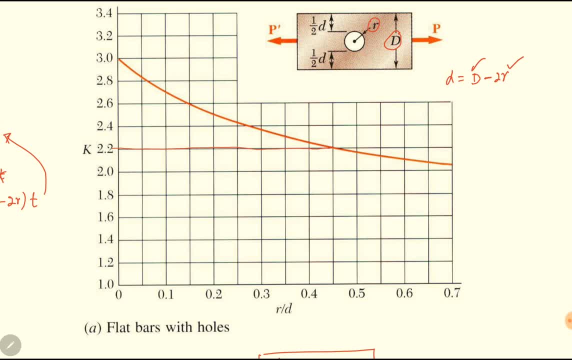 if D and R changes, K will change this curve or in this chart. R over D is the horizontal axis, r is radius of the hole and small d is given in this expression and on the vertical axis it is stress concentration factor, k. So for different, 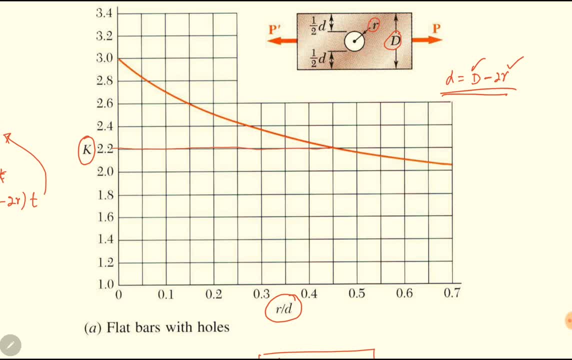 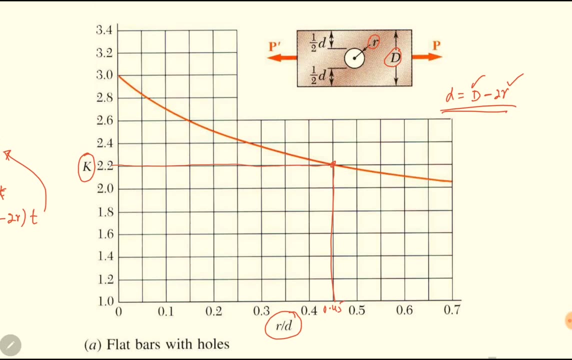 ratios of r over d, we have different values of k. For example, if r over d is 0.45, k is here, which is equal to 2.2.. This k has no unit because it is a ratio between similar quantities. Okay, so we can find k for this geometry for a plate. 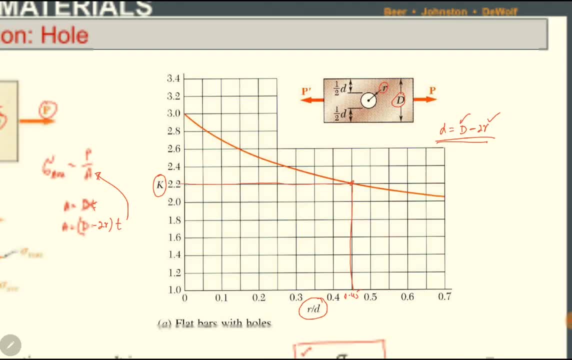 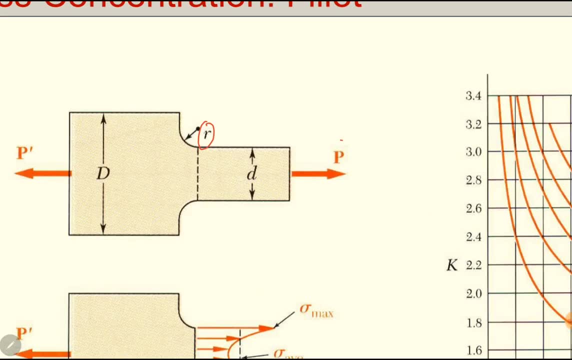 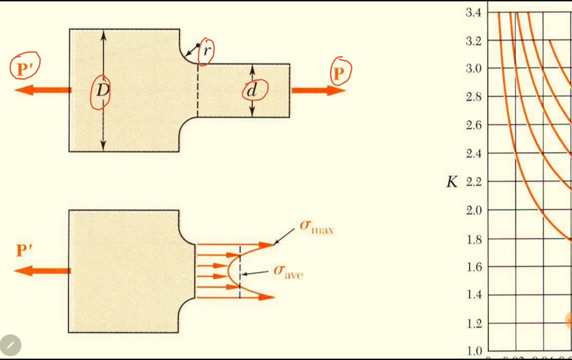 with a hole in the center. Similarly, if we have another kind of configuration, a fillet of radius r and external force P is applied. it has two thicknesses: this bit larger thickness, capital D, and a smaller thickness, small d. Remember that you have to see in different books different. 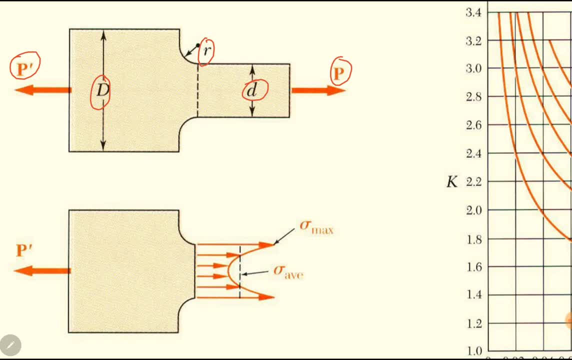 symbols which are written in different languages. If you have seen, the book are used for thickness and width. so in this specific book capital D and small D have been used. even in this book the charts are different in different editions. in this specific edition this graph is from the third edition. you can 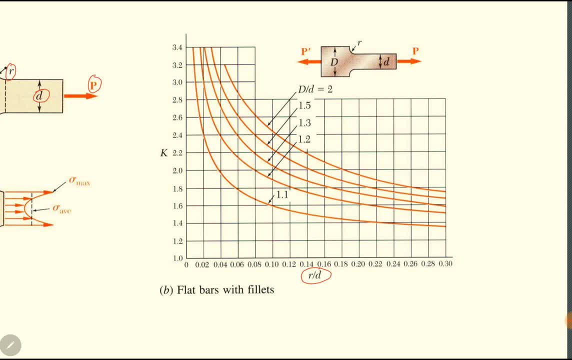 see, the horizontal axis is R over D. in the other edition it may be 2R over D, so you have to use it according to the edition. the net answer will be same, but some charts are. some charts involve different ratios and different values. okay, in this case, horizontal axis is R over D, where R is radius of the. 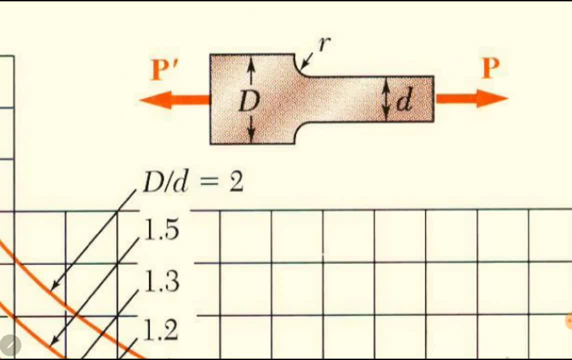 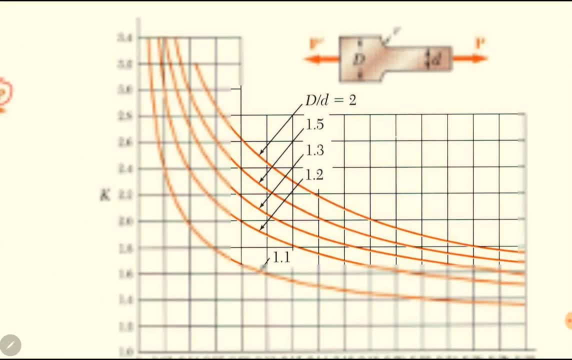 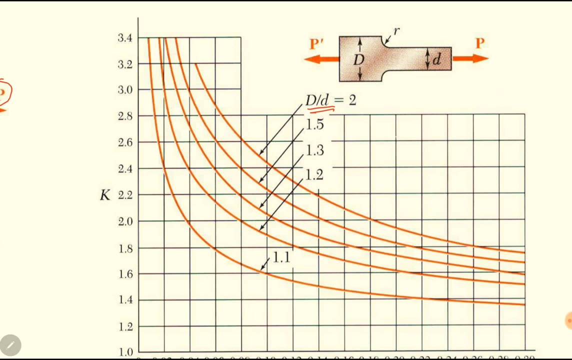 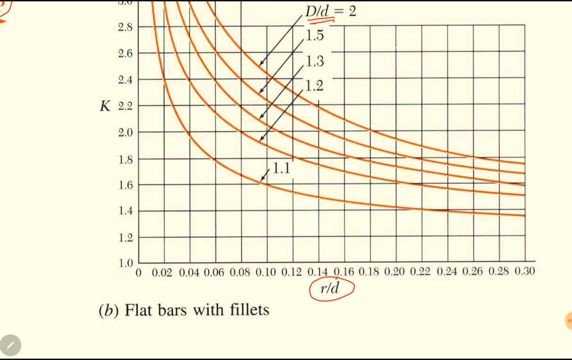 palette and small D is the smaller width, are the width of the smaller part of the plate. okay, there are different curves, all for different D over D ratios, capital D or small D ratios. so, for example, if we have a configuration where our R over D ratio is, for example, 0.18 and our capital D over small D, 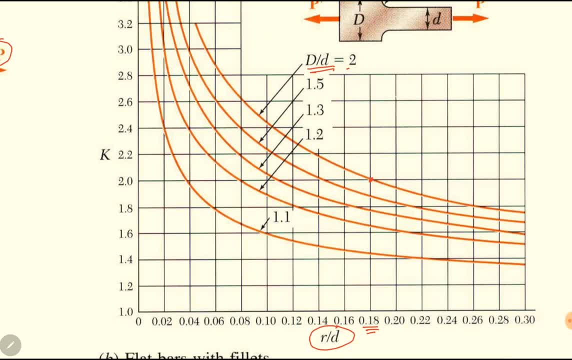 ratio is, for example, 2, you have to use this curve, outermost 2, so for 0.18. extend this line and where it intersects the curve, you can see the value of K, which is 2 in this case. it will be different in different cases. if the 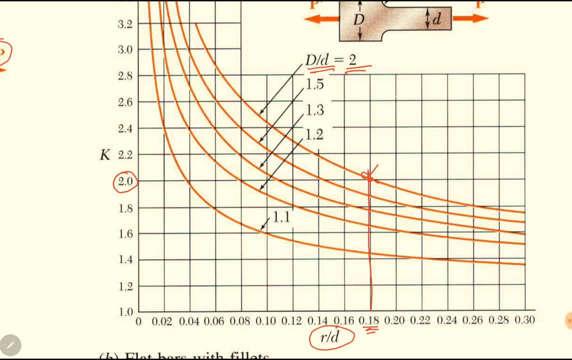 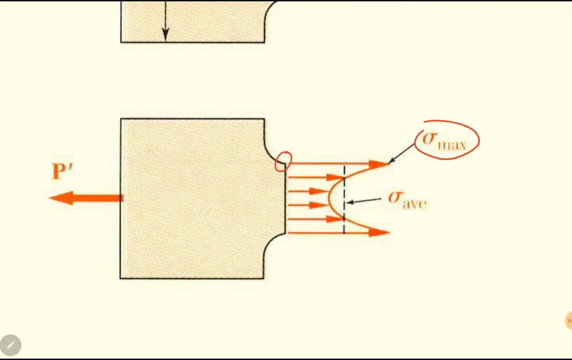 given. if over D, over D ratio is not present in this chart, we have to use interpolation method. we have to find the value of K for different curves and then we can use interpolation. something in between them. here we can see again: stress is maximum near the edges of the fillet, and it will be. it will decrease as soon as we go. 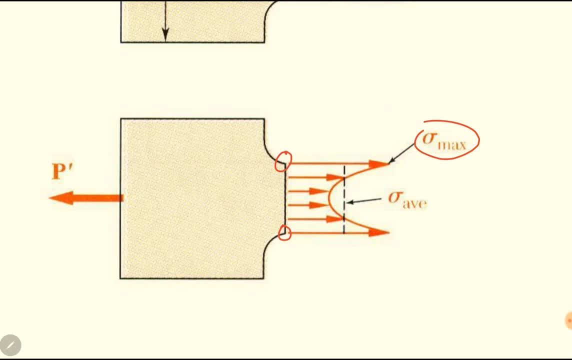 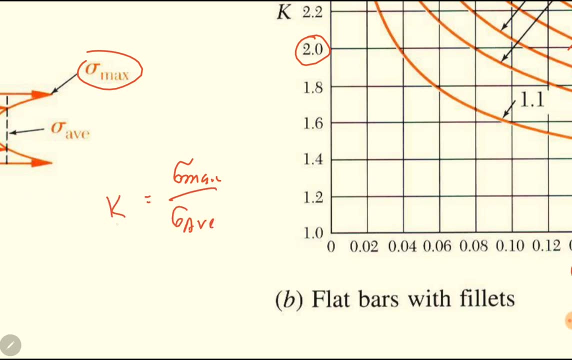 away from the sharp points again, in this case maximum stress over every stress, and it will decrease as soon as we go away from the sharp points again. in this case, maximum stress over every stress is equal to K. so if we can find K from this chart, K is a geometric property and we find sigma average. 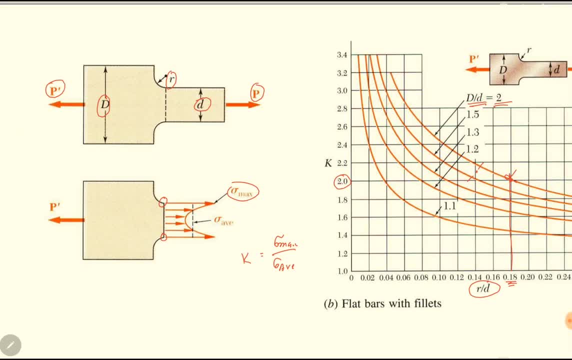 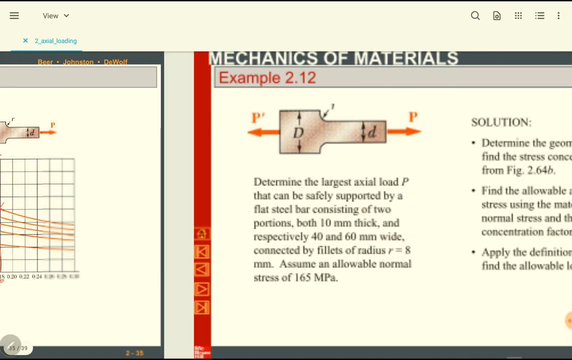 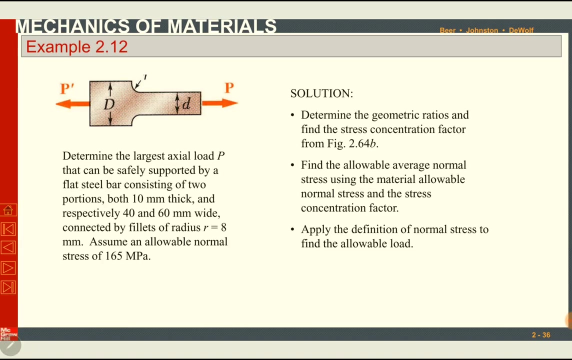 will have to use minimum area so that stresses maximum. there are two areas here. one is this one and the other one is on this side. we have to use the minimum one to get the maximum stress. okay, here is an example problem- example 2.12- where a plate with two fillets is given. determine the. 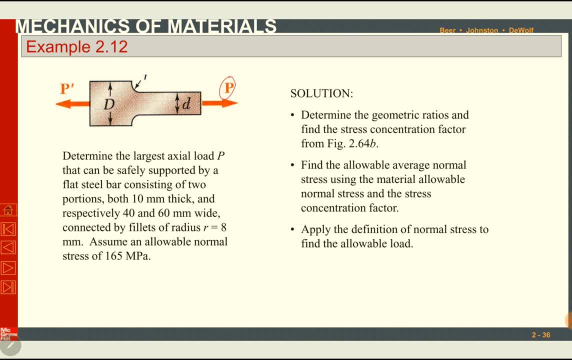 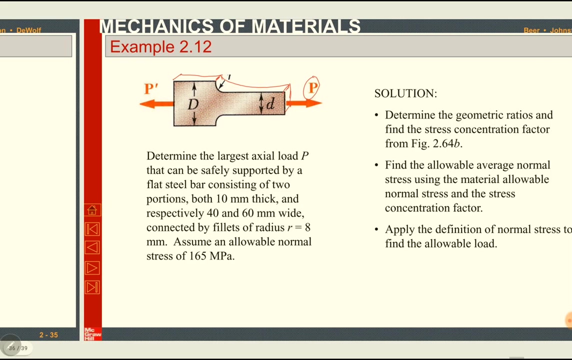 largest axial load, P, that can be safely supported by a flat steel bar, which is given in the figure, consisting of two portions, both 10 mm thick. for this bar, which has two portions, one with the larger width, capital D, and the other with smaller width, small d, it has a thickness of 10. 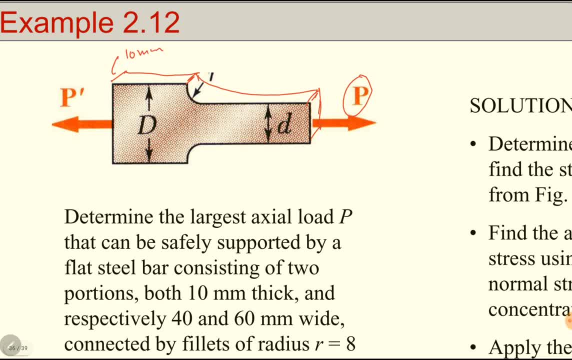 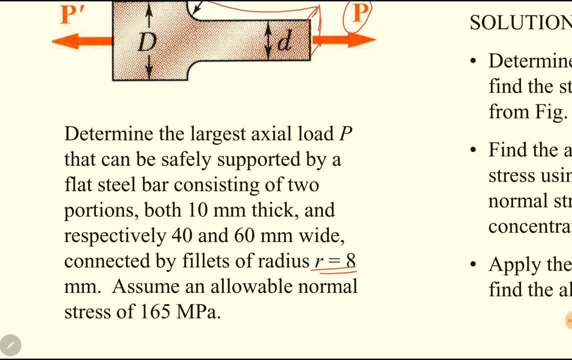 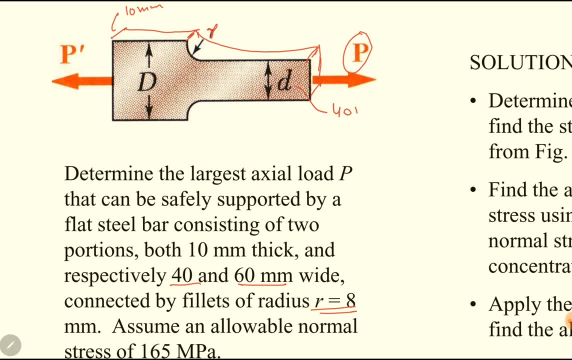 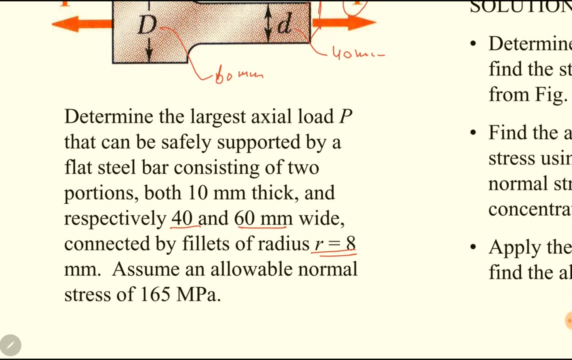 mm for both the portions. radius R is 8 mm, okay, 40 and 60 mm wide. the small d is 40 mm and capital D is 60 mm. assume an allowable normal stress of Sigma allowable R Sigma maximum allowable is: maximum is 165 megapascal. it. 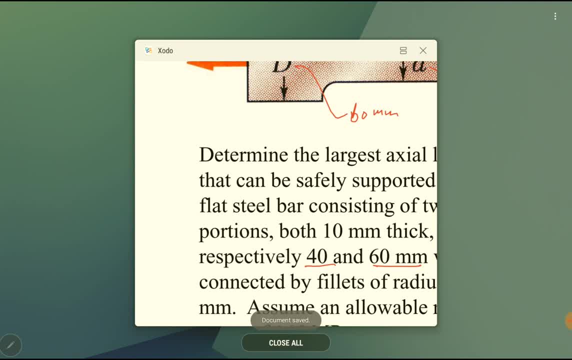 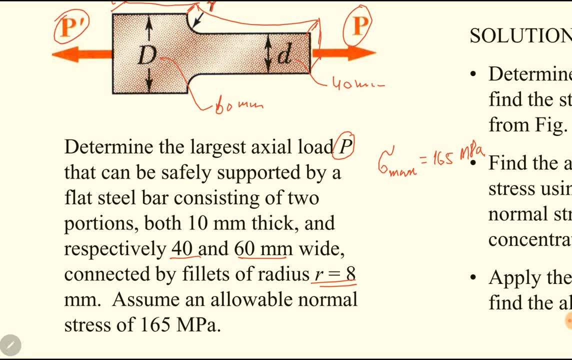 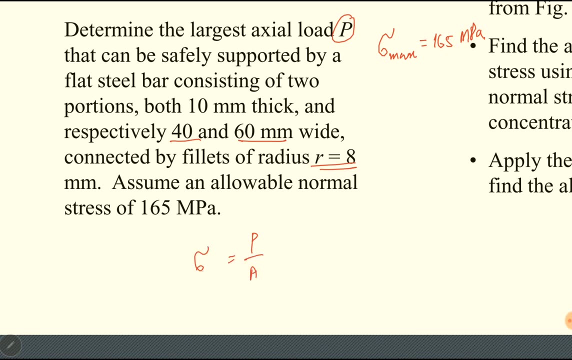 is given to us, in this case, what we have to find: largest axial load, P. how can we find P? P can be calculated from the average stress. okay, from the average stress we can find P, but how we will find every stress? every stress will be calculated from this expression. maximum divided by average is equal to K Sigma maximum. 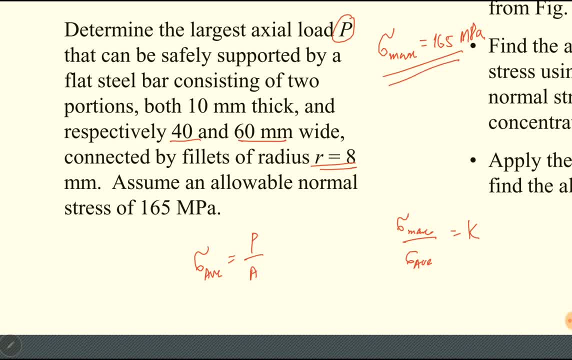 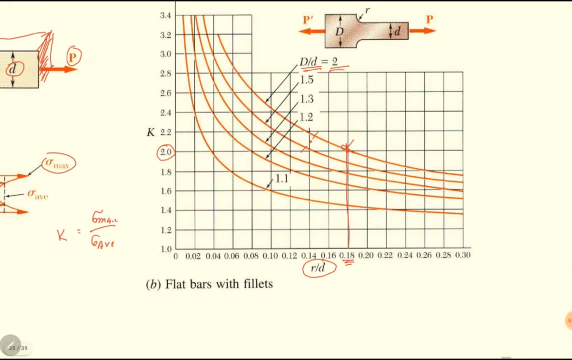 is given to us. K can be found from the tables, from the- sorry- from the chart given charts. so K will be known from the chart maximum stress is given to us. we can find Sigma average and from Sigma average we can find P. okay, so the next task is to find K. for K, we need small R or small d ratio and capital D. 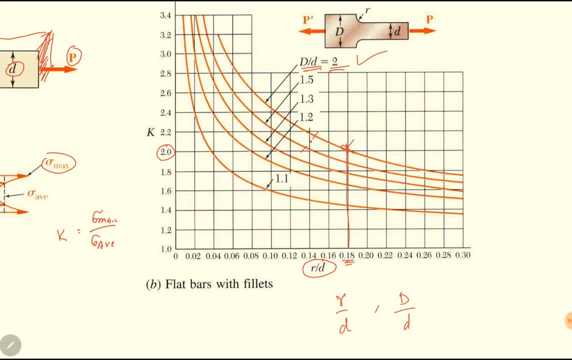 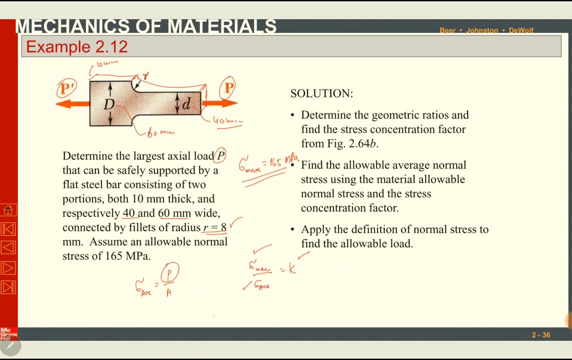 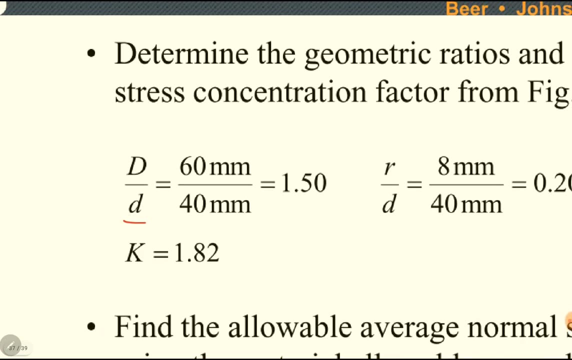 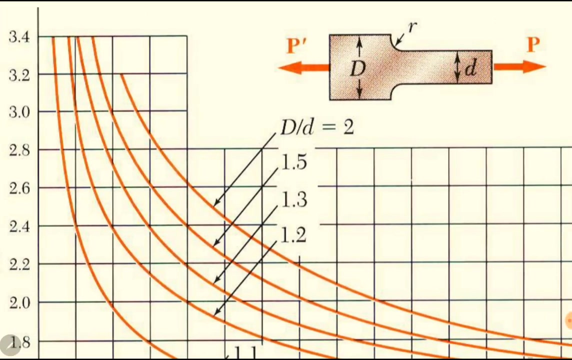 or small d ratios. small R is 40 mm, sorry. small R is 8 mm, small d is 40 mm and capital D is 60 mm. here we will find ratios. capital D over small d is 1.5 and R over D is 0.2. the going to the chart: 0.2 and 1.5. 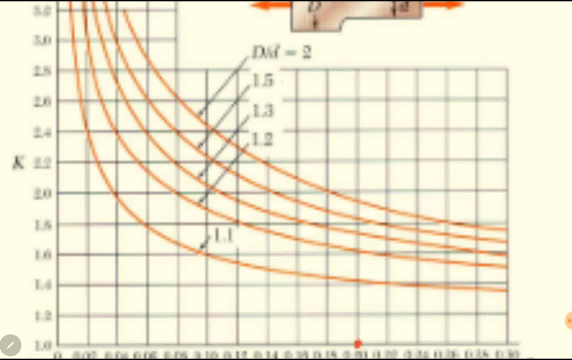 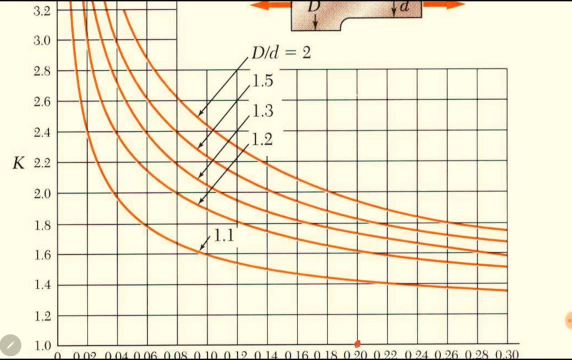 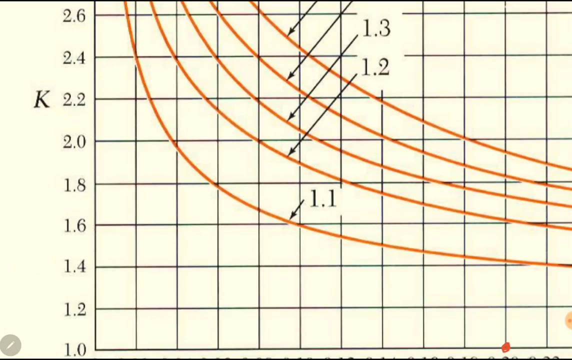 here is 0.2 and we have to use the chart of 0.5, this one, this chart, this line is here by extending this one here. if you have ruler on the paper you can see this is almost 8.2. approximation should be. approximation should be near to the value given on the chart. 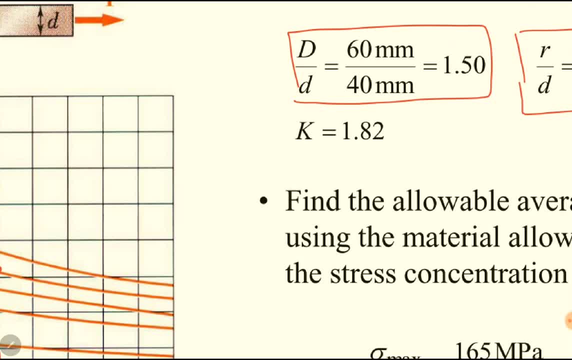 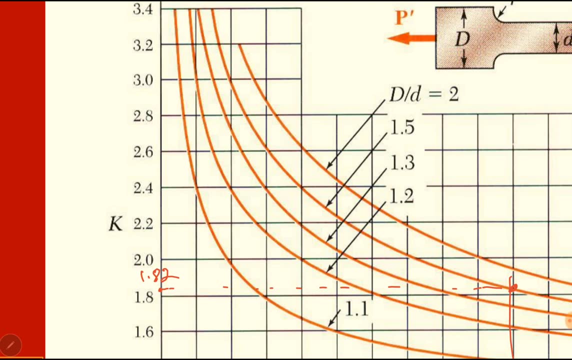 so that I said before about how can we find MIN chart. it is almost 1.82. some people may think like it is 1.83 or 1.81. that is also correct. so k is equal to 1.82. you cannot just assume it as 2 or less than 1.8. it is something between. 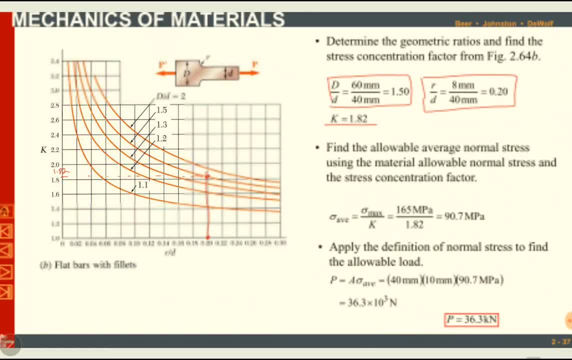 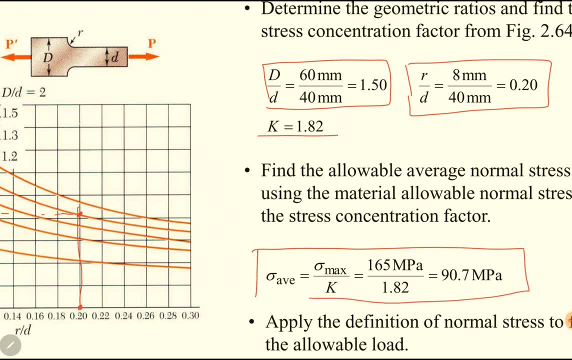 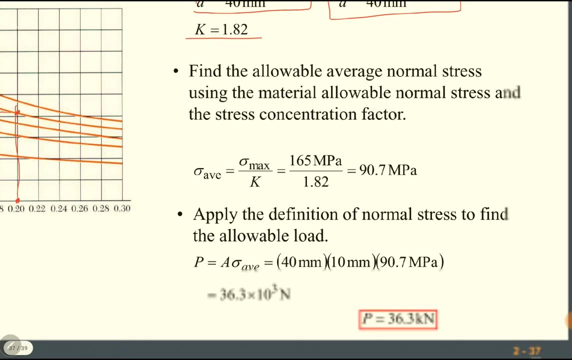 1.8 and 2 and it is near like 1.82. k is 1.82. sigma maximum is given to us, so by using this expression we can find sigma average, which is 90.7 megapascal. now p is equal to p over area is equal to sigma average. 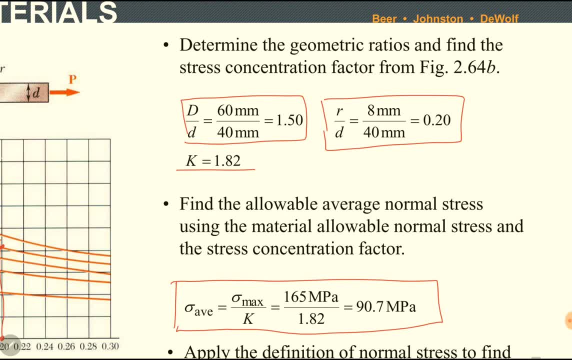 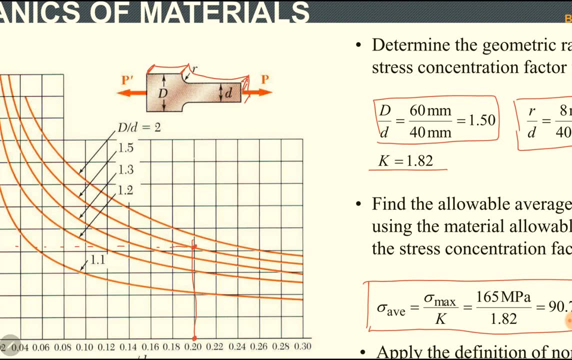 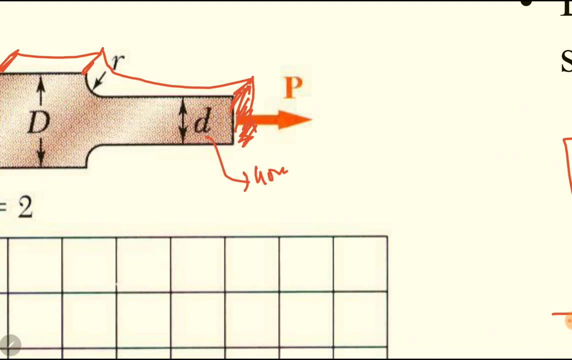 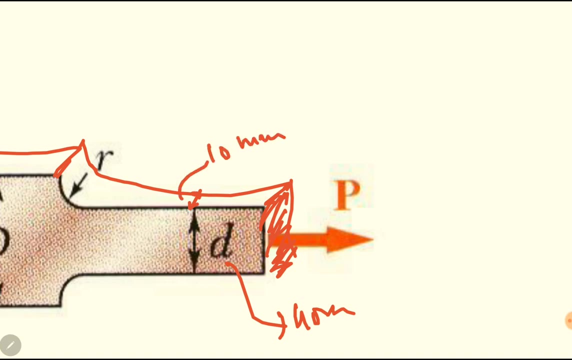 as discussed earlier, i have told you that we have to use the smaller area, this one. so this part of the plate has a width of 40 mm and thickness is given to us which is 10 mm, given the problem. so area is 40 into 10. we will not use this thickness. 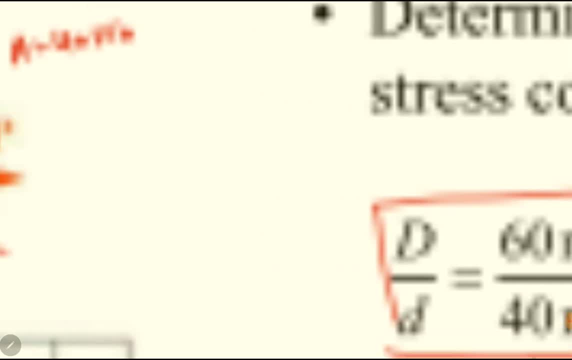 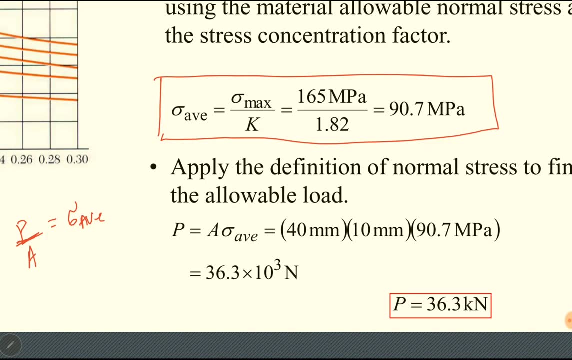 we will use the smaller area because with the smaller area stresses are maximum, which is important. maximum stress is always important. so area is 40 into 10. sigma average has been calculated as 90.7 from the previous expression occurring. the value is: p is equal. 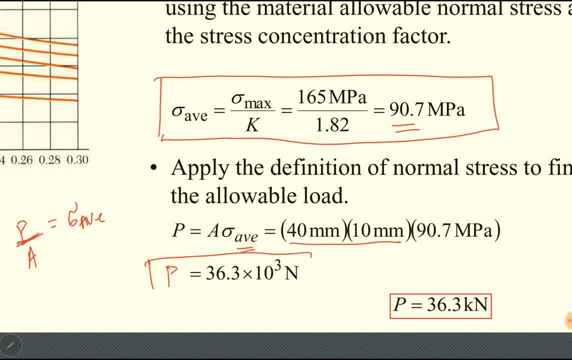 to 36.3 into 10 powers 3 Newtons. remember that 90.7 into 10 power 6 Pascal has to be used- sorry if it has been mega Pascal and length as in millimeter. you can directly use them, either convert the length and my. 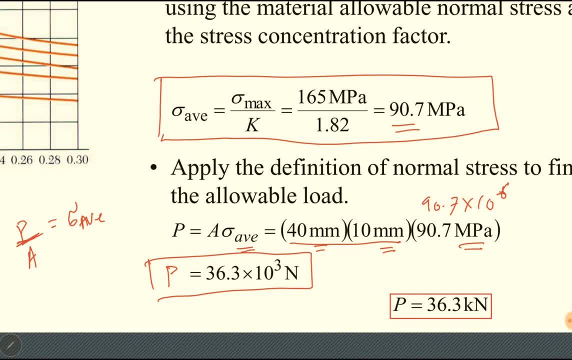 mega Pascal length into meters. meters and stressed into Pascals are u stress in media Pascal length in millimeters. so P becomes 36.3 kilonewtons. it was very easy, just you have to find the correct value of K and use the expression of K Sigma maximum. 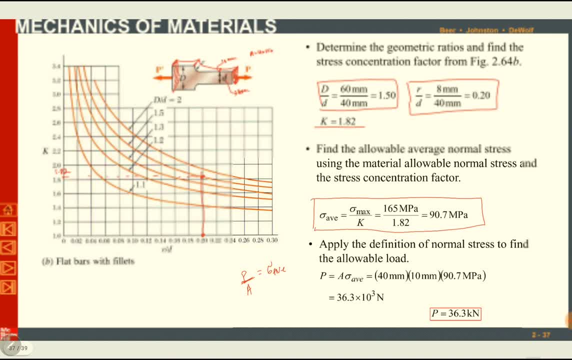 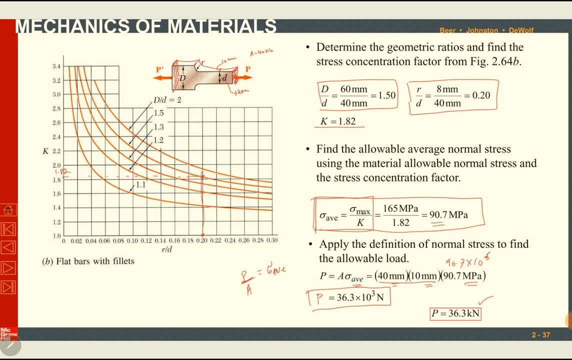 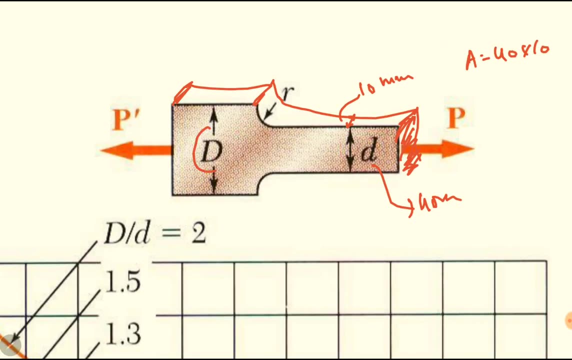 and Sigma average. okay, we will move. there are many other problems on this topic in the exercise of the book I recommend you to use to solve some of the problems. even there is. there are some problems, example problems and exercise problems- where there will be a configuration having both whole and the 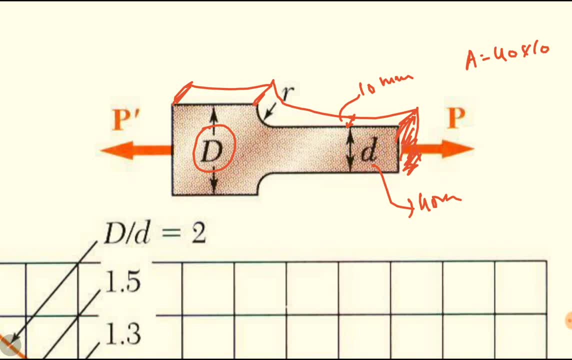 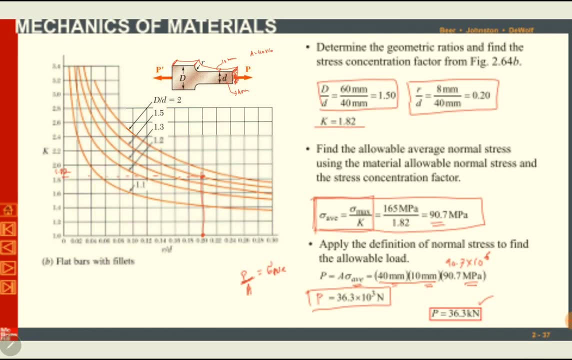 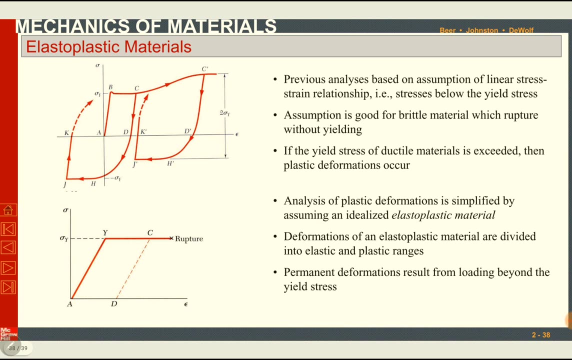 fillets. so I have solved one of such kind of problem in the exercise in a separate lecture. you can see that lecture. okay, another top. the next topic is elasto-plastic materials. up till now we have discussed about elastic behavior of a material and then in the slant. 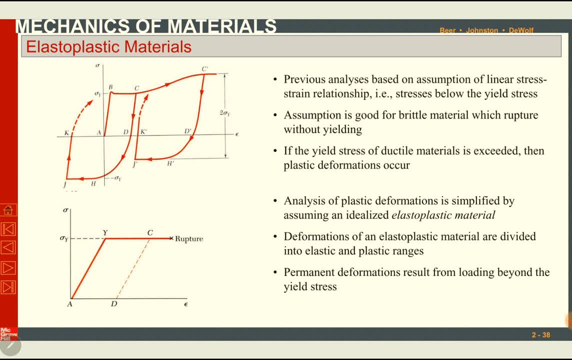 diagram. you have also discussed about plasticity. are the permanent deformation okay up till now in our example problems and the recent topics we have discussed about linear stress-strain relationship. are the elastic behavior. the elasticity are the elastic behavior is good enough for brittle materials, but there is no brittle. 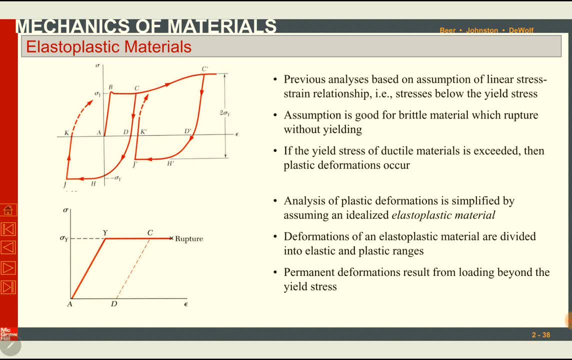 materials do not undergo the permanent deformation and they do not undergo yielding. if the use stress of a tactile material is exceeded, the plastic deformation occurs. in the brittle materials there is no yield limit on yield stress and the Britain were and the tactile materials. if we cross the 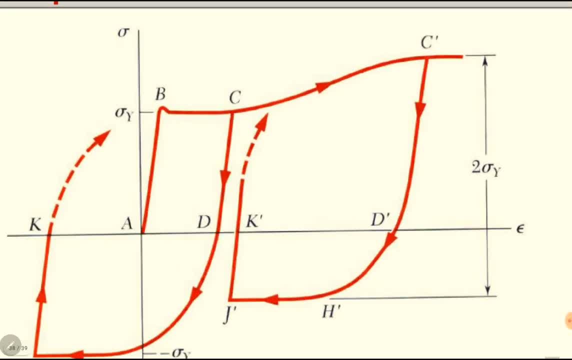 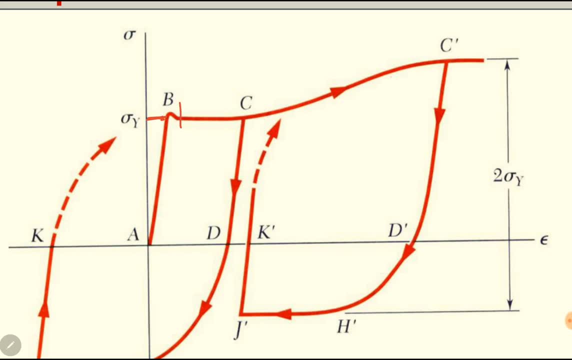 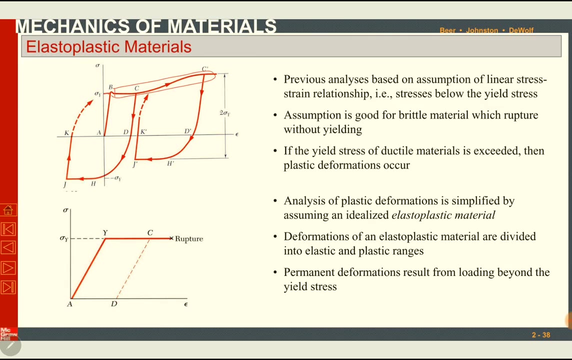 yield limit, the material will be permanently deformed, just like here. here's a yield limit at point B, and if the stress increases, we will enter into a plastic region. this one material will be permanently deformed. in our analysis of plastic, deformation is simplified by assuming an idealized elastoplastic material. 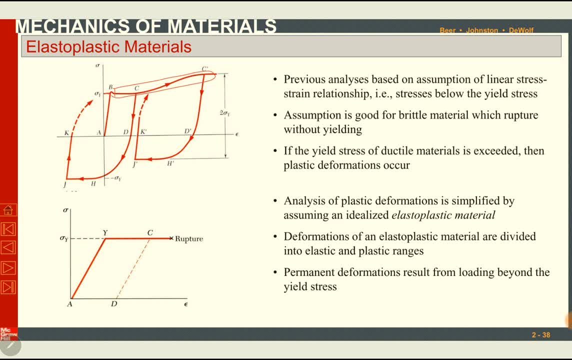 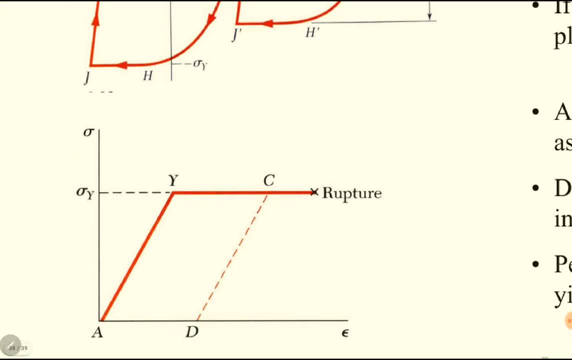 Deformations of an elastoplastic material are divided into elastic and plastic range, and permanent deformations result from loading beyond the yield stress. Here is an assumption. this is a perfectly elastoplastic material. this is an assumption that material will undergo elastic deformation until yield strength and if we remove the 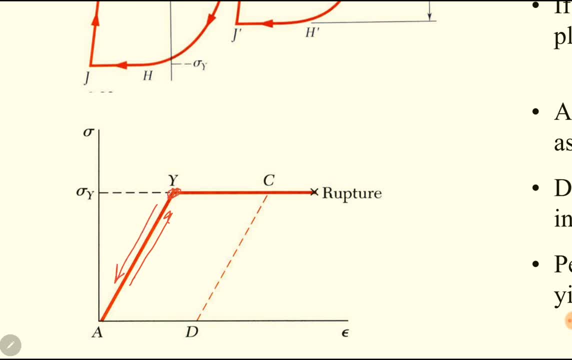 load it will return to its original position After yielding. it will be permanently deformed. there will be no point of return. it may return, but it will not return to zero strain. there will be some permanent strain, which is indicated here In a perfectly elastoplastic material. we do not. 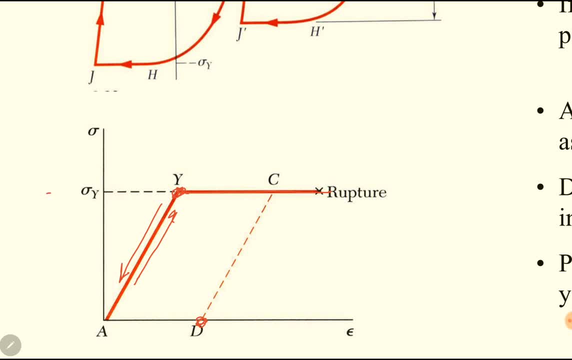 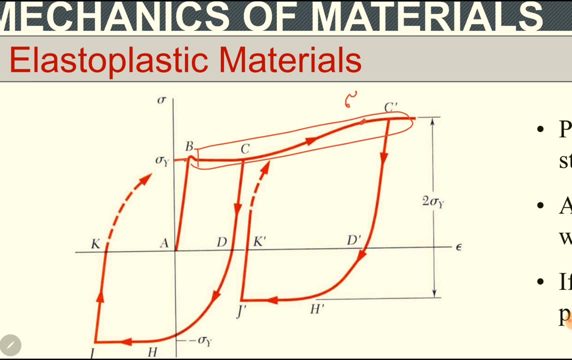 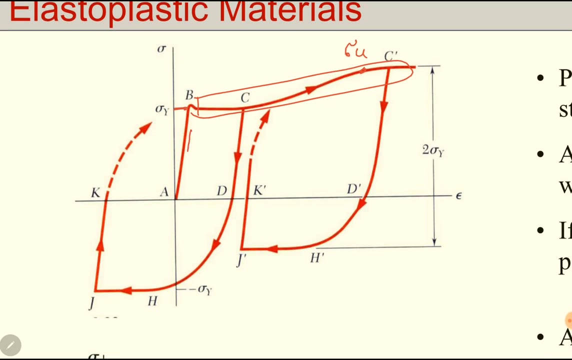 go beyond yield strength. so we have flattened the curve at yield strength, but actually they go above the yield. there is an ultimate strength or ultimate limit. If we unload a material within the elastic limit it will return to zero. but from a plastic region, like at point C, which is in plastic region, if we unload a material it will return. 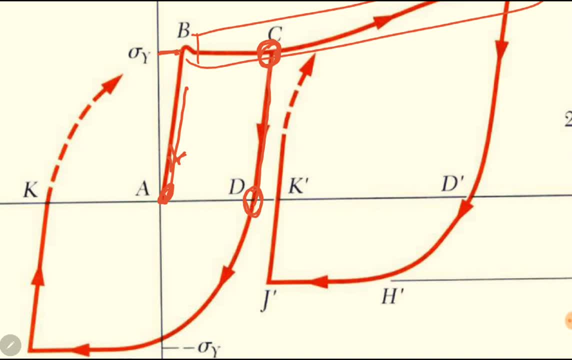 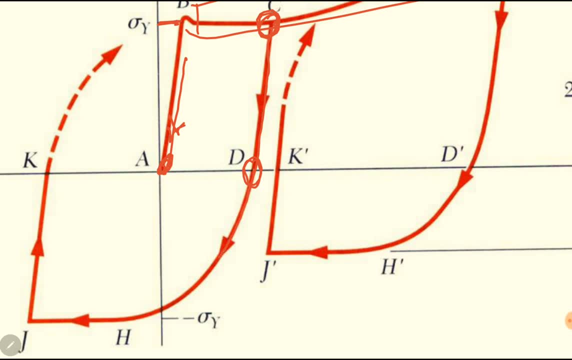 to a non-zero strain At point D and if we further apply a reverse load compression on it, it will undergo negative compression, negative stress. it will be a negative stress. Upon further loading it will be negative strain again if we apply a positive load. 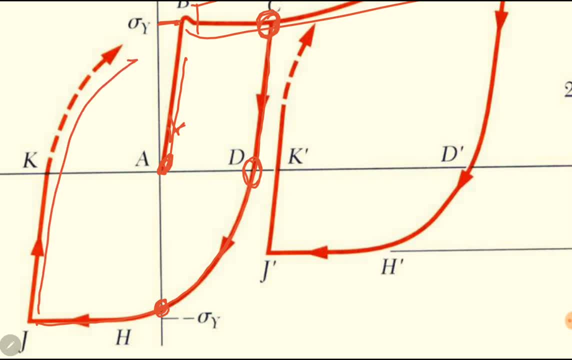 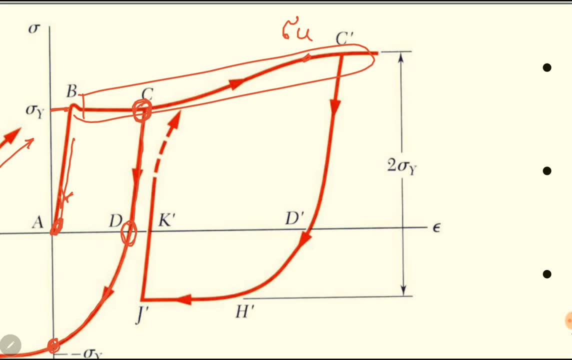 or positive stress, there will be tension. Similarly, if we un-stress a material or apply a reverse load from any point in the plastic region, it will return. there will be non-zero strain upon compression. there will be negative stress and negative strain and from any negative stress and negative strain region again applying. 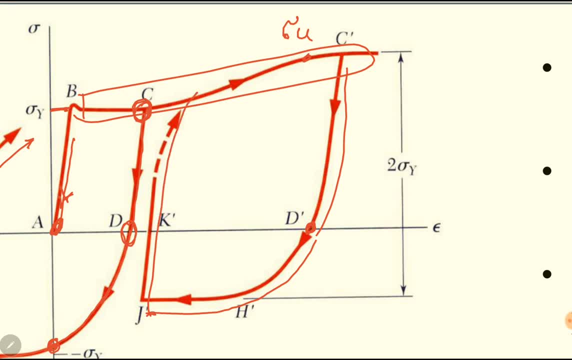 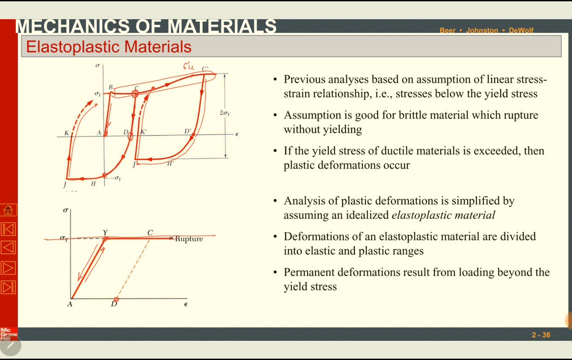 tensile load it will again follow the same curve, it will touch it here. so this is elasto plastic behaviour of a material. by unloading a material from the plastic region it will return to some positive strain point. it cannot return to initial position. and if we apply, 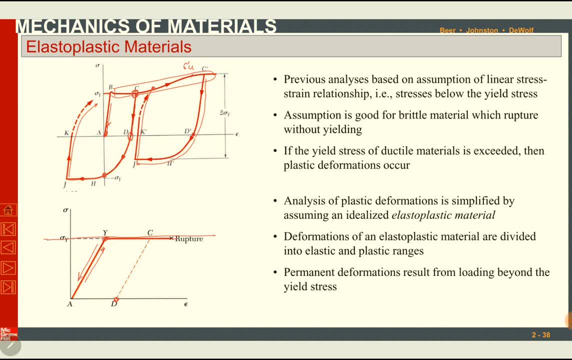 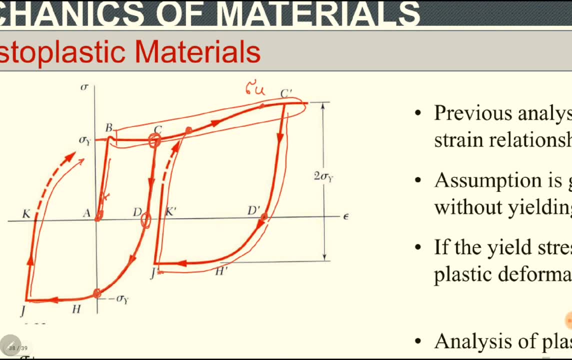 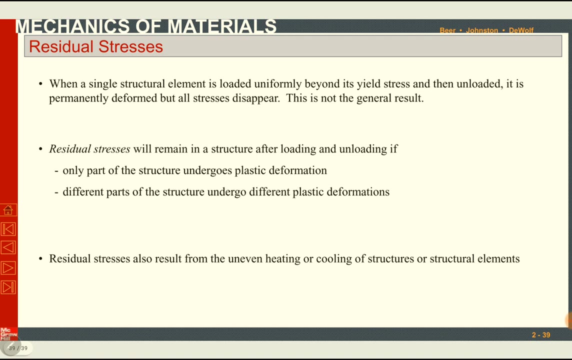 reverse load, compressive load- there will be negative strain and negative stresses. upon applying tensile load again, it will follow the same value of e and it will touch the curve, the initial curve, somewhere in the plastic region. the next topic, and the last one, is residual stresses. 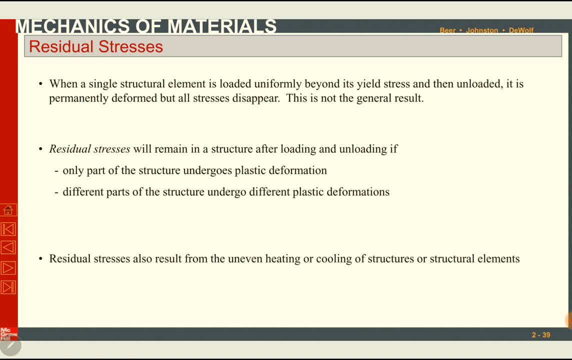 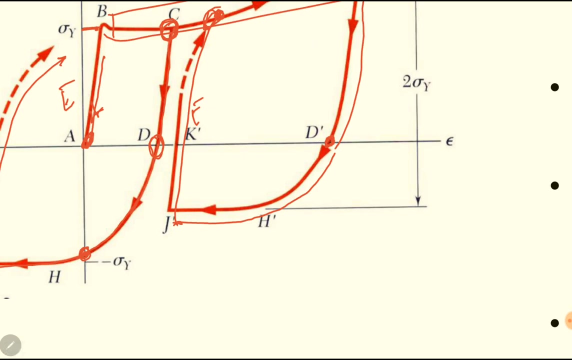 residual stress is a permanent stress. when we apply reverse loading on a material, or if we apply or if we relax a material from the plastic region, it will recover but it will not return to its initial position. there will be some permanent strain in the material, just like at point D or point D' we have shown that materials have returned. 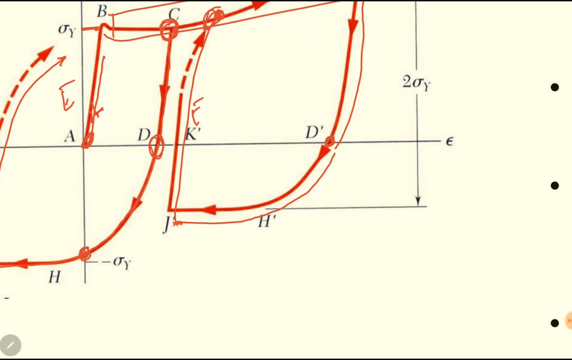 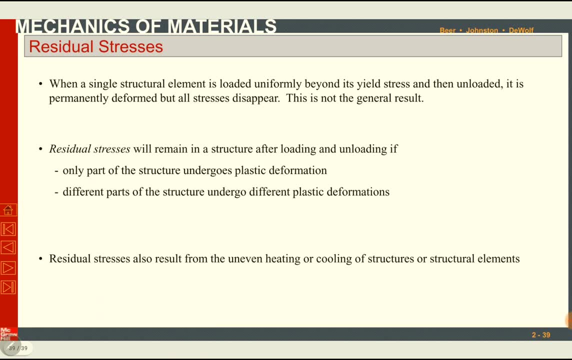 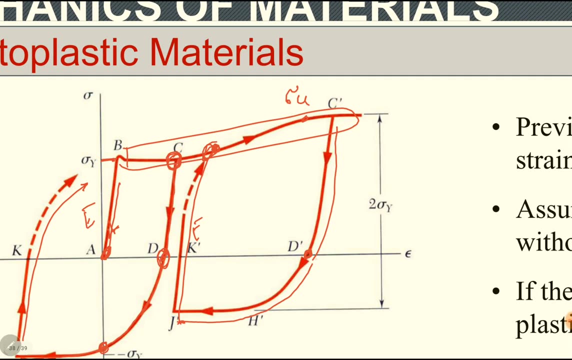 but there is some permanent strain in the material, permanent deformation in the material. due to this permanent deformation. although we have removed the applied load at point D and point D' we can see that the value of stress is zero because it lies on the horizontal axis. 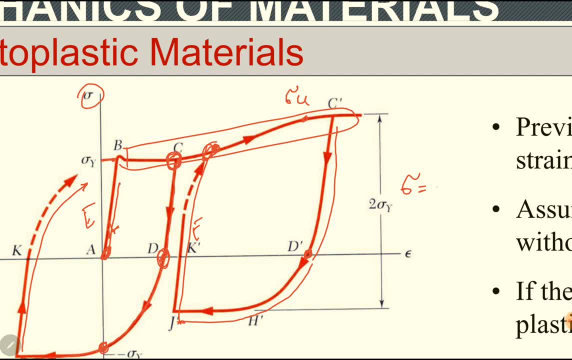 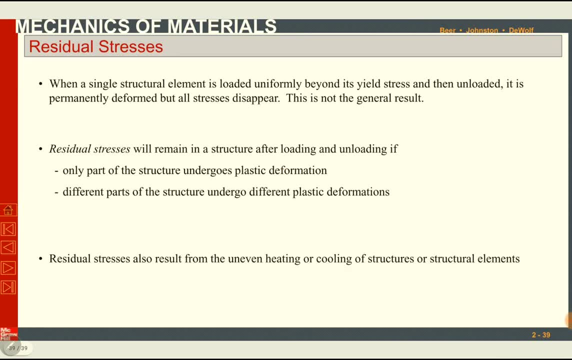 stress is on the vertical axis. so there is no stress because load is zero. there is no applied stress. but since there is some permanent deformation, so there must be some permanent stress in the material which remains forever, and this stress is called residual stress. so when a single structure element is loaded uniformly beyond its yield stress, 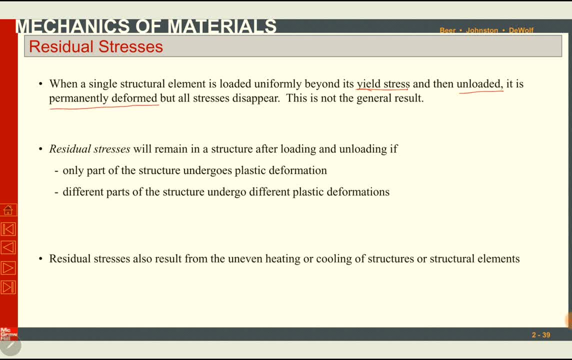 and then unloaded. it is permanently deformed, but all stresses disappear. this is not the general result. in the stress-strain diagram we can see that if a material is unloaded from its plastic region, it will return to a zero stress state. there is permanent strain but no stress, because stress is on the vertical axis.